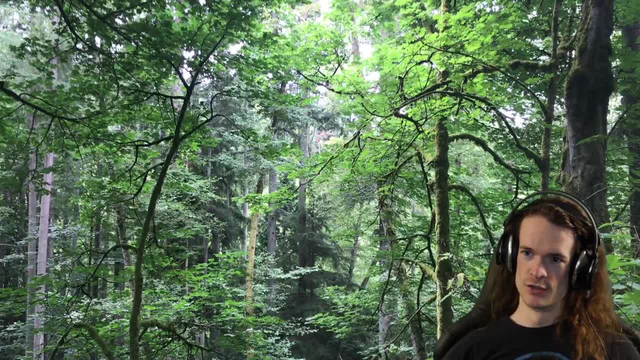 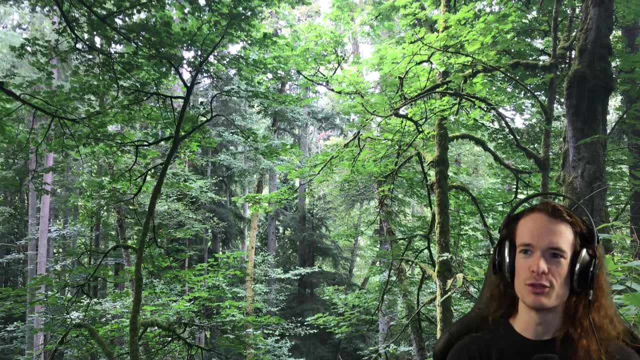 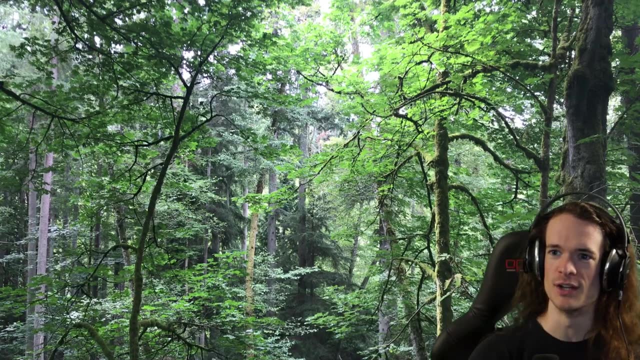 Ladies and gentlemen, welcome to another episode of The Voice of Neuro. We are back, for the second ever math lecture available on YouTube and in podcast form, with none other than Brett the legend. What is up, Brett? Hello Neuro. Thanks for the introduction. 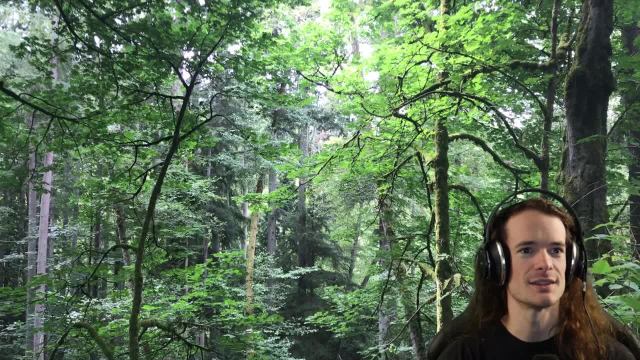 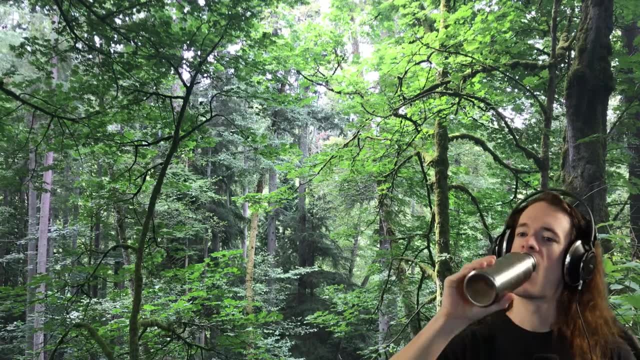 You're welcome. It's good to have you. I'm thinking that this time you're going to give us a little bit of wisdom about logic. Is that true? Yeah, So we were talking last time about how the point of this is to. one of the benefits of this is to help people think carefully. 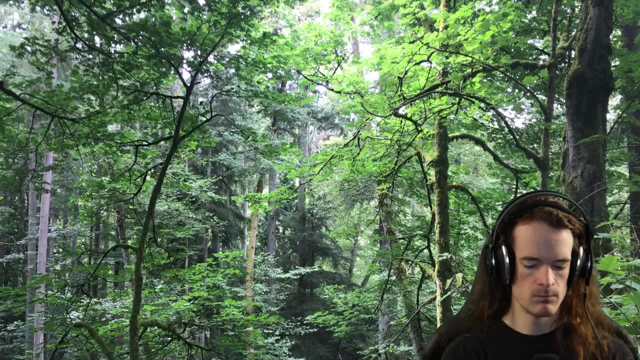 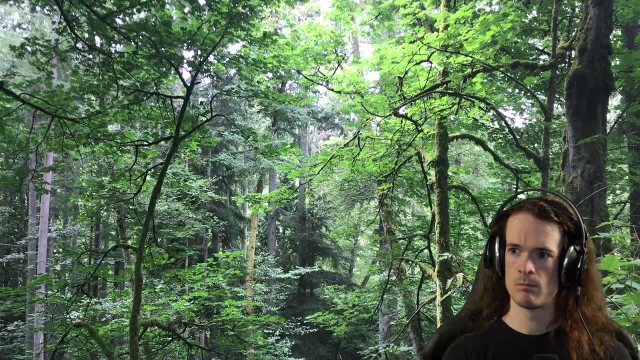 If they're doing philosophy, if they're thinking about current events or if they're applying it to technical things or even to the games they play. So logic is a good place to start, with no prerequisites, to help people think more carefully and rigorously about ideas. 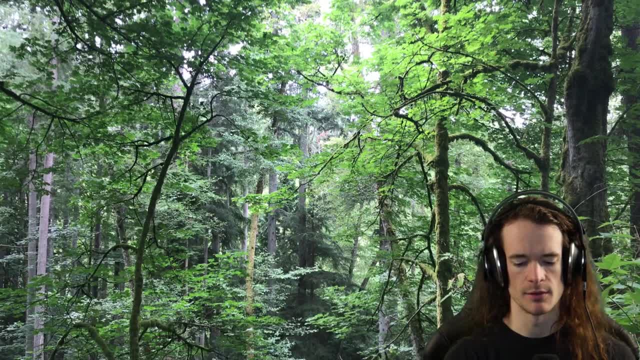 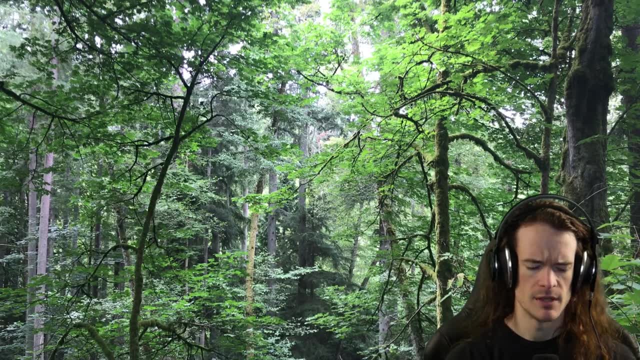 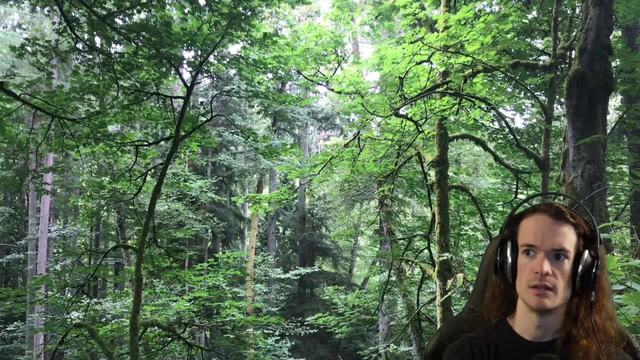 Yeah, we talked in the first discussion about the practicality of math and how. that's one of the the main shortcomings and pitfalls of a lot of math education that people receive is they don't really get shown why it's cool and where you can apply it in daily life. 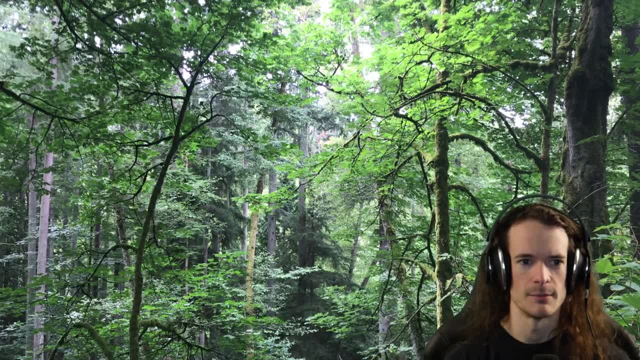 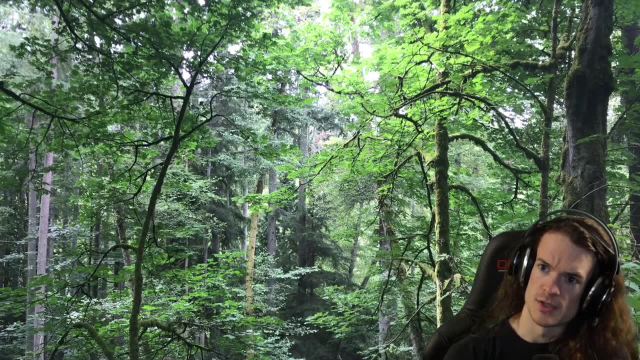 They think, oh well, this particular formula is never going to come up in my line of work. Therefore, I'm just going to half-ass this class as much as I can, rather than thinking about how the structures of mathematics apply to even things such as basic conversation that you have with your friends. 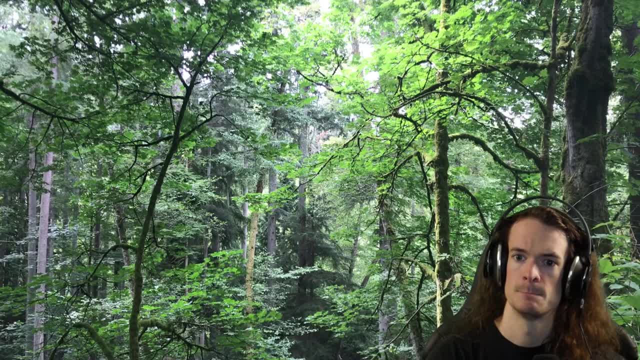 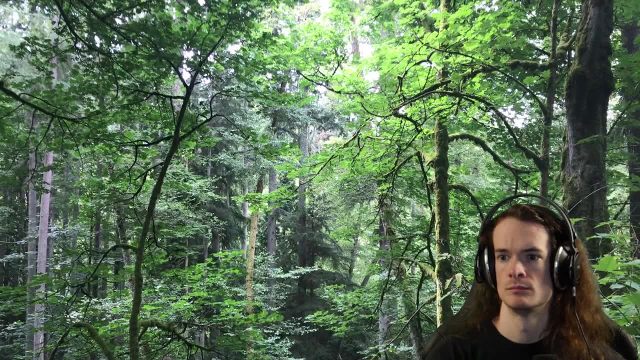 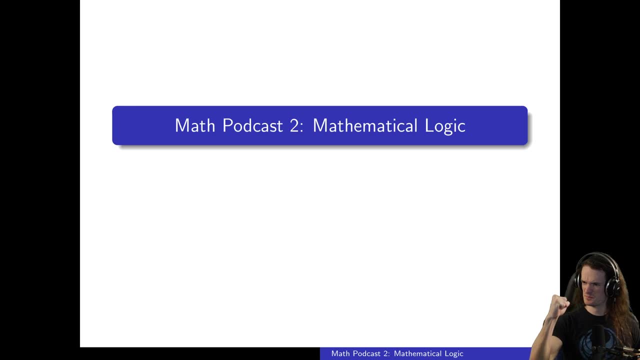 Yeah, And speaking of the conversation, some of the topics of the logical statements we'll be using for this lecture will come from the games you play. So there'll be some StarCraft II sentences and examples, maybe some World of Warcraft examples with your favorite character, Brunt the Tauren, strong warrior. 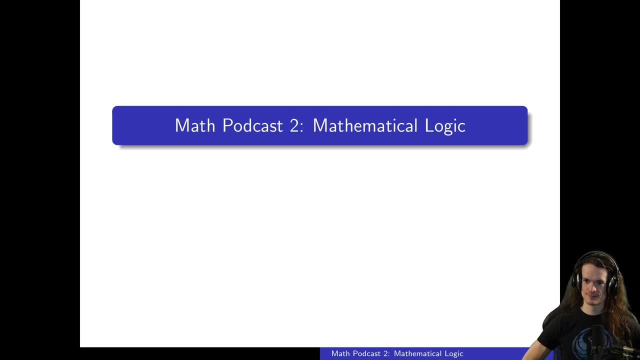 So he'll come up. So we'll try to integrate some of the games you play into the into the top, into the math. we do Also, and this is not the main reason for this, But if someone's interested in this, please feel free to contact me. 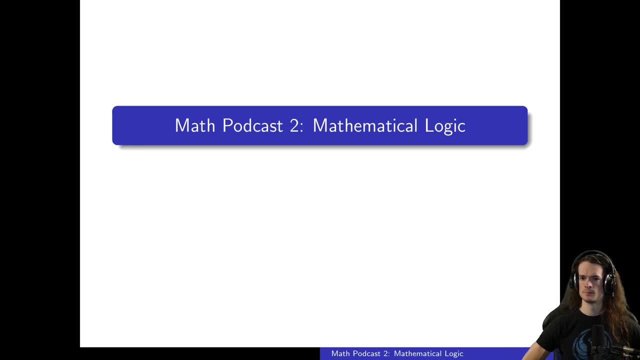 If someone happens to be interested in doing some kind of programming, or they do programming in their work or they're studying some kind of programming at school. logic certainly plays a role there and can help them directly. Sweet, So what you're saying is, with the power of mathematics, people can power themselves up IRL and get stronger and smarter. 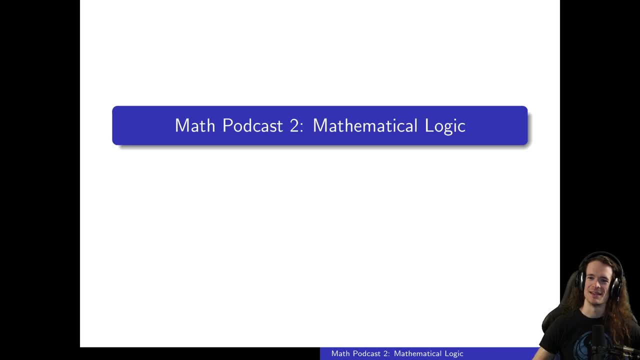 There's a possibility. Yeah, It may or may not happen. Find out on this episode of the math podcast. One Other disclaimer, just a heads up, is that the way I teach- and I've done this for throughout my life when I've taught university and elsewhere- is that I try to make the lectures very interactive, and the way this will work for this type of podcast YouTube setting is there will be a lot of examples that are posed as questions that will give a moment to think about, and then we'll talk about the answer and a chat. the live chat wants to chime in. 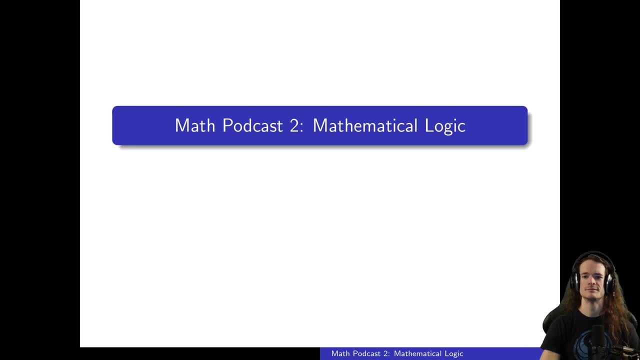 Please do so. We're love to hear Your responses to these questions and if, at home, if you're watching on YouTube or listening to the podcast, pausing during those times, if you want to take a little more time to think about them, it's fine too, or not, totally up to you, but there will be moments like that we'll. we'll be looking at questions and then thinking about the answer and trying to discuss why the answer is what it is. 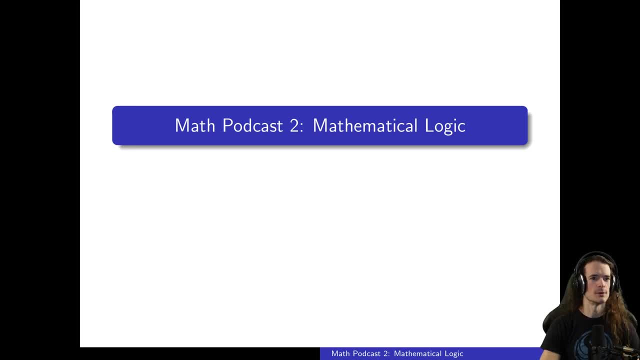 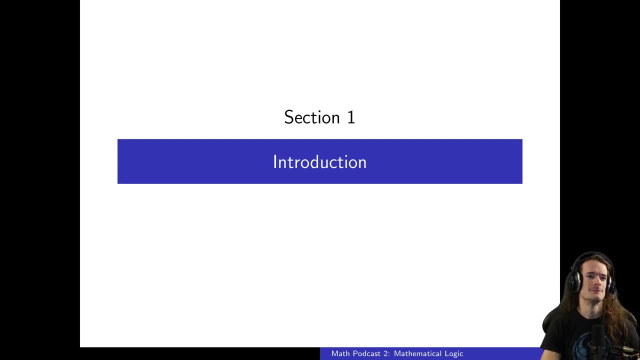 Fantastic, Strap yourselves in. we're about to get going. Section one, Introduction: Wow, All right, so I'll try to keep in sync with you. All right, so, Without further ado, here's the introduction. So we're going to start off. you had those bullets. That was good. That is the introduction. 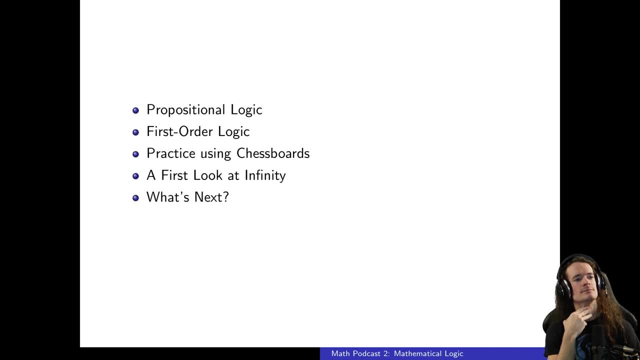 So the logic we're going to talk about is divided up into a few parts. Basically, let's first talk about what is called fancy names. you'll see that they're actually not so fancy when we get to them. It's propositional logic. 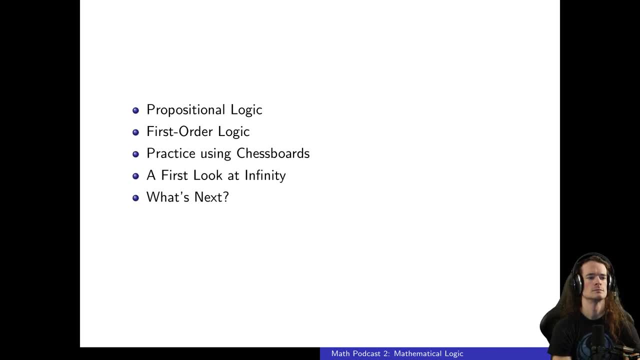 Which is Basic statements, Things that are true or false, and then how to put statements together like this and that or this or that. So we'll be talking about these simple things. Once we're done with the propositional logic, we'll start talking about first order logic. 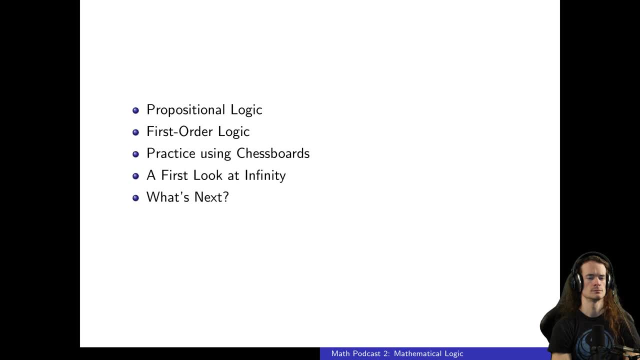 Which lets us say things like something is true for all things or there is a thing. So that'll really help us make more statements and more interesting statements. I think Then we're going to have some practice to see if we've understood the first order logic using chess boards. 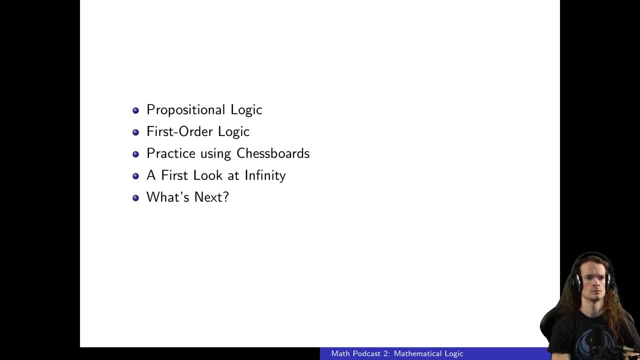 And if we have time, we'll even think, start thinking about some examples of infinite things, and talking about infinity And the various dilemmas surrounding infinity might be an interesting topic for future podcasts, And we're always looking for suggestions for future podcasts. So 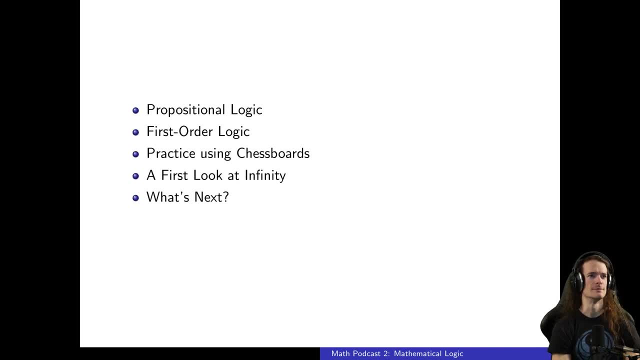 Please let us know. Have at me First order logic, not going to lie. first thing I thought was Star Wars- Is this like Empire or Sith? first order and what their take is on logic. That's exactly right. Oh, it is Nice. 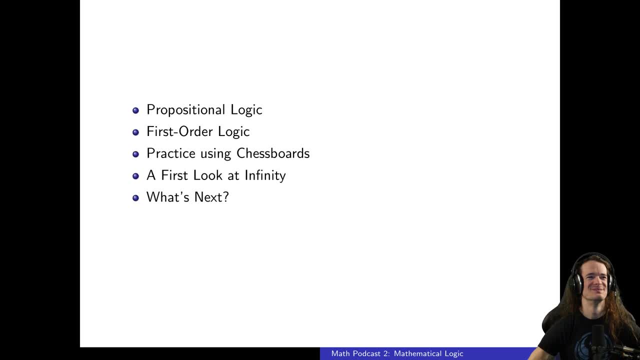 No, no, it's not No, no. First. yeah Well, I don't want to spoil it. We'll get to first order logic soon. As you see, it's the second topic. It'll be here before you know it. 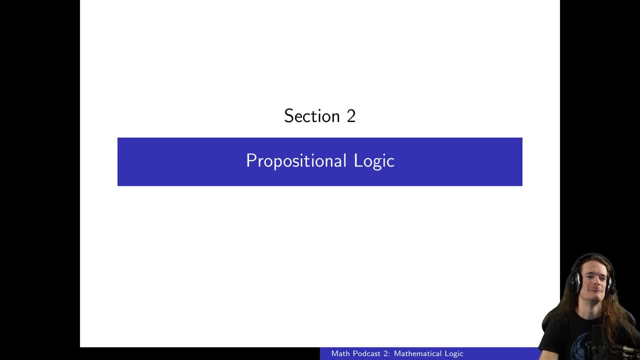 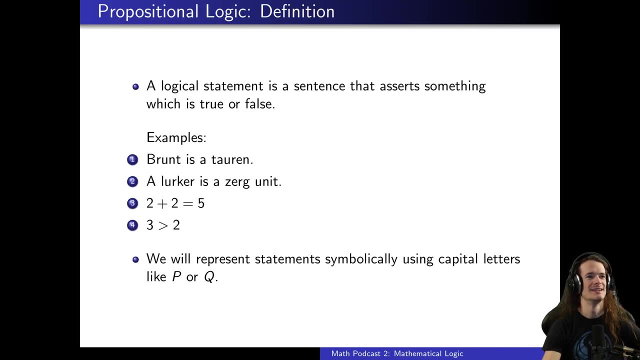 We're going to do them in order, then Propositional logic, Okay Yeah, And then we're all Jedis here. No Sith stuff, All right. See, we're already at section two. This is moving too fast, All right. So the first thing we're going to talk about is a statement, And a statement is simply a sentence that asserts something that is true or false. 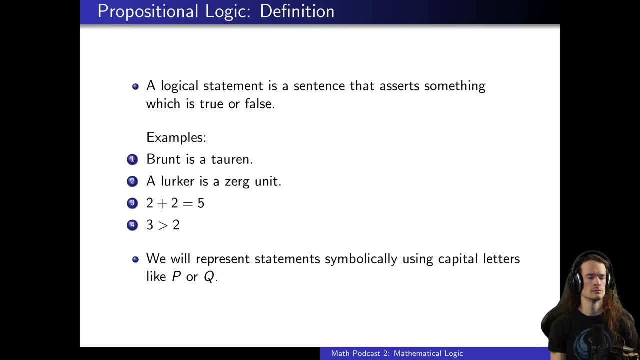 So an example of a statement would be: Brunt is a tauren, Brunt being the character that Nero plays in World of Warcraft And tauren being the. What is the right way to describe what a tauren is? Is that race or species? I'm not even sure. 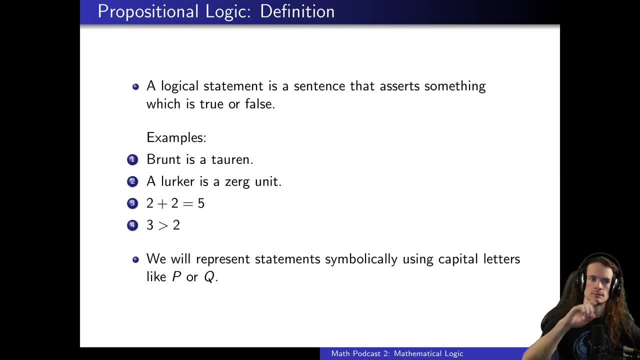 Yeah, you would say race or species, Both would be correct. All right, Then we also have a. lurker is a zerg unit. So lurker is an example of a unit from the zerg race in Starcraft, Another game Nero plays frequently on stream, as I'm sure all of your viewers know about. 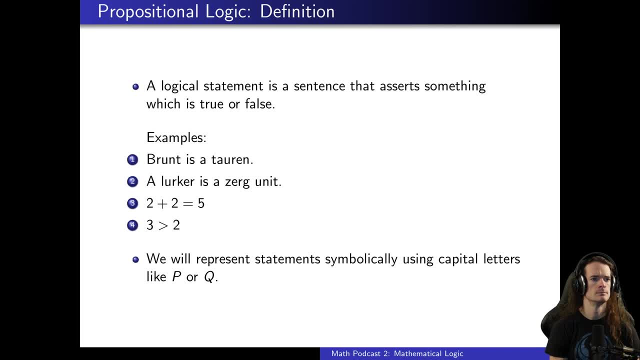 Some math examples. We have the statement two plus two equals five. That is a false statement, The quick maths you were describing earlier. We also have the statement three is greater than two, a true statement. So what makes these statements is that they are true or false. 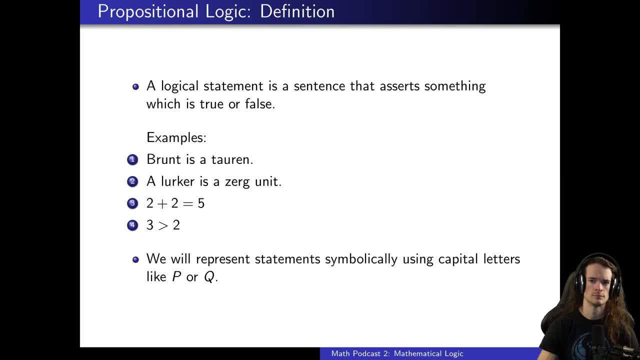 It's possible that in different universes, they might have different meanings, but they're always going to be true or false, And that's what makes them a statement, And we'll also, throughout, have a symbolic language for describing these statements and more complex expressions. 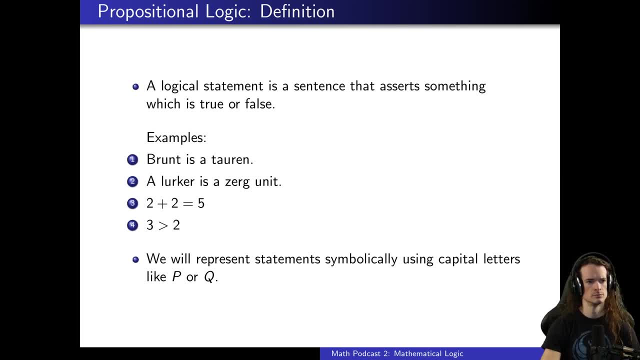 And whenever we talk about a statement- one of these things that can be true or false- we'll use a capital letter like P or Q. So statements are like the atoms, the base parts that we're going to use to build up the rest of our logic. 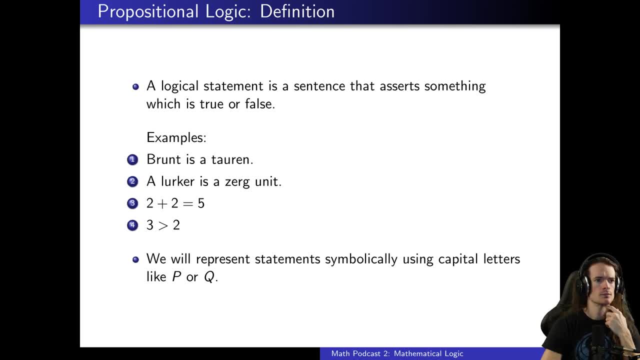 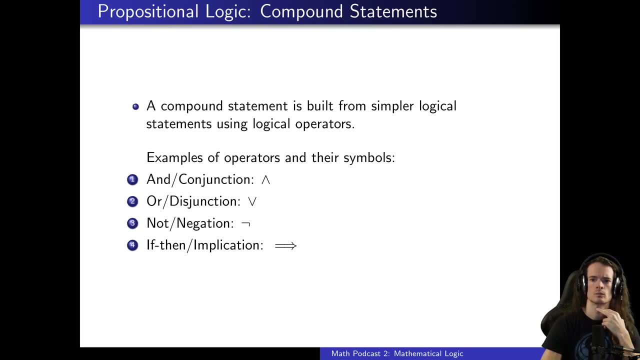 So we'll start with these things. that can be true or false, and then we'll make more complex things out of it. So let's get more complex. So on the next slide we show how to take simple statements and make them into more complex statements, called compound statements. 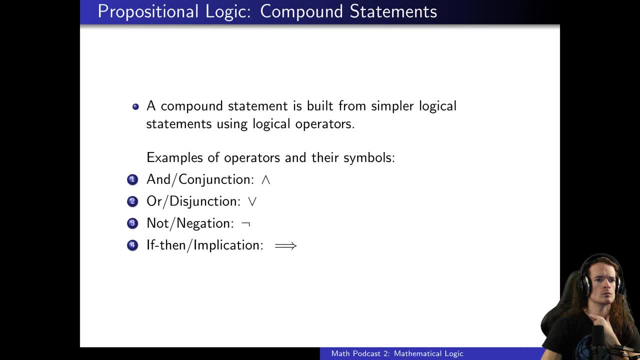 And the way you do this is by combining simple statements with these operators, So this is going to be very familiar to everyone that uses them in their daily language. the word and. So one thing is true and another thing is true, or or Not. a negation to negate something, to say something is false. 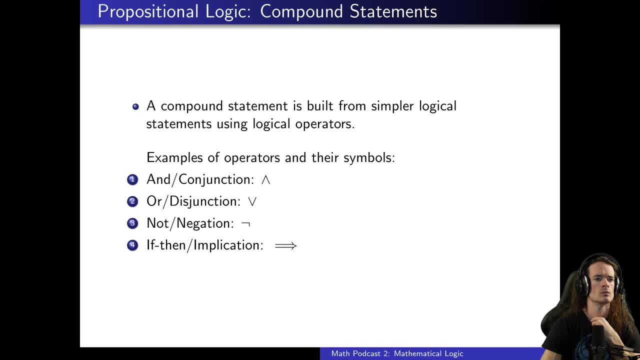 And then something like if, then if this is true, then that is true, Also called implying or implication, And so we're going to go through each of these four things separately, And each of these four things has a little symbol associated with it that we'll use in our symbolic logic. 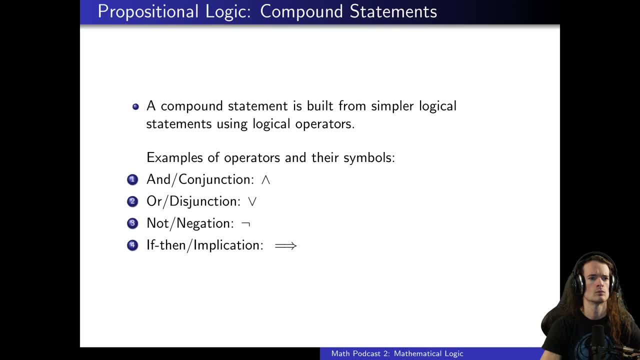 So for- and we use this upside down V symbol And for, or we use a V symbol For not. we use this like hook symbol. It's an Allen wrench. Ah yes, I guess Allen wrenches are for negating things. 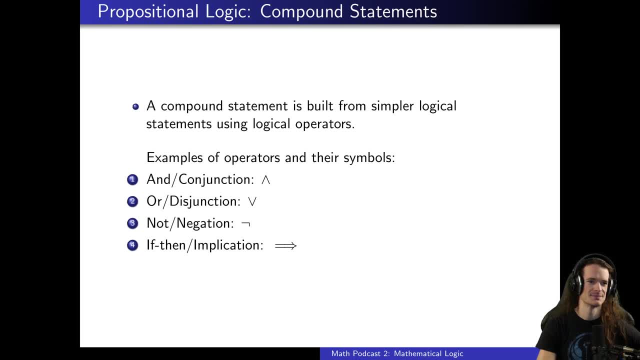 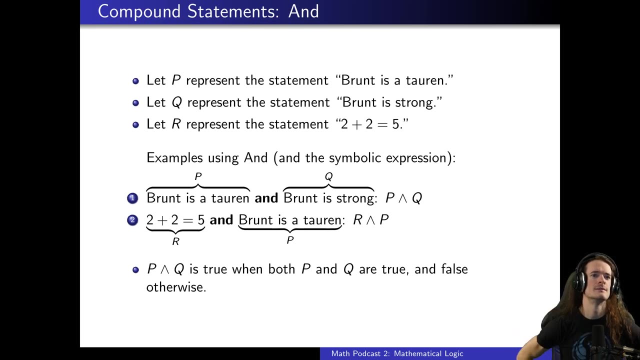 And then the right arrow for implying. So we have the double right arrow for this implication. but I like the double right arrow Kind of cool looking. So we have the double right arrow, So we should start to noise Great. So on the next slide we should be talking about and. 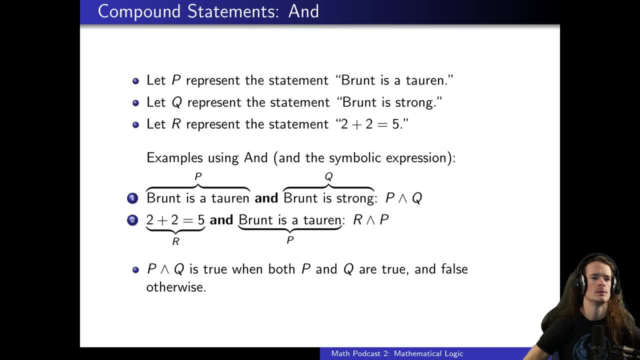 Start simple, So we'll let P represent the statement that brunt is a torrent- A true statement for those not familiar, but I'm sure almost everyone here is familiar with your wow escapades. And then Q will be the statement: brunt is strong, Also true. 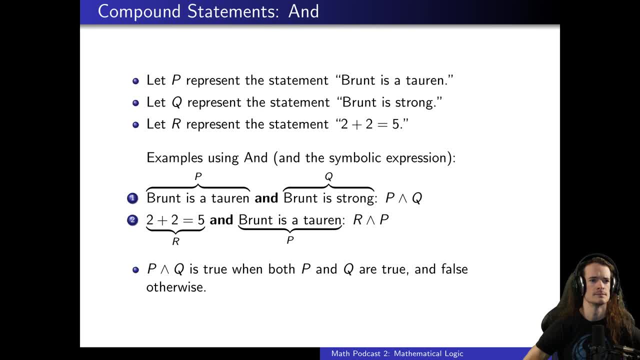 Don't want to disparage brunt And we'll let R represent the statement. two plus two equals five. That one's false. I did that just now. So an example would be to say: brunt is a torrent and brunt is strong. 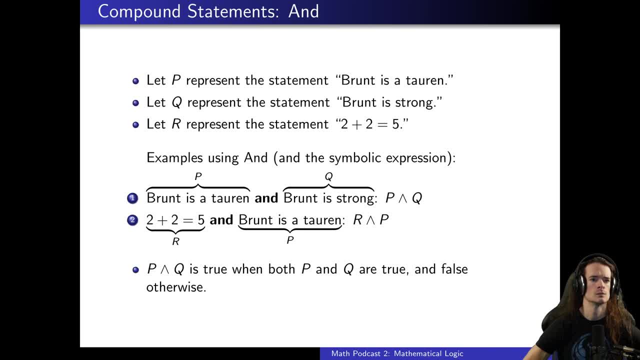 And that statement is true because both parts of it are true And we connected them with an and And we write this by saying P and then that upside down V symbol and then Q. So another statement, Another example of this compound statement. We can take the statement: two plus two equals five. 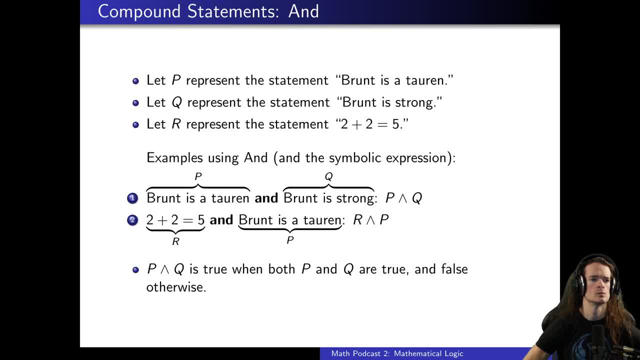 And then combine that using and with brunt is a torrent to get another statement: Two plus two equals five and brunt is a torrent And that is false because one of the parts is false. So, more generally, for a compound statement that uses and to be true, both parts have to be true. 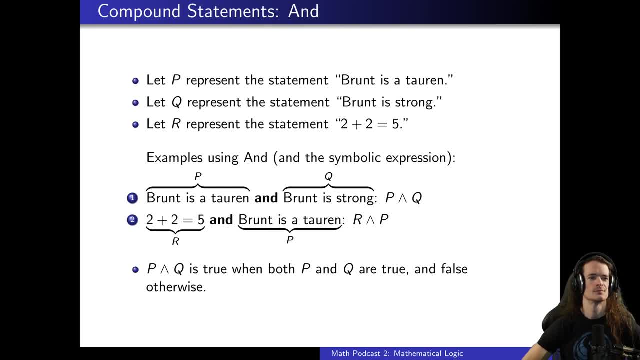 And otherwise it is false And that really lines up with the meaning of: and So far I think things are doing fine. It's a word that we use commonly and this is a way of making that nice and formal and clear for us. 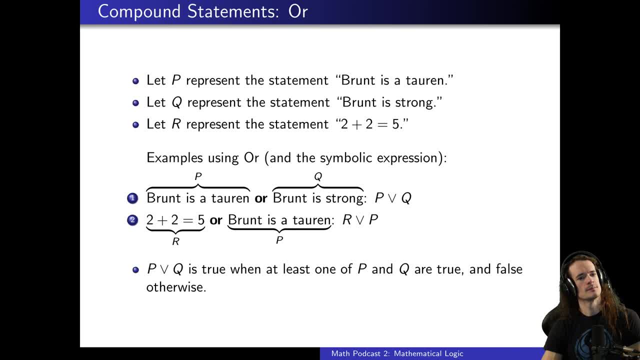 Yeah, And so chat can thank us for learning about. and I didn't know what and was, but then I watched a math lecture on Neuro's Twitch channel and now I know, Yeah, I learned this word and and I use it all the time. 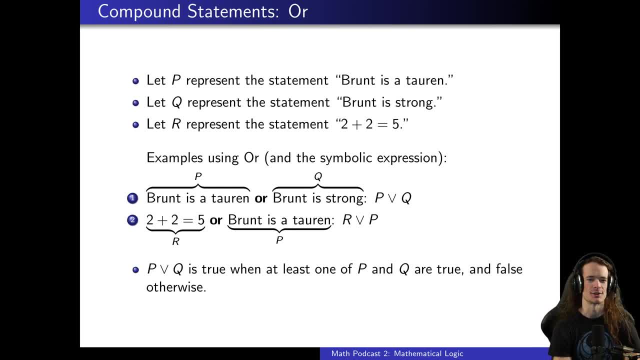 It's so useful. This is the most useful lecture ever. It is a great word of power. So now I'm going to use- or We're just going to cover- all the words. You're going to be so, so full of words. 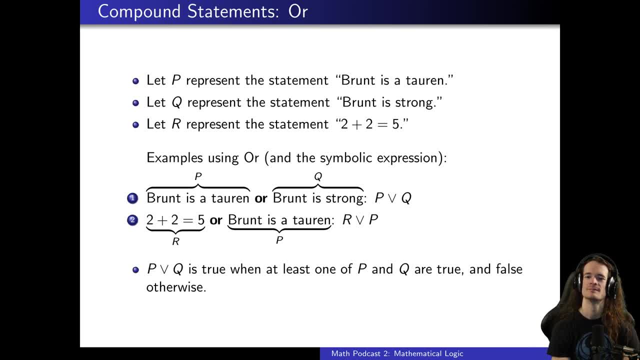 Yeah, So so we can do a similar statements that we had before, Like brunt is a torrent or brunt is strong, and both parts are true, So the or is true And we use this V looking symbol for or. So if P is brunt is a torrent and Q represents brunt is strong, 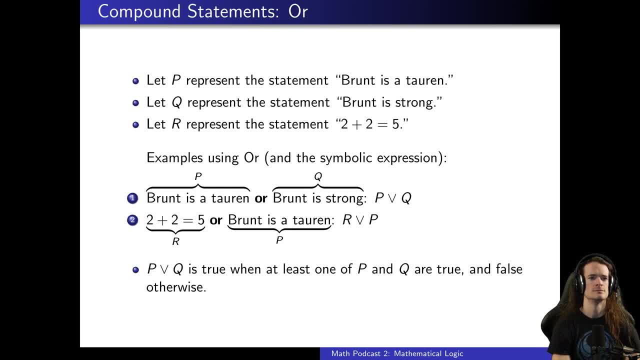 Then brunt is a torrent or brunt is strong, can be represented symbolically as P V, symbol Q. Similarly, we can have two plus two equals five, or brunt is a torrent, which is still true because it's, or, and we don't need both parts to be true. 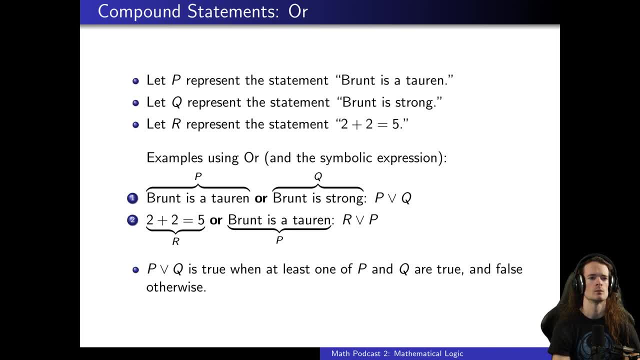 The one thing that makes mathematical logic sometimes a little different than English statements, where someone's trying to speak logically, is that when we say or, in math we always mean either or both, So at least one of them is true. It doesn't mean that one has to be true and not the other. 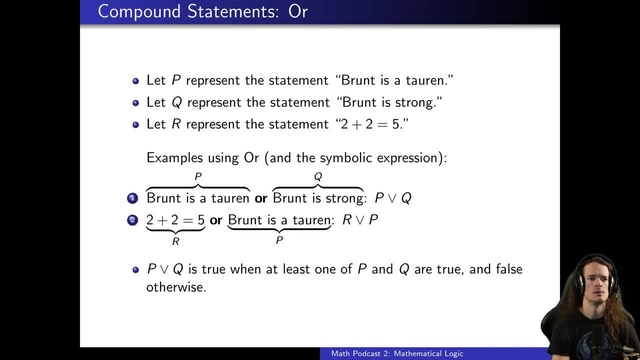 So, or, as they say, is always inclusive in mathematics. Yeah, I think in language it's oftentimes expecting the listener to choose one of them and that both is not an option. That ends up being a really interesting conversational tactic is the way that you frame questions, because you can frame a question in a way that leads someone in a certain direction or puts them into a trap or something like that, where oftentimes, when people give you an either or question, both may be the best answer. 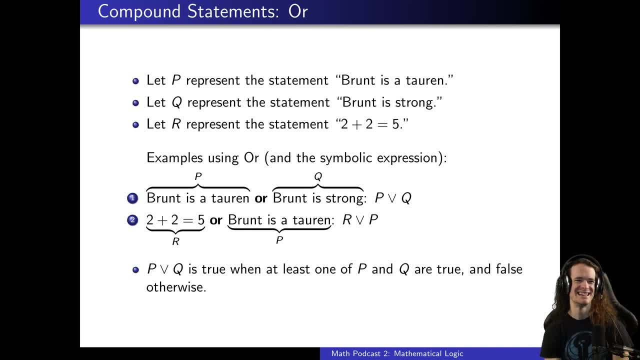 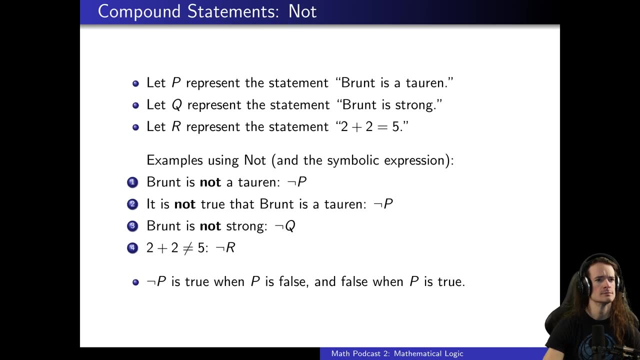 Yeah, you just use the word or. That's my guard. Yeah, and I think some of the ambiguities of the English language definitely help people to frame things the way they want. It's definitely a tool. So we've done or and an or. 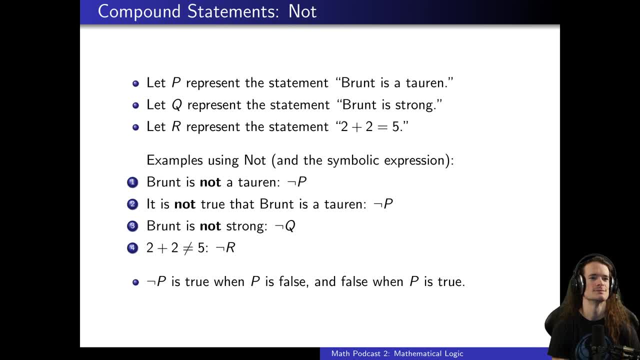 We are so helpful Everyone. you now know how to say and an, or. So the next one we have is not the Allen wrench symbol as you put. So we can say something like the first statement. So if P is Brunt is a Torin, if we put the Allen wrench symbol, this hook symbol, in front of it, we get Brunt is not a Torin. 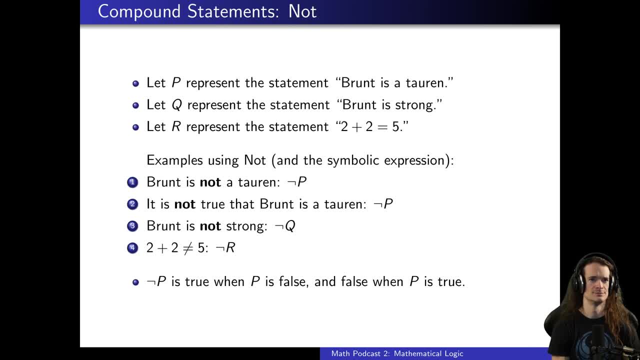 Which isn't true, and I don't want to make Brunt feel bad. Just being clear on that, Or a similar way of English statement of saying the exact same thing would be: it is not true that Brunt is a Torin, So we can just this hook symbol and then P. 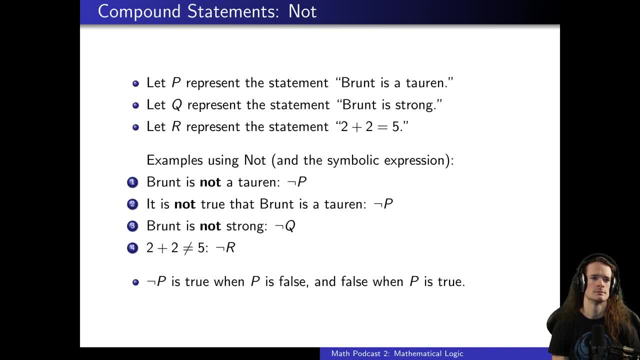 And that's the same exact symbols, for Brunt is not a Torin, just different English corresponds to the same thing. So another way thing we could say again sorry to Brunt, this is false- is: Brunt is not strong. 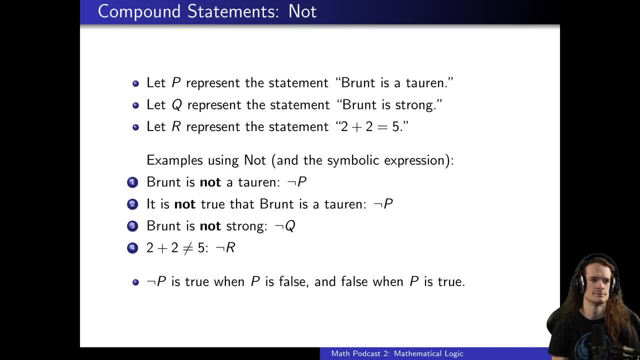 And we have this not symbol Q, where Q means Brunt is strong. We put the not symbol in front of it and it becomes: Brunt is not strong, Or it is not true that Brunt is strong, Or it is false that Brunt is strong. 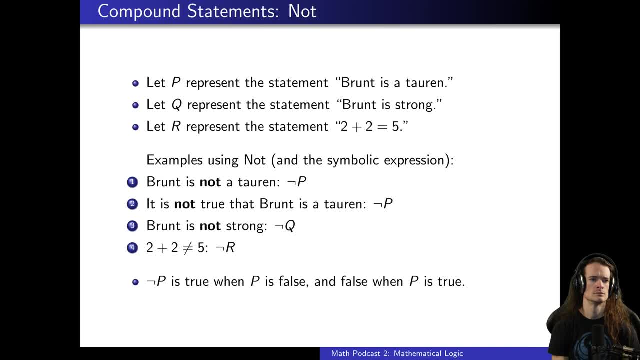 There's a lot of English that corresponds to the same logical statement. Another example would be: if 2 plus 2 equals 5 is R, then not R is 2 plus 2 is not equal to 5.. And since 2 plus 2 equals 5 was false, not R. 2 plus 2 is not equal to 5, is true. 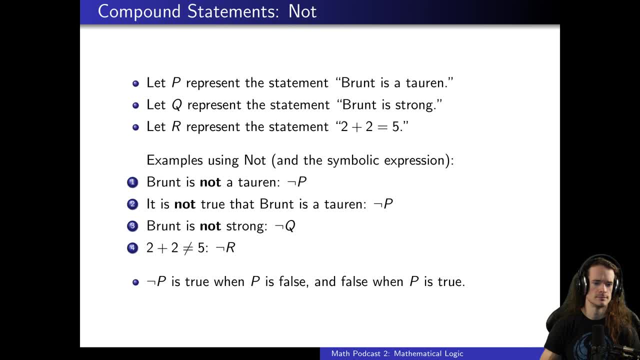 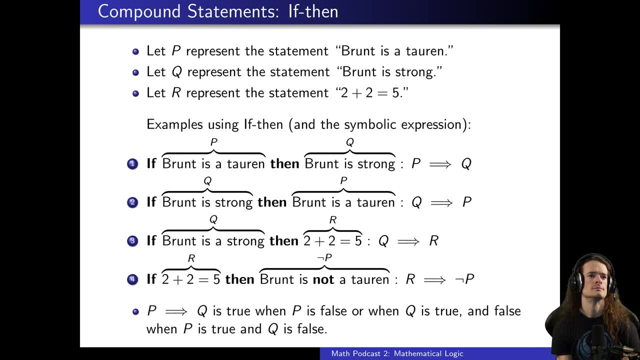 I think I did that math correctly, so that's good. All right, we got not, So the theory we've got are pretty straightforward. So just as everyone's getting really comfortable, let's do the one that's less comfy. Now we will descend into pure chaos. 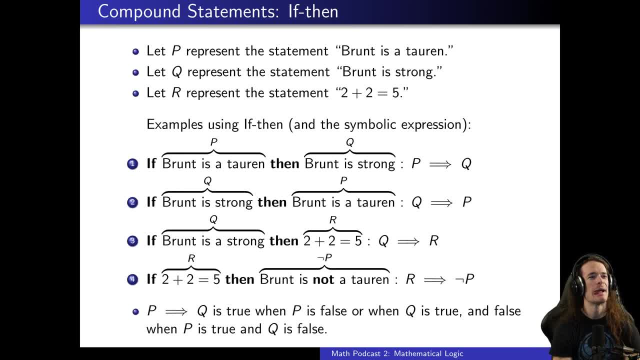 Yes, If-then, also called implication, is probably the most confusing one, And part of it is because the mathematical logic sometimes in a strong way disagrees with what the English meaning is, And we're going to talk about this now, And I think it's going to be a little clearer when we get to first order logic, because a lot of the times when people think of if-then. 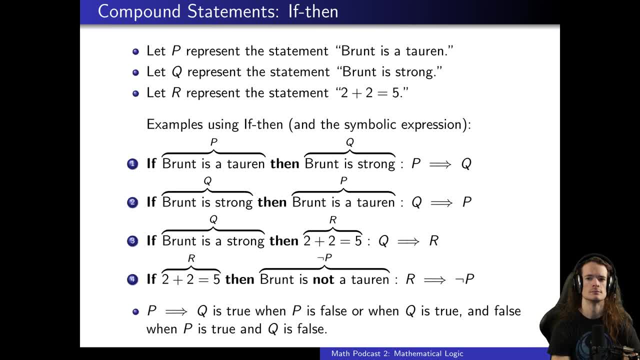 they think of it in kind of a first order sense, even though they don't realize that. But let's just get right into it. So we'll make a statement like: if brunt is a torrent, then brunt is strong. So if P represents brunt is a torrent and Q represents the statement brunt is strong, then we can write: if P, then Q- P arrow, Q- right arrow. 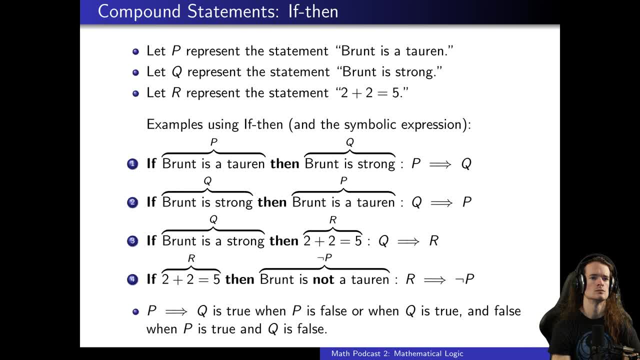 And we can do similar for the other ones here. But let me talk about when is an implication statement true. So the statement if P then Q, which we write as P right arrow Q, is true when either P, the hypothesis, the thing you say, if P then Q, the P. 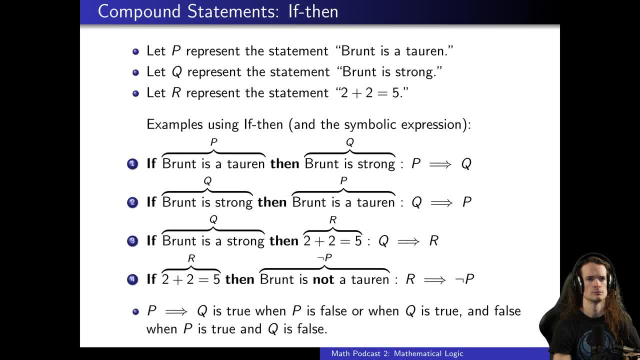 If P is false, then we consider the entire statement true. Another case where we consider it to be true is when Q is true. the conclusion: So if P, then Q is true, Exactly when either the hypothesis is false or the conclusion is true. 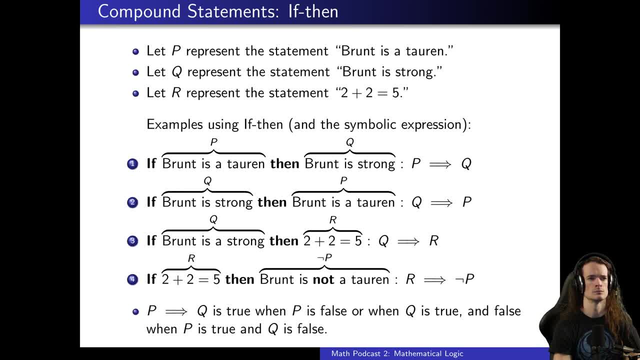 Another way of saying this is that if P, then Q is false, exactly when the hypothesis P is true and the conclusion Q is false. So there's a few things about this that throw people for a loop. The first is they don't like the whole business about P being false, making the statement true. 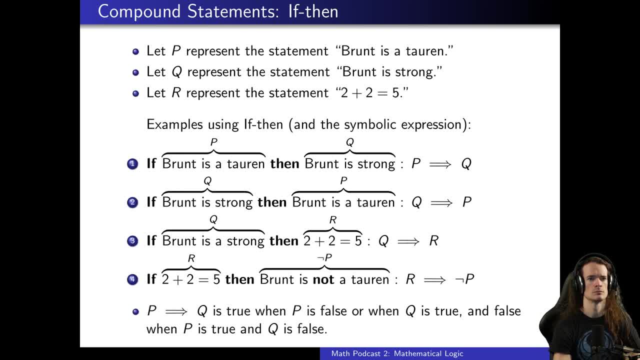 The logic behind that is that if the hypothesis if P then Q- like if brunt is a torrent, then brunt is strong. If brunt is not a torrent, it's kind of like saying the whole statement just doesn't have a say on the topic. 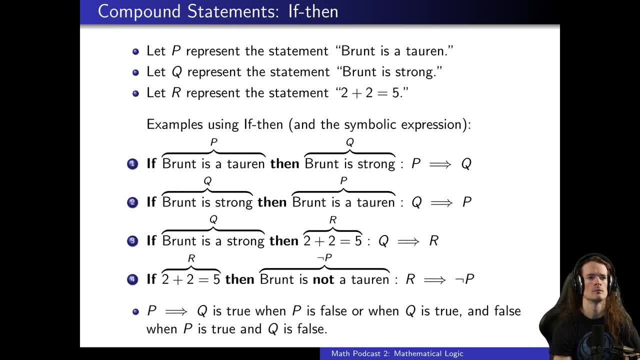 So we'll just, by default, call it true. So this condition isn't met. So then this statement is just not applicable. we'll call it true. And the reasoning for that, I think, will be even clearer when we talk about first-order logic. 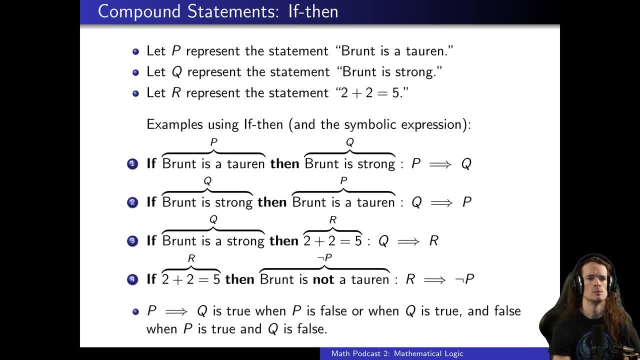 One of the other things. so let's read number two and then I'll try to talk about one of these other reasons why people find this a little bit confusing. So the second one is: if Q, then P, where Q is brunt is strong and P is brunt is a torrent. so we can say if brunt is strong, then brunt is a torrent. 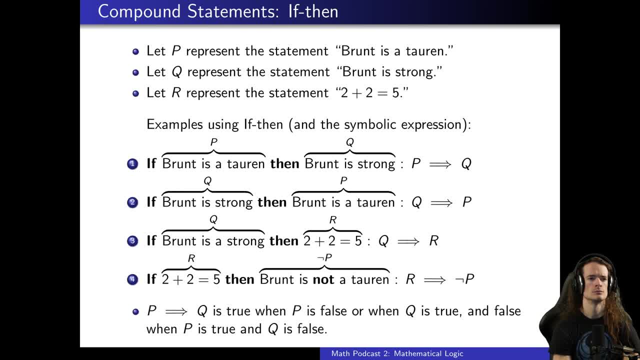 And this is so, both the statements- if brunt is a torrent, then brunt is strong. the first one and the second one: if brunt is strong, then brunt is a torrent. both of those are true, But this kind of sometimes rubs people the wrong way because they're like: okay, torrents are strong. 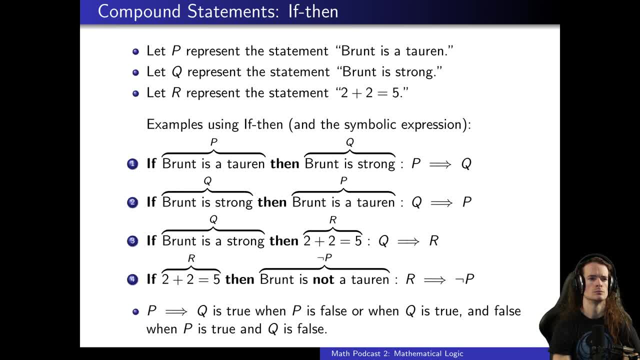 So being a torrent implying that you're strong, that makes a lot of sense to me, But going backwards and saying that's true, that doesn't make so much sense to me, Because it's kind of like: isn't there supposed to be some kind of causal link here that you're missing? 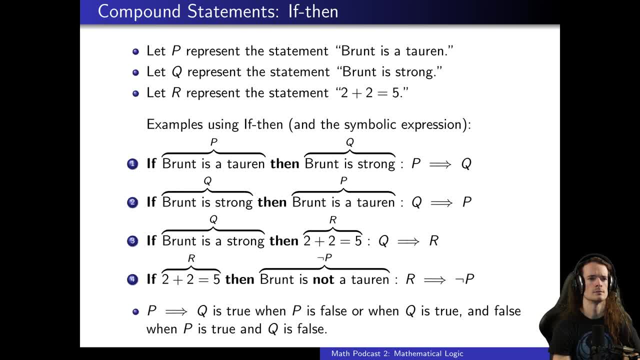 So I don't want to say that if brunt is strong, then brunt is a torrent, But mathematically both of those statements are true, Because in both cases P is true and Q is true, So that the statement is true. 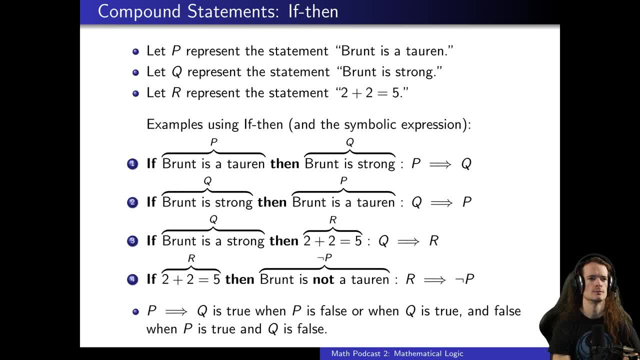 Because the conclusion is true, And so there's a little bit of a disparity here between the mathematical definition of what implication means here and the fact that in logic, in English, there's different meanings for when you say if-then, And I think some of the ways we say if-then conditionals will be better modeled by first order logic. 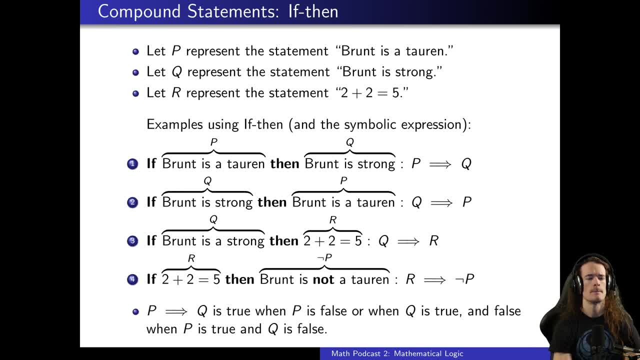 But in general this isn't the perfect mapping onto all the times we say if-then in English. So basically what you're saying is the rules of logic are not necessarily the same as the conventions we use for language and expression. Yes, Yeah, exactly. 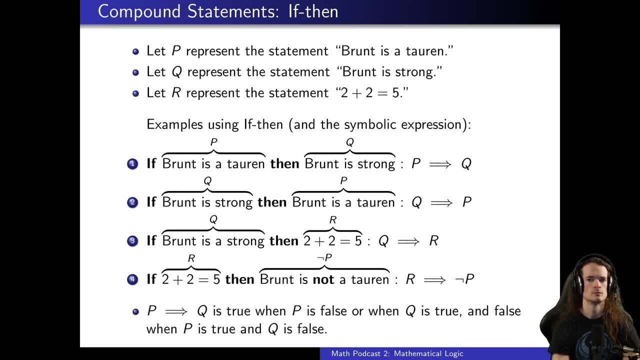 The rules, this mathematical rules of logic for if-then which. so in this case, this is- I believe I'm getting this terminology right- This is called material implication, where it's just like you just have a flat out definition. 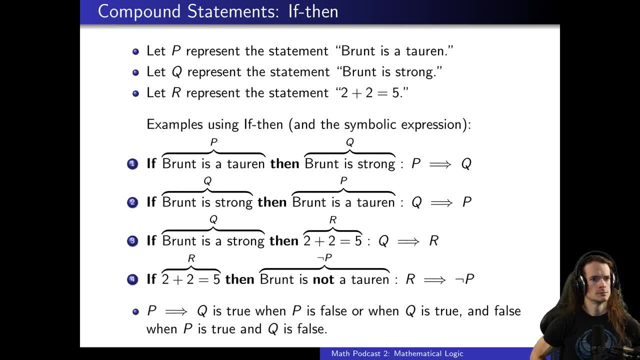 You have a hypothesis, you have a condition, and then you have those rules for determining truth. Is the conclusion true or the hypothesis false? But there's other types of implication, meaning when we say if-then in our language, and some of those aren't conveyed by this mathematical symbols. 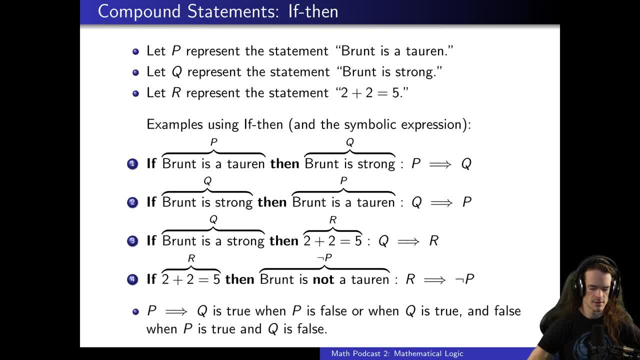 And it's just a different meaning. One thing that jumps out at me as a immediate application for this kind of awareness is having a really strict look at the premise of a statement. A lot of times we'll just passively absorb what someone is pitching to us. 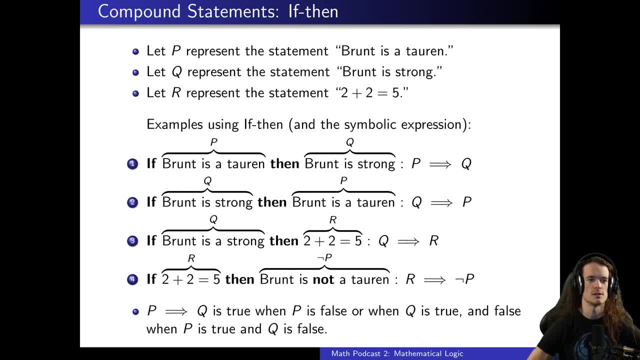 And sometimes they'll start from say P, which ends up being really faulty, So they can't really build off anything useful from that statement. But if we don't evaluate the truthiness of the premise, of the pitch that's being given to us, sometimes we can end up in a really weird situation where they're kind of leading us along in a way that isn't logically sound. 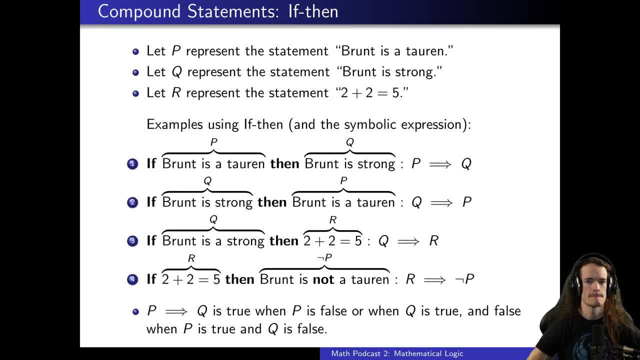 Yeah, sometimes people can use logic to sound like they're saying something very precise and very true, But if you don't meticulously follow the sequence of implications, they can just break one link in the chain and the whole thing is false and they've led you to someplace you didn't want to go. 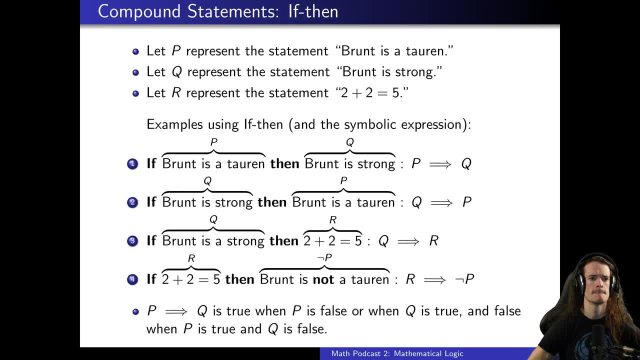 In fact, there's a whole class of examples of these fun examples where people prove things like one is equal to zero by sneaking in a false implication along the way. So there's all these classic proofs of oh, one is equal to zero and other similar silly facts. 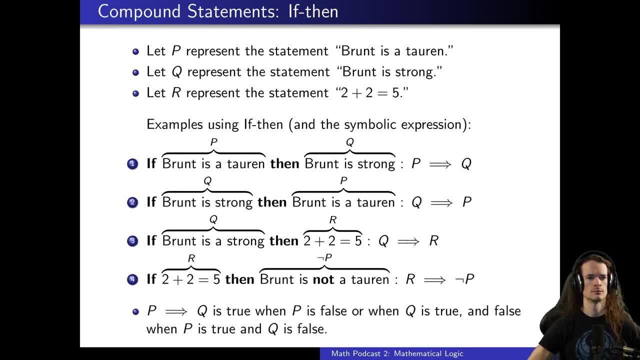 So two plus two is equal to five, And I prove it. and then they give you a proof and they just try to, sort of like a sleight of hand, cover up the one place where you wouldn't expect the false implication to be. 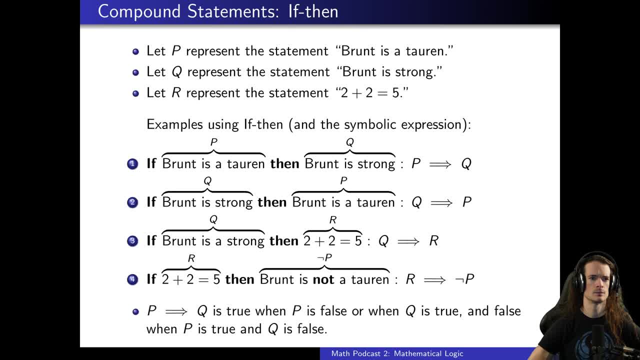 So this may be a little unsettling at the moment. Maybe you don't like the fact that it doesn't exactly map up to English. Maybe you don't like the fact that when the hypothesis is false, the whole thing is false. Maybe the whole statement is true. 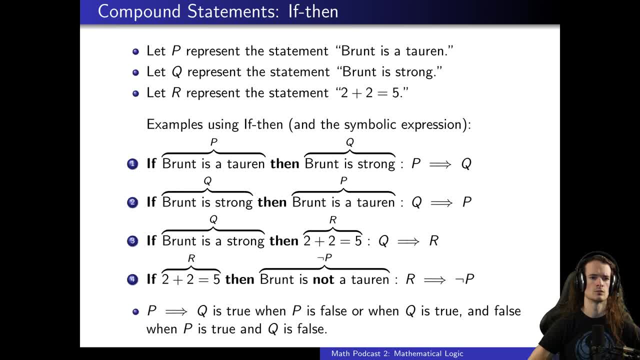 But I hope that a little later, maybe in about 15 minutes, when we come back to the same exact thing in first-order logic, it'll resonate a little more. But for now we're just going to take this as a definition That if you have, if p, then q, which we write p, right arrow q, then that is false, when p is true and q is false and it's otherwise true. 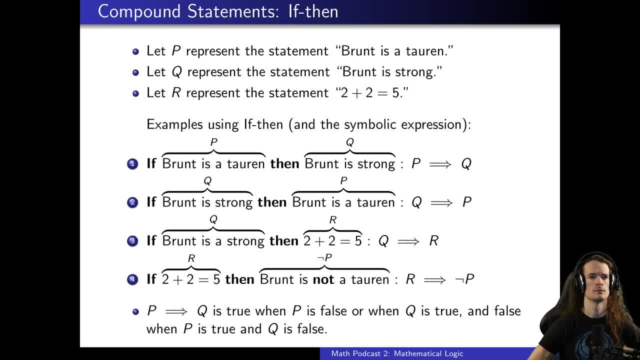 So it's true when either the hypothesis p is false or the conclusion q is true, And that's exactly when it's true. So I'm going to take this sort of as a definition and I claim later it'll feel better, But we'll see. 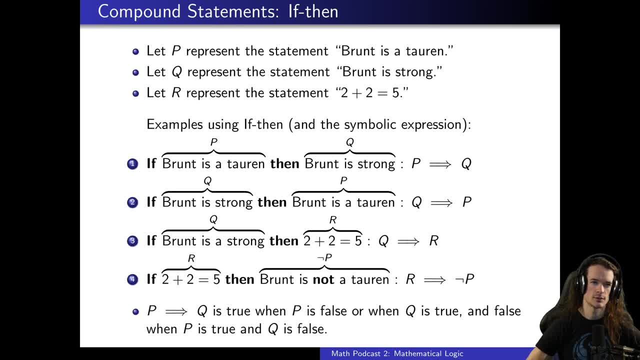 But, as we pointed out in the first session, a lot of times the correct answer for math or physics or whatever doesn't necessarily line up immediately with your intuition. and that's okay, Exactly Because sometimes people they'll listen to a sequence and they'll say: all right, like what? 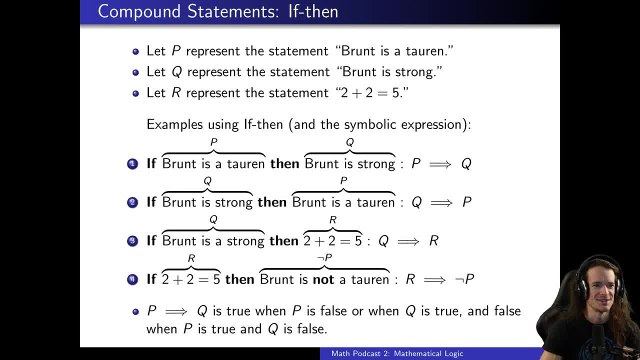 That's okay to have that as your immediate reaction. We're just getting started here. Certainly Part of it is like learning curve and discomfort, and that's natural. It actually means you're learning something, You're actually being exposed to something you haven't seen before. 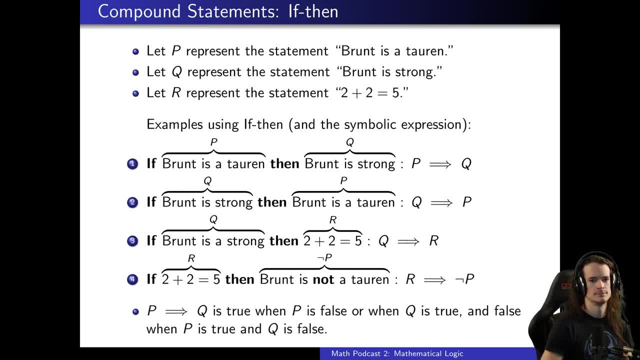 That said, logic in some ways is very core to the way we reason, So it should make some sense, and it is a little unsettling that this doesn't jive exactly, but I hope to make it jive more in just a few moments. 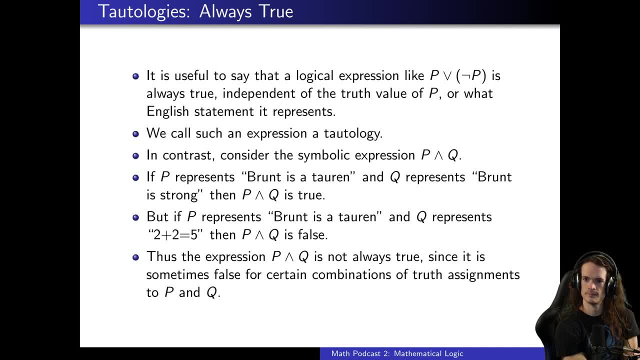 Cool, All right, So let's talk about compound statements. So we just have two more things we want to talk about in propositional logic, and one of them are tautologies, things that are always true. So it's a warm feeling to think about things that are just true all the time, independent of the meaning. 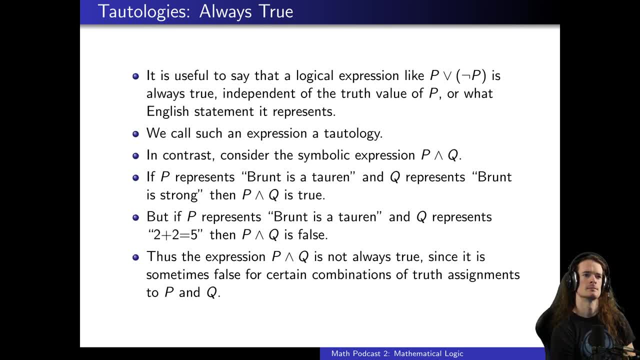 So an example of that would be a statement like P, and the V symbol here means, or just to remind you, not P. So an expression like P or not P, independent of what P means, if P is true or P is false, independent of that. 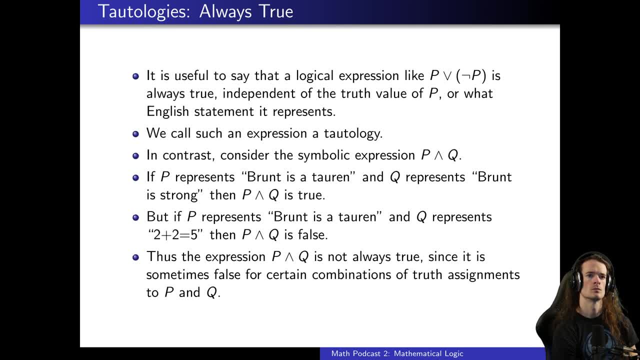 P or not. P should always be true, because either P is true or not, P is true and one of them is true and then the or is like. either one being true immediately gives it to you And it is inclusive right. So both is also an option. 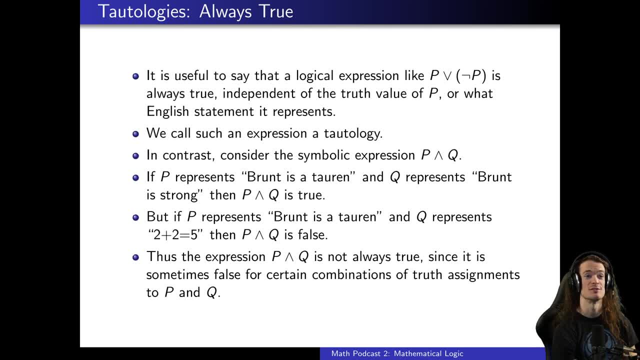 But it would be very hard for P and not P to both be true. That's a superposition of P. Yes, There are times when people talk about these logics where things can be sort of one thing or the other, but we're not going to be doing that. 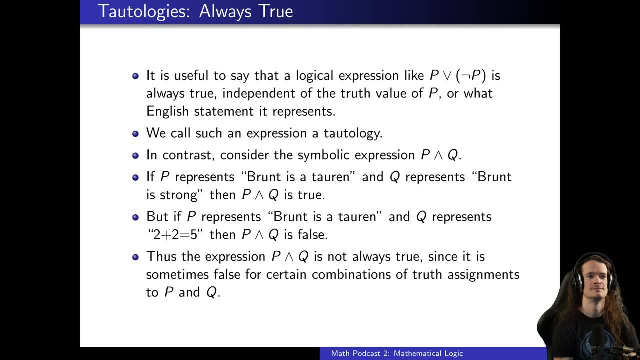 So here, either P is true or not. P is true one And yes, so the P or not, P is always true. So we call such a statement a tautology. Independent of whether P is brunt is a torrent, or whether P is 2 plus 2 equals 5, P or not, P is always true, and we call that a tautology. 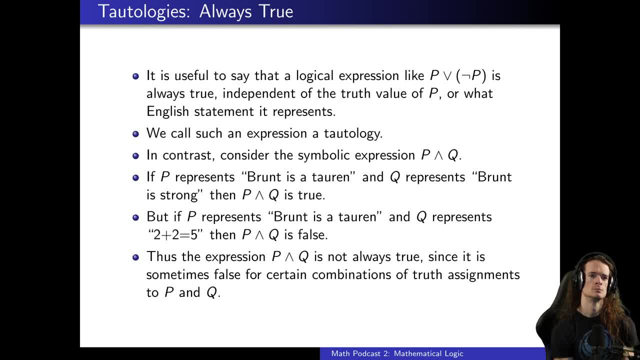 In contrast, consider another expression like P and Q. So remember the upside-down V is the and symbol. So P and Q. So if P represents brunt is a torrent and Q represents brunt is strong, then P and Q is true. 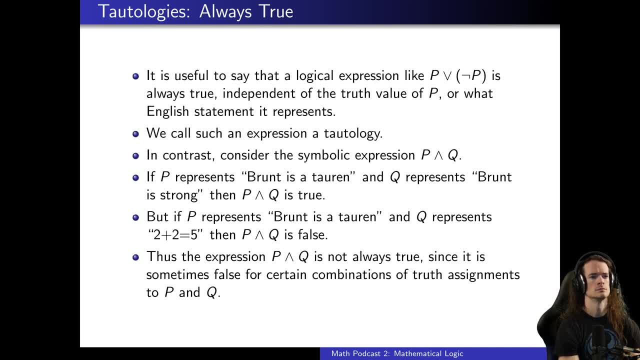 Success. That's a true case. P is true and Q is true. so P and Q is true. But if instead we let P represent the logical symbol, P represent maybe a statement like brunt is a torrent, and Q represent 2 plus 2 equals 5, then P and Q is false. 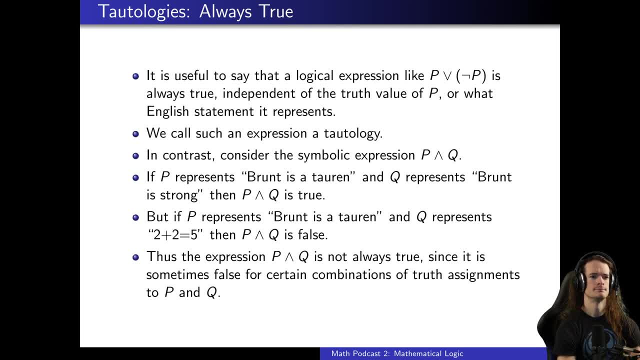 So there are ways to assign truth values to P and Q. that makes P and Q false. So P and Q is not a tautology, because there are certain ways of assigning values to P and Q that makes it false. And tautologies are reserved for those expressions that are always true, those cornerstones where we can always rely on them, logically impeccable. 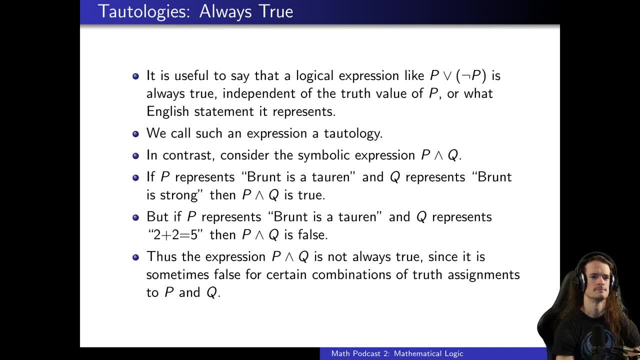 Perfect, Yes, So let's go through one example. I apologize if this frightens people. We can spend almost any time on these things, But one way to verify whether something is true on the next slide is using a truth table. So you might have seen this before. 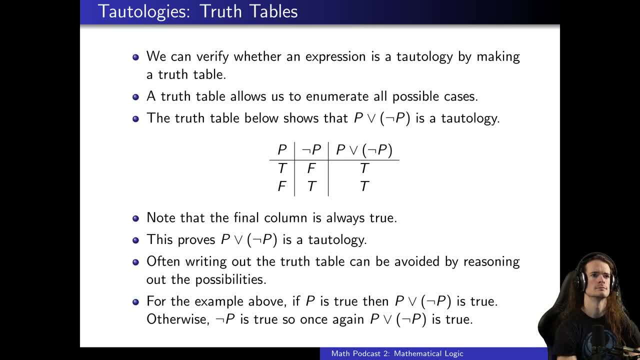 Maybe it's scary. We're going to do like two minutes on truth tables, just so we, because it's good to see them, and then we're not going to do it anymore. So how do you check if a statement is a tautology? 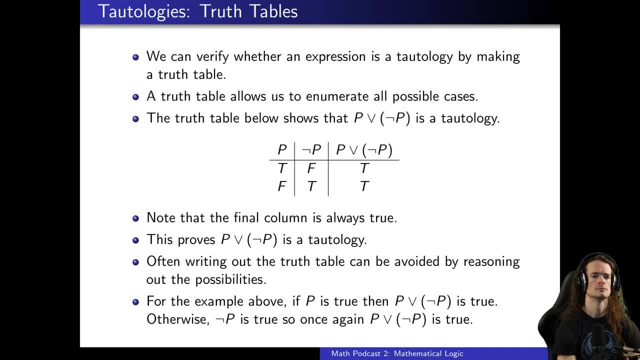 And one of the methodical ways of doing that is to just go through all the cases. So if we have this statement- P or not P, Let's say we wanted to check if it's a tautology. So one way to do that is to say what are all the possible values P can possibly take. 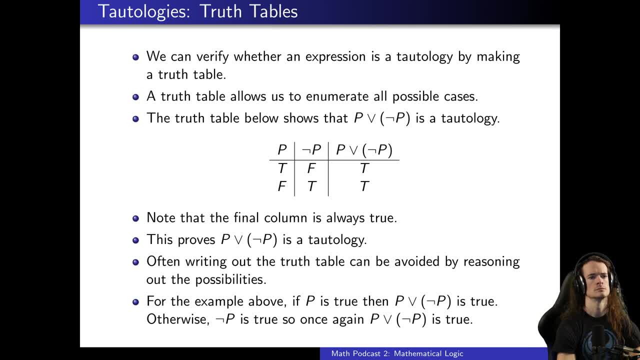 Just true or false. If that's the case, that was the first column of this truth table. The second column says all the values, given the value of P, that not P can take. So if P can be true or false, then not P is false or true. 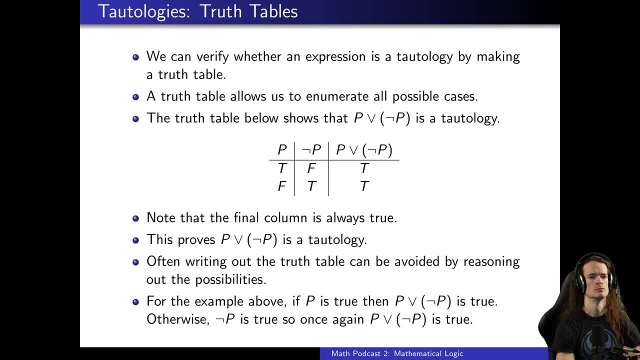 And in both of those cases, as we put in the third column of this truth table, P or not P is true in both cases. So in all possible truth values for P, the expression P or not P is true. So we could say: the upper case is brunt is strong and the lower case is 2 plus 2 equals 5, for example, 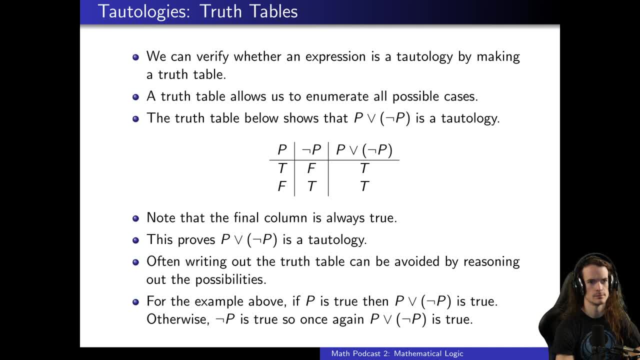 Is there a Oh, yeah, sure, Yeah, the upper row. So if in the first row we were in the world where brunt is strong is the Is P, Yeah, And then we would never say that brunt is not strong. 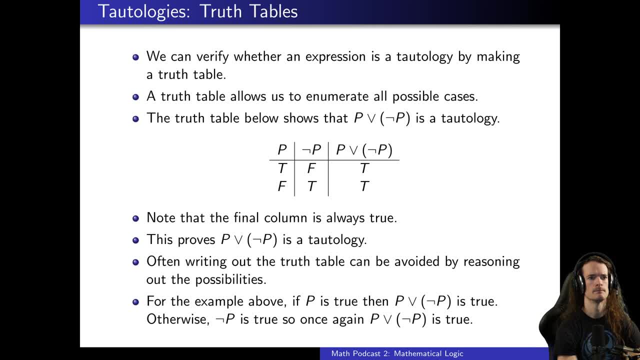 It could be a valid way of scientific. So yeah, So another example would be: 2 plus 2 equals 5. And that would be like false. And then, yes, But in both cases, P or not, P is a true statement. 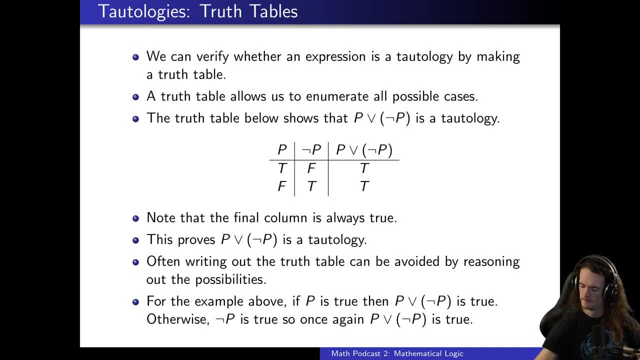 So, P or not, P is always true And we've checked it by checking all the combinations in this table. So it's sort of like visually apparent And this was what proves that P or not P is a tautology, But often you can get away with not writing out the table, just by reasoning it. 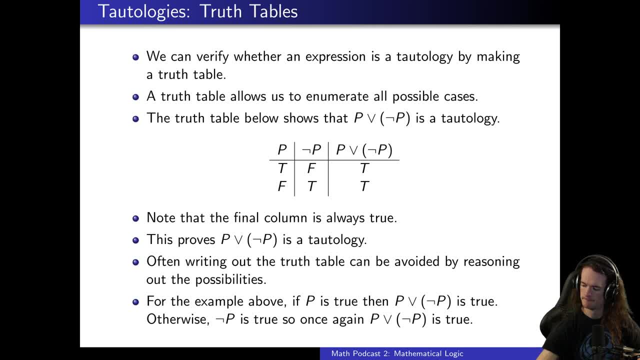 And I think that's a good skill: to just think about why one of these statements is or isn't a tautology. to sort of just reason it out, Say, well, let's think about P or not P. Either P is true, in which case P or not. P has to be true because it has a P in it and it has an or. 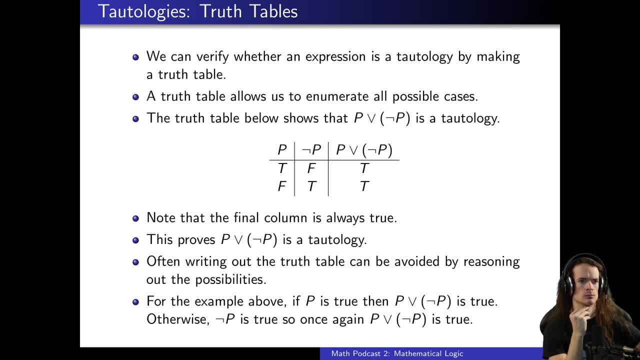 But if P is false, the other case, then not P is true. And this P or not P has a not P in it also. So then in both cases it's true. So we kind of like reasoned out in our mind what is going on in the truth table and sometimes thinking it through, 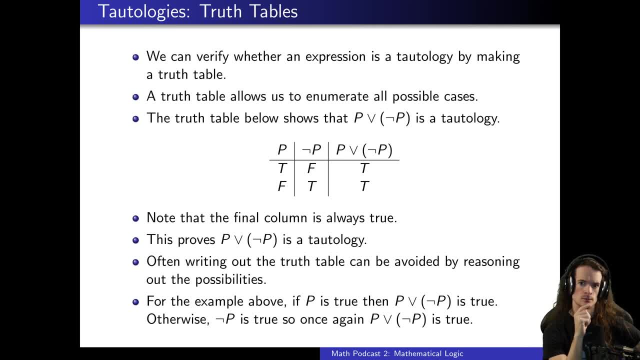 And just it should, in some way getting to the point where it rings true that, P or not, P is always true. Just from like, pure reasoning is a good place to be, So you don't always have to rely on the truth table. The truth table is like a honestly a crutch, but a good way to start off. 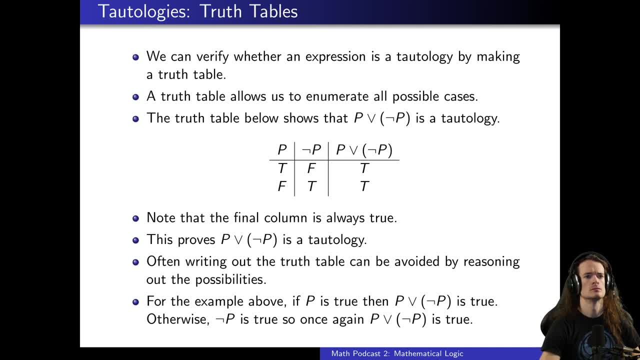 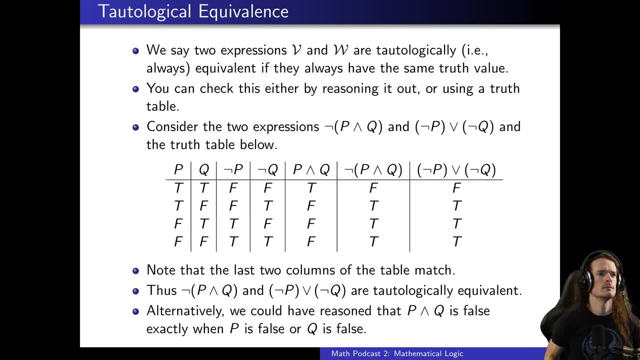 But sometimes thinking it through is good too. The truth table is a visual aid. You can see it represented in front of you. Sure, And we have one more truth table in us, So I'm going to talk about one more concept that's going to be useful to us. 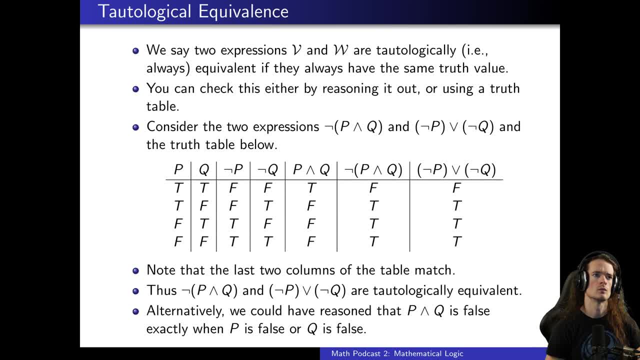 And that's called- has a fancy name- Tautological equivalence. So you can say that around the coffee table to sound fancy at a party or something, But all it means is that two expressions always have the same truth value. So one way to check if two expressions always have the same truth value is to reason out all the cases. 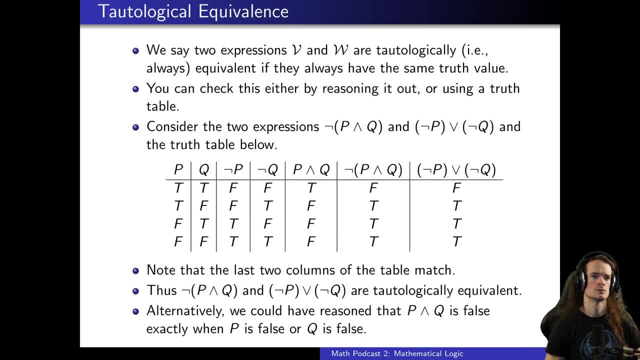 But a visual aid for doing that is a truth table, And I wanted to come up with one more, slightly more complicated truth table just to show what a nastier looking truth table looks like. So let's consider two expressions. here We have the negation of P and Q. 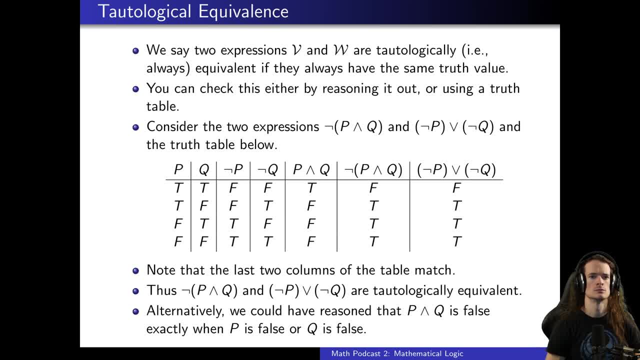 And the second statement is not P or not Q. And we're asking: are these two statements, do they always agree on their truth value? Is it always true that if not P and Q is true, then not P or not Q is true? 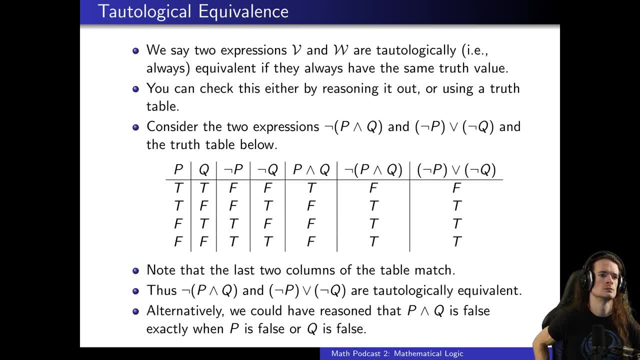 In addition, if not P and Q is false, then not P or not Q is also false. So this is actually a law. This is called De Morgan's law, But we're going to prove it. We don't need to rely on existing concepts. 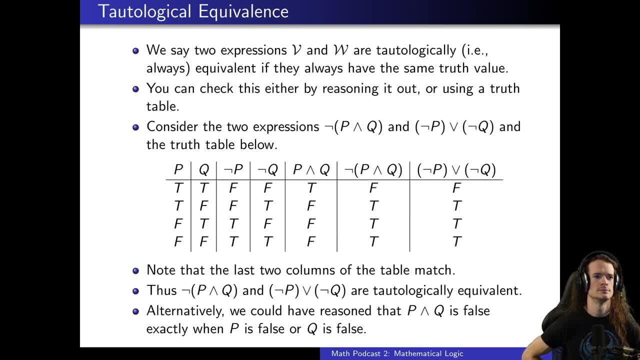 We're just going to prove it with this truth table, And the game here is we're just going to write out all the combinations. So if we have, P can be true or false and Q can be true or false, it turns out there are four combinations. 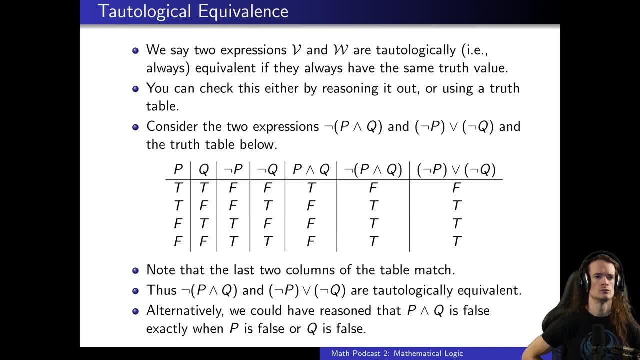 For what P and Q can be. They can both be true. They can both be false. P can be true and Q can be false. Or maybe P can be false and Q can be true. So we have all four combinations of the truth values. 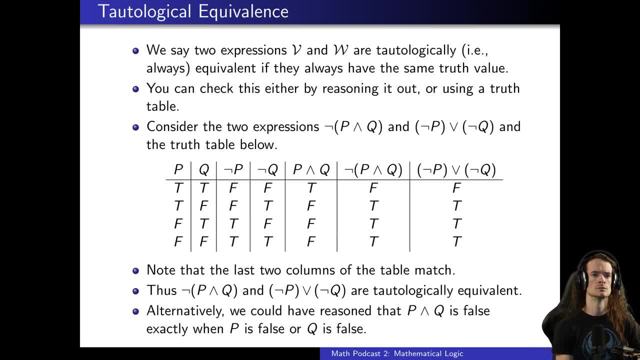 And we put those in the first two columns All four ways, So that we've exhaustively handled all the cases. And in the second two columns we've written what not P and not Q are given the first two columns And now we can build up the more complicated statements. 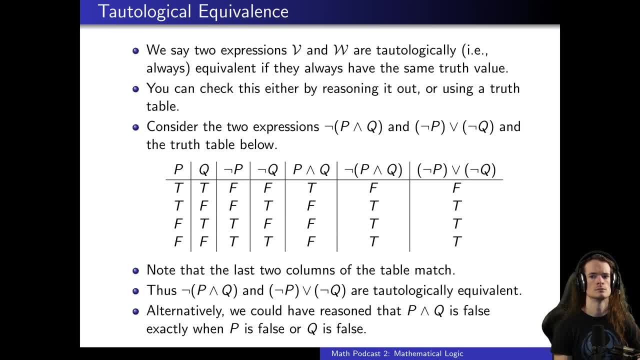 So the first statement we were curious about The value of is not of P and Q. So let's first figure out what P and Q is. So let's recall: So P and Q and the symbol for and again is the upside down V. 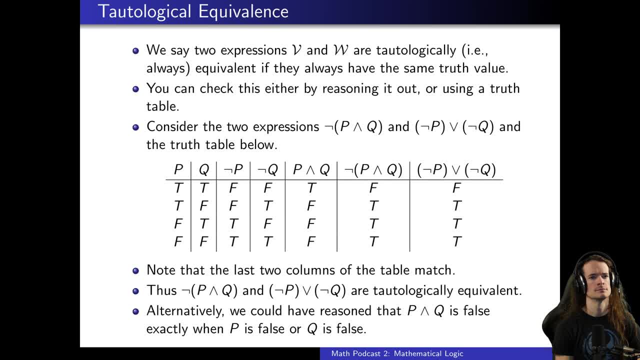 That is true when both are true, And that only happens in the first row of this truth table, when P and Q are both true. The other three rows have at least one of them false. So as we see, true, false, false, false in that P and Q column. 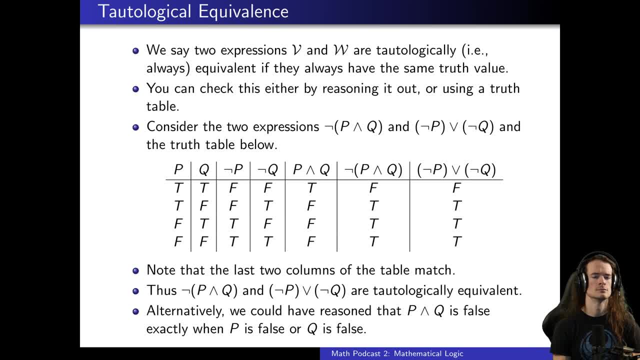 And then the negation of that. we just flip them all. So in the next to last column we have false, true, true, true. And I got that just by flipping the column before it Because we negated it. And negation just flips true to false and false to true. 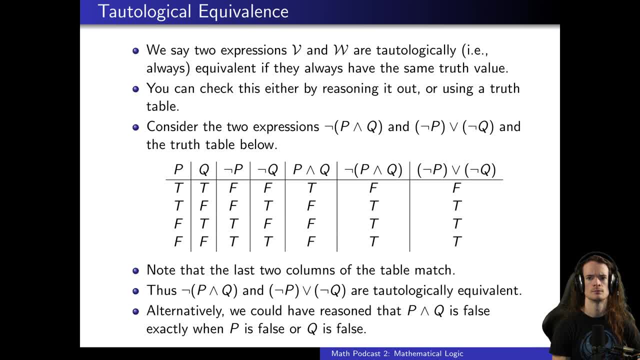 Lastly, we already have columns for not P and not Q, So we can OR them together. So we put a true when at least one of them is true. So the first row, both false, is false, And the remaining rows all have at least one true in them. 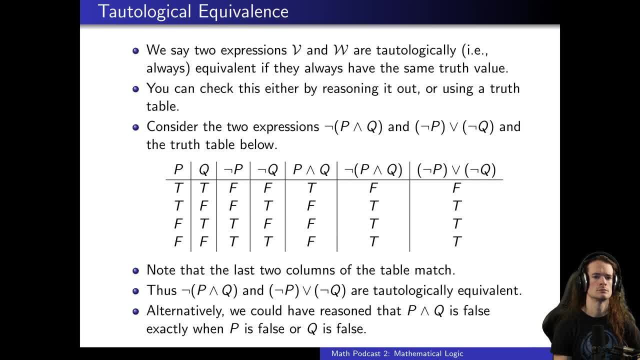 So we get false, true, true, true. And then, now that we've made this full table, we can look at the last two columns And we can say they are exactly the same. So not of P and Q, and the expression not P or not Q are always the same. 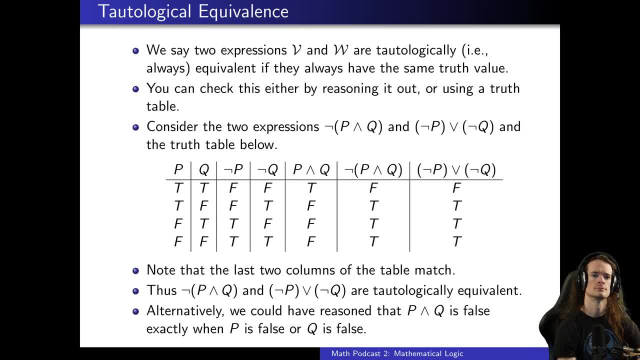 They are tautologically equivalent. So we've proved the law of logic That, independent of what meanings and sentences you assign to P and Q, those symbols, those symbols, these two expressions are always the same. So it's so, and we can also reason it out. 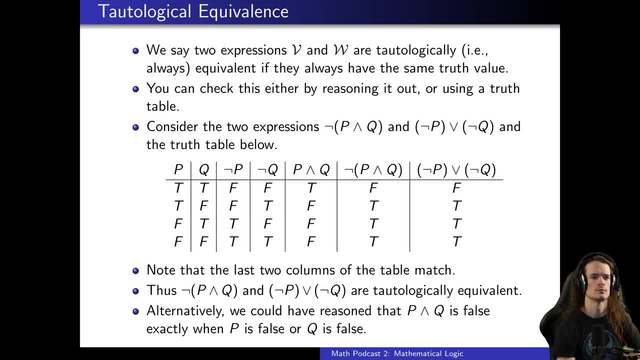 So when is the statement P and Q false? So, based on the definition, it's exactly false when at least one of them is false, And that's exactly what the statement not P or not Q is saying. So, logically, just reasoning it out speaking, it does make a lot of sense that those two things should have the same columns. 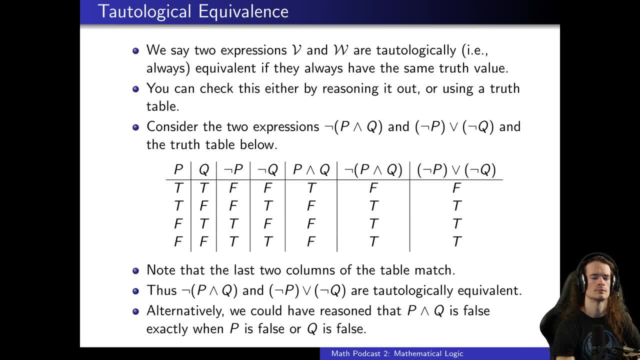 Because logically it seems to jive. But the truth table then just like seals the deal. It's like: oh, I know your logic is you're reasoning it out, But let's just go through all the cases. And we did. 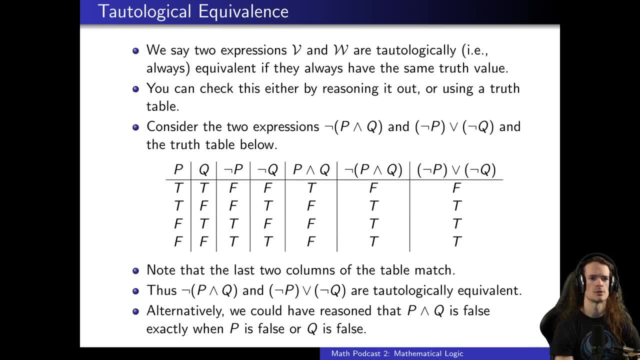 All four cases And they do indeed agree. I think the truth table also is a way of breaking it into smaller pieces, where you can basically reconcile each individual one rather than trying to tackle the whole thing all at once. Because I think when you first start with this comparison of 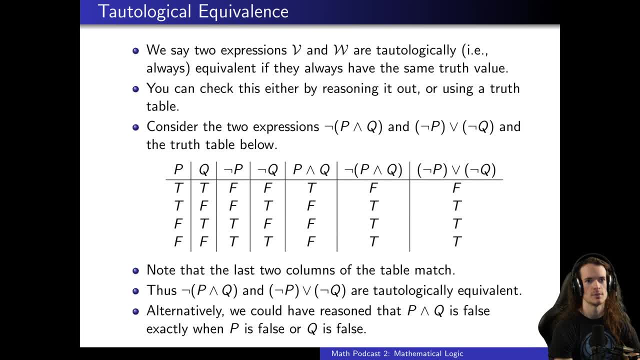 Yeah, Not P and Q, and not P or not Q. It's not obvious that they're going to be the same, But being able to see all of that in front of you, then double check, it is pretty helpful. Absolutely, Yeah. 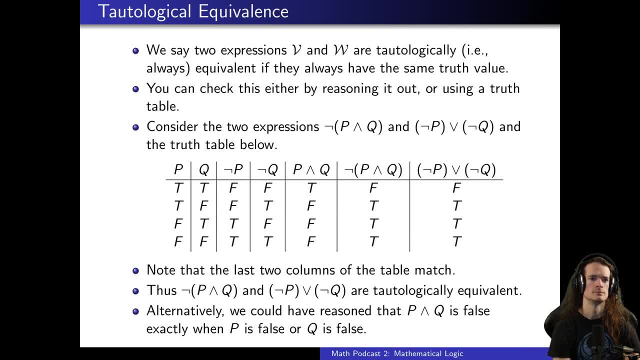 You could be worried like, oh, maybe I missed the case that I actually handle everything, And yeah. So I think I think it's good to have the truth table to check and definitely work through- And I think that's great- And also be able to think about. does it make sense that these two statements- because I think it's also good to sort of try to integrate these concepts- 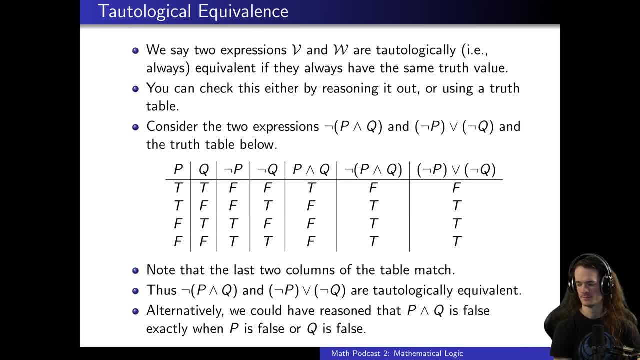 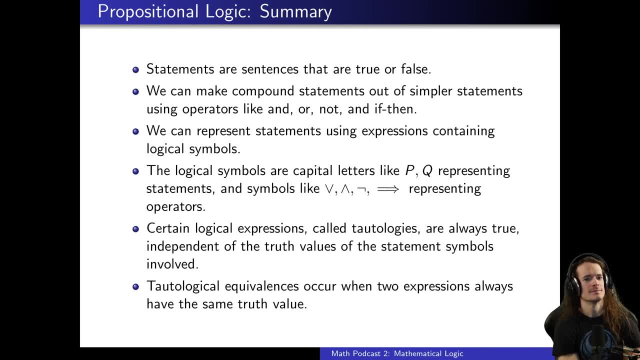 Which we proved using truth tables into our logic. So I think that's all I have for propositional logic. So that was a section done. Hopefully wasn't too bad, And I've summarized it in the next slide. So we have that statements. 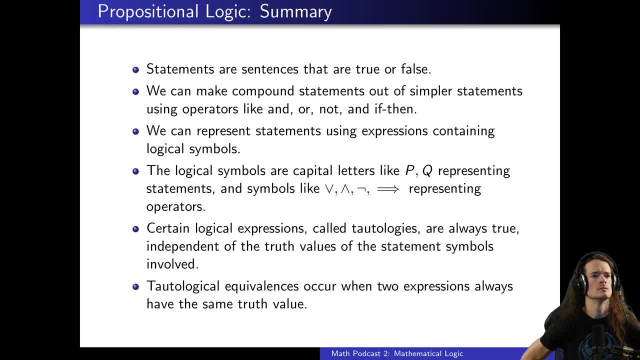 Our sentences that are true or false and we can represent. Oh, so I'll get to that in a second. We can make compound statements from these simple statements by mixing them with things like and or not. And if, then We can represent these. 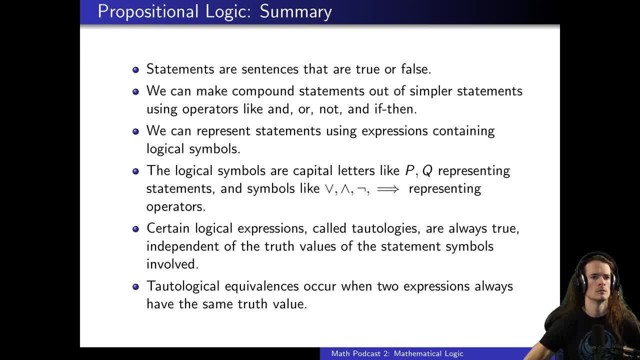 Statements and compound statements using Expressions containing logical symbols. So we'll use P and Q to be these Symbols that represent statements that can be true or false, These truth variables, if you like. And then we have the symbols: the V symbol for, or the upside down V symbol for, and the hook or Allen wrench, or not. 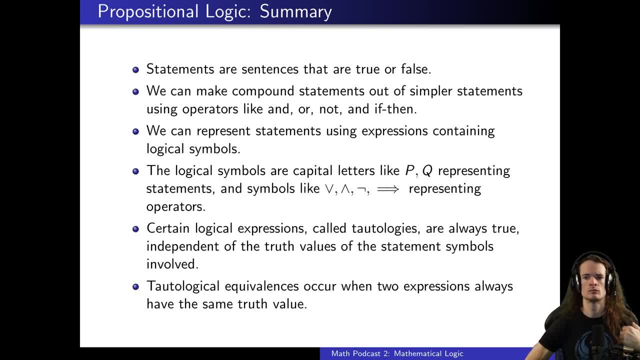 And the right arrow for if, then, or implication implies. So Sometimes, when you read the right arrow, you can read it as if then, or you could also read it using the word implies. And then we said that certain logical expressions, called tautologies, are always true, independent of the meanings of that you assign to the variables of them. 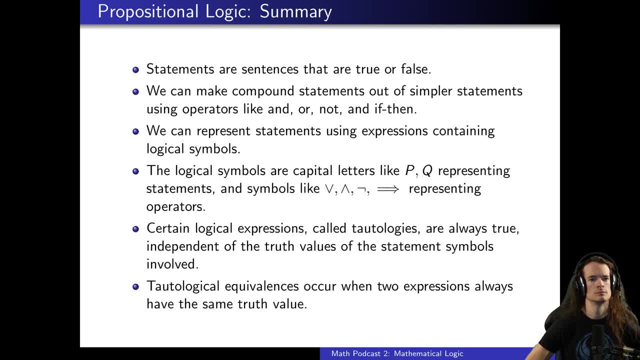 So for all cases of the truth values of the variables in this expression. it is always true And we said also, tautological equivalences are when we have two expressions that always have the same value. So they are equivalent logically. In all cases they always have the same truth value. 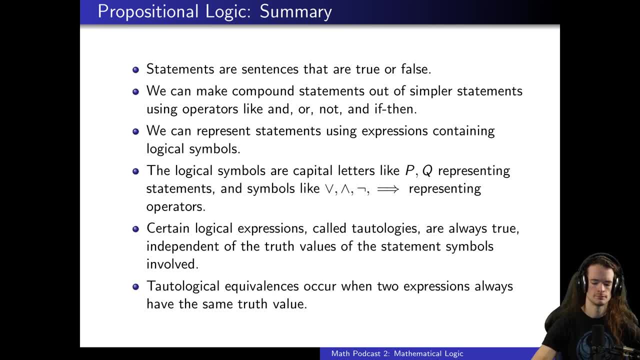 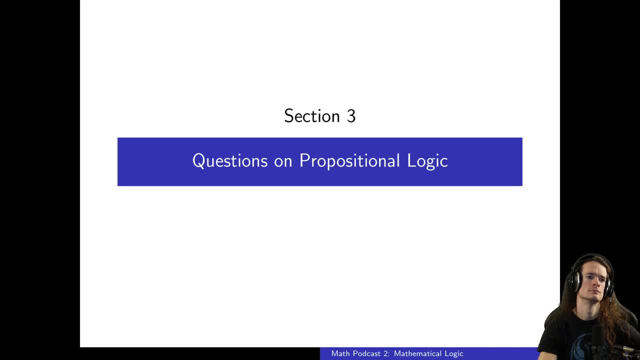 And that concludes propositional logic. So I think this would be a good time for us to stop Teaching new things and to review using a few interactive questions. We can do with chat, So you want to? just when we ask these questions, you can just scream the answer in chat. 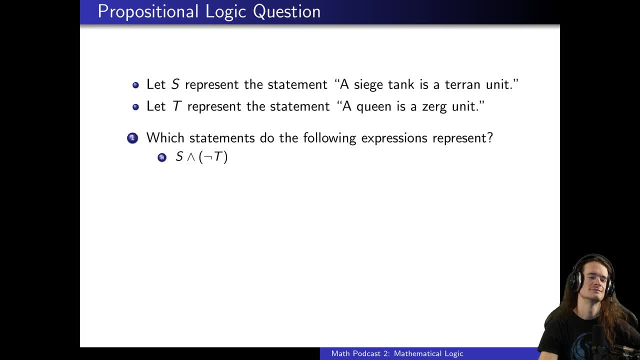 Mean Neuro. Maybe I'll peek. We'll also go over the answers together. So let's think about this for a moment. So we're going to let S represent the statement. A siege tank is a Terran unit. This is from Starcraft 2.. 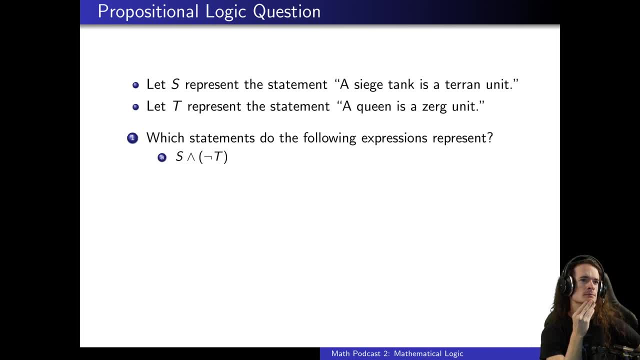 We'll let T represent the statement. A queen is a Zerg unit. So I put a symbol. there S upside down V, and then the hook symbol, T or Allen wrench, And so I want to know what does that state? what does that expression mean in terms of the statements? 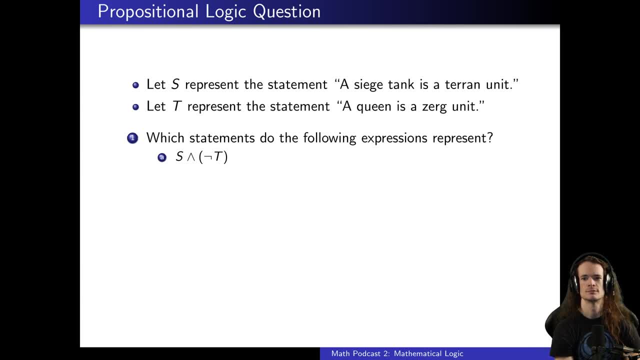 So take one second to think about that and then maybe we'll go over the answer. So the point of this And also, as I said, if you're listening for any of these, they'll get a little harder. If you want to pause and think about them, please, please, do so. 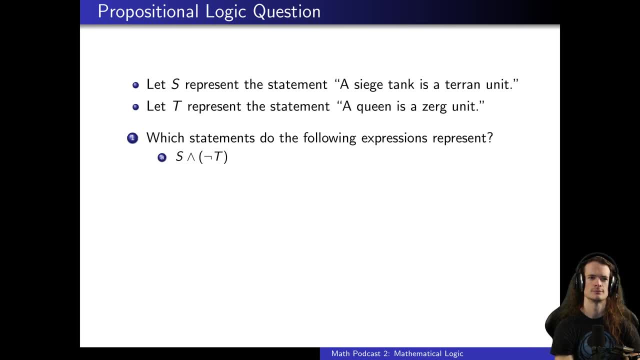 So let's see. So this is trying to remember what these symbols mean. So in this first case, A, the answer is: A siege tank is a Terran unit and a queen is not a Zerg unit, And that should be from the next. 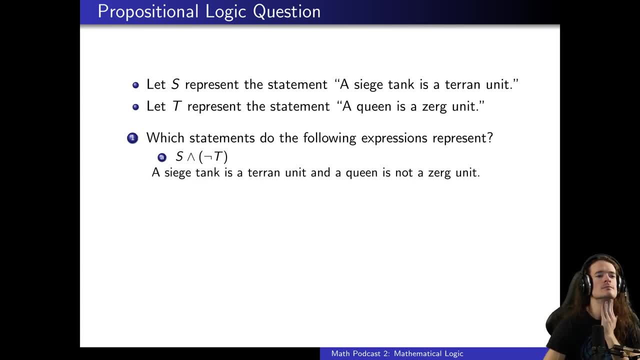 If you click ahead, I think that will reveal the answer. I think I got it right. Good, I know some logic, Good to know. So the next question, part B, is going to have this hook symbol S and the V symbol, then a hook symbol T. 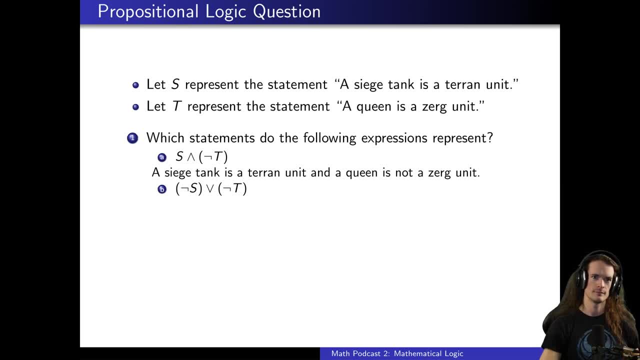 Or Allen wrenches, as you put, instead of hooks. So what does this mean? Can you take a moment to take a look at it? Remember your symbols. Can I take a guess, Please, please? And if you see anything from chat also, you're like the conduit for chat. 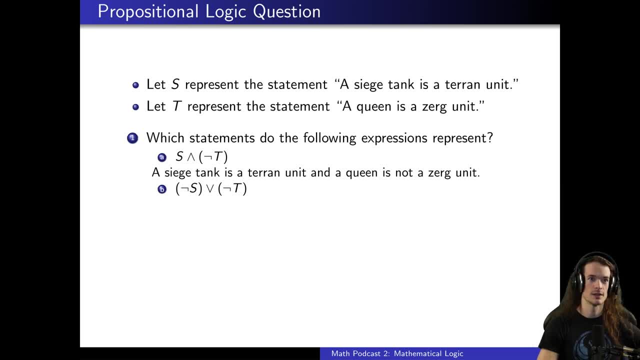 A siege tank is not a Terran unit, or a queen is not a Zerg unit. I feel like I'm not needed here. Super smart, Yeah, Neuro can just teach it. Well done, sir. Couldn't have said it better myself. 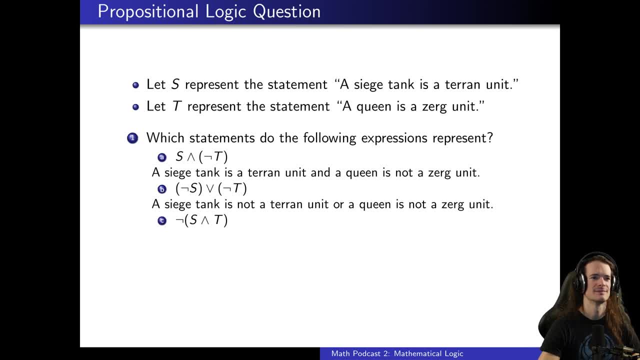 Let's move on to the next one, And I see some answers in chat. I'm liking it. People are learning, Learning is occurring And yeah, just, there's no need to raise your hand in chat, Just scream the answer. 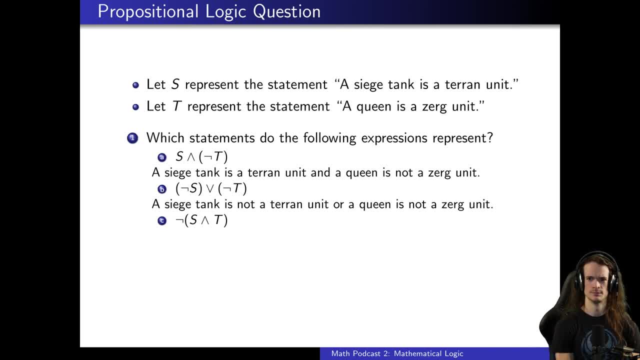 Let's do C, So C is going to be the hook symbol, And then in parentheses, S, upside down, V, T, Close parentheses. What does this say? Yes, And as is being asked in chat. I'm glad I spotted this. 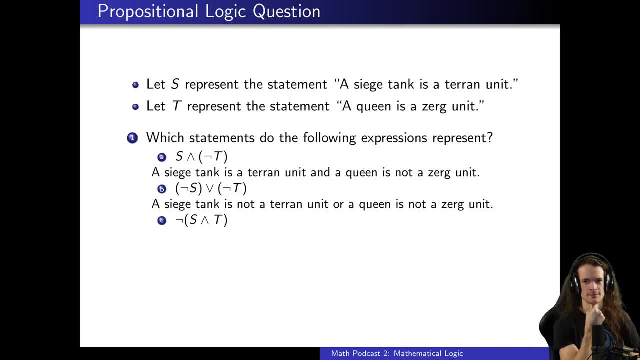 I'm making no claim that these statements are true. In fact, the first statement is false because a queen is not a Zerg unit And there's an and there And in part B, both statements were false because a siege tank- saying a siege tank- is not a Terran unit and a queen is not a Zerg unit. both of those are false. 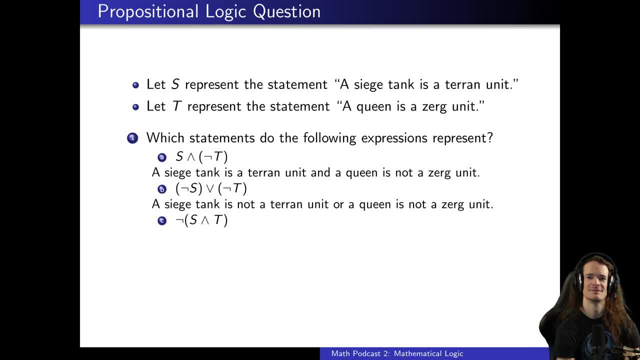 And we orred them. But that's exactly the case where or is false, because both of them were false. So, C, what do you think? Or should we just let them have it? It is not the case that a siege tank is a Terran unit and a queen is a Zerg unit. 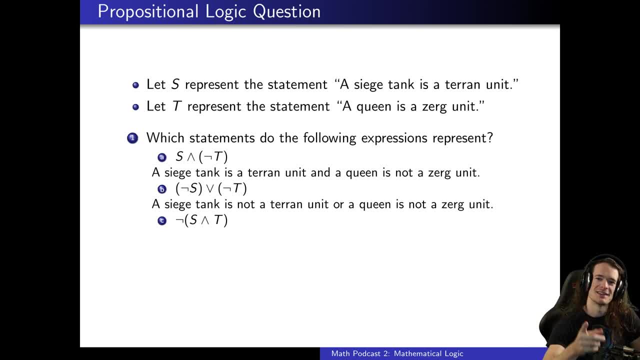 Wow Sounds good. I like the way that Pillage framed it. You just say a siege tank is a Terran unit and a queen is a Zerg unit, Not A modern way of saying it. yes, Yeah, So let's see if I have it right there. 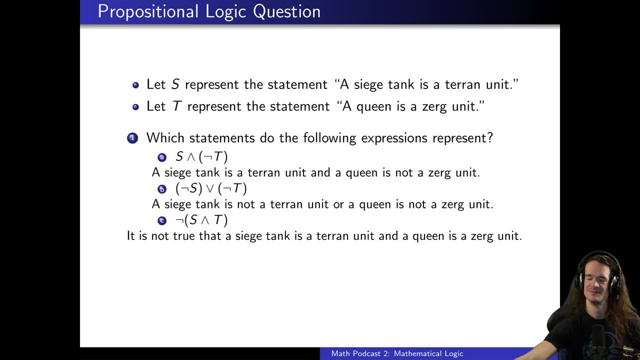 I have it almost exactly the way you said it. So well done, Well done. Maybe we'll do. do I have one more? Are any of these tautologically equivalent? Hmm, Are any of these statements tautologically equivalent? Okay? 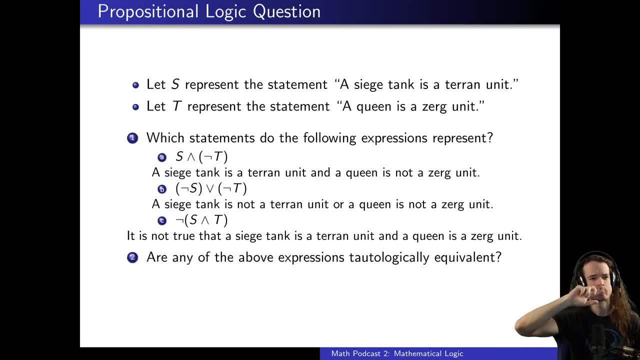 So take a moment, So remember the three statements: We had S and not T, We have not S or not T, And we have not of in parentheses, S and T. Are any of these statements tautologically equivalent? Hmm, Hmm. 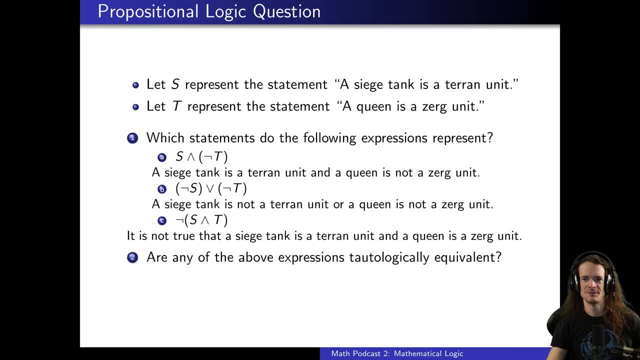 Oh wow, Chad's just jumping on it. They are good, Incredible. So Chad is screaming B and C, And that is indeed the correct answer. So let's think about this for a moment. And this is the flip of the one. we did the truth table on. 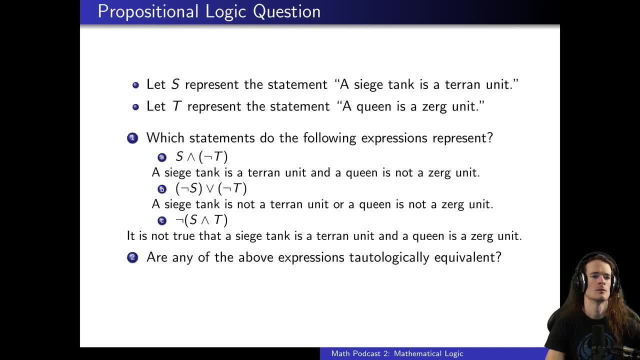 What does it mean to say something is. what does it mean to say: it is not true that S and T is true, So not of S and T. When is it true that? so let me say this differently. What does it mean to say it is false that S and T occurs? 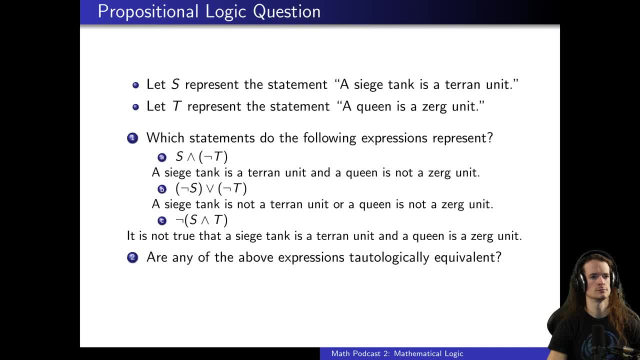 So for that to be false, for S and T to be false, it is exactly the case that either S has to be false or T has to be false. So C and B are saying the same thing. The first B is saying S is false or T is false. 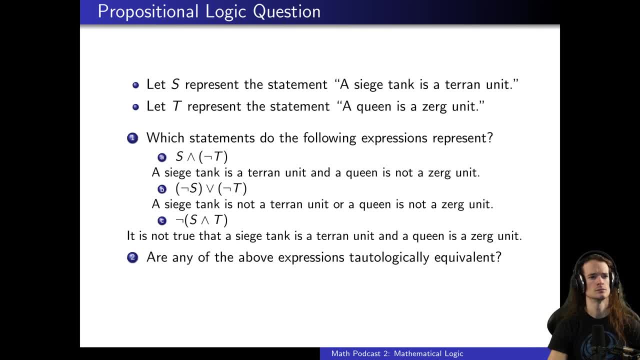 And C is saying S and T is false And those are exactly the same thing. And if we wanted to- I don't have it here, but if we wanted to- we could check that with the truth table. This also hits with a general awareness that you can have two correct answers for something, or you can say the same thing in two different ways. 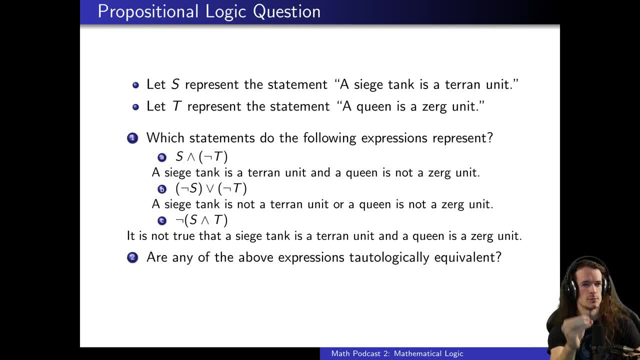 I think a lot of times there's a desire for it all to boil down to one thing that is on its own, Whereas here we see different shapes that are basically equivalent to each other, Absolutely. Yes, And A is not the same, So an example would be: so let's suppose that S, let's see what would be a good way. 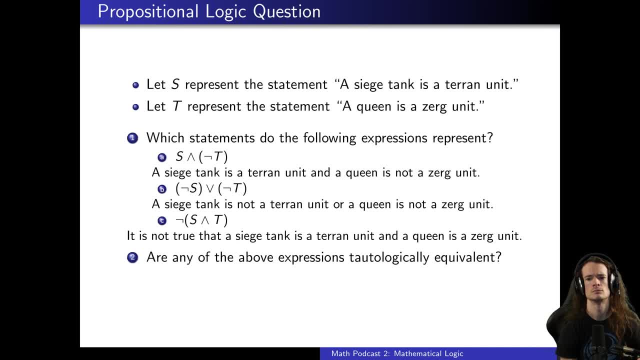 So if we have S is false and T is false, so they're both false, then the statement B would have true or true, but the statement A would have false and false. I'm sorry, false and true. So those are not the same. 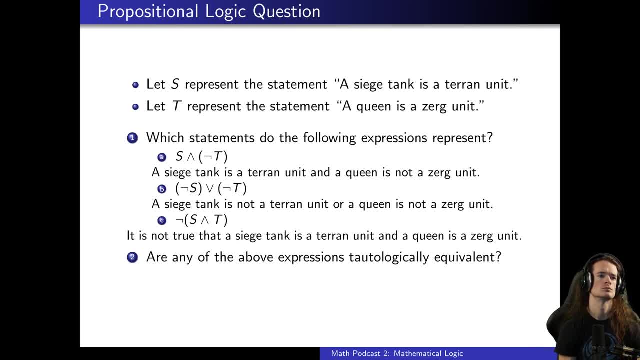 Okay. So if I said it again, if S and T are both false, then A will be false and B will be true. So those are not tautologically equivalent, But B and C are the same And chat jumped right on that. 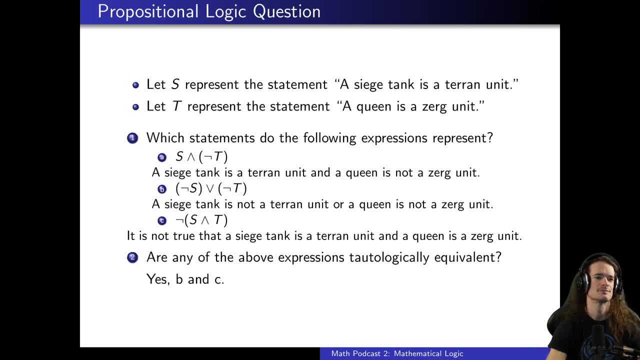 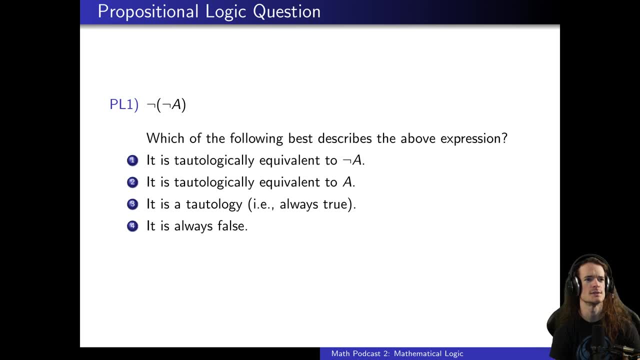 That was amazing. They got it. They got it. Let's try something else. Propositional logic, question number one: Okay, So here we have Not A. How would you best scribe that expression? Is it tautologically equivalent to not A? 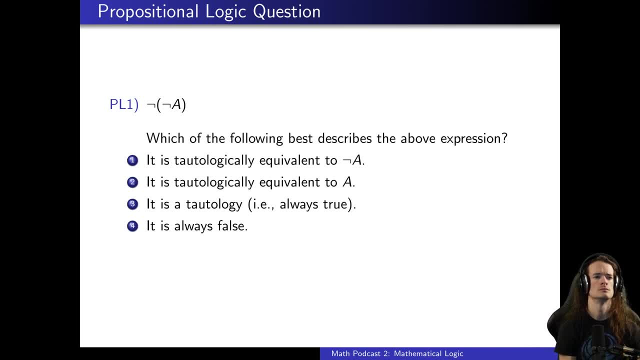 Is it tautologically equivalent to A? Is it a tautology, In other words always true, Or is it always false, Sometimes called a contradiction? You have some rock stars in chat. Yep, Logical geniuses. Chat is going with number two. 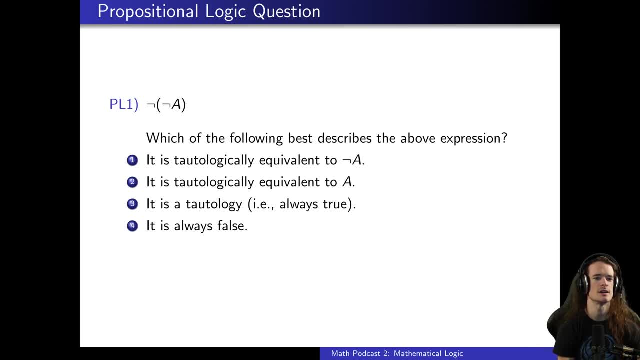 It is equivalent to A, because the not not cancels out Double negation. Yeah, So when someone uses double negative, that's like saying the same as if you were saying no negatives. So not, not. A the same as A, And we could also draw a truth table for this. 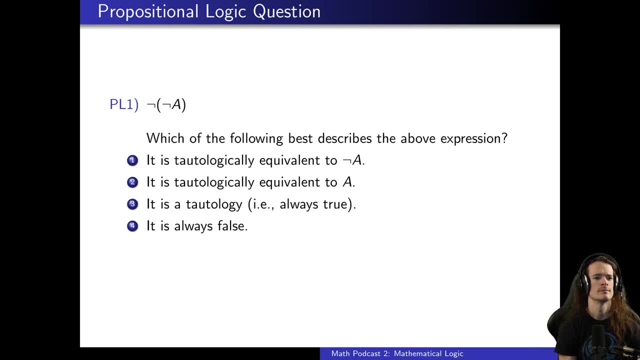 And you would see that not not A and A are the same thing, Because you'd negate once to get not A and then negate again to get back to A. It is not true that brunt is not strong. Brunt is strong. Brunt would be happy with that. 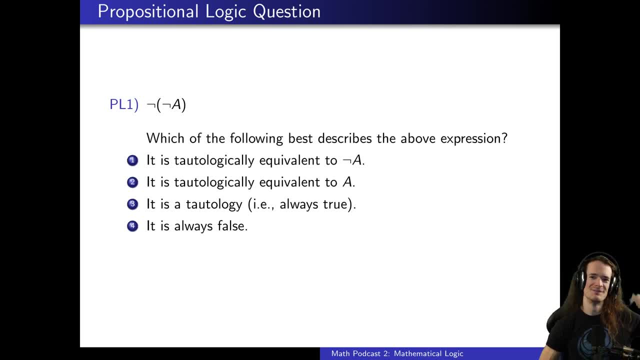 Yes, Brunt. Brunt stands by that statement. I don't not watch Naruto, There you go. So I think number two- Not of A or B- is best described by which of the following: It is tautologically equivalent to not A or not B. 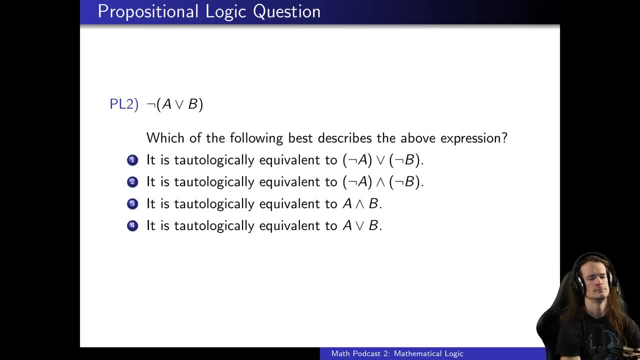 It is tautologically equivalent to not A and not B. It is tautologically equivalent to A and B, Or it is tautologically equivalent to A or B. Hmm, Answers are starting to come in, So let's see. So which of these is equivalent to? it is false that A is true or B is true. 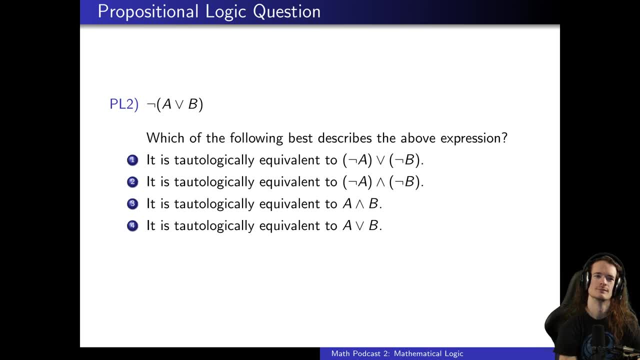 So it's A or B is false, Which is the same thing as saying that What has to be true for A or B to be false. Wow, Not only do we have some twos, we even have a two with a box around it. 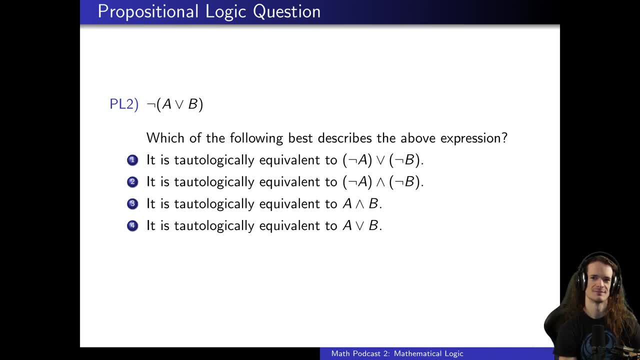 Yeah, Impressive. So for A or B to be false, You need not A to be false. I'm sorry, You need A to be false and you need B to be false. So again, the answer is two. Yep, This kind of looks like a similar format to the previous example that was given. 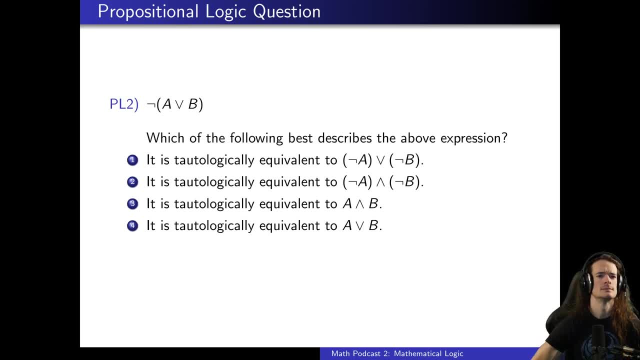 Indeed, And these are both instances of what is called Yeah, This is examples like this, or instance of something called De Morgan's law. So this is. we had a similar example in the earlier statements and we had something just like in the truth table. 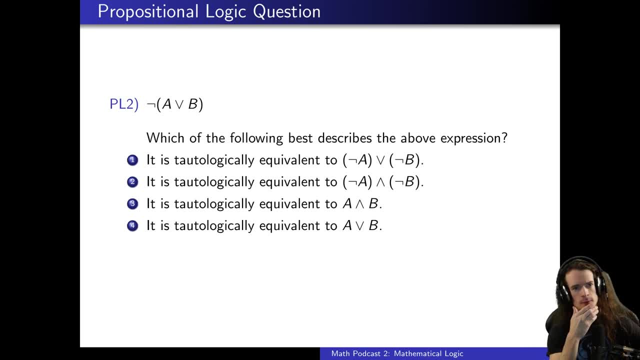 And so what happens when you negate? This happens when you negate an or or an, and and the or or and flips to the other one. So basically, you flip everything. So let's just think about this as like, just like a, as if we were like a robot. 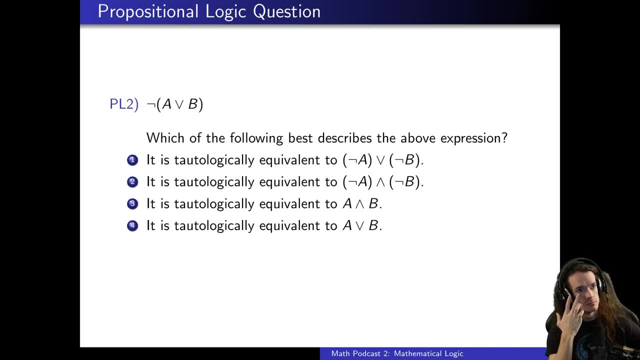 So you have this not applied to A or B. You negate everything and you flip the upside down V to the V to an upside down V or vice versa. So we take not A, flip the V not B, So you just flip everything. 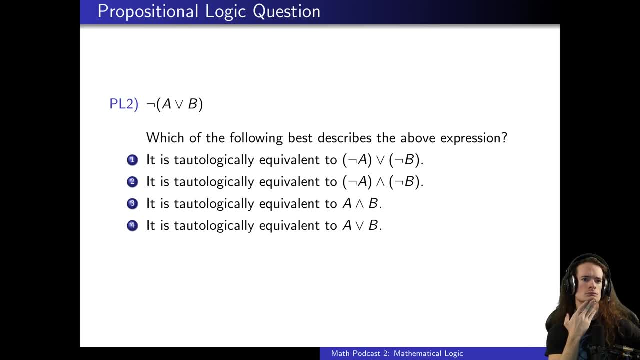 So it's just, we can just. Instead of thinking of it logically, we just think of it like a robot, just the symbol manipulators. And if we flip all of the symbols, we get option to not A and not B As a result of negating A or B. 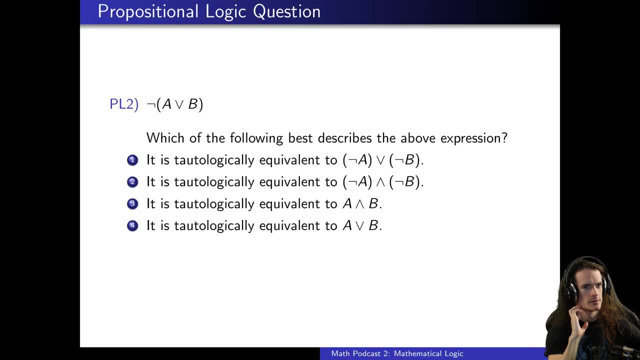 And it's okay to, to use different strategies for whatever appeals to you. Intuition the best. Yeah, I remember when I first learned this stuff. Yeah, Whatever, Whatever worked, worked. Yeah, I've talked with some other friends who took similar courses with me. 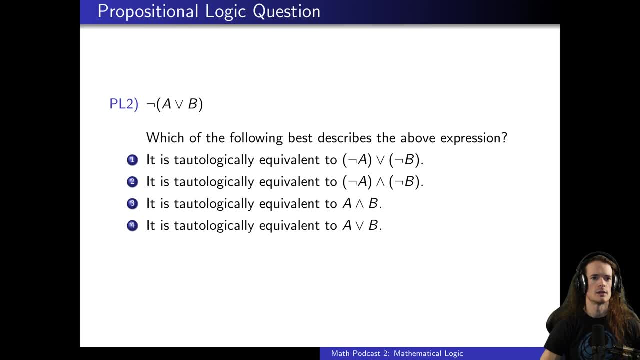 And it's interesting to see how different people's minds work and how they can frame the same problem with an approach that is more in line with their intuition. There are some friends who I would describe as having a very builder oriented mindset, where they want to make sure every block they understand why it goes there. 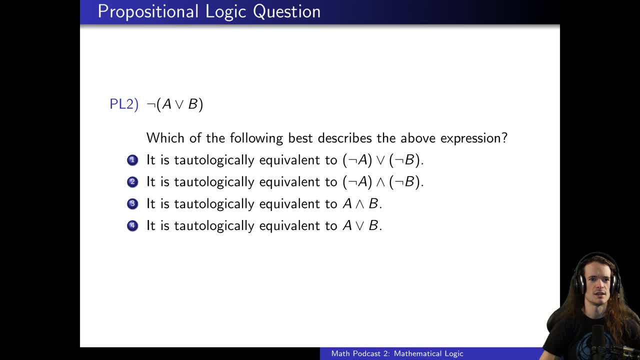 For me. I tend to see a big pattern and I go with my instinct. And if that's right then I consider my intuition up to snuff. But I don't necessarily look at every single piece For this one when it popped up. my instinct goes for two. 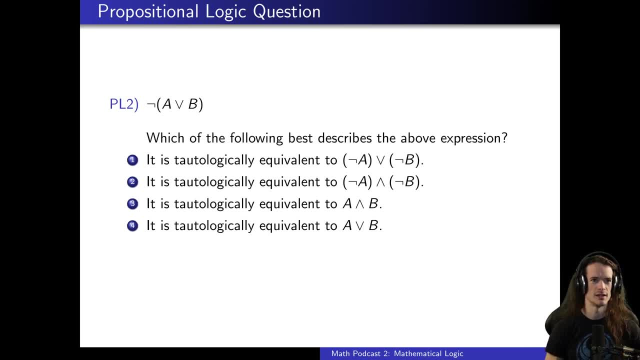 But I didn't necessarily have that full understanding of why It was just seeing the pattern pop up again. Yeah, absolutely I think. I think this is like a real dichotomy of how people. some people think bottom up and want to take all the little pieces and build it into like a building. 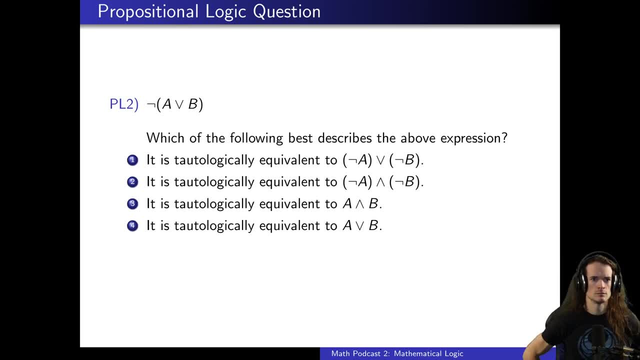 And the other people are trying to appreciate what buildings look like and then try to chop the building up and say, oh, it's built out of blocks. And coming at it from both ways is, I think there's two very different but totally different. 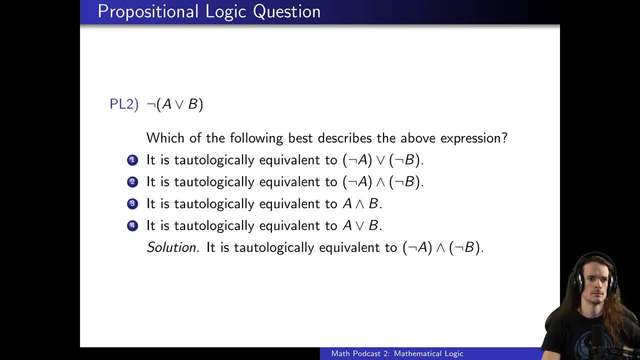 Yeah, Acceptable ways. Let's see if we have another one, Number three. Ooh, So we have A and B implies B, Or stated differently? if A and B, then B. Which of the following best describes this? Is it tautologically equivalent to A? 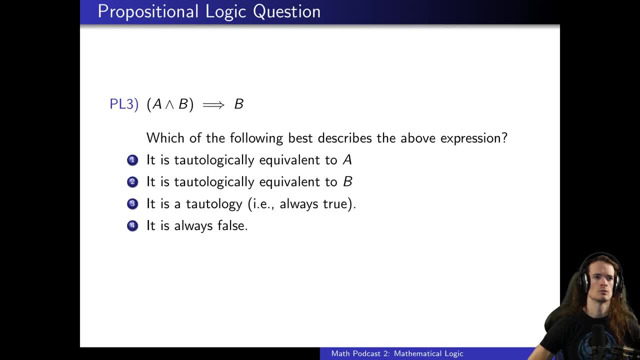 Tautologically equivalent to B. Is it a tautology that is always true, Or is it always false? Hmm, I think it's easier here to assign each letter to a phrase that we visited before. Oh, please do Do so. 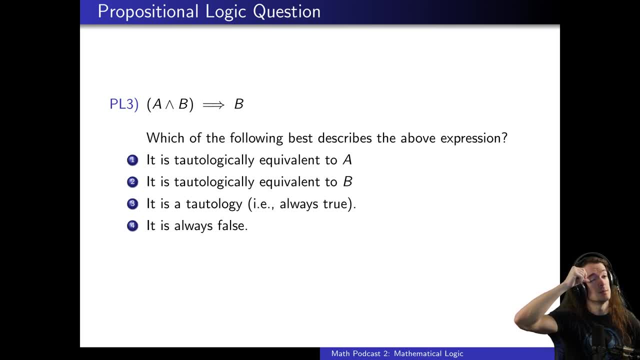 Let's say: A is brunt is a tauren, B is brunt is strong And then B- brunt is strong. If brunt is a tauren and brunt is strong, then brunt is strong. So that seems like a tautology to me. 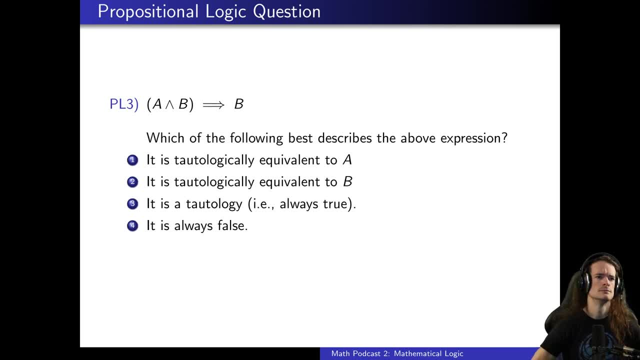 Absolutely. So you established a case where A and B are both true, And it's certainly true And, in general, if A and B are So, yes, having A and B should imply B, because you have both of them, So both should imply just one of them. 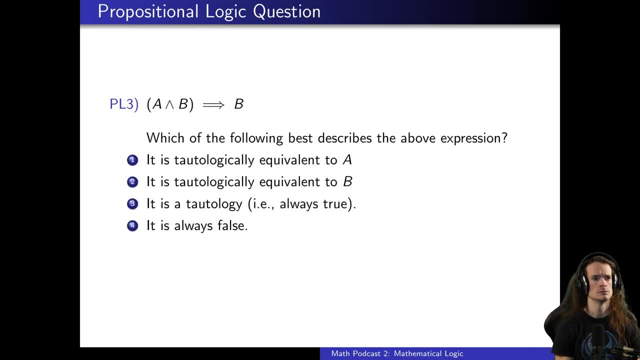 And similarly it's also the case that A and B implies A is also a tautology. So, right on the money, If we could also have used the truth table or reasoned it out like: okay, if B is true, then the conclusion of this conditional, this implication, is true. 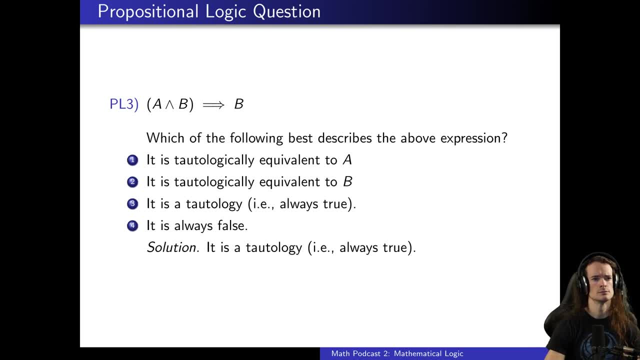 So then we're immediately good If A is true. Oh sorry, Let me say this differently, Let me not talk about A. I said: if B is true, then we're done. If B is false, then the hypothesis is false. 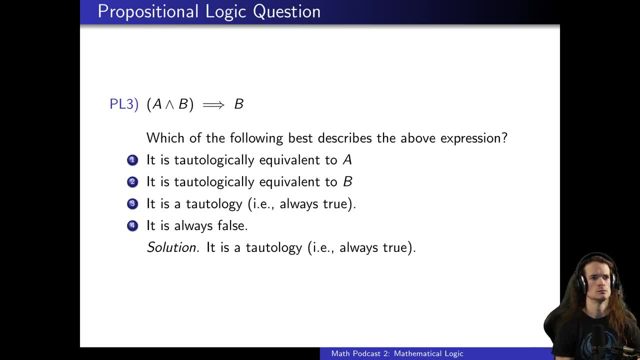 And then we're again true. So, reasoning it out, we could also see that it's always true, The two cases being: B is true, the conclusion is true, B is false, then the hypothesis is false And we're good. Well done, sir. 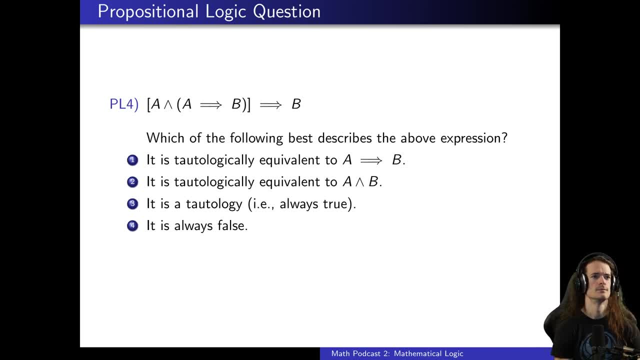 Intuition is good. Yeah. Number four, I think. yeah, we just have two left, And then we'll move on to first order logic. So let's see what this one is. Ooh, It has more symbols in it. 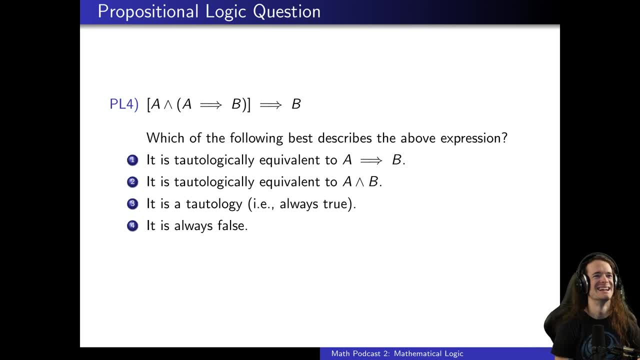 We have brackets now. Oh no, Okay, Let's think about this. We're getting a little trickier. Hmm, We'll see how chat does? They've been knocking them out of the park so far. So if A and A implies B, then B. 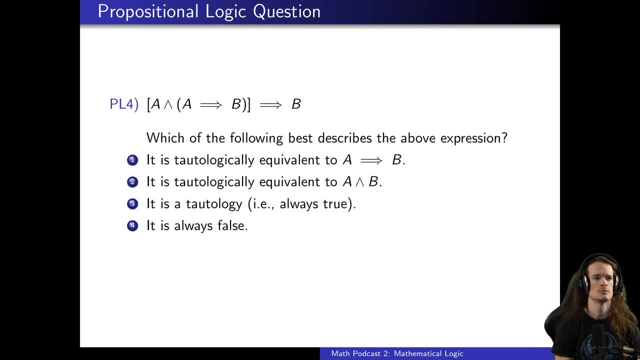 So let me say that one more time: If we have A and we have that A implies B, then B. Which of the following best describes this expression? It is equivalent to A implies B. It is equivalent to A and B. It is always true. 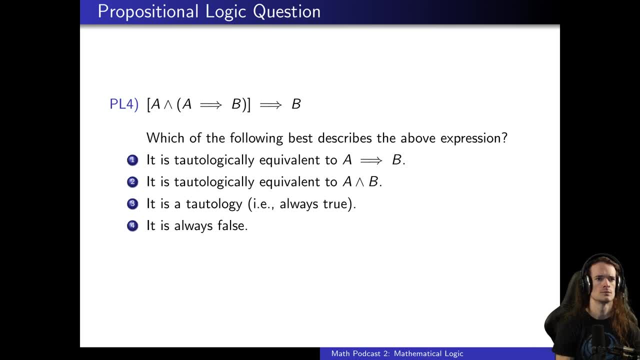 Or it is always false. Hmm, Very active chat, So let's think about this. So varied answers. I see also the same people answering different answers, So it's just like hidden all bases. Good, So the idea here is that if A is true and A implies B is true, right? 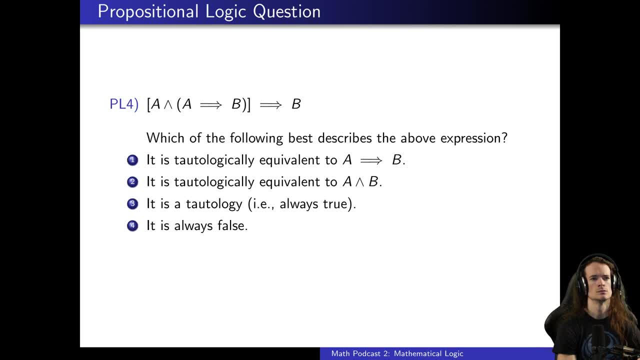 We would expect that to imply B all the time. So this is exactly the case of where I would say: let's say, if it rains, then the lawn is wet, And I also tell you that it rains, Then we would always expect that to then to be able to conclude that the lawn is wet. 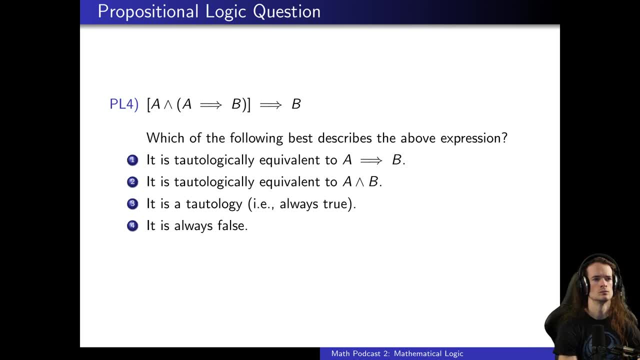 So we have a premise implying like a condition, a hypothesis implying a conclusion, And I tell you that the hypothesis is true, Then you should be able to conclude the conclusion. But let's think about it a little more methodically, by just going through what the values are. 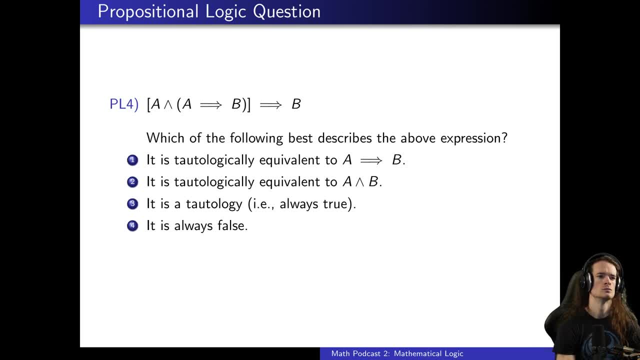 So if B is true, we are done, Because then the conclusion is true. So we only have to handle the case where B is false. Now, if B is false, Then we look at A, And if A is false, we are done. 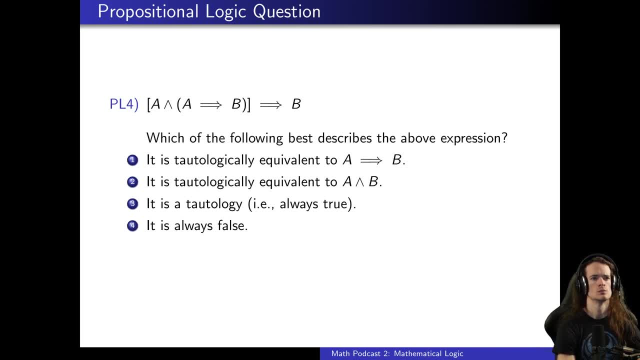 And if A is true, then A implies B is false And again we're done. So that's a little harder to work out mentally And maybe a truth table here, if you want to like fully get it all down, is like the best methodical way to go. 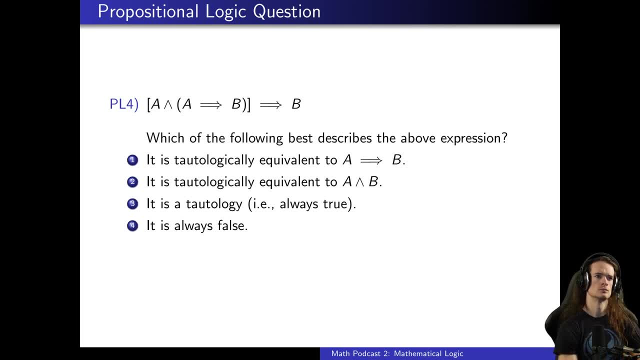 And I invite people to do the truth table And maybe in the future we could do a few more truth tables if we want. But if you do the truth table here, you will see that it is always true And this is what you'd hope this would always be true, because this is what you want to be, is one of your ways of like deducing something. 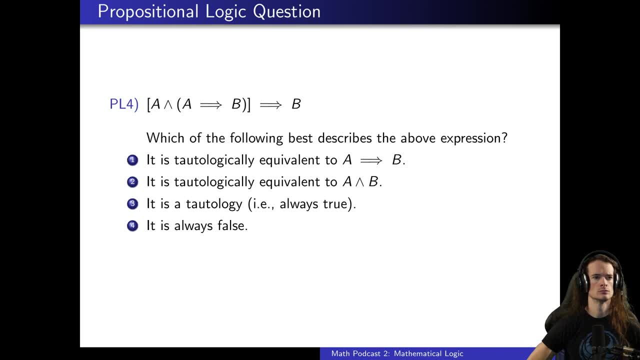 You want to be able to say that if you have something true and then you know if that's true, then something else is true. you want to be able to say that other thing is true. So if you have A and then you know that A implies B, then you want to say that B must be true, and that is the case. 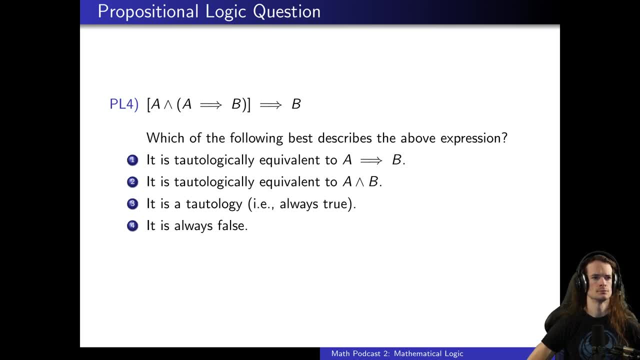 So if you have A and A implies B, then it is true that you have A, And if you have B, then it is true that you have B. Yeah, And this is a deduction rule. sometimes Got a mixture of ones and twos in the chat for this one. 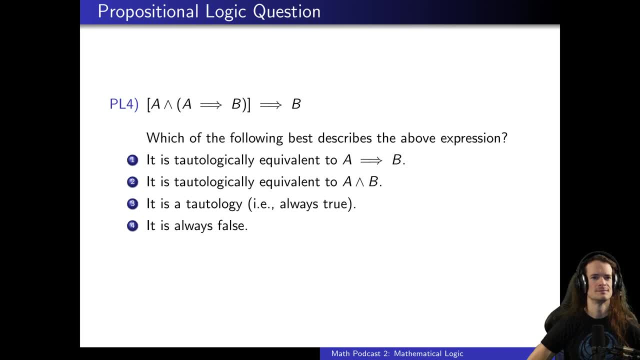 This one is sneakier. I mean, we had a lot of letters here, So it is not the same as saying A implies B, So A implies B is sometimes false. So an example would be: let's see how they're different. So A implies B is false, when A is true and B is false. 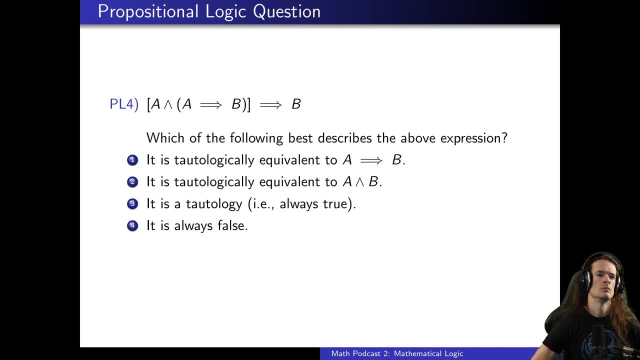 So let's see what happens when we plug A true and B false into the statement we have. So let's try to do that. So if we plug A true, we have true for the first day and we have true for that second day. 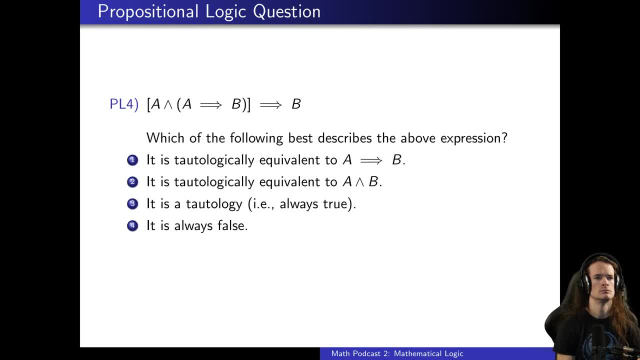 And then we have B false, So A implies B is false. when A is true and B is false, Which means this entire and statement is false, Which means this implication is true. So it can't be the same as A implies B, because when A is true and B is false, number one is false. 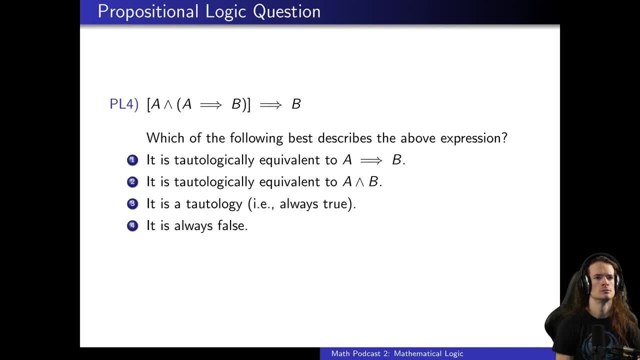 But the question PL4, the statement in the question is true in that case. In fact it's always true, And the same case breaks number two and shows that it's not the same as the question. So it is indeed always true. 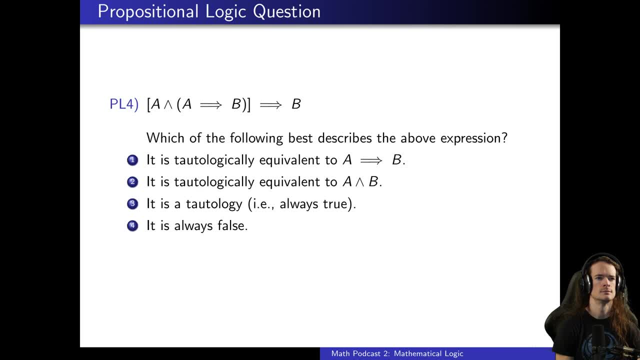 And this was a little tricky, And sometimes it's good to have something that's a little tricky, Because I know you want to have something that challenges your thought and makes you have to think a little more deeply, Because sometimes all the exercises are just obvious. 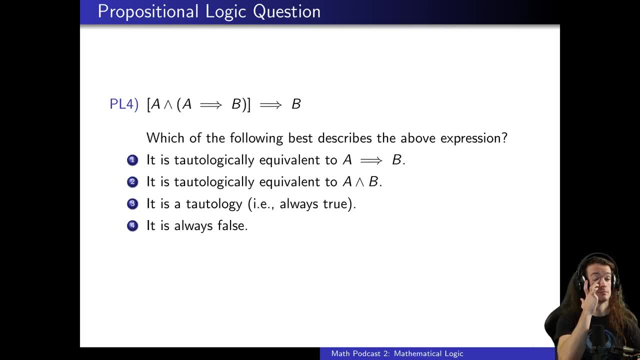 You don't have that moment where you have to pause and really like think a little deeper about it, And sometimes it's good to just have one or two that are just tricky a little bit, And this one is a little tricky, So we'll have one last one and then we'll move on to another topic. 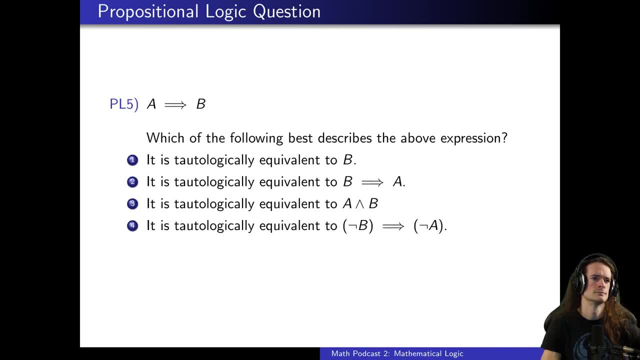 A implies B. Okay, That's less symbols. I've seen this one already. Less to read. What best describes the above expression? A implies B. It is the equivalent to B. It is equivalent to B implies A. It is equivalent to A and B. 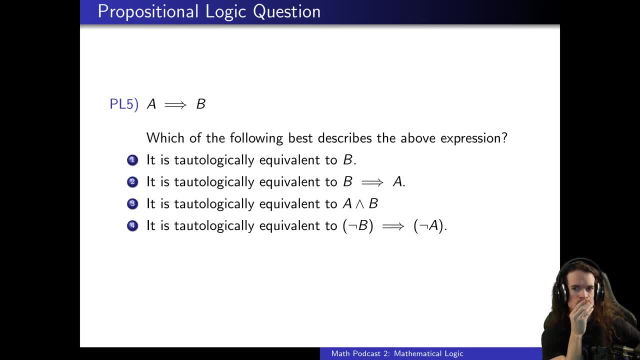 Or it is equivalent to not, B implies not A. Oh wow, People jumped on this one. Yep, Lots of fours. Oh my Okay, So let me first talk about two. So when you have the statement if A, then B also, or stated equivalently, A implies B, if you flip them around and say B implies A, that is a different statement. 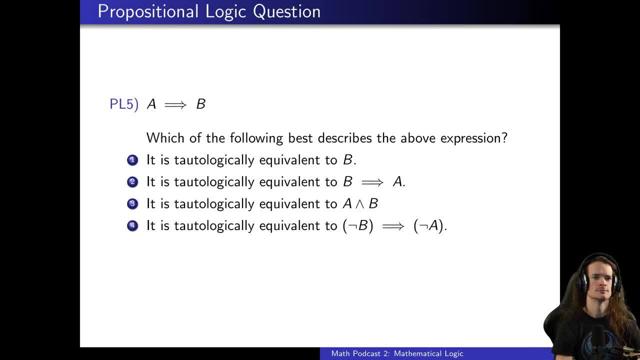 And that is called the converse And that is different. So as a statement, we'll come to later. If you were making a statement like all torrents are strong, If you're a torrent, then you're strong, That should be different than saying if you're strong, then you're a torrent. 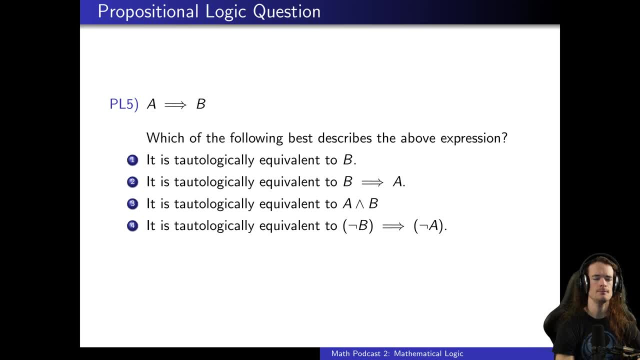 Yeah, Because one is saying that torrents are strong And the other is saying everyone who is strong is a torrent. So those are different. So the first statement and two should be different. Unfortunately, the argument I just got, that very intuitive argument, is a first-order logic argument that we're going to talk about later. 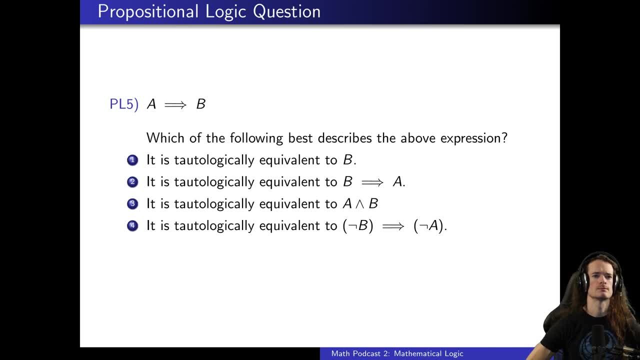 So here you can just go through some cases and figure out. Let's go through some cases and see that they differ. So one case they differ on. So suppose A is true and B is false, Then the implication A implies B is false. 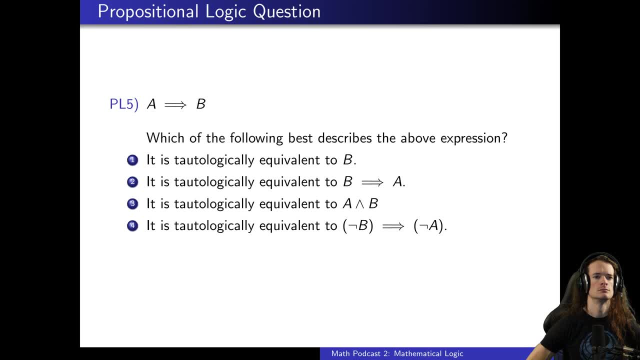 But B implies A is true. So you already see a place where they differ. So A implies B and B implies A can't be the same because they differ when A is true and B is false. As an example, Just to tie in here. 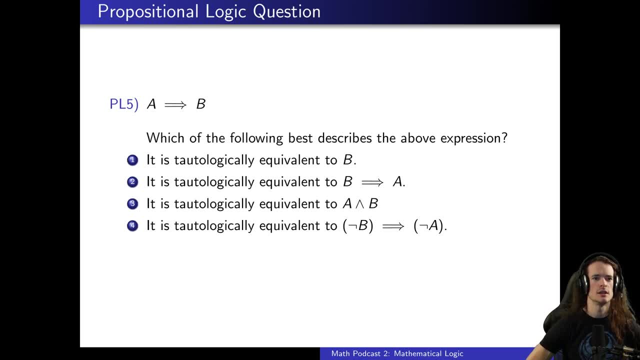 Converse then would be flipping what you're looking at horizontally, And A would be flipping it upside down, So the regulars would become nots. Yeah, So I think I haven't specifically talked about negating an implication, But you could do that too. 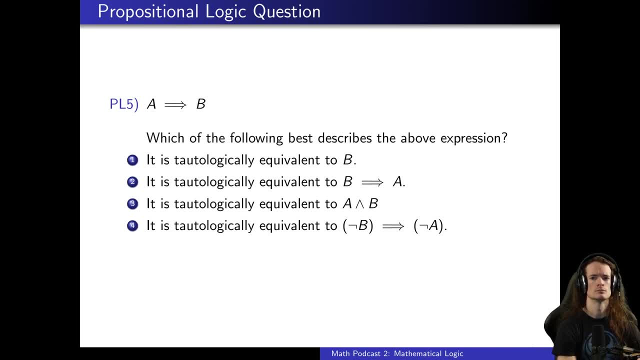 So maybe we'll talk about that right afterward, because that's a really good point. So the correct answer is 4.. And the way you get that is you converse and you negate both parts, And that's what you call the contrapositive. 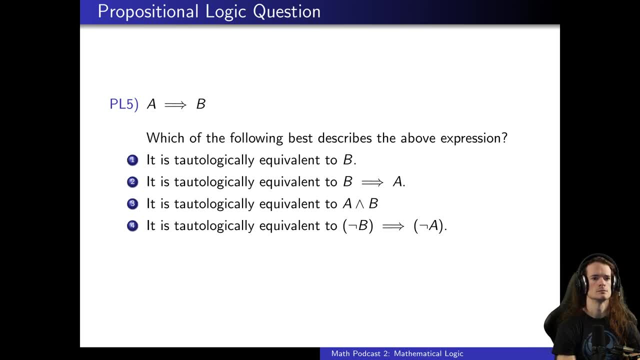 And so 4 is the same as the statement. 4 is the correct answer. So what is the negation? Neuro asks a great question. What is the negation of A implies B? So when is A implies B false And the negation of A implies B is? so how do we get A implies B to be false? 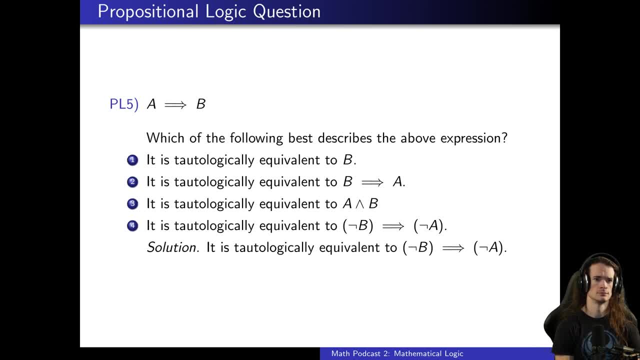 We need A to be true and B to be false. So the negation of A implies B is A and not B. It would have been smart if I put that as one of the options. In hindsight I'm like, ah, that's a great idea. 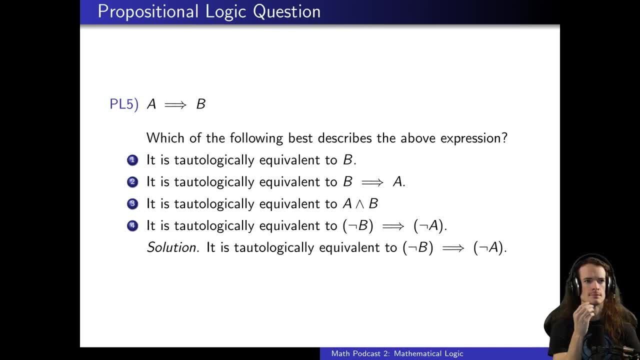 So the negation of A implies B, which I don't have here as an option, is A and not B, Which is the premise, the hypothesis is true and the conclusion is false, That's, the negation of A implies B. Great question Neuro. 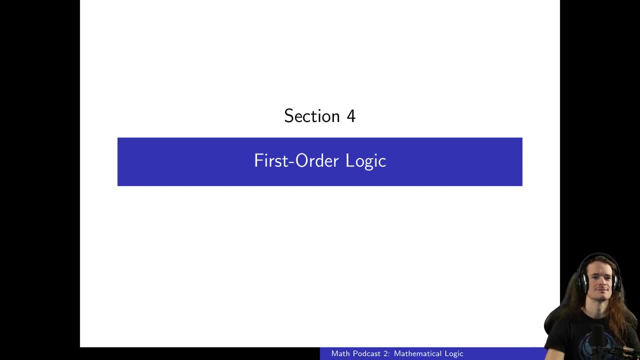 Superb. So we did it. We did some warmups, We learned about prepositional logic, We did some questions. It's great, And now we're into it, Section 4, first order, logic. And there's a lot of things we can't do with prepositional logic that we're going to be able to do now. 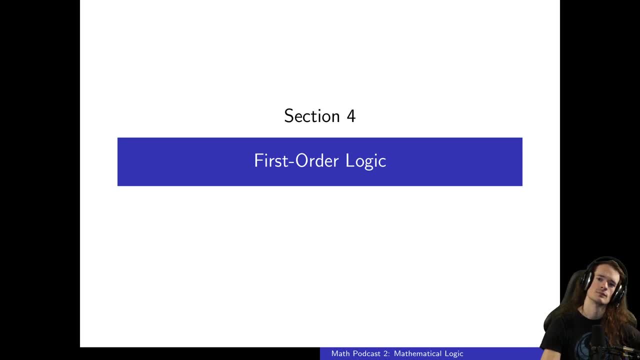 And so a lot of most mathematical statements you make in first order logic, And you'll see why- Because there's a few things you want to say that are crucial, that you can't say yet, And basically it's going to be variables and quantifiers. 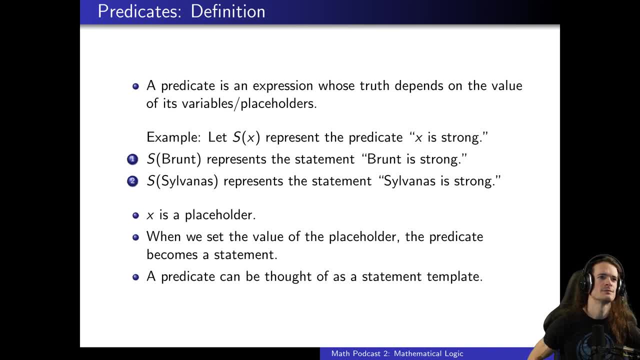 So let's get right into it. Let me say it Predicates Definition. So we have predicates. So a predicate is an expression whose truth value is predicated or depends on the value of its placeholder or variable. So let me give you an example of a predicate. 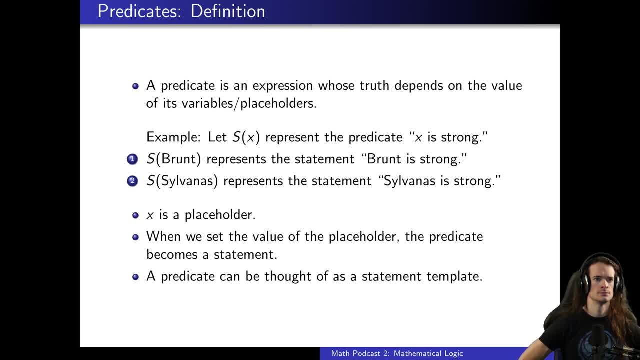 The predicate which we represent with a symbol S and then in parentheses, X represents the predicate X is strong. So let me give you two examples of how we could use that predicate to make statements. So suppose we plug in for X. X is a placeholder. 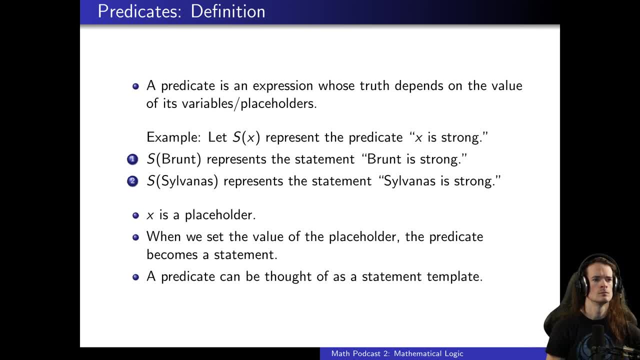 So we replace X with the name brunt. So if we just plug brunt in where X is in the predicate, we get the statement brunt is strong. Or if instead we plug Sylvanus in where X is, we get Sylvanus is strong. 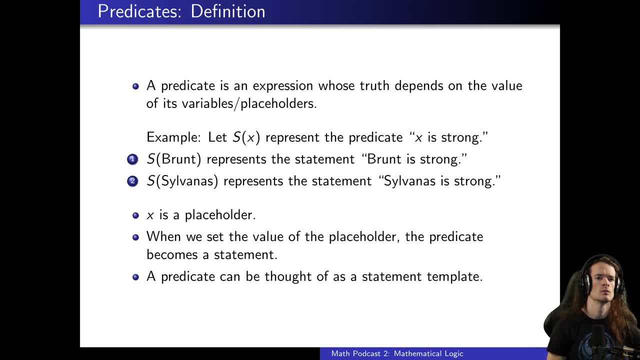 So this predicate S of X- that's how you could read it, the S parentheses, X parentheses- you could read it like S of X- is a statement template. It's like a statement maker: You plug in things for X and then you get statements. 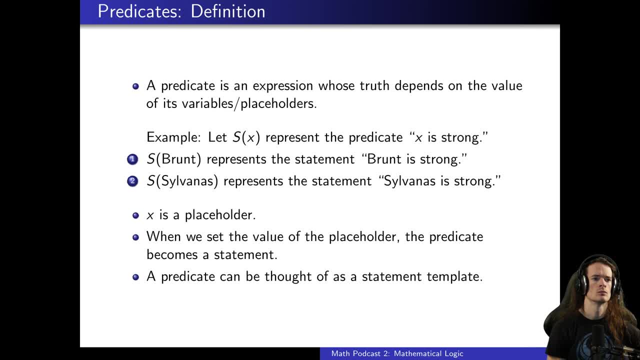 It's kind of like a template letter, Like you're writing a letter to all your characters and you just plug in brunt and you get: brunt is strong. And then you want to also send a letter to your other character but plug in their name. 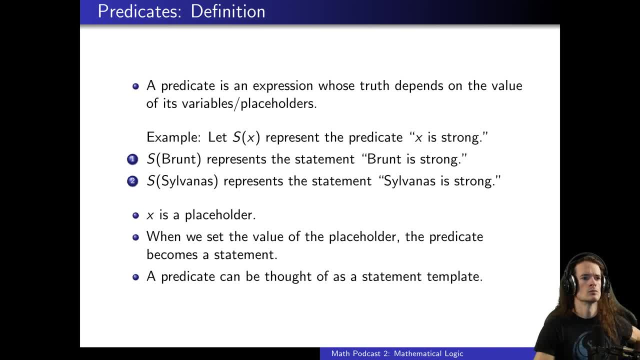 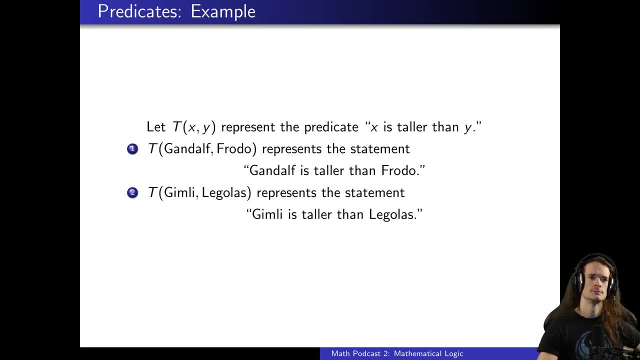 So it's a template for making statements and you just plug in for the place for the X and you get new statements each time. Now we know what a predicate is. Got predicate Okay. So here's another example: A predicate that uses two arguments. just to show you can do that. 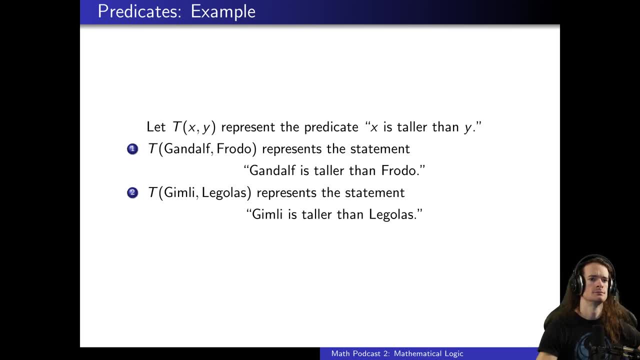 They could have more. So this is an example from Lord of the Rings. So let TXY represent the predicate that X is taller. So if we have T of Gandalf comma Frodo, that will represent Gandalf is taller than Frodo. 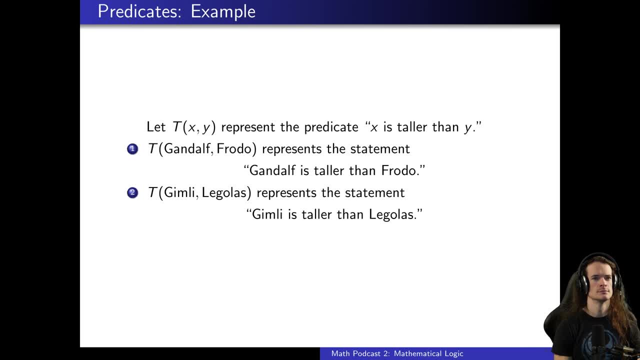 And if we have T of Gimli comma Legolas, that would represent the statement: Gimli is taller than Legolas And the first is: Gandalf is taller than Frodo is true and Gimli is taller than Legolas is false. So another example of using a predicate: 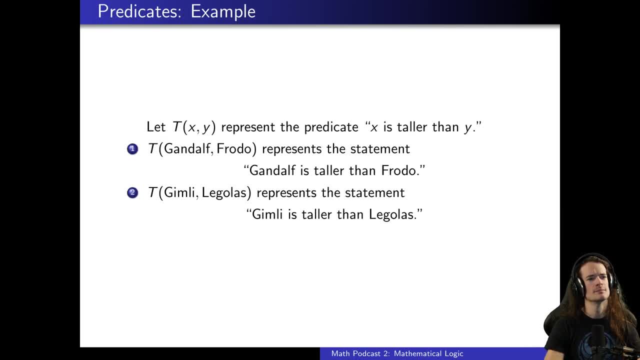 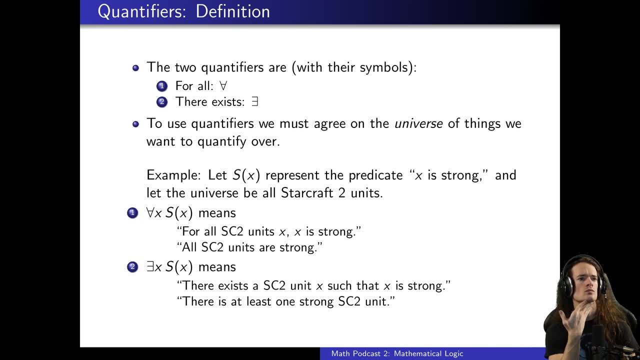 And then you get these variables X and Y, and then you can plug in for them, And one of the great things you can do with predicates comes next Quantifiers. So this allows us to say things like something holds true for everything or holds true for something. 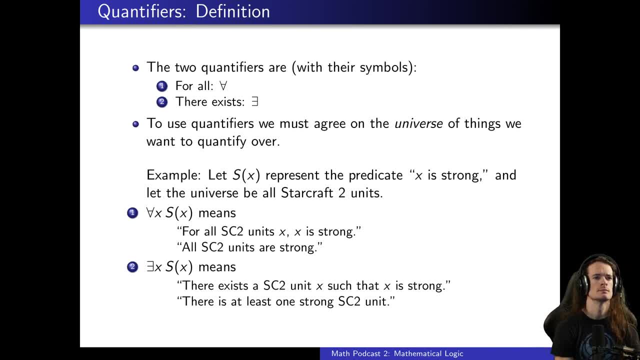 So the two quantifiers are for all and the symbol you use for for all is the upside down A, A like all. So you just make the A upside down and you get for all. That's the symbol. And then, for the quantifier there exists, use an E, but a backwards E. 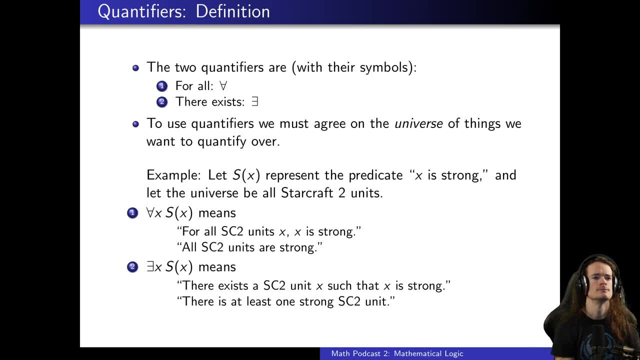 A backwards capital E. So an upside down capital A for for all and a backwards capital E for there exists. And then to use a quantifier, you have to agree on what the universe is you're talking about. So when you say for all, you want to make sure you confine yourself to some domain of interest. 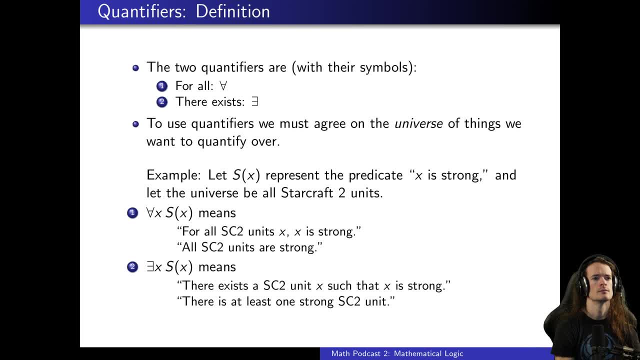 So maybe it will be all Starcraft 2 units, Or all World of Warcraft characters, Or all characters in the Lord of the Rings universe, Or maybe all numbers Or all sets when we later talk about it. For all Twitch streamers there exists a terms of service agreement. they must abide. 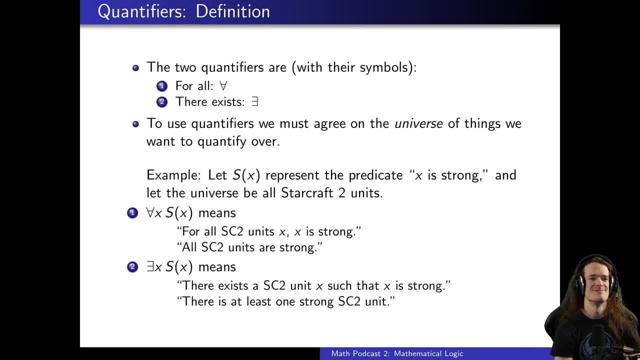 Indeed Very relevant to Twitch streamers. Yeah, So here's an example where we'll talk about Starcraft 2 units. So we'll let S of X be the predicate that X is strong, And we'll let the universe be all Starcraft 2 units. 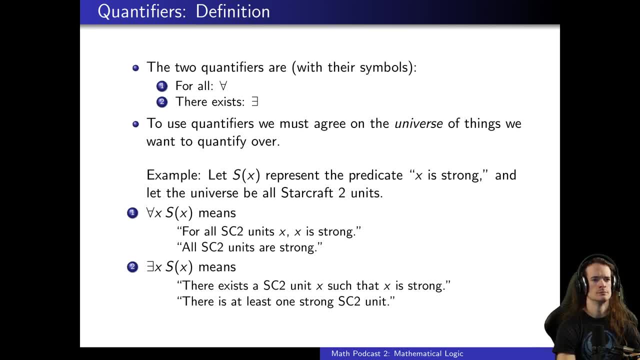 So if we use the upside down A X to mean for all X, So if we have for all X, S of X, that means- and there's a few ways, there's a lot of equivalent English ways you could say this, but a few ways would be: for all Starcraft 2 units, which I call X. X is strong. 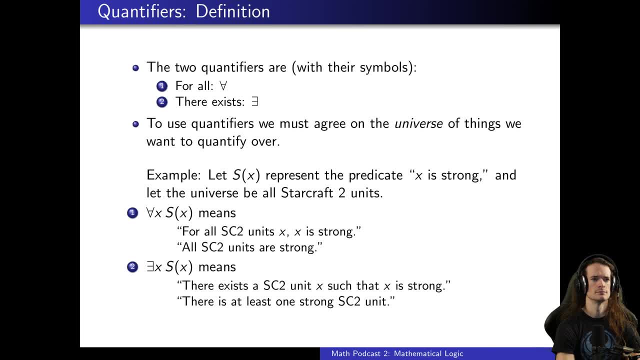 But maybe a more Common way of saying this would just be to say that all Starcraft 2 units are strong. So that's what this, for all X, S of X means, given that the universe is all Starcraft 2 units. 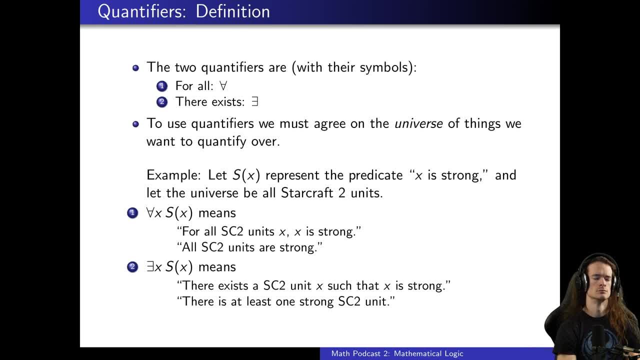 And S of X means X is strong. So we can use this sequence of symbols to say all Starcraft 2 units are strong. If instead we use the backward Z symbol, we get there is at least one strong Starcraft 2 unit. 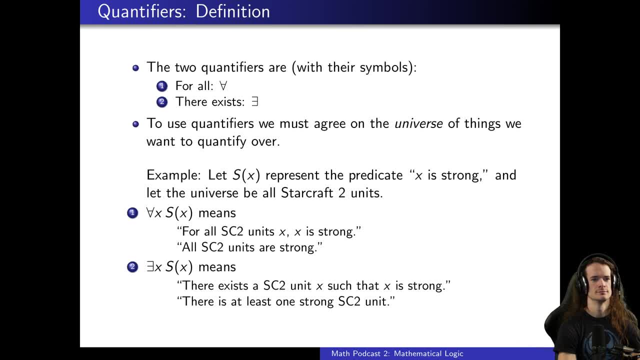 Or another way of saying it is: there exists a strong Starcraft 2 unit, Or there exists a Starcraft 2 unit which we'll call X, such that X is strong. Lots of different ways of saying there is at least one. 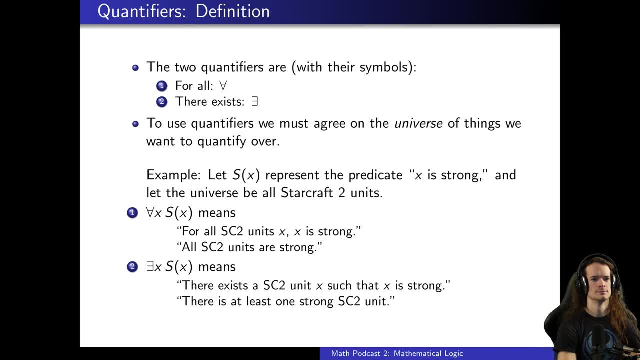 So exists means another way of saying there is at least one. So we have two quantifiers. We can say everything for all and we can say there exists, And now we've got. we've got, that's got first order logic. 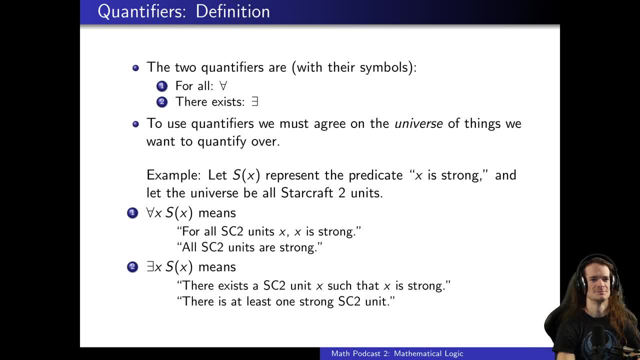 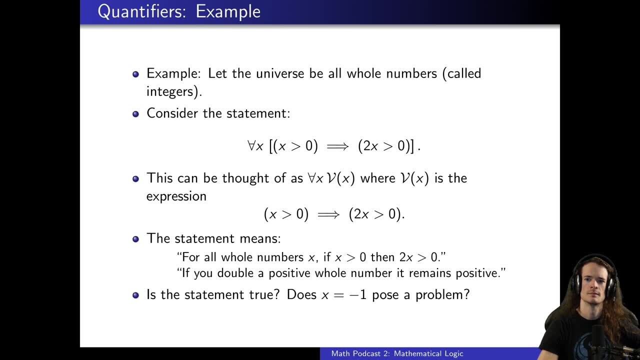 Maybe we thought it was going to be terrible, but that was it. So let's, let's go through another example to test out our understanding of first order logic, And this one will be a more mathematical example. So we're going to let the universe be all the whole numbers, also called integers. 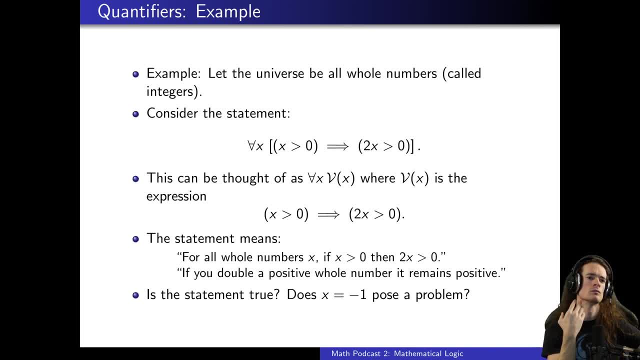 So this is like the positive number, whole numbers like 1,, 2,, 3,, 4,, 5,, 6, 7.. The negative ones: negative 1,, negative 2,, negative 3,, negative 4,, et cetera, 0.. 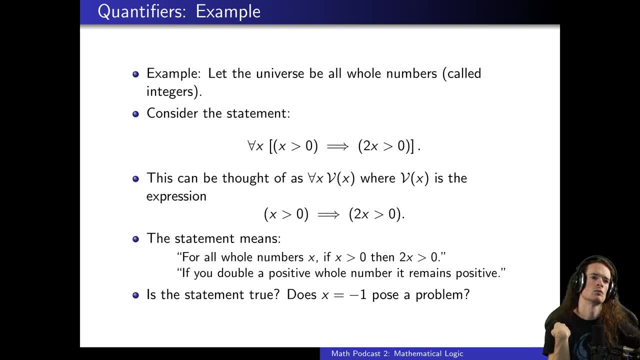 So all the whole numbers, no fractions here, And I want to consider the following statement: For all X, The following, And the following is: X is greater than 0 implies 2X is greater than 0. And you can think of this as being like for all X, and then an expression V of X. 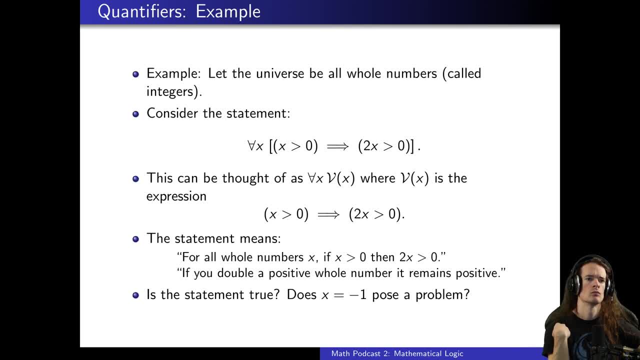 And V of X is that expression X is greater than 0 implies 2X is greater than 0. So this is for all X, V of X. where V of X is X greater than 0 implies 2X greater than 0.. 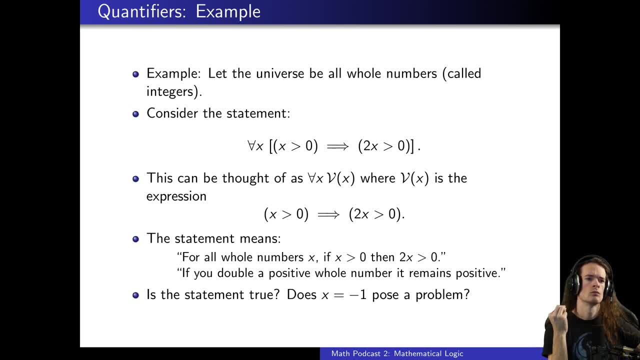 And what is the meaning of this statement if we, kind of like, set it out in English instead of me reading out the symbols For all whole numbers: X, if X is greater than 0, then 2X is greater than 0. Or maybe a little easier to say would be: if you double a positive whole number, it remains positive. 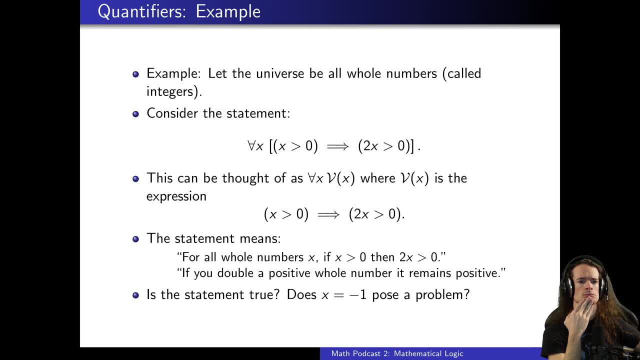 Now, first let's think: Does this statement feel true? If we take a positive whole number like 1,, 2,, 3,, 4,, 5, and we double it, add it to itself, do we still get a positive number? 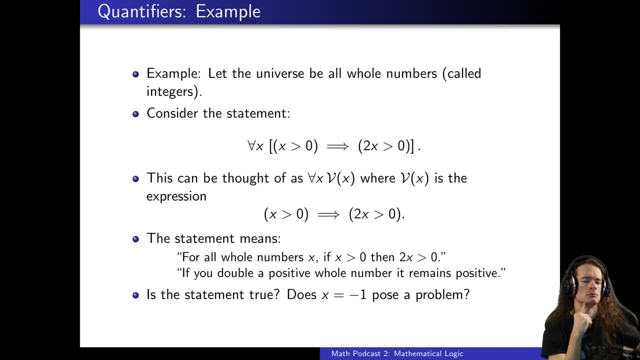 That seems true, That is a true statement. But here's a question: Does X equals negative 1 pose a problem? Because negative 1 is an integer, It's a whole number. It's a negative whole number. Because negative 1, when you double it, it's negative 2, which is not positive. 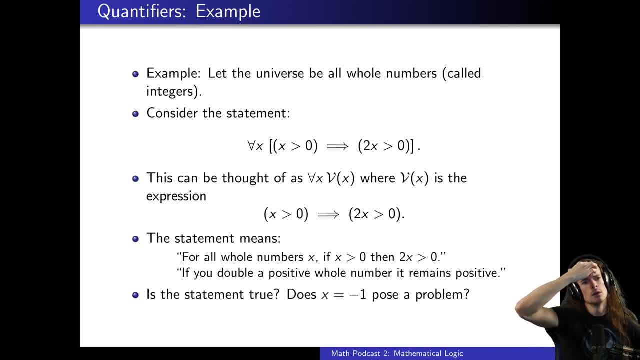 Does that mean that this statement, our statement, our for all statement is false? No, Because, as we learned earlier, if the condition statement that you start with is false, then you're done and it's correct. You don't have to worry about the conclusion. 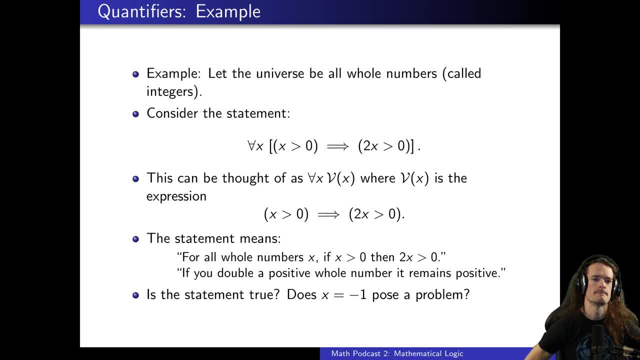 Exactly right. And now it makes a lot of sense why we would want that to be true, Why that we want, if the condition fails to hold, that we don't hold it against the statement. The statement should only be measured where the condition holds. 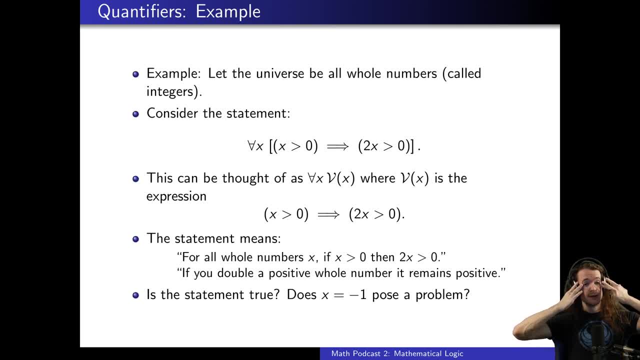 So we want to say that this statement X greater than 0, this predicate X greater than 0 implies 2X greater than 0, is always true for all X, Because, even if you, Even though the conclusion has issues when X is negative 1,, the condition didn't hold. 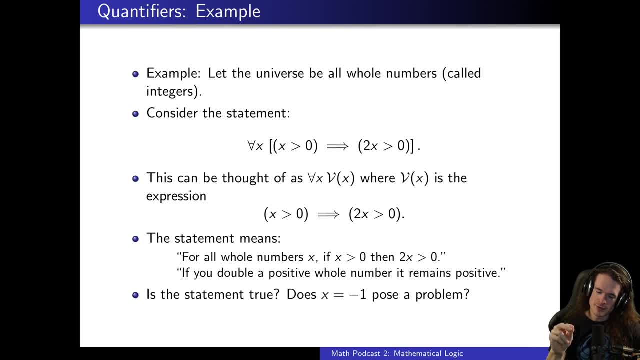 So it's like: why are you holding me against something I didn't even assume? Look, look, look, It's not the printer's fault. You can't put waffles into the paper slot. It's not meant to take that. 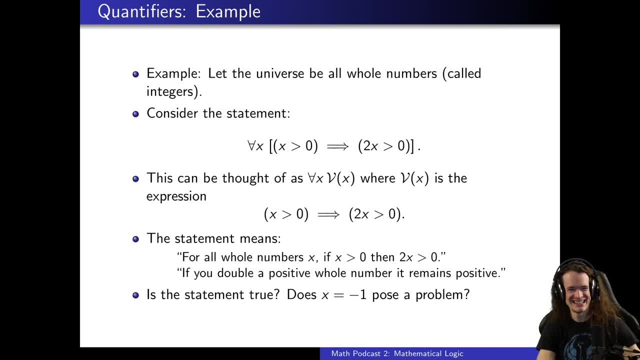 You should. I mean this is general advice. I mean, there's so many life lessons being learned on this stream. All the printers saved. Yeah, Everyone's just wondering what's going to happen if you put a waffle into a printer. 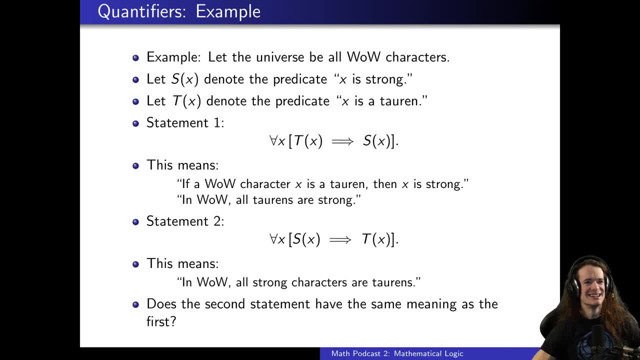 Yeah, And they're going to start putting honey and syrup in for their ink or toner. Yeah, Don't do any of these things. Don't mix printers and breakfast. The printer is fine. You're using it wrong, So let's do. another example from World of Warcraft. 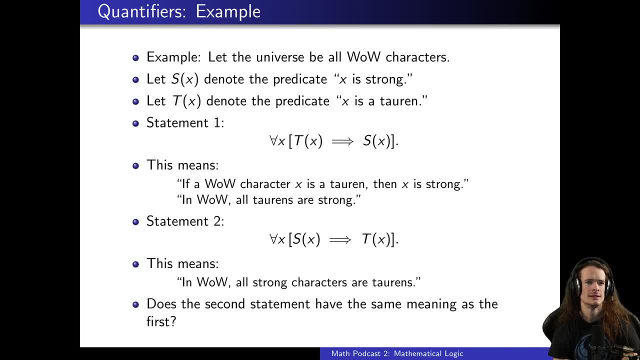 So we'll let S of X denote the predicate that X is strong, And we'll let T of X denote the predicate X is a tauren. And so now we'll do statement number one For all X. T of X implies S of X, which means not in symbols but in English. if we associate: 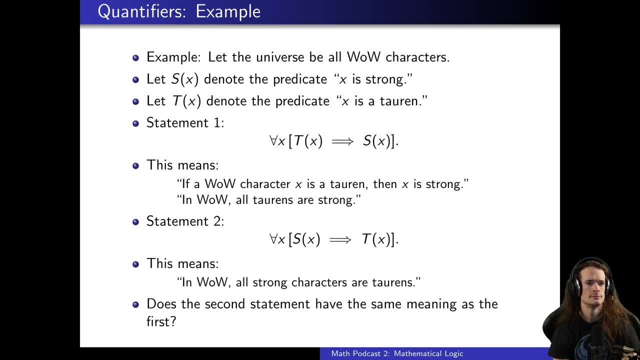 those meanings of the predicates we have. if a wow character X is a tauren, then X is strong. Or in other words, in wow all taurens are strong. So both of those are legal ways of reading those symbols. Okay. 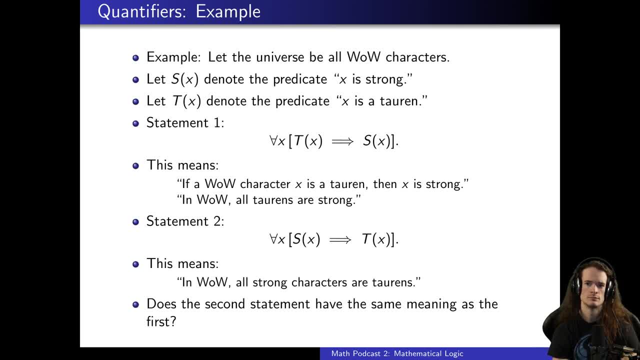 So taurens are strong. So you're saying for all units, if they are a tauren, so we restrict to the case. that's our assumption, that for all units. we're making a statement only about taurens, because that's. 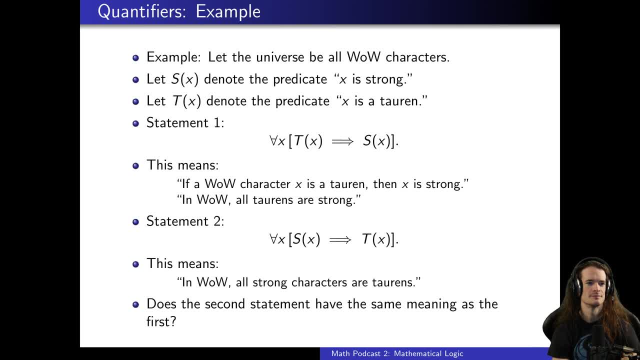 our hypothesis And we're saying: if you're a tauren, then you're strong. So we're basically saying that all taurens are strong. Now let's look at statement two For all S. S of X implies T of X. 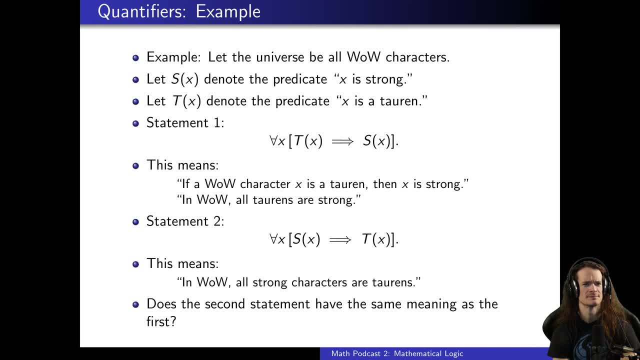 Or in other words, in wow, all characters, all strong characters, are strong. All strong characters are taurens. Or in other words, if you are strong, then you are tauren. Do these two statements have the same meaning? No, 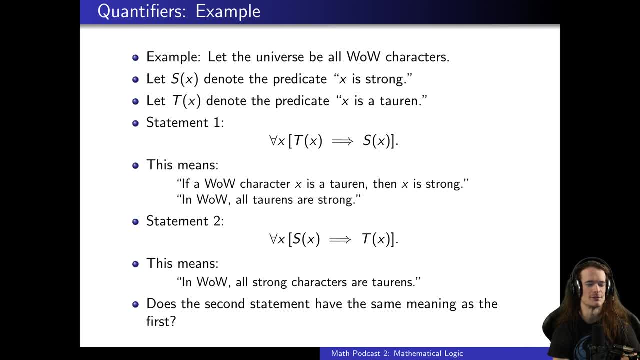 Unless strength in and of itself is inherently a tauren fighting spirit capacity, which is kind of getting into some weeds Right. So if we believe that, for example, Sylvanas is a strong character and Sylvanas is not tauren, then we're in trouble with this statement. 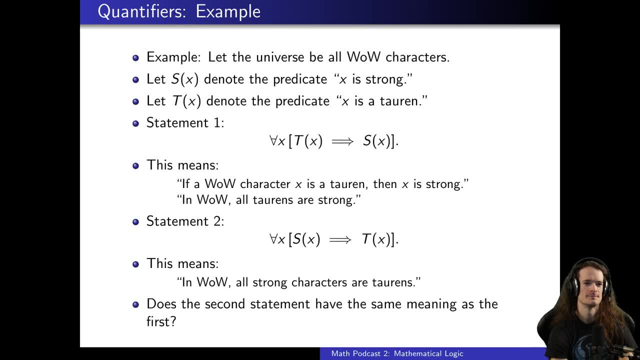 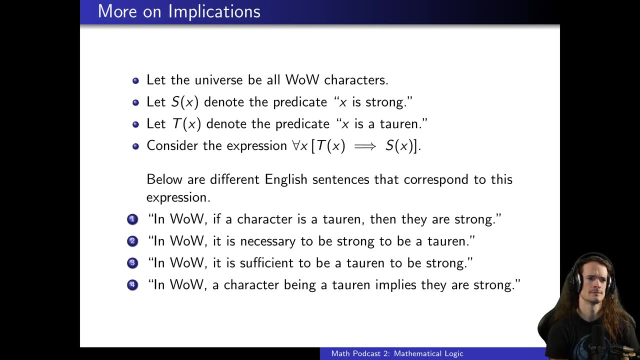 Yeah, Brunt may think this. I don't know, We could ask him. So let's talk a little bit more about implications, And then we'll be basically done with except for one more thing to say about first order logic. We're going to talk about negation after this. 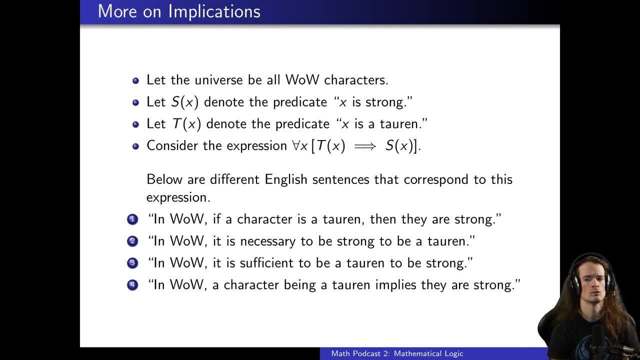 But a little bit more on implications. So let's again have S of X, be X is strong and T of X be X is a tauren, And we'll again consider this statement For all X. T of X implies S of X. 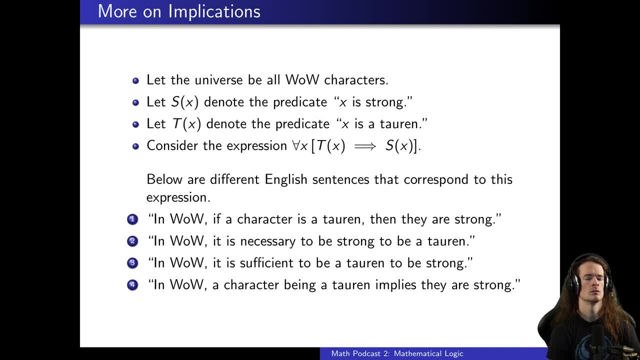 So we have different English sentences that correspond to this And I just want to get people comfortable with the different English sentences because these come up sometimes in English- definitely in math a lot. So you can say in WoW if a character is tauren, then they are strong. 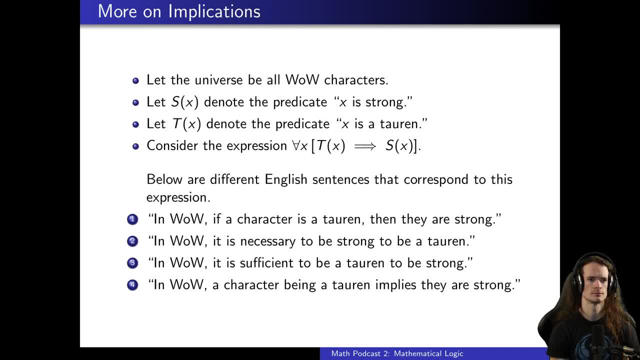 That's the one we had, one of the English sentences we corresponded with before, Another way of saying this. let's think about this: It is necessary to be strong to be a tauren. That is equivalent to the expression I have above there. 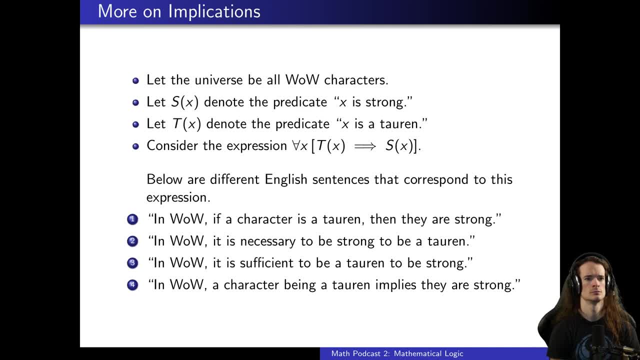 It's another English meaning And this is true If we believe that all taurens are strong, the saying it is necessary to be strong to be a tauren is a true statement. Let's think about that, Let's think this through. 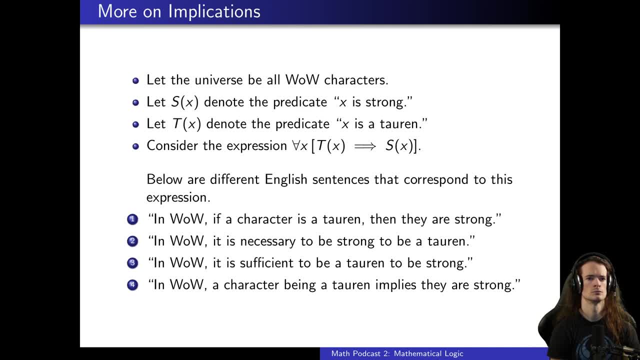 If you are not strong, you're definitely not a tauren. if you believe that all taurens are strong, So a necessary condition to be tauren is to be strong, Well you're huge. So if you're not strong, you can't move. 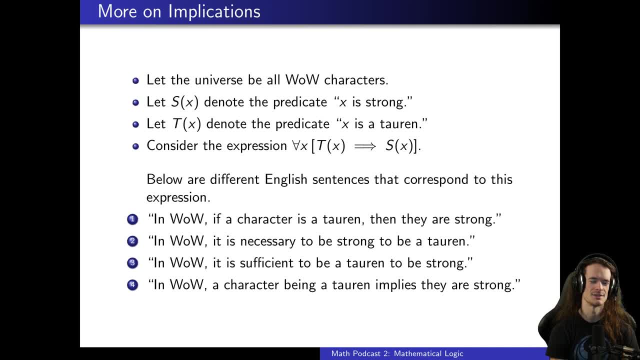 And then you die. Yeah, That's bad. It is actually vital to move yourself, to get bread from the baker Indeed Or go for a hunt. These are bits of knowledge from an experienced WoW player. Brunt: half a ton mist runner. 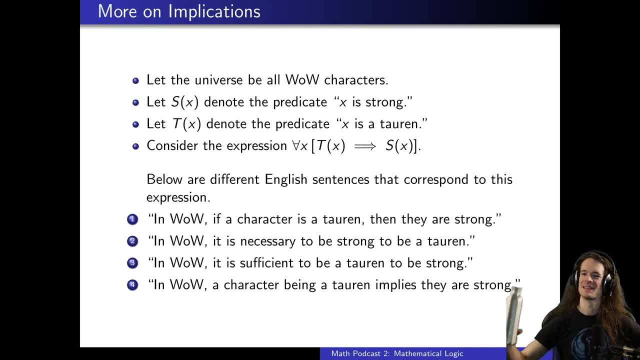 Brunt, half a ton mist runner. Brunt, half a ton mist runner. so another way of saying the exact same thing is to say that in world of warcraft, it is sufficient to be a tauren to be strong, so it is a sufficient condition. 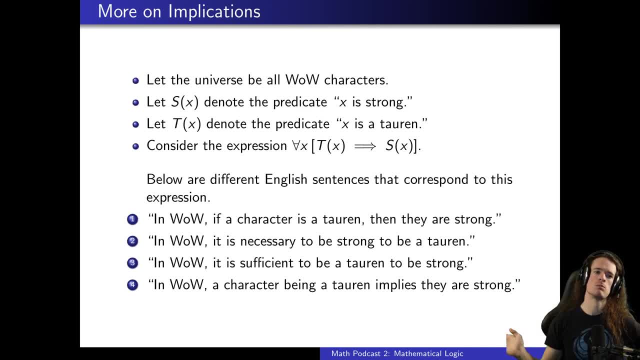 to being strong is to being a tauren. so if you know someone's a tauren, then you know they're strong. it's sufficient to know someone is strong. if you want to, if you want a sufficient condition to tell you whether or not someone is strong, it's sufficient to know they're a tauren. because if you 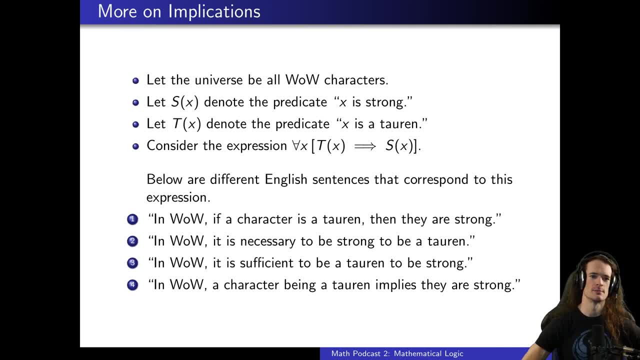 know they're a tauren, then they're strong. all i need to know about this bodyguard mission is the person applying. if they're tauren, they're fine, they're going to be strong enough. so someone's asking in chat, so the sentence: all taurens are. 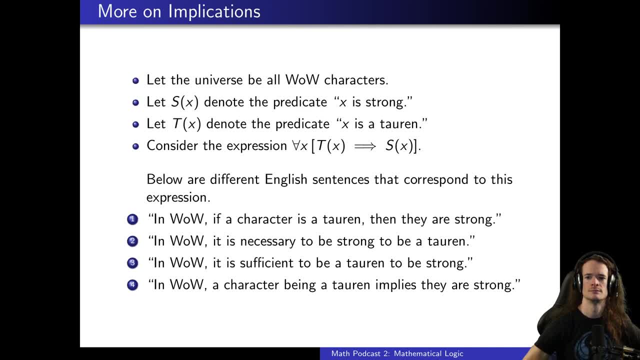 strong does not ban the possibility that elves are strong. correct, if and if this and if i said instead only taurens are strong, then nobody else can be. yes, so you definitely with that statement nailed that whole: t implies x versus s implies t. we had before. 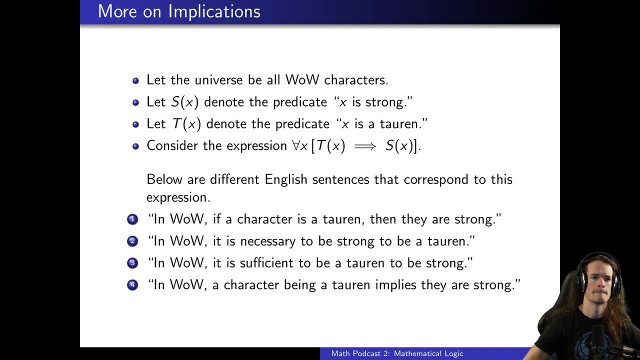 that's, that's correct. good comment from chat. um, good way to rephrase it. um, so, yeah, so we have that. so all these four statements are saying the same exact thing as the implication that it's necessary to be strong to be a tauren, that it's sufficient to be a tauren to be a strong. 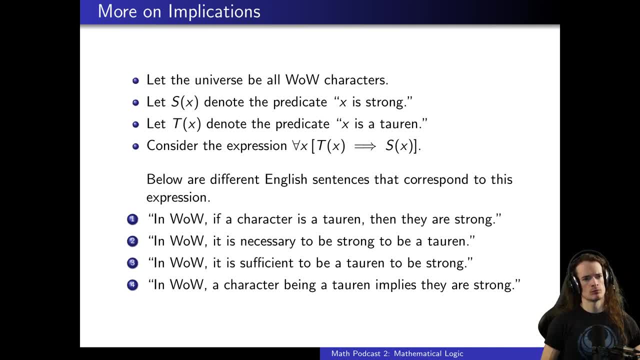 or in other words, um. the fourth one is in wow, a character being a tauren implies they are strong. so this is another way of saying if, then using the implies word. so these are all equivalent ways of saying the same thing. so this is another way of saying if, then using the implies word. 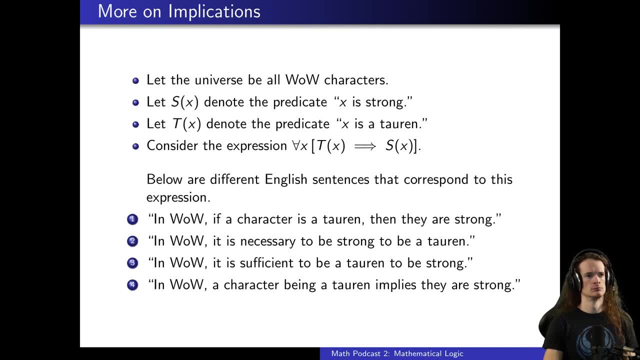 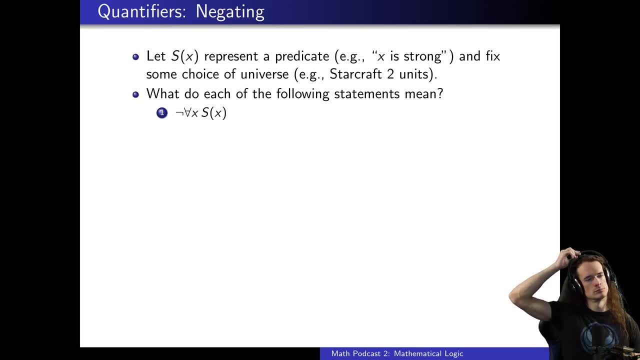 the same thing using different english letters. sentences: all right, the last thing we have about quantifiers negating. so let's think about this. so we'll let s of x represent x is strong and we'll think about some universe like, let's say, starcraft 2.. so what does the statement not? 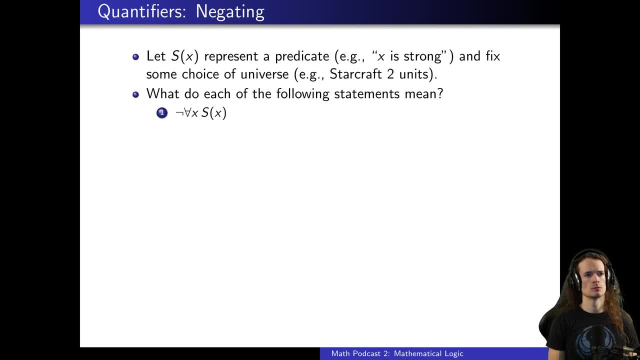 and then we have the upside down a and then x and then s of x. what is that statement? and then we have the upside down a and then x and then s of x. what is that statement? so if chad wants to answer anyone's answer, go for it. here's, here's, a chance for you to 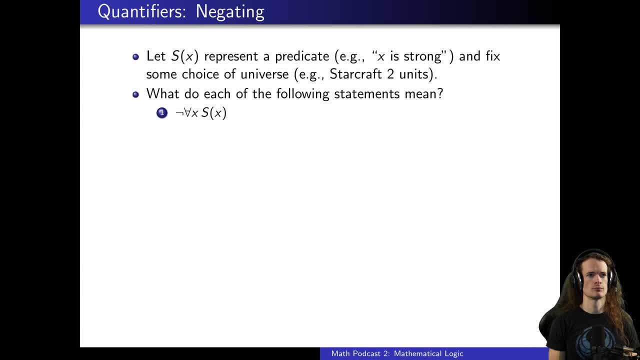 try to understand what the symbols were saying. try to remember, also integrate this negation: all starcraft units are bad. so let's see. so this is so saying, um, we could say it is not true, it is not true that all starcraft units are strong. well, the not being next to the all is kind of tricky, so let's so. so maybe, maybe it would. 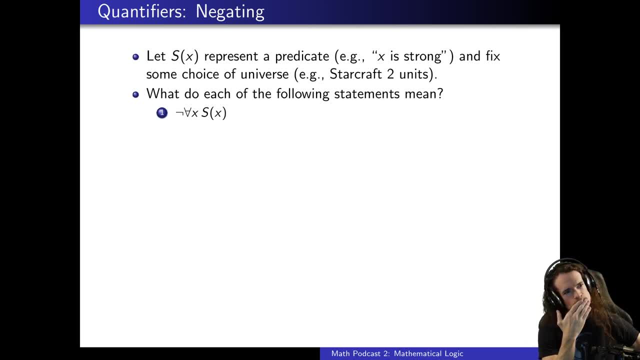 have been clear if i had parentheses. i intend to not to apply to the whole statement, so you? so you have to imagine the statement being for all x s of x. it's the whole statement and then i just put a not on that statement. it is not the case that all starcraft units are strong, so it's not true that all starcraft units are strong. 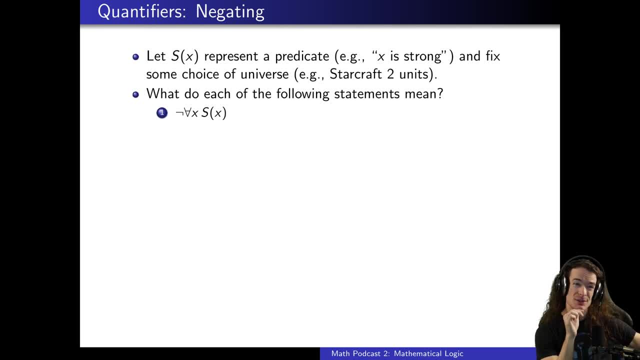 all starcraft units are strong. there you go, which doesn't necessarily mean they're all bad. it just means that there's at least one bad unit in there. oh you're, you're jumping ahead, sir. you are a slick logician. let's, let's see. so that's, we have this. it is not true that every se2 unit is strong. 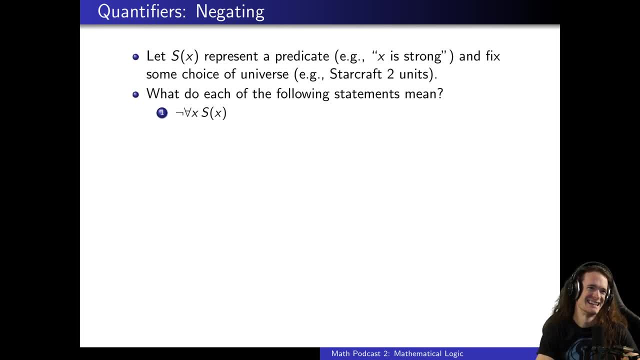 and i think that's exactly what they are: just weaving in some balance wine here, folks. yes, okay, i shouldn't say this because now the stream is going to hate me, but i am a terran. i apologize. it's okay, we probably have a terran viewers here. 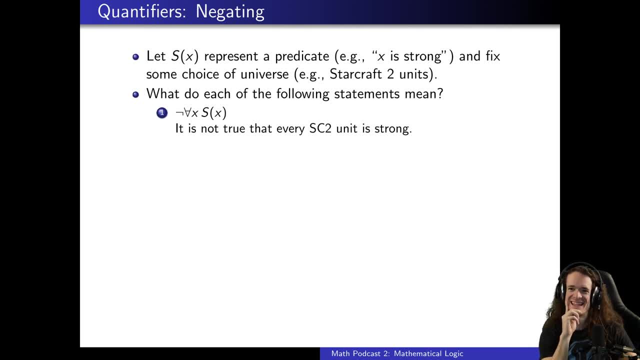 you're welcome, i'm sorry. um, so what about this one number two? we have the negation symbol, then the backward z, x and then s of x. what are we thinking? someone in chat said: at least you're not protos. yeah, agreed, sorry. no, all due respect to protos. 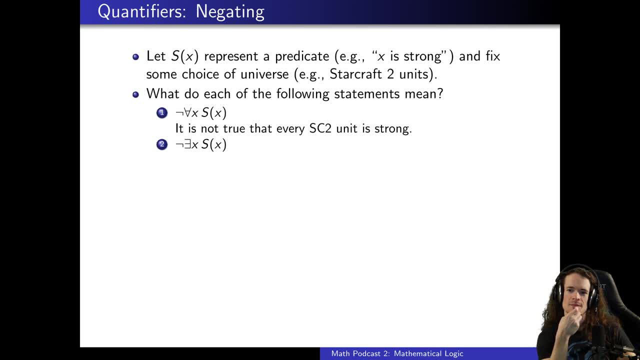 yes, they should. they deserve it. i'm trying to say that with a straight face. so let's see the not symbol, the backward z, x, s of x. what does this say? it is not the case that there exists a strong starcraft unit, correct? or in other words, there does not exist a strong unit. 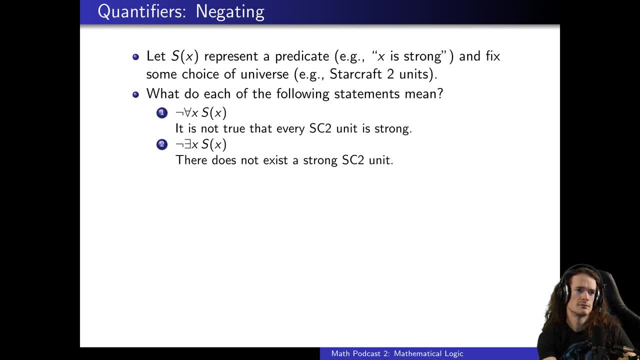 which you could also say all starcraft units. starcraft units are bad, whoa, whoa. yes, we're getting there. let's do number three. we're gonna have all combinations. number three: we have the upside down a x, the negation symbol s of x. so now the negation symbol is only applying to s of x and it's inside of the for all. 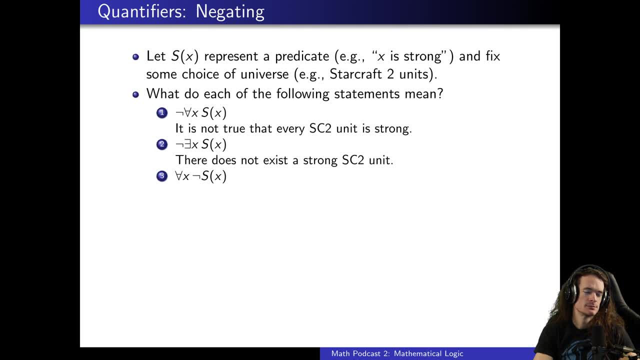 so this is the for all x negation symbol s of x. what is that? so this one's going to be for all starcraft units? they're not strong. so so for like you can say, for all starcraft units, x, x is not strong. 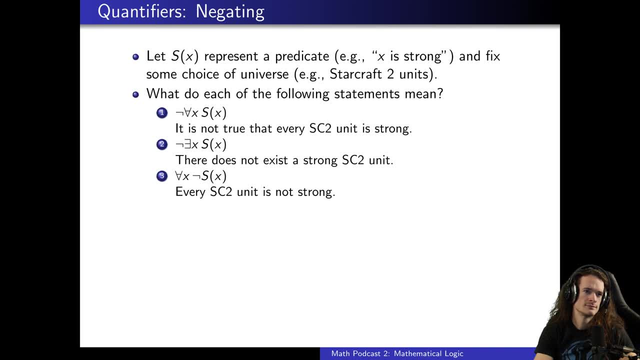 you can say every starcraft unit is not strong. this is an ironic way of doing this. so, just like blanket everywhere, she mac where. and now we have the final one, number four. now the backword x, x, s of x, x, x, the negation symbol, s of x. 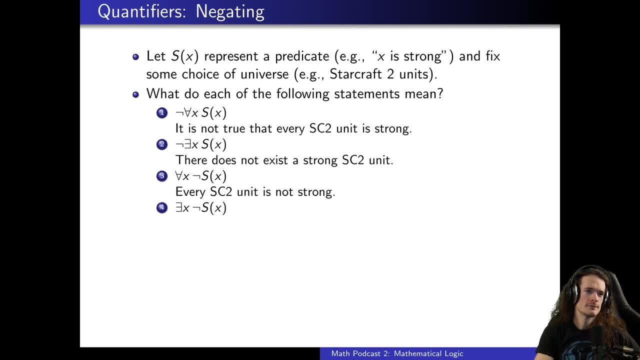 symbol s of x, and this one is: there is a starcraft 2 unit that is not strong, and earlier you said the ultra. there exists at least one bad unit. at least one bad unit. okay. so now the final question for this page: are any of the previous equivalent meaning for any universe? starcraft 2, wow, whatever. 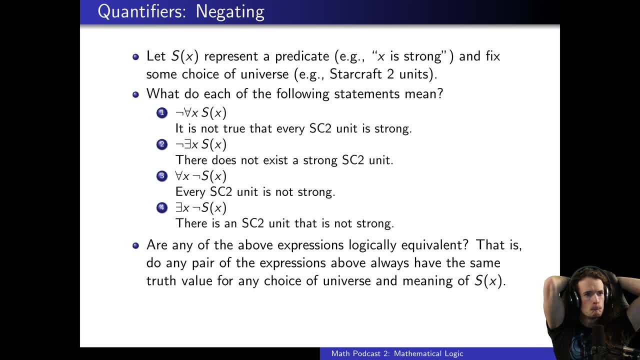 and for any meaning of the predicate s? are there any statements here that are always the same meaning? and you basically spoiled this with your brilliant comments. oh man, we should have practiced darts. fader is luke's dad. well, i wasn't metagaming, i didn't read ahead this uh slide. well, yeah you. 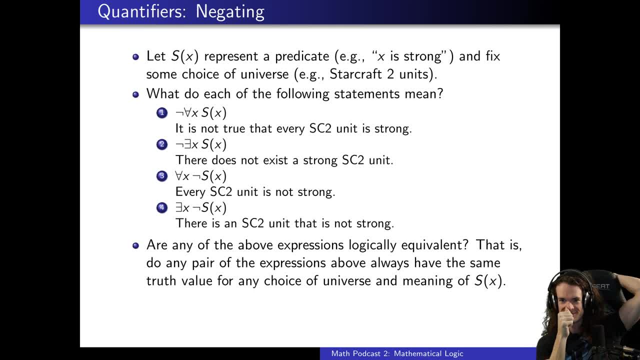 just intuited it. yeah, well done, good job. no, i'm not upset at all. you, you really. uh, you, you foreshadowed it was really good and people are answering there. i think it seems like people are agreeing with your foreshadowing. they're trusting you, so they're saying one and 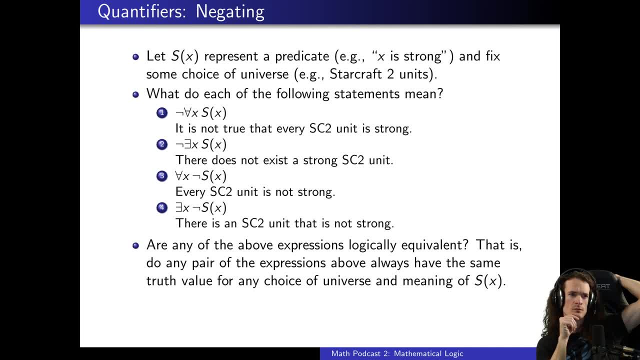 four and two and three. so let's see. so it is not true that every starcraft 2 unit is strong. so how is that the case? how is it the case that it is not true that every starcraft 2 unit is strong? then there must be one that isn't strong. so one and four should be the same. 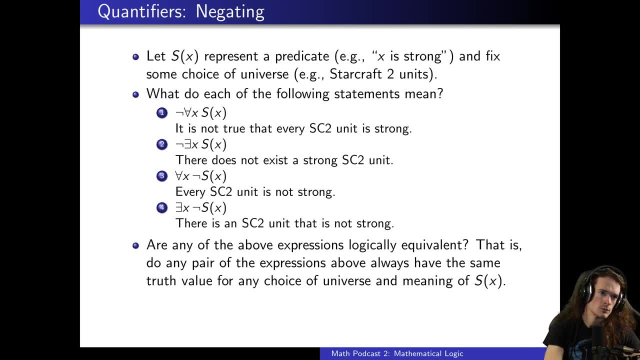 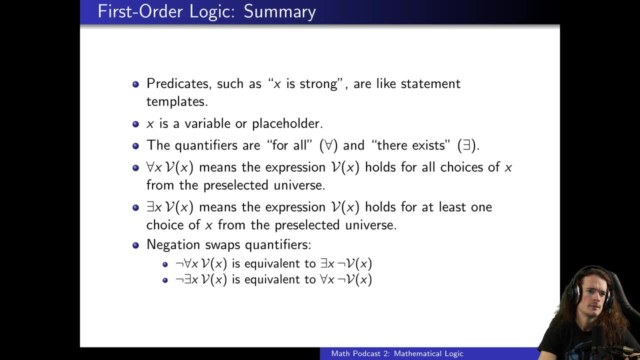 two and three. saying that all starcraft 2 units are not strong, they're all weak, is the same thing as saying there does not exist a single strong one. so one and four and two and three are the same, and hopefully i have that written and i do. yep, go, slides, all right all. 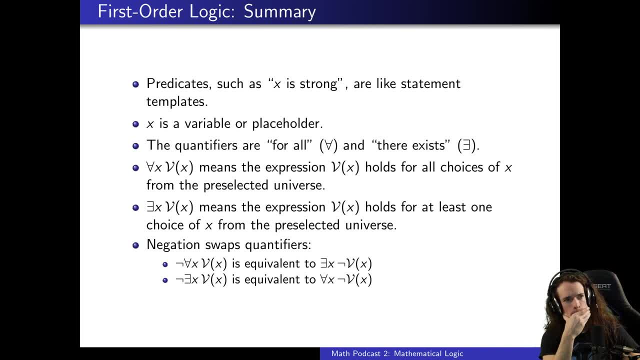 right. so now we can summarize: we've learned first order logic. we are, we are so good now. so we have predicates such as x is strong, or like statement templates where x is a variable or placeholder, and we have quantifiers where we can say: for all which we use a upside. 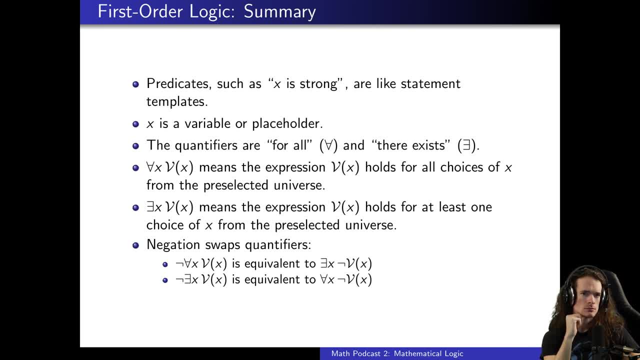 down a as a symbol and there exists where we use a backwards e and then we have the meanings of for all. once we have for all x, v of x. so i use this calligraphic v here looks fancy to mean that the expression v of x holds for all choices of x in the universe. 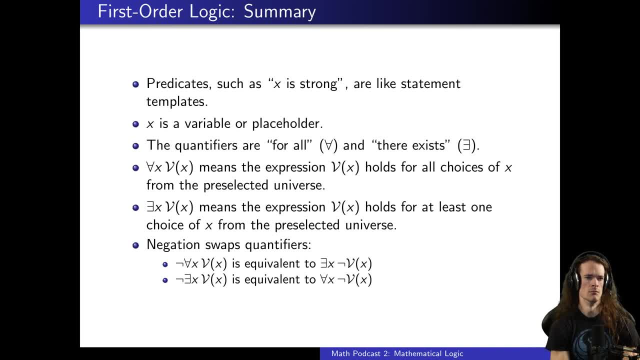 that you've pre-selected. so maybe it's the starcraft 2 universe or the wow universe, and then you have the backwards e. x exists x. there is at least one x, such that v of x means that this expression v of x, when you plug in for x, has to hold for at least one thing in your universe, like at least one. 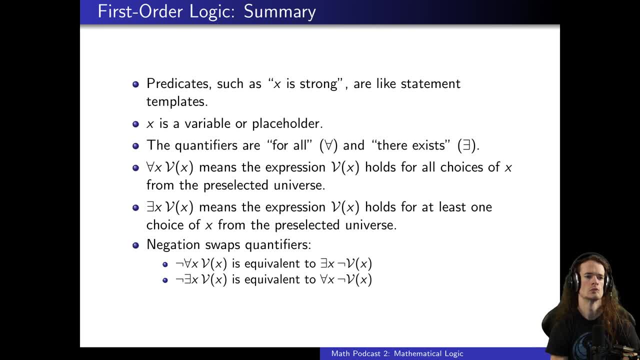 starcraft 2 unit, or at least one wow character, and we learned that negation- if we just want to be symbolic robots- swaps quantifiers. so you take the negation to the for all, it becomes an exists and it just moves right in. so when you take the negation, you just move it right. 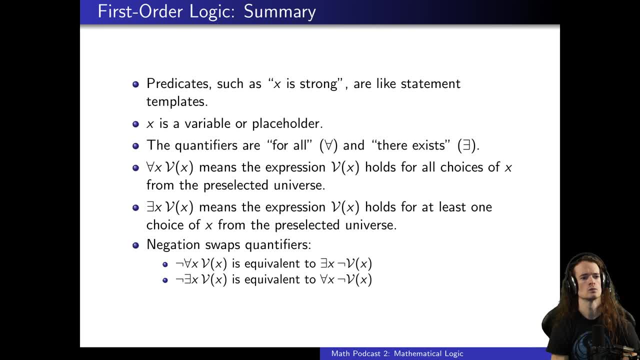 over the for all, it just becomes an exist and goes inside and you take the negation, you move it over the exists, it just becomes a for all. so saying it is not true that something holds for everything turns into existence of something. so this comes up in math a bunch. 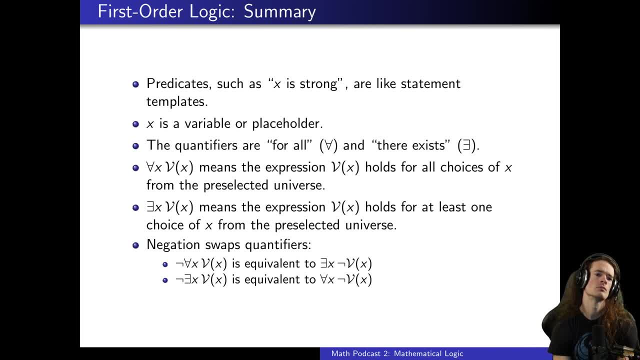 when you're trying to disprove something is true for everyone, or for all numbers, or for all things, you just have to establish one counter example, you just have to prove a there exists. when you're trying to negate a for all, so someone says no, no, no, no, all units are strong. you just have to establish one unit isn't strong an. 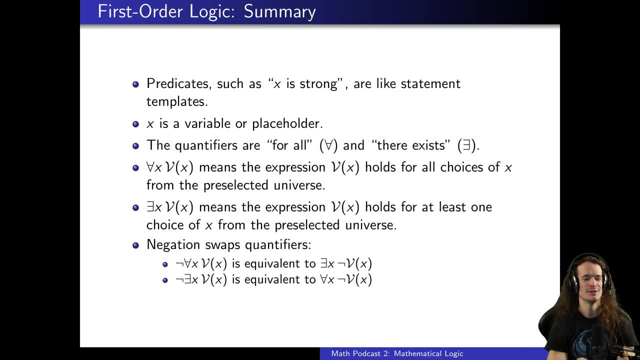 ultra. name me one bad unit. done, they're all strong. name me one bad one. you cannot disprove the fact that they're all strong units and you say, ah, have you looked at the ultra lately got them not doing too good, and if you want to prove that something is not that there. 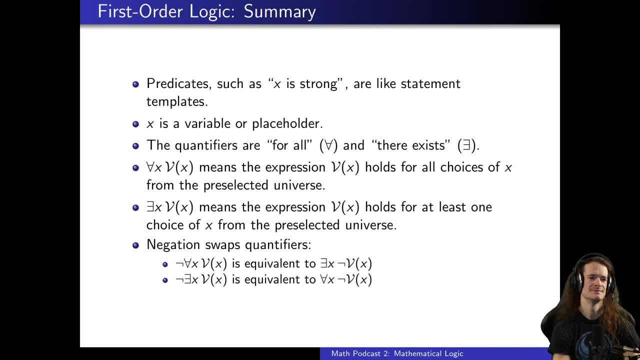 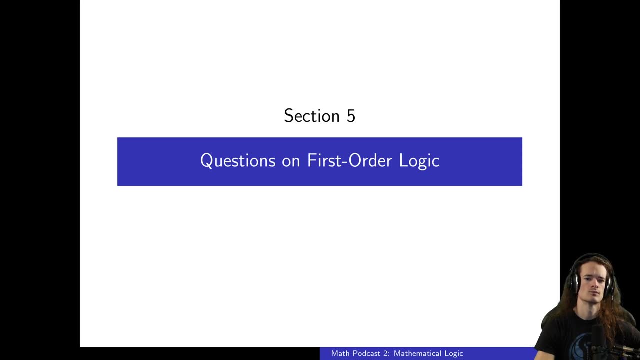 does not exist something where it's true, then you have to prove all of them are false. a little bit of a harder thing to do than to establish one counter example. all right, so i think we're ready for some questions on first order logic, and then i have some review puzzles, so we'll see okay. 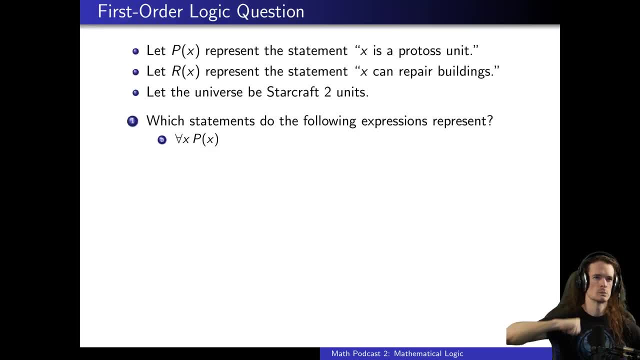 so let's let p of x represent the statement x is a protos unit. the protos come into play now and we'll let r represent the statement that x- sorry, that r of x, so of x- is x is a protos unit and r of x represents x can repair buildings. let the universe be. 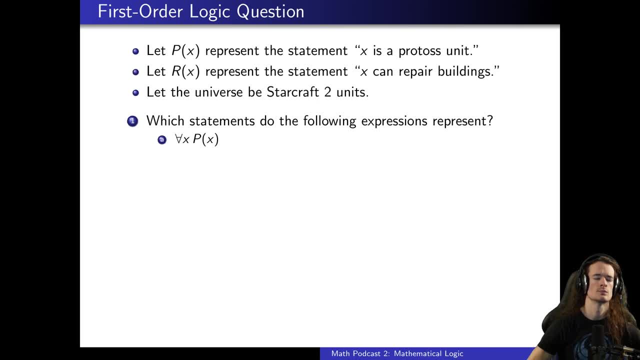 starcraft 2 units. which statements do the following expressions represent? so? so i have this upside down: a x, p of x, so we'll do this one quickly. what is that saying? that says all starcraft 2 units are protos. not true, but that's what it says. 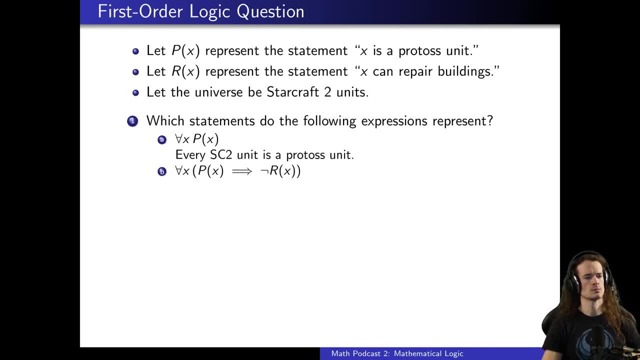 all right, let's do b got a little trickier. the upside down a of x and p of x implies not r of x. so what does this say of all starcraft units? if it's a protoss unit, then it cannot repair shed. absolutely correct, well done. it says protos units cannot repair buildings. 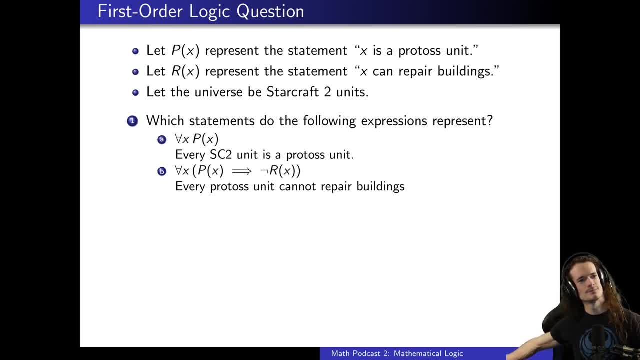 they just destroy them with their silly air units. c, the upside down, a of x. and then the statement we're taking: the for all of is not r of x implies p of x. what does this say for all starcraft units? if it can't repair stuff, it's not a protoss unit. 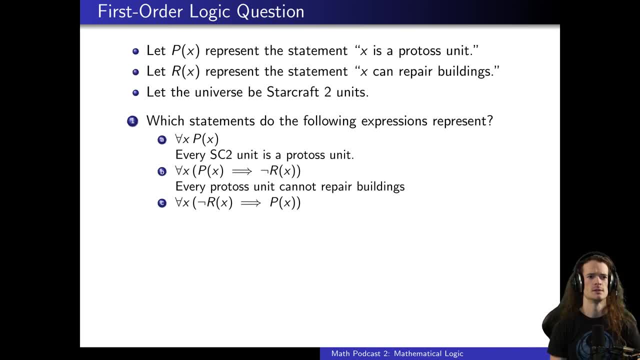 then it's a protoss unit. is this one true? no, not necessarily. could be a zerg unit. sure, zerg units are not too good at repairing. they just seem to destroy my barracks- good at destroying buildings. so that one's not true either. let's see d. so we have exists x, p of x and not r of x. 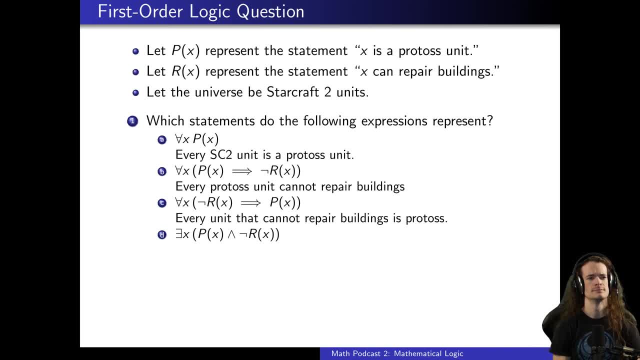 so this says that there is a protos unit that cannot repair buildings right there, or there is a unit that is protoss and it does not repair buildings, colossus, and that, yeah, colossus does not repair units, buildings or units it. yeah, it shreds infantry is what it does. it reverse, repairs the enemy base. yeah, it makes you cry. it's a crying cry. 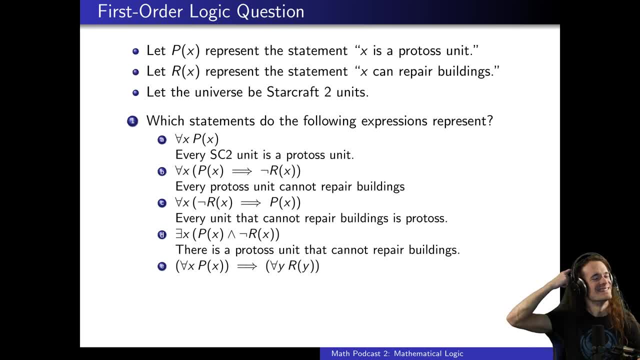 makes you cry. it's a crying cry, it's a crying machine. oh no, um. okay, now let's look at this one. this is an interesting one. it kind of flips, makes us think a little. so we have for all of x, p of x in parentheses implies for all of y, r of i. what does this say? 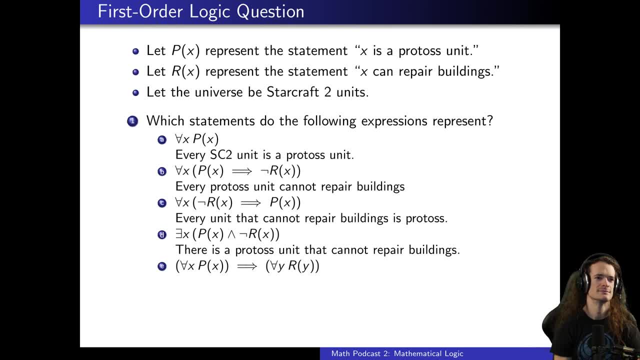 this is a little, a little bit trickier, but i think we can get it. what does this say? any ideas from chat? um, it's like: where did this y come from? cobra thinks i'm biased. you're noticing my terran coming out? yeah, a little bit. 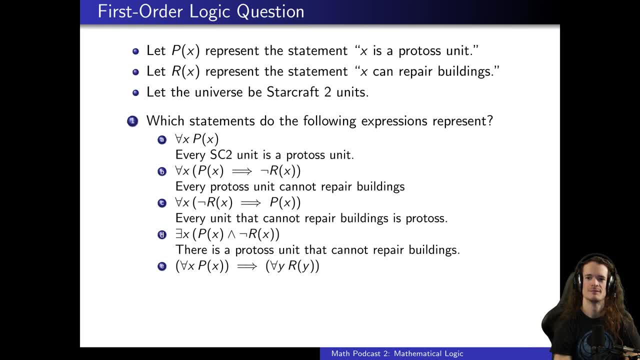 so what this says is, oh, oh, perfect. a great answer from chat. if every starcraft 2 unit is protos, then every starcraft 2 unit can repair buildings. exactly, and this statement, this statement is true, weirdly why? because the premise is false. exactly, every unit is not protos. well done, excellent. 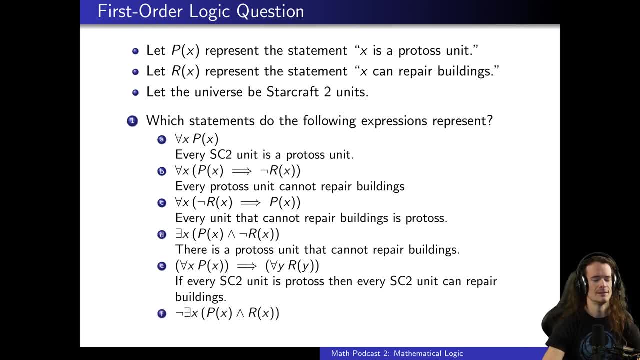 excellent. last one, the negation of there exists x, such that p of x and r of x and that will be. there does not exist protos, a unit that is protos and repairs buildings. there is or there is no protos unit that can repair buildings. true, and that's true. 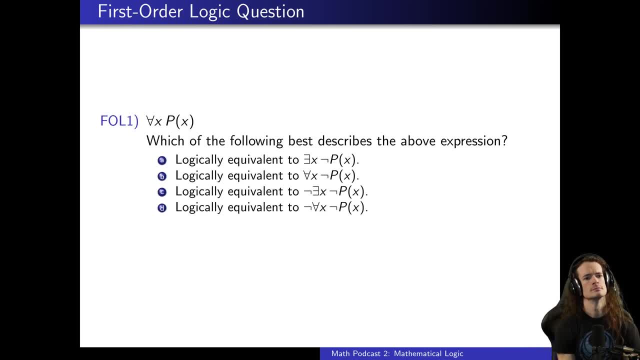 all right, let's we. only i think we're going to make a small point now. i think we only have three of them, so we'll do some three first order logic questions and then we'll move on to chess boards, and i think we'll be that'll be it. so let's talk about these first. 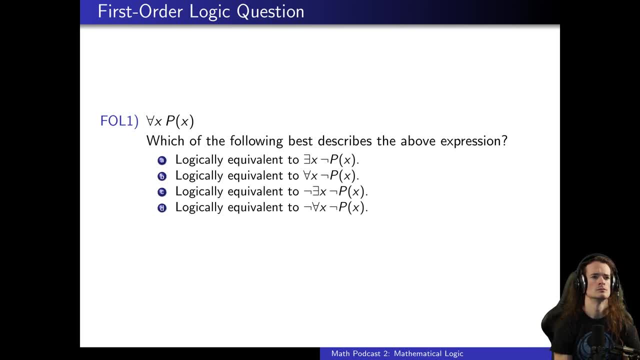 order logic questions. so number one: so we have the statement for all x, p of x. which of the following best describes this? is it equivalent to: there exists x, not p of x. for all x, not p of x. it is not true that there exists x, not p of x and it is not true that for all x, not p of x. which of these? 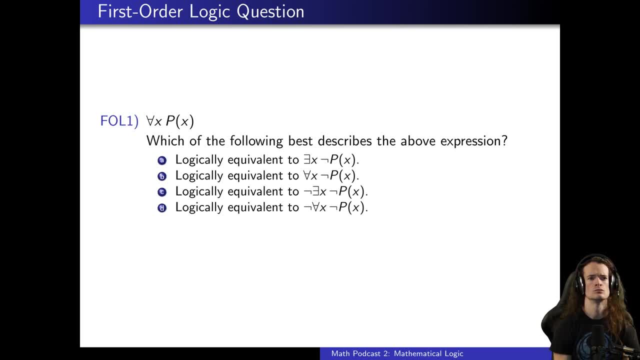 is the same as for all x, p of x a, b, c or d, and that should be true, independent of the universe. and what p means? i wasn't having a weird day, but then i had to think independent of the universe and i've been confused ever since. things got weird. 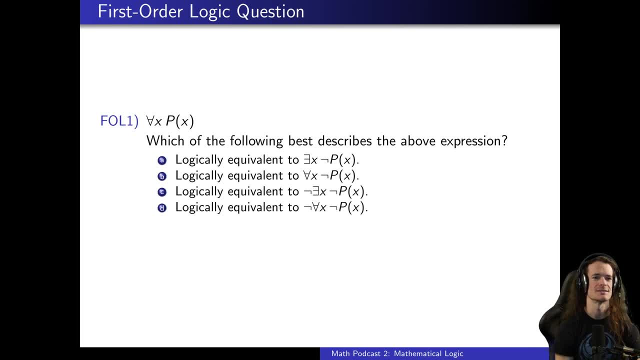 up, looks like chad is in consensus. yeah, so you said. you said later you'll be doing a starcraft 2 stream with someone and you'll be like: wait a second, let me think about this strategy, independent of the universe. let me just step outside the universe for one minute. 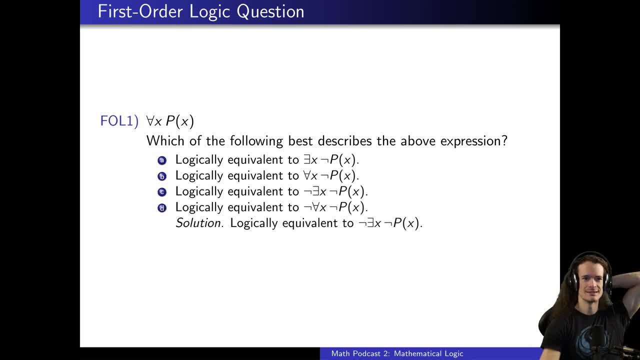 chad has a consensus of c. so if we just act like a symbolic robot and we look at c and we take the knot and we move it across the exists, it becomes a for all and then the double knot turns into p. so that is exactly correct. if we want to think about this logically, we can say what it. so maybe we think. 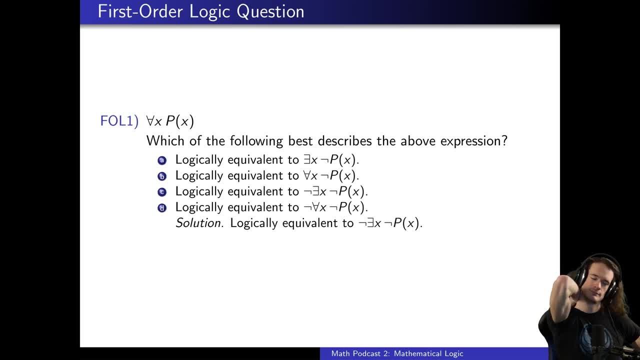 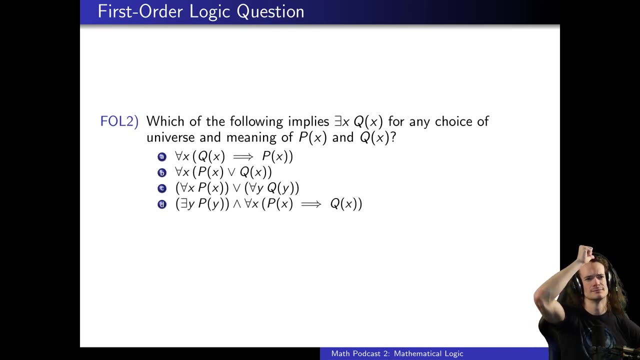 about it as, like for all x, p of x. that's the same thing as saying there does not exist an x where p of x is false. so well done, chat. there was even a big capital c, vehemently c from chat. i'm liking it. number two, which of the following implies that there is exist an x such that q of x. 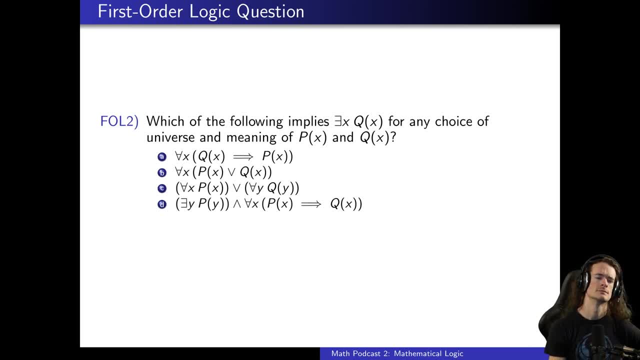 for any choice of universe and meaning of p of x and q of x. so the first choice is for all x, q of x implies p of x. the second is for all of x, p of x or q of x. the third is for all x, p of x or for all y, q of y. 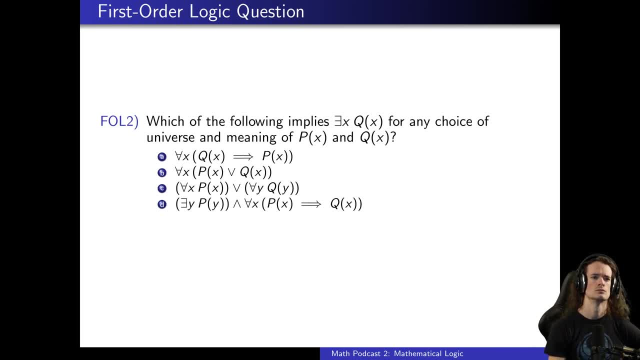 and the last choice, d, is there is a y, p of y and for all x. p of x implies q of x. which of these four choices implies there is an x, such that q of x. it says nasty, nasty. what did you do with that? we only have one one left, so i wanted to make 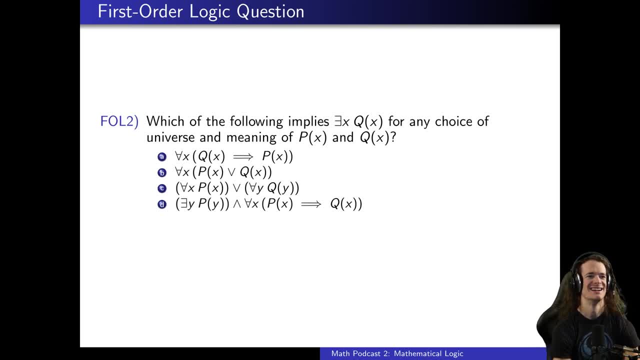 it a little. oh wow, someone jumps out two d's correct chat. well done. so let's just read d and try to parse it. so the first part says there is a y, such that p of y is true. so we have some. there is going to be some y there is maybe there is some. 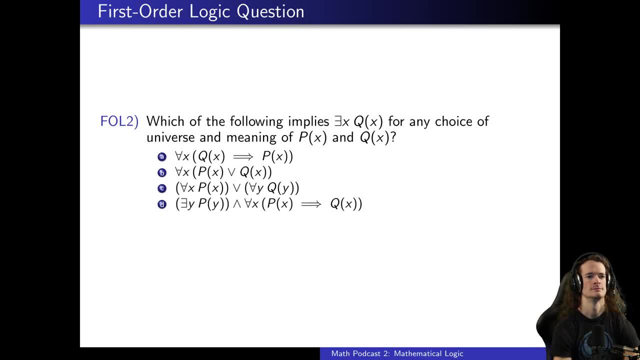 there is some tauren unit, if p is tauren and q is strong. and there is some torrent unit. and the second part of d says it's also true that if you have any p, any x that satisfies p, it has to satisfy q also. so there, if you have any, 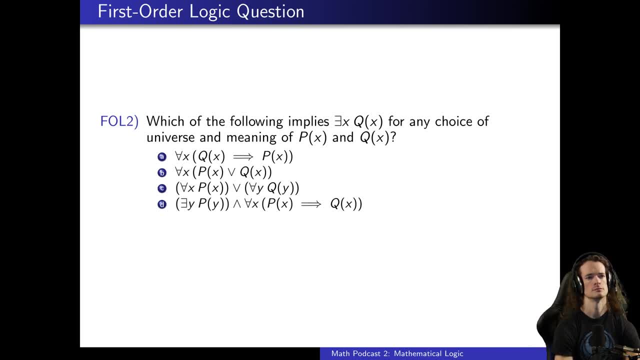 any unit that is torrent, then it's also strong. so the first part would be saying if p means torrent and q means strong, that there is a torrent, and the second part would mean all torrents are strong. this guarantees that there must be a strong unit. so maybe there exists a torrent, maybe that's brunt. 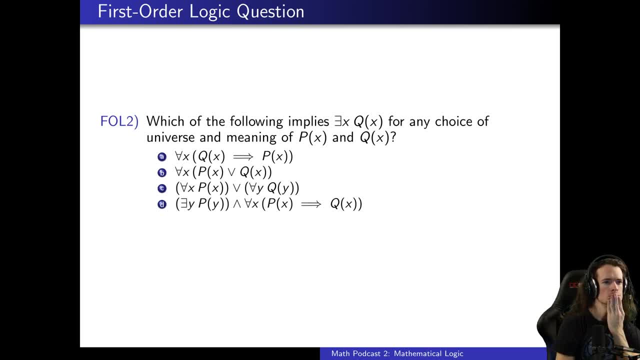 and then the second part says: well, all torrents are strong, so that must mean that brunt is strong, so d having there be something that satisfies p, and then saying that all p's are q's gives you that there must be a q and the others don't provide this. so well done, chat. we've showed how. 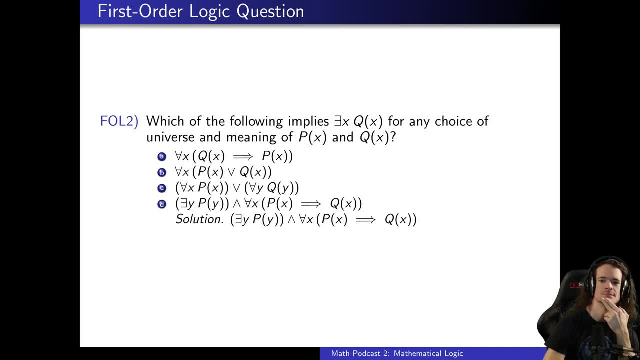 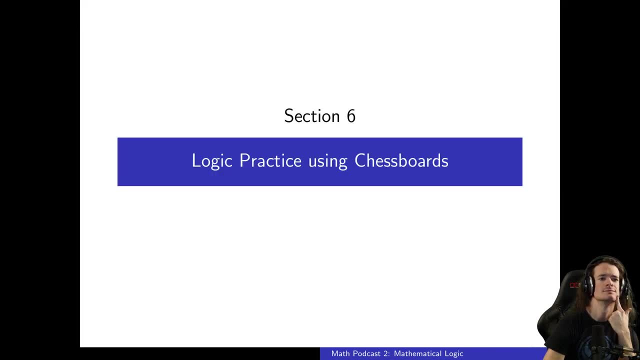 to start with there being something and then using the implication to get something else. this is logical implication. so our final, first order logic question. oh no, i think i just ended there. great, we're gonna have, we're gonna. now we're gonna practice logic using some visual cues. so 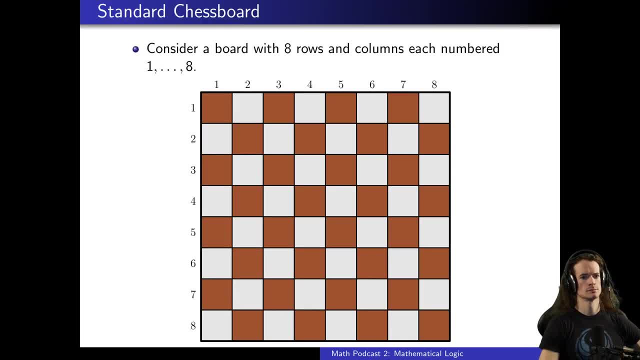 i think whenever you can introduce some visual aids to help, to help review logic and to help understand, that's good. so we're going to take a standard chessboard, eight by eight chessboard. it's going to have eight rows and eight columns and each of them i'm just going to number them. 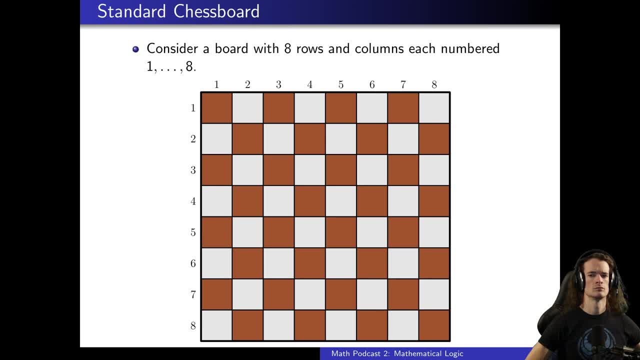 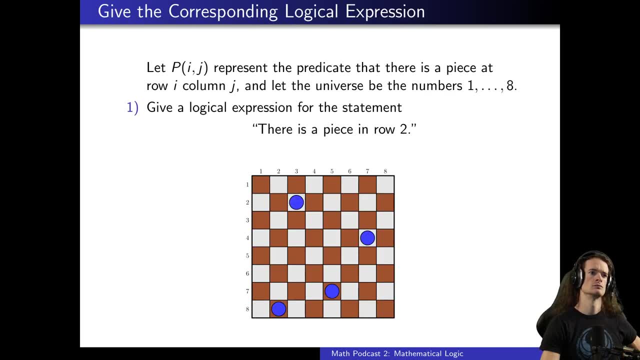 one through eight, rows one through eight and columns one through eight. i'm not going to use any chess lingo, just both numbered one through eight, and then on the next slide i'm going to define a predicate. so what p i j means is that there's a piece of the chessboard that's going to 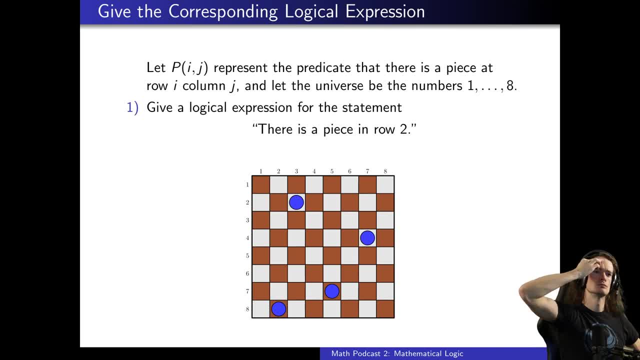 be a piece in row i, column j. so what i want to do now is just give the logical expression for the statement: there is a piece in row two. how would you write that, using the predicate and maybe other stuff? how do we use the logic, the first order logic we've learned to say there is a piece in row. 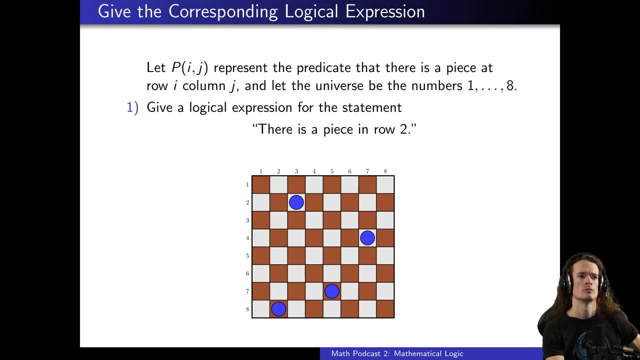 two, oh man, we've even got the backwards capital e in the chat. in the chat, that's impressive. i've even i've thought about, like maybe there should be some math emotes. someone can math on somebody with a crazy emote. so oh, and someone's doing a math emote. 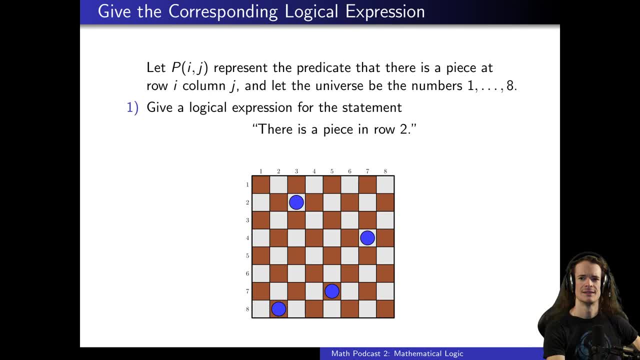 echoing. so in chat. the answer is: there is an x such that p two comma x. so let's see, the answer is: i think i use j here, so i have the solution being: there exists a j such that p two coma j. so what is that saying? so remember p i j means there's a piece in row i, column j. 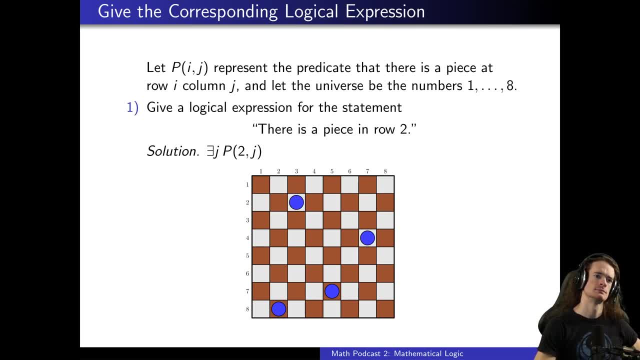 so we're saying: there exists a column such that there's a piece. there exists a column j such: there's a piece in rowez, column j, row two. column J, That's saying, there is a piece in row two. So we've used our first. 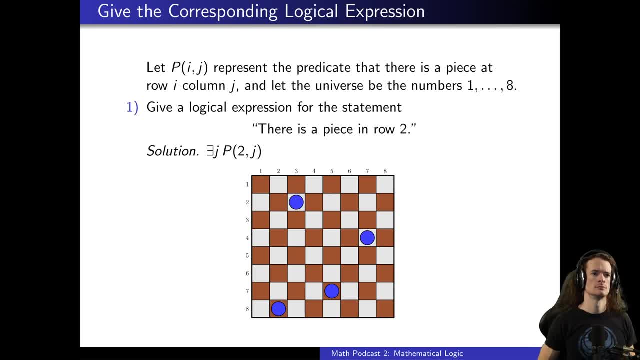 order logic to describe something about this board Very good. Another thing we could have done- which maybe the answer is not cheating, but it was a little less compact- is to just write out eight statements. We could have said P21 or P22 or P23, or eight times, And 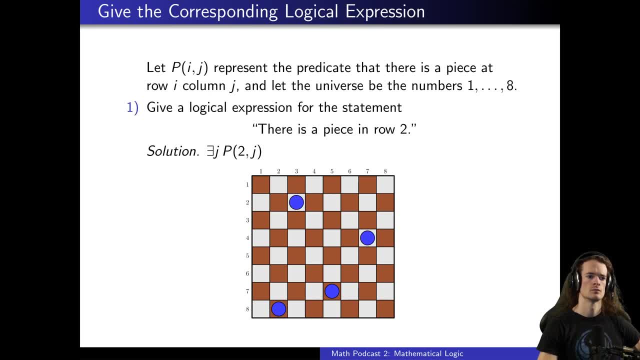 that wouldn't be the most elegant way of writing it, but that would have been true. also, And someone's asking in chat: is there a symbol for such that? So when you say so in the English, when you translate the symbols, when you write, exists the backwards, E, J and. 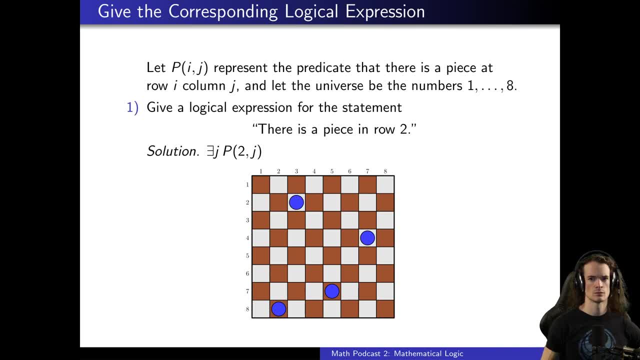 then a statement, you naturally add the word, such that in between There are sometimes symbols people use for like conclusions And sometimes, when we're not talking about this today- but if you're using like set notation, sometimes you can think of the bar and the. 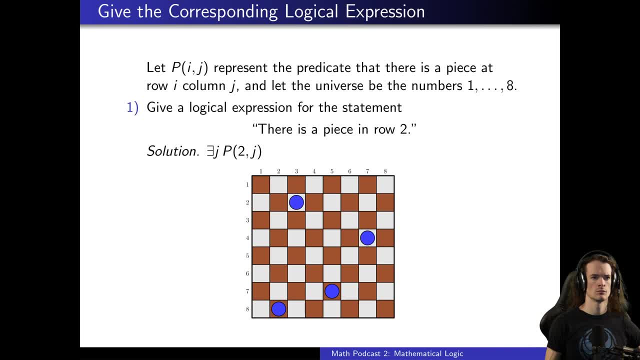 set as being such that, But you get a such that Such that for free when you use exists when you translate it into English. There exists a J, such that P2J. Let's try another one. See how chat does on this one. Number two: 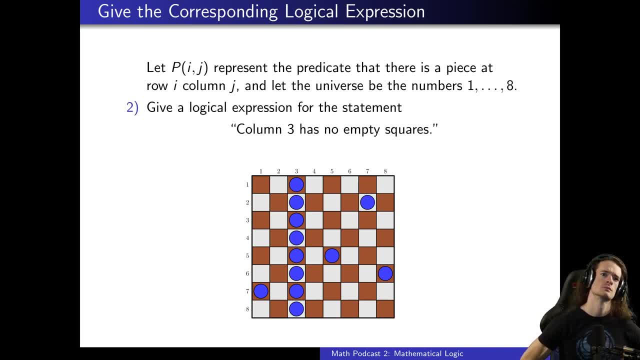 how would you come up with a logical expression for column three has no empty squares. We're going to get an upside down A. People are trying to figure out how to type that. I think people can copy off of the comment. Someone just wrote all of the symbols ever. 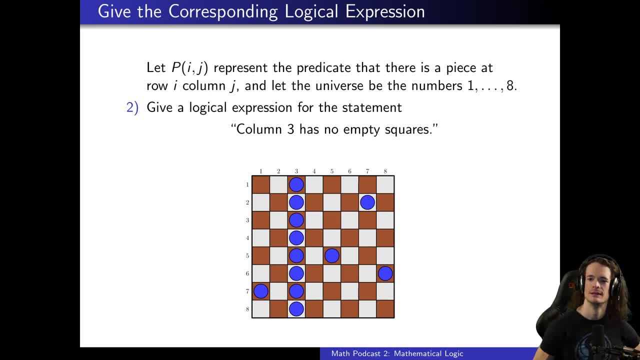 So someone's saying for all X, PX3.. So that's very good, That's one way of writing. Can we think of another way of writing it, So that one says every for all rows? there is a piece in row X, column three. Very nice. 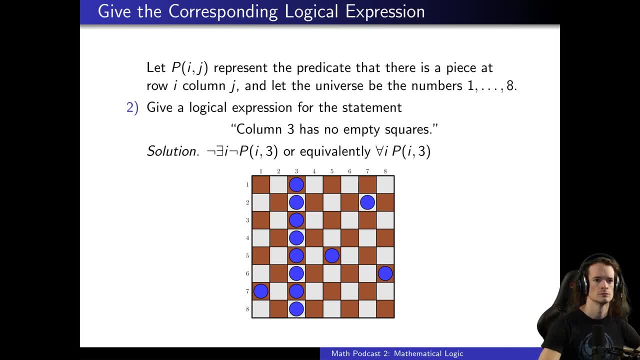 So another way we could say it is using negation, that there doesn't exist a position. where there's no position, There's no piece in it. So there does not exist an I such that, not PI three, which means there does not exist a row where there's no piece. in row I, column three or equivalently. 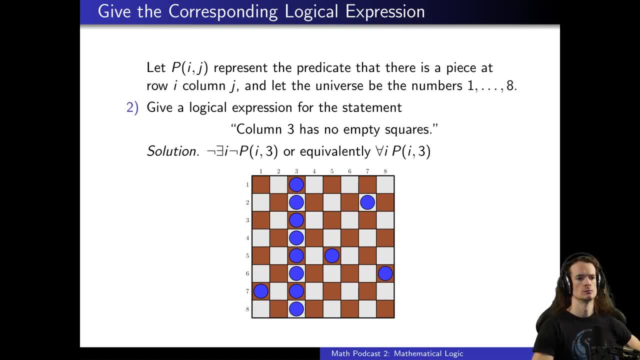 every single square in column three, in all rows is: is has a piece in it. So we say for all rows, for all I PI three means for all rows there's a piece. and row I, column three. Very nice, Let's try one more. 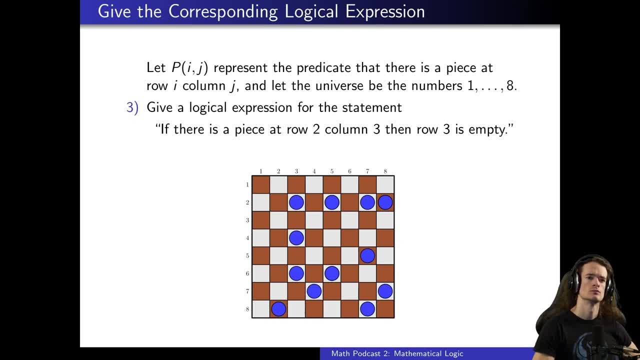 So if there is a piece at row two, column three, then row three is empty. So we first need to think about so this is an if, then statement. So we should definitely be thinking about having an implication somewhere in there. So think about that And then we want to. 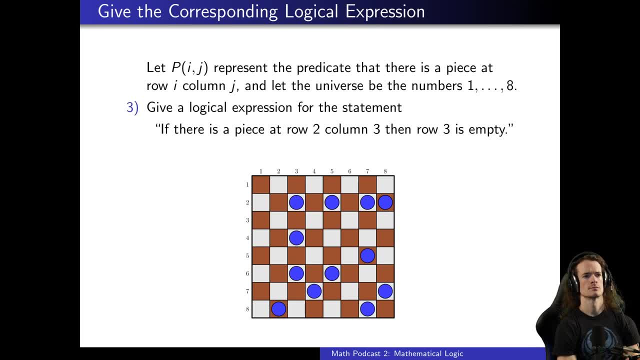 start with the condition of implication. So you want to say: how do we say there is a, there's a piece at row two, column three, And then, lastly, we want the conclusion, the, the conclusion of the. if, then statement, which is row three is empty, There are no pieces. 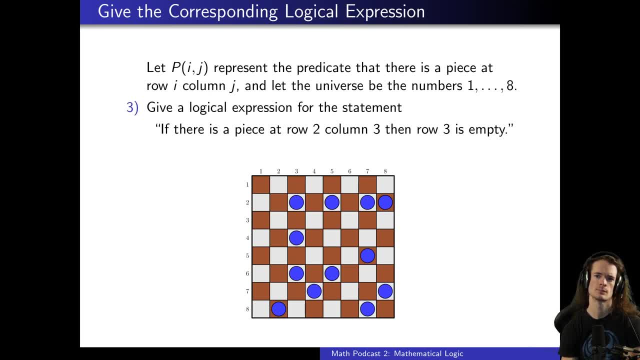 in row three. So let's see. So we can write as the solution: P, two, three, meaning there's a piece in row two, column three, And that implies that We can either Yeah, We can either say for all columns J, there's not a piece in row three, column J, or, if you like, 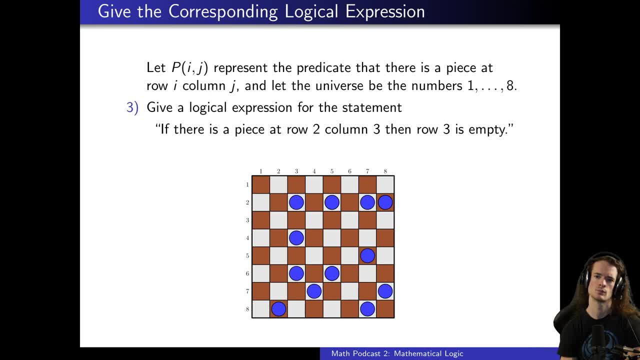 we could have also done this with the exist statement. So that's and that's the solution. So, and hopefully what I have on the slide agrees with that. I think it does Very nice slides, correct so far, Nice to see. So we could have also written this as P two three implies not there exists, P three J. 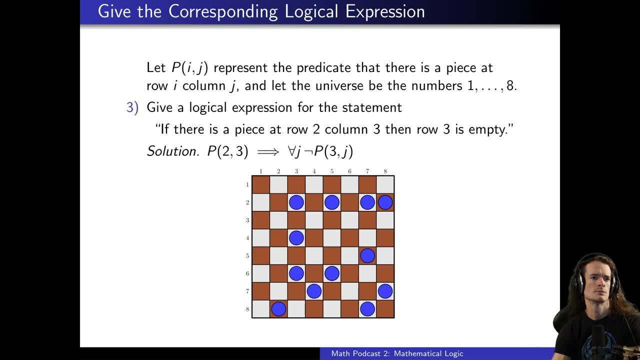 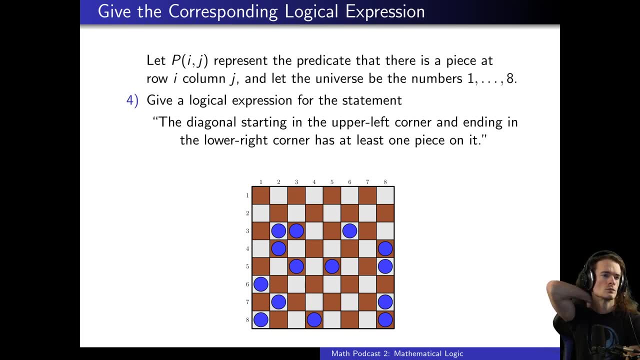 Just the equivalent negation form of the conclusion. Very nice, Chatted Great, I think I just have two more of these. The diagonal starting in the upper left corner and ending in the lower right corner has at least one piece in it. 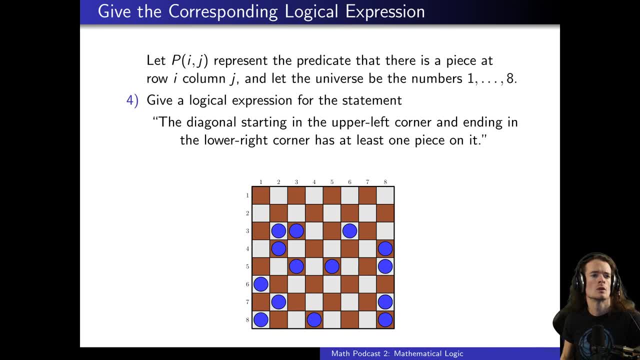 So let's think about this. You think so. Firstly, let's think: Do you think we're going to for all, or an exist for this one? Okay, So the diagonal, and we're saying it has at least one piece, So that to me sounds like there's going to be an exists. 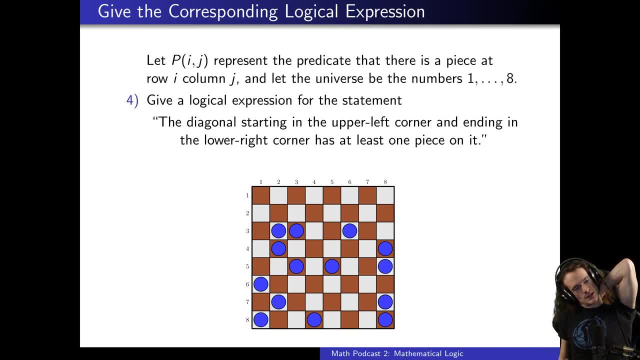 And now we need some way of this for all: I and J where I is equal to J. So, and then we're going to want to say something: So yes, we could talk about I and J where I is equal to J, That is, that is. 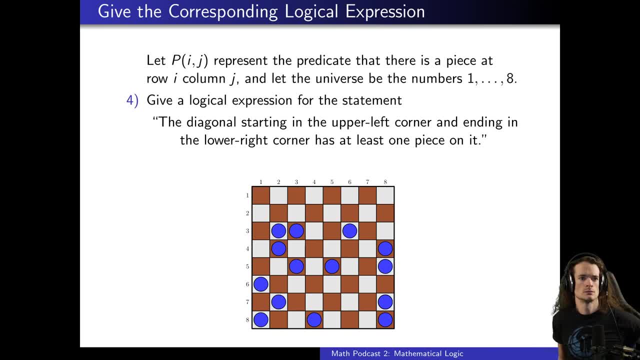 Yes, So we, we could. we could integrate something like a for all in there. I think I have this one just using an exists. There are other ways you could have written it if you want to have an I and a J and setting them equal. 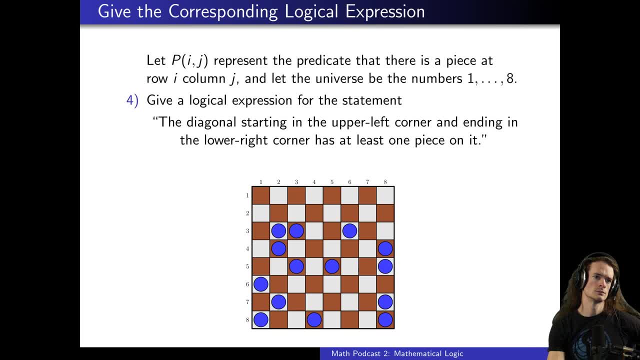 I think, for here I just use one indication like one variable, And I said there is an I such the PII. So I kind of use a little bit of an economy of of symbols. But we could have also done something where we had an I and a J and then we force them. 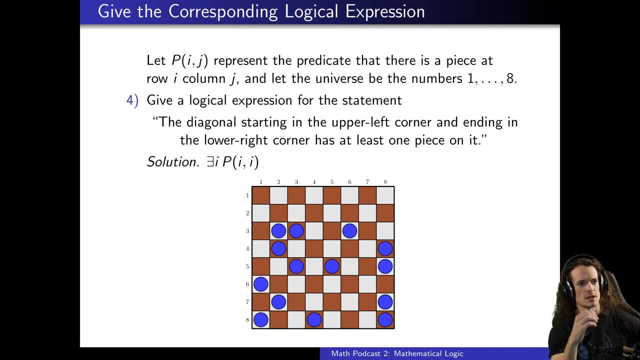 to be equal. That's an interesting aspect of finding an answer, because you have different arguments. One would be: what is the answer you can write out that takes the least amount of time, That's the fastest and the most compact, Or you could have an answer that maybe allows you to understand the problem more effectively. 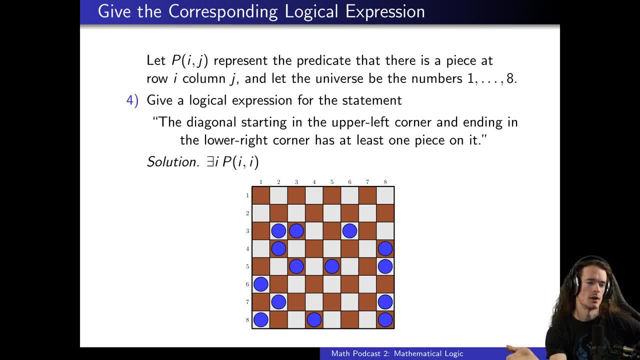 And you could play with multiple of them. to say, you get a problem on your homework. Sometimes you could take one route and see what that feels like And then you could take another route. I know I did that quite a bit in my analysis course that I took. 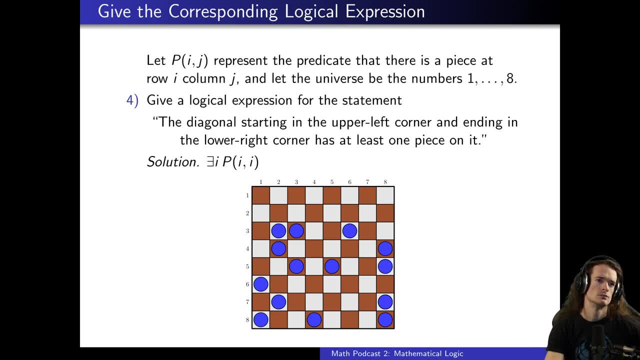 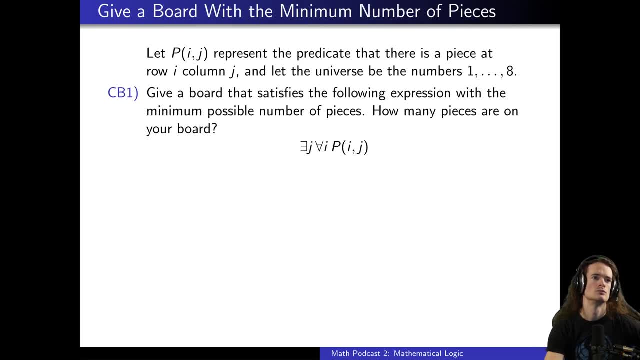 Yeah, So for this one we could say there is an I and there is a J, such that I is the same as J and PIJ, And that would be on this equals type thing, which is good. So that would be another way of writing and that would be a very nice way too. 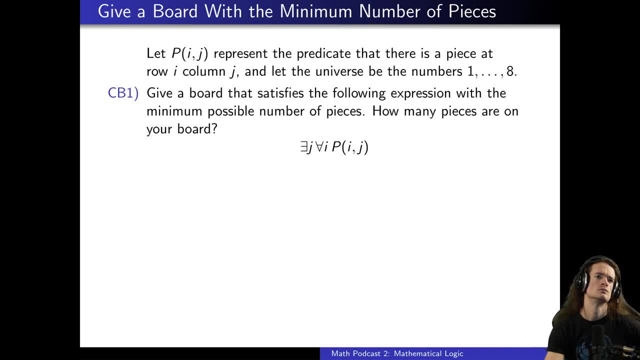 So I like it, Oh, okay. So now we're going to switch gears a little, Okay. So now I'm going to give you the statement, And what I want chat to think of is what a board would look like that would satisfy the. 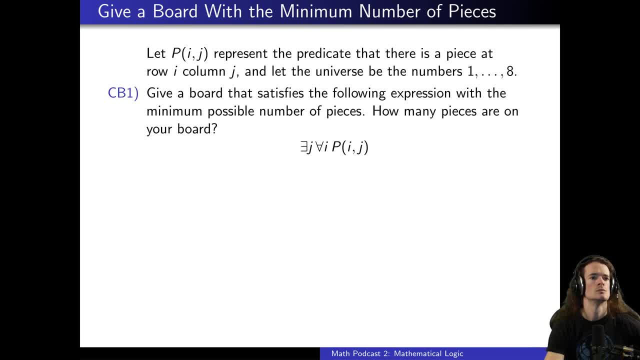 statement And try to make the number of pieces minimal And tell me how many pieces are on that board. So think of a board that satisfies this statement And then try to make it have the minimum number of pieces and tell me how many pieces are. 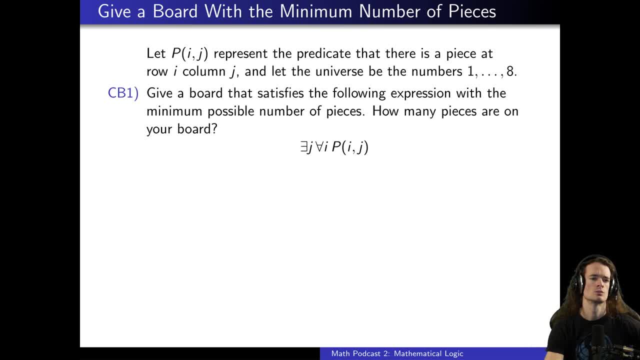 on your board. So here's the question, Here's the statement. There is a J such that for all I PIJ, And recall again that PIJ means there's a piece at row I, column J, and the universe is all numbers from 1 to 8.. 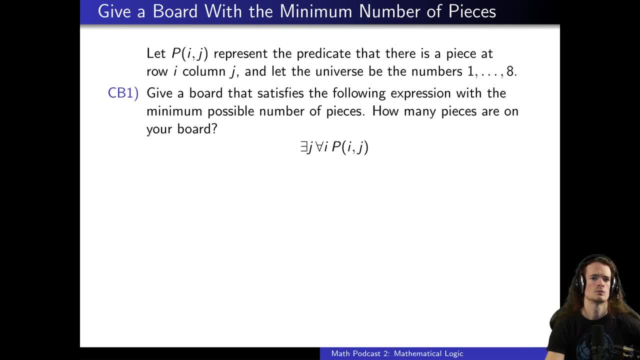 Okay, So let's try to first think before we answer the question. What does this mean in English? So exist J for all. I, PIJ, I would say for all rows. there exists a piece in each column. Okay, Now you, just you are so good at this. 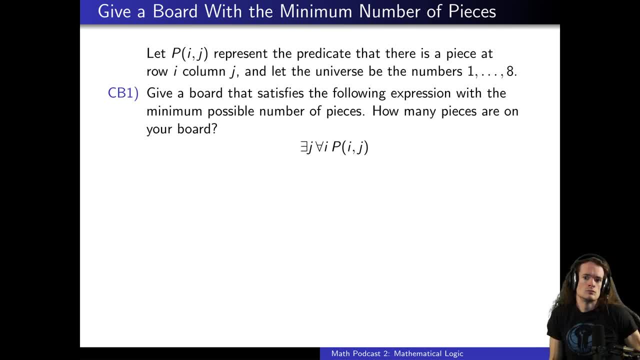 So what you highlighted was: we have to be careful. There's a difference between having the exists before the for all and the for all before the exists. And that was exact. You nailed it on the head. So now we have to be clear on this. 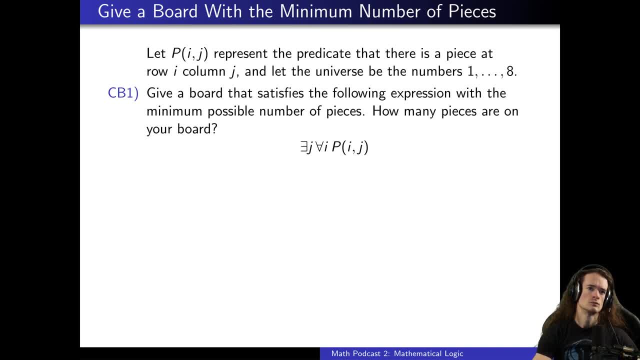 Do we mean so? are we saying there is a column such that for all rows or are we saying for all rows there is a column And those, as you'll see, have different meanings? So the order of exist and for all is crucial. So this one, I think the order I have here- seems to say there is a column. 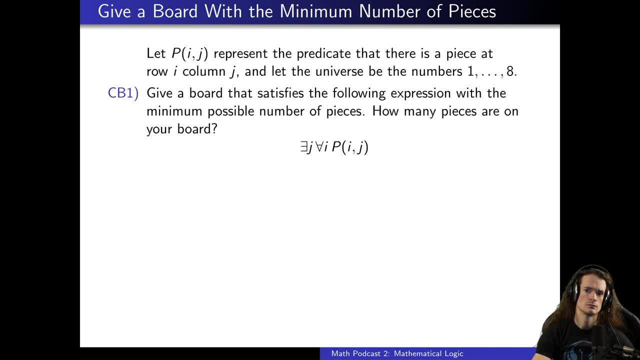 Such that for all rows PIJ, And if we flipped it around and it was for all I exist, J, that would mean for all rows there is a column. So I don't remember, but you may have stole my second question. You have this uncanny way of exactly figuring out the next thing I want to ask. 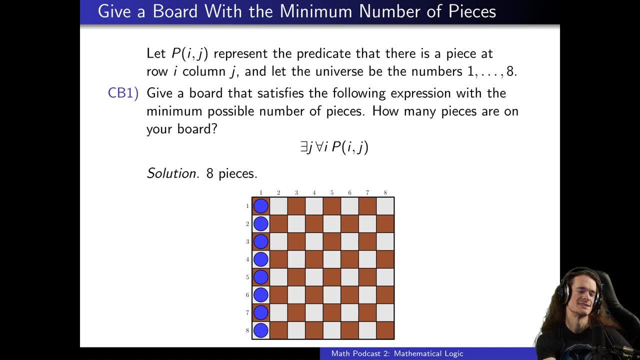 Okay, So we get the solution for this one: Eight pieces. So there is a column such that for all rows there is a piece in that, And if you want to have a minimal possible answer, you choose one column and fill it up and you get eight. 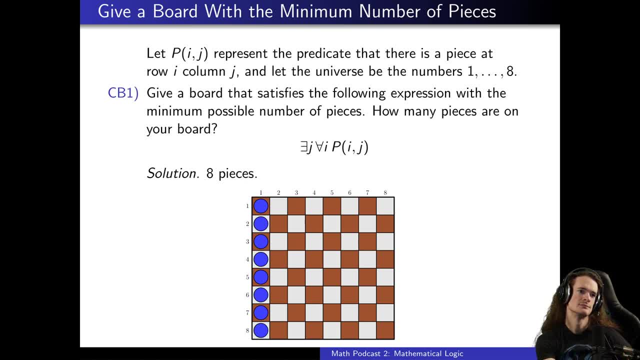 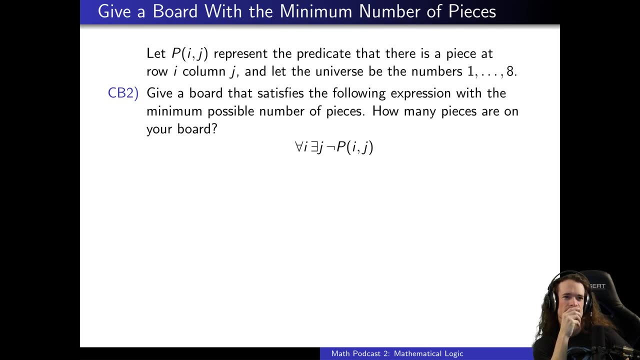 There's a full column. Very nice, Let's do number two, You see, Yeah, No, but it's amazing, You're so good at this. Yeah, Very nice. So now we have for all I. there exists J, not PIJ. 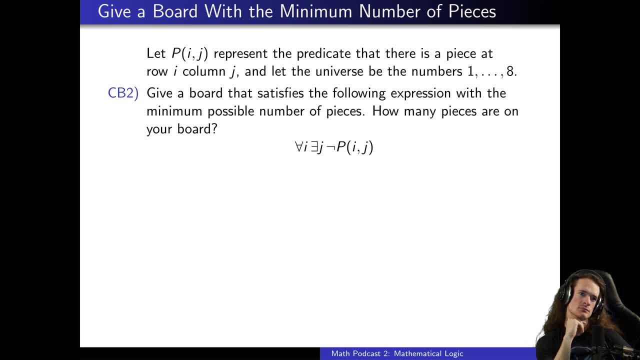 So here PIJ again represents. there is a piece, row I, column J, and the universe is one through eight. So to repeat, for all I, there exists J, not PIJ. Think of a board with a minimum number of pieces that satisfies this. and how many pieces are on your board? 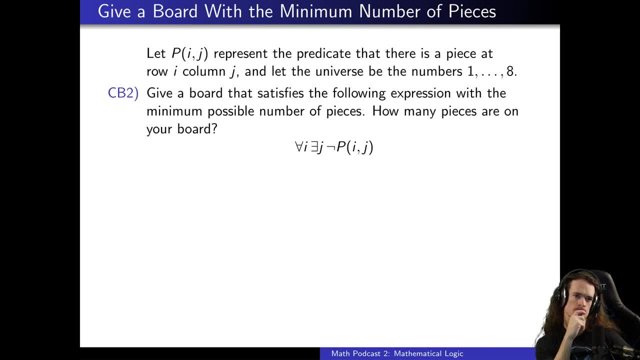 Before we do that, Let's think about what this means. in English. This is saying: let's see, So the for all comes first. So it's saying: for every row there is a column with no piece in it. So what's the least number of pieces we can get away with to make this true? 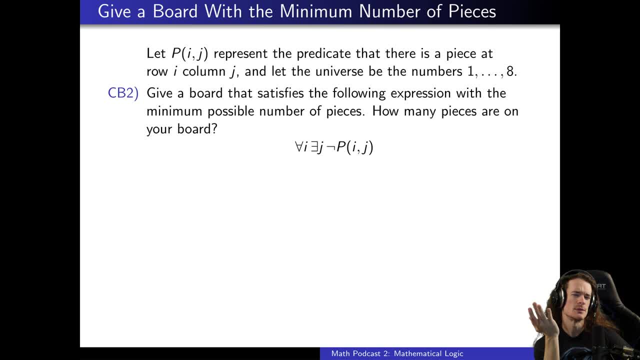 So there's lots of boards that satisfy this. What if it was an empty board? An empty board satisfies it, right? An empty board definitely has, in all rows, at least one column with no piece Empty is very simple. Now there's lots of other boards that satisfy this that aren't empty. 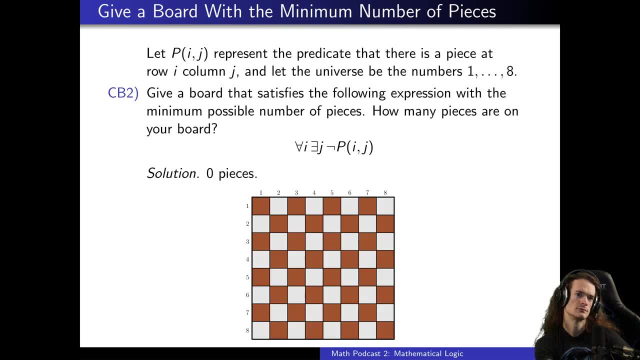 But if we wanted the minimal possible example- zero pieces, Because empty boards definitely satisfy this statement- All right, But there's such a strong cognitive bias to want to put a piece on the board. Pieces on boards are nice, Yeah. What is this board doing? 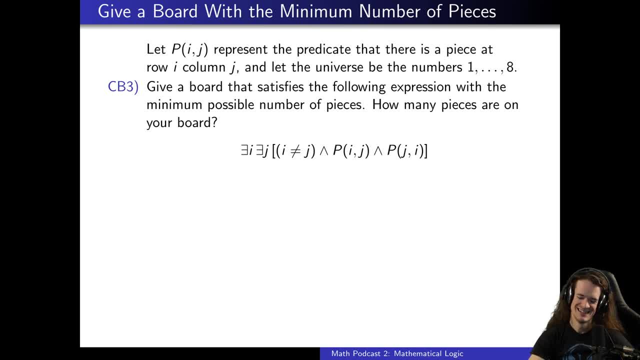 It's like the board yearns for some kind of piece, some use. Okay, Let's see Now this one Same setup: There is an i and there is a j, such that i is not the same as j, i is not equal to j. 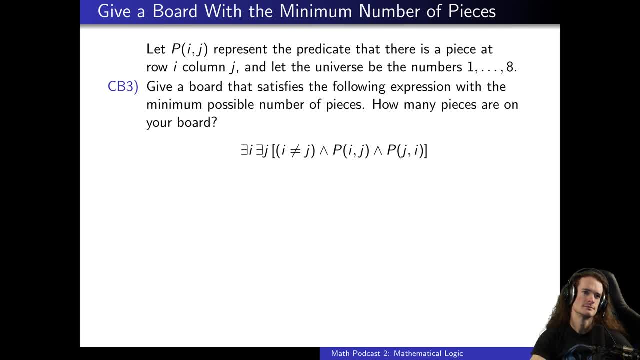 And pij and pji. So again: pij represents: there's a piece in row i, column j, pji then would mean: there's a piece in row j And pij is row i, column j. And then so again one more time. the statement is: there is an i and there is a j, such that i is not equal to j and pij and pji. 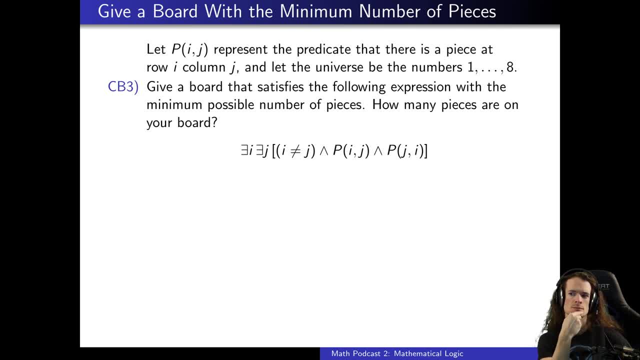 I want a board with the minimum number of possible pieces And think about what that board looks like. So what are we thinking? Okay, Chat is screaming this one. So they're saying: what if we had two pieces? Yeah, So that sounds like it will be true. 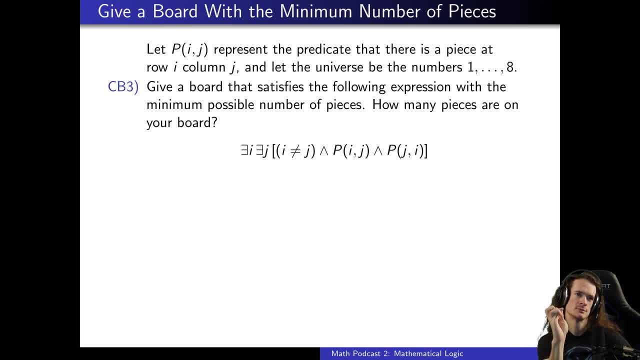 So let's think of the English statement first. This is saying there is an i and there is a j that are different. So we have two numbers between 1 and 8 that are different And there's a piece in row i, column j. 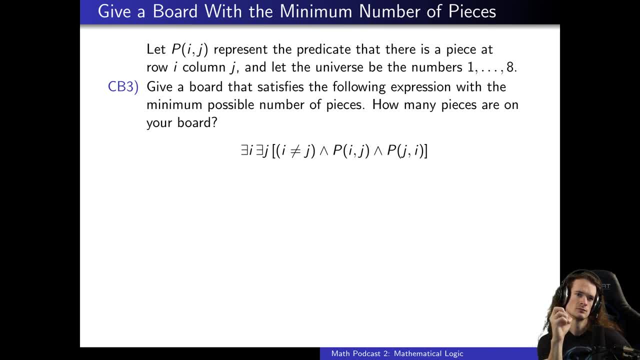 And there's a piece in row j, column i. So let's look at the picture. The solution that chat came up with is two pieces is correct And you can have, and what it means is that they're, in sort of, the pieces will be symmetric with respect to the diagonal that goes from the upper right to the lower, the upper left to the lower right. 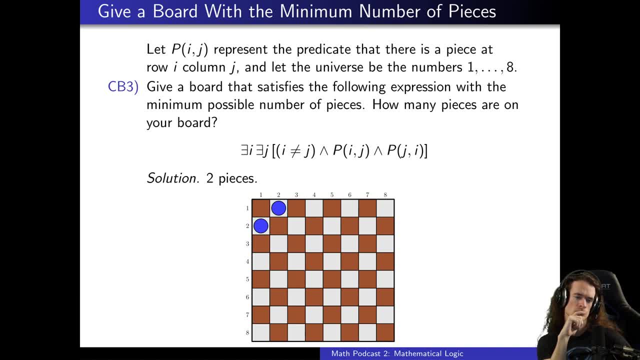 So you'll have one piece in row 2,, column 1,, let's say, and then another piece in row 1,, column 2.. So it's symmetric with respect to the diagonal And you can't And you don't need any pieces on the diagonal. 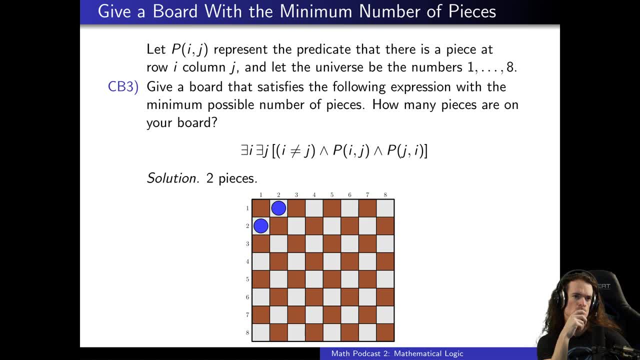 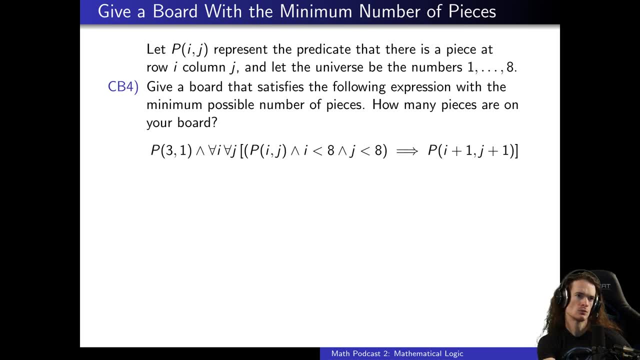 Because this is saying there is a piece that has a row different from its column. Very nice chat, Very nice. I think we have. I believe we have two left And that ends this section, But we're getting a little sneaky. 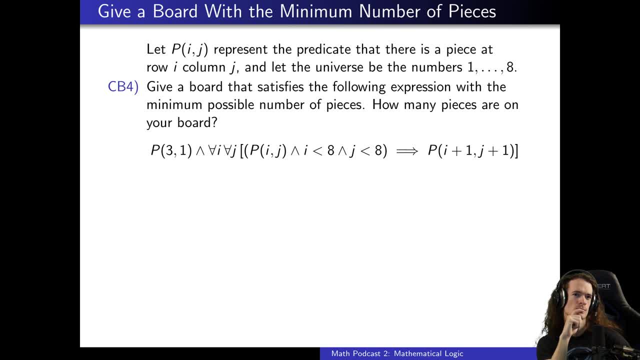 So this is going to get sneaky. So these last two are really going to make us think. We're going to have to ponder about these last two. Hopefully it will stretch- Yeah, Stretch it, Stretch our minds. So here's the statement. 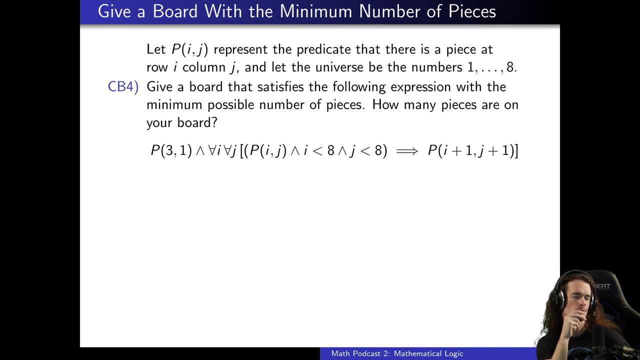 P31 and for all i and j, if pij with i less than 8 and j less than 8, then pi plus 1, j plus 1.. So let me say that one more time. We have p31 and another thing. 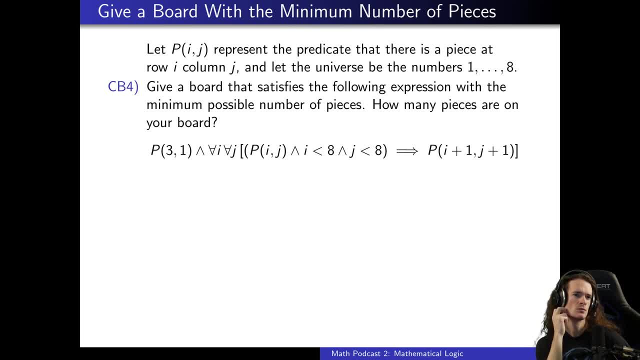 For all i and for all j. If pij and i less than 8 and j less than 8, then pi plus 1, j plus 1.. Again, pij here represents there's a piece in row i, column j, And the universe is the numbers 1 through 8.. 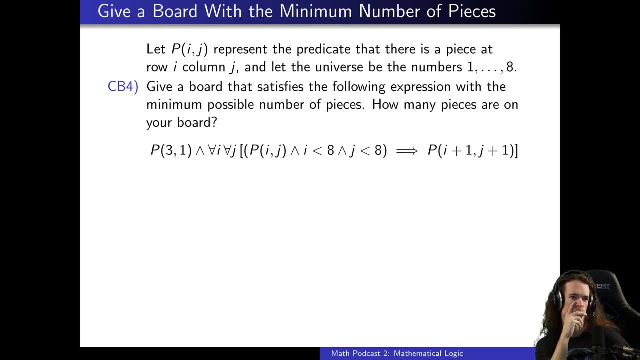 What is a board that satisfies this? What is the minimum number of pieces on your board? So what's a piece we know for sure is on the board? We can't get away from having this on the board. 3, 1.. 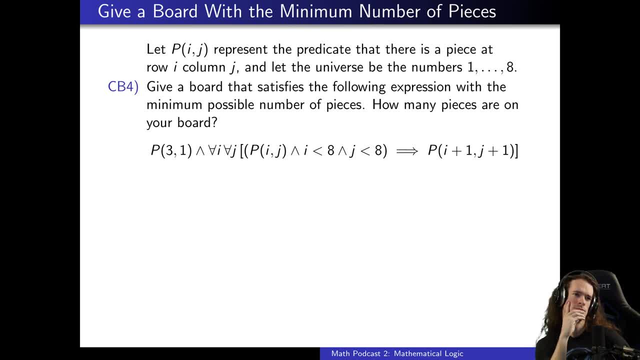 Absolutely So. we definitely have a piece in the square 3, 1.. Now does the next part force us to have more pieces? So if we have a piece in 3, 1,, does the second part of this statement, of this and statement say that we must have another piece too? 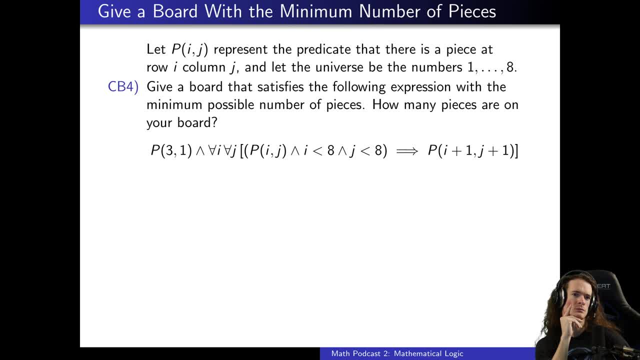 So let's see. So for all i and for all j. it says: If you have a piece in the row i, column j, and i is less than 8 and j is less than 8, you better also have one in row i plus 1, column j plus 1.. 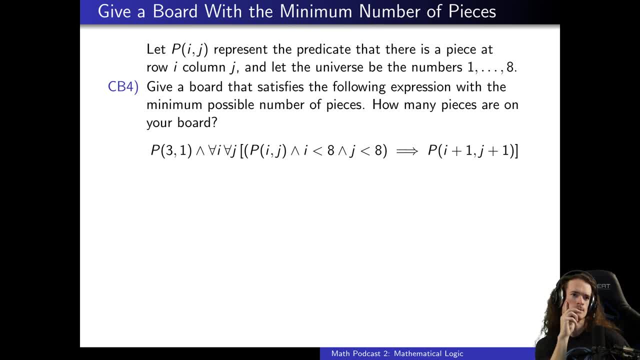 So what happens when we plug 3, 1 in for i and j? Let's see, So we have piece in row 3, column 1. And then we plug in 3 and 1 for i and j And this statement, which is true for all i and j says: 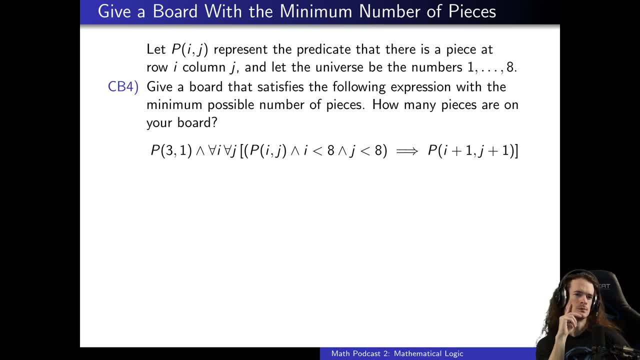 Let's see So 3. If you have a piece in 3, 1, with 3 less than 8 and 1 less than 8.. You also have a piece in row 4, column 2. Hmm, Okay. 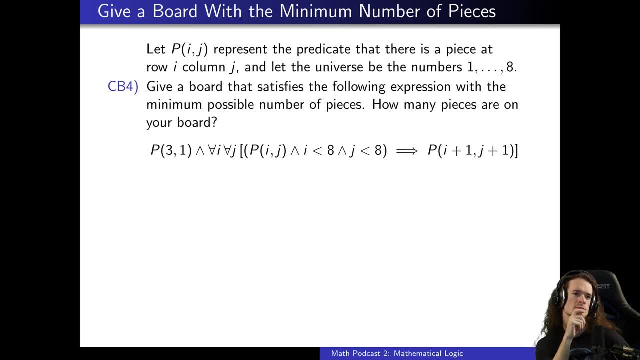 So does that mean two pieces? Well, hold on a second. Now we have to see if this statement also applies to 4, 2.. So we plug in: i equals 4 and j equals 2.. It says: if you have a piece in row 4, column 2, and 4 is less than 8 and 2 is less than 8,, then you also have a piece in row 5, column 3.. 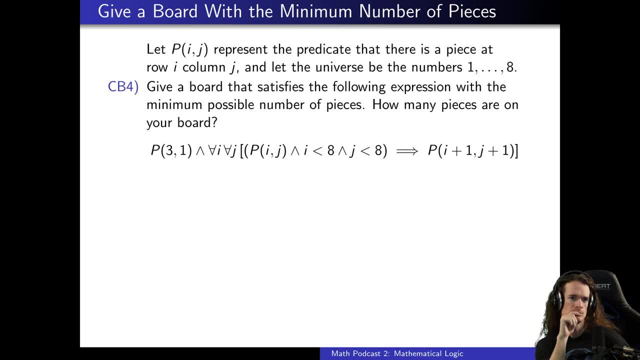 And we can apply it again and again until we get to. So we just had 4,, 2,, 5,, 3.. Then we have 6,, 4,, 7,, 5,, 8,, 6.. 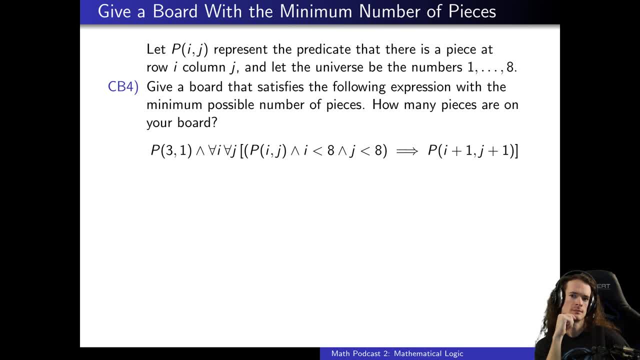 And then we hit the bottom of the board. So, if that reasoning is correct, there should be something like 6 pieces, which I see a bunch of people in chat screaming, which is nice, But I think we got it right. 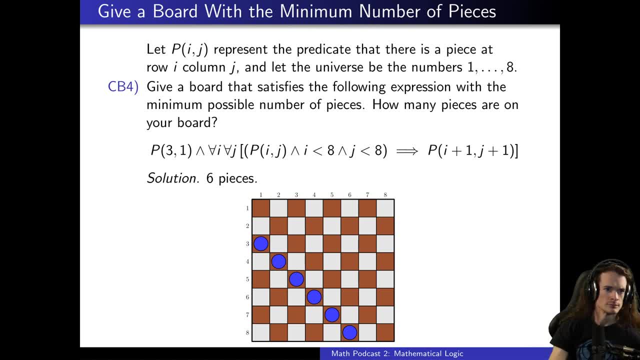 So we have this piece in 3, 1. And that piece in 3, 1, by the second statement forces there to be 1 in 4, 2. And then gives us 5, 3.. 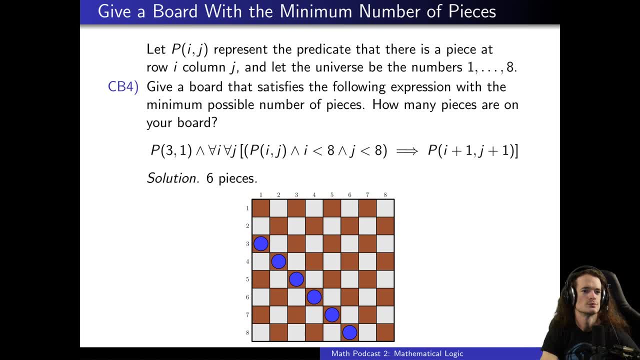 And then 6, 4.. And then 7, 5. And then 8, 6. And we get 6 pieces. Now there are boards satisfying this statement that have tons more pieces, But the minimal example only has 6.. 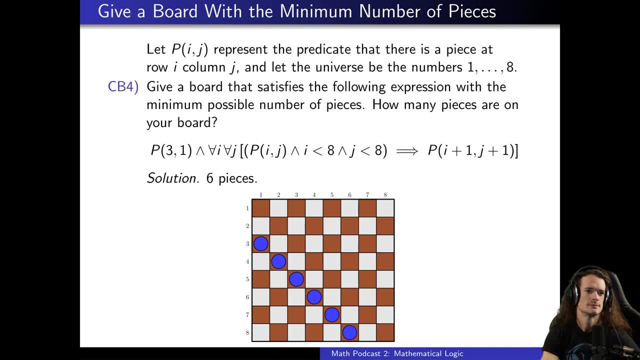 Trying to find the best fit answer. Yeah, So, and you shouldn't stop at 7, 5, because 7, i equals 7, j equals 5 is still less than 8.. And that still guarantees that you get 8, 6.. 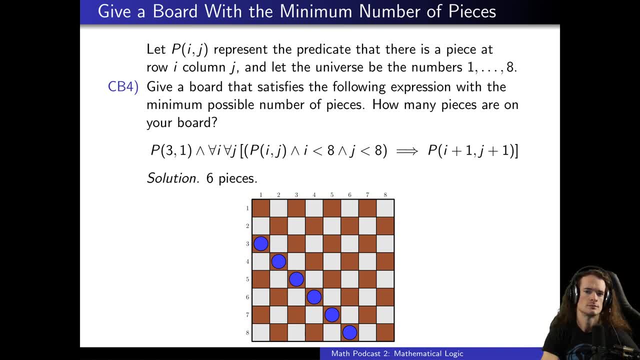 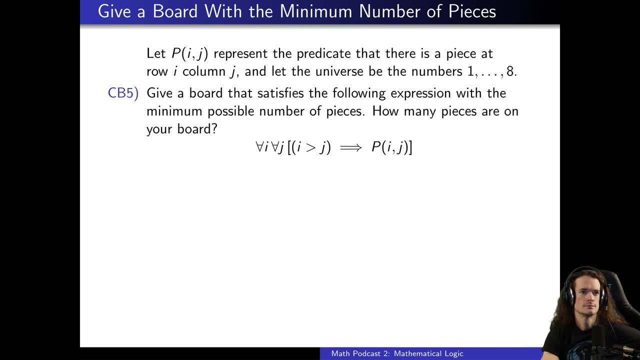 But good question. I like these questions from chat Really nice. Last one, Maybe we'll see how this one goes. It's shorter, Maybe it's still a little tricky. Suppose for all i and for all j, i greater than j implies pij. 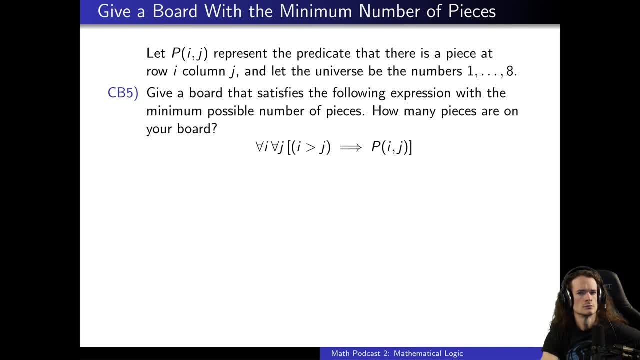 What is the board with the minimal number of pieces and how many pieces are on it? Again, pij means there's a piece in row. i column j. So we have to think about what is this statement saying? So what are the? so we're saying for all i and j. if i is greater than j, then there's a piece in row. i column j. 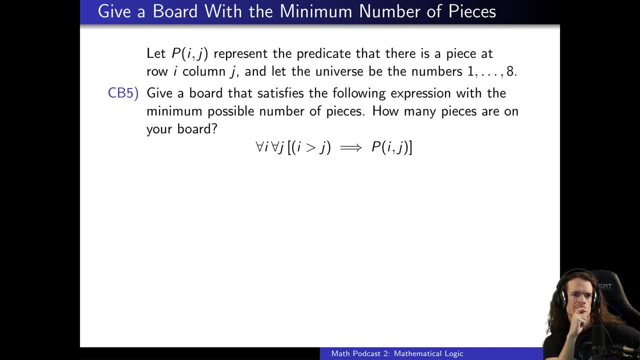 What are the what? where do those pieces look like on the board? So what are the pieces that have the row bigger than the column? So let's think of some squares on the board and then think of whether the row is bigger than the column. 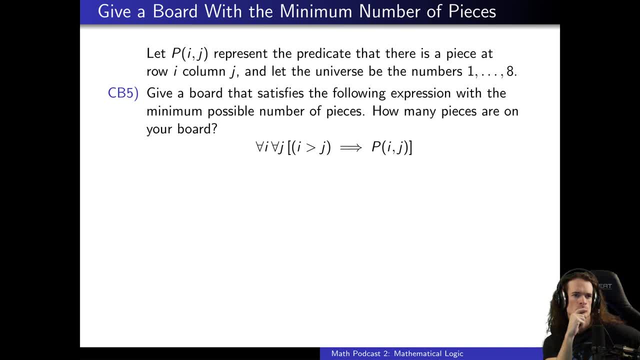 So suppose we have a square on the diagonal. What are those squares? Those are the squares where the row is equal to the column, So those don't count. Okay, Now let's try a square like 2, 1.. 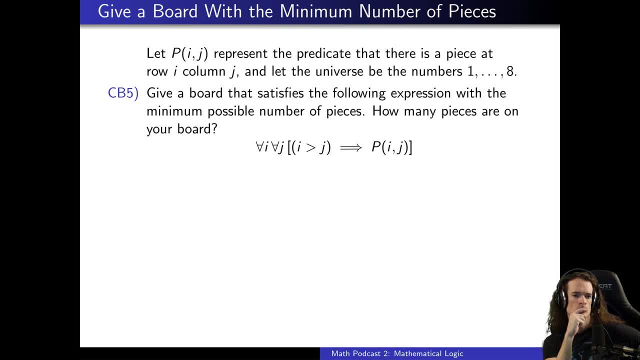 2, 1 has the row bigger than diagonal. The same is true for 3, 1 and 4, 1 and 5, 1, all the way down to 8, 1.. And then, in the second column, what are the squares that have the row bigger than the diagonal? 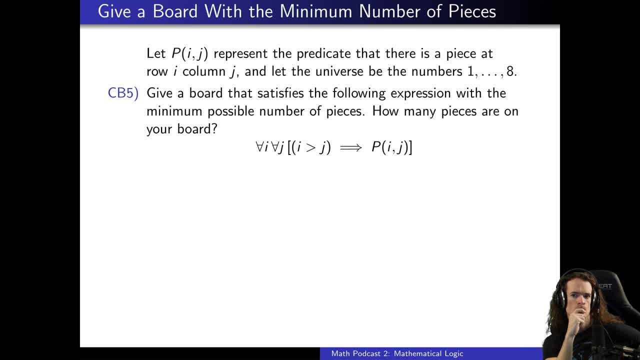 That would be 3, 2,, 4, 2.. When I say 3, 2, I mean row 3, column 2, row 4, column 2,, row 5.. So this condition is saying: for every square that's below the diagonal, there's a piece there. 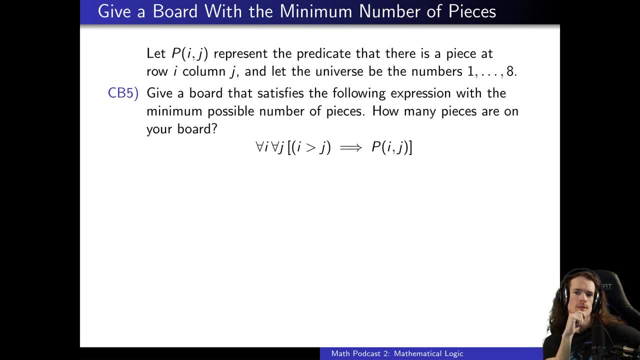 So we just have to count up how many are there. And counting problems like this come from a field of math called combinatorics, Where you have to count things, So it's like how many squares are there below the diagonal? So is there some way we could do this? 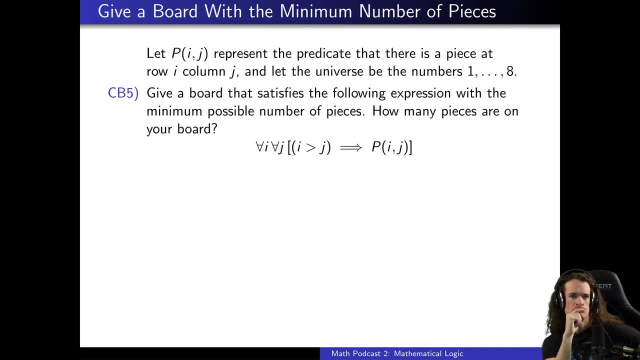 Now people are saying: why don't I try adding 1 plus 2 plus 3 plus 4 plus 5 plus 6 plus 7? Something like that could definitely work And we have to do that arithmetic. Sometimes you can use other ways like symmetry. 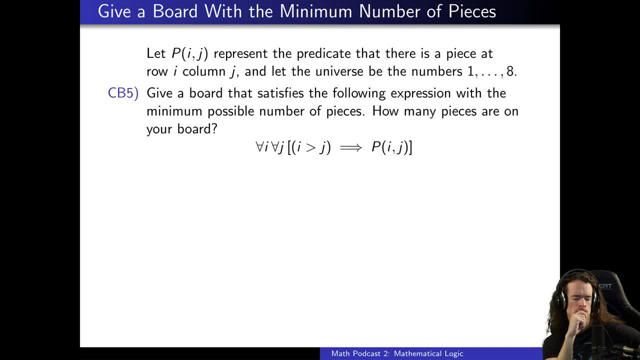 So we said that none of the squares in the diagonal work, So that removes 8 squares. So we started with a total of 64 squares. We had an 8 by 8 board. We removed 8.. That brought us down to 56 squares. 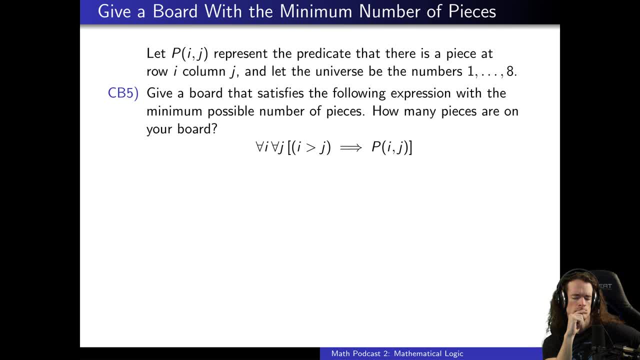 And then of the remaining 56 squares, half are below the diagonal and half are above the diagonal. So 56 divided by 2 should be 28.. And that's another way of computing the same exact quantity: 1 plus 2 plus 3 plus 4 plus 5 plus 6 plus 7.. 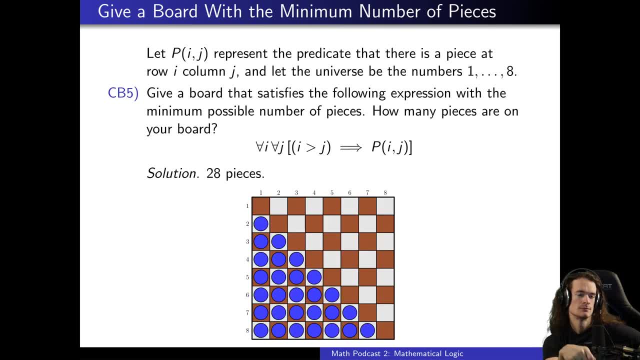 So let's see if that's right. Cross fingers: 28 pieces, Oh my, And you can see they're all below the diagonal. So this gets it, And that's the end of our review of first-order logic. 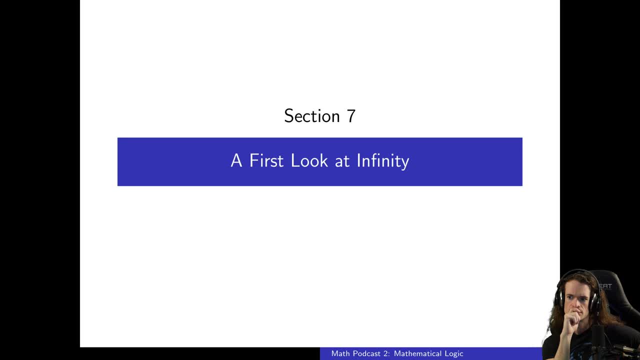 So this is up to you. We could spend a few minutes talking about infinite things, or we could save that for next time. It's up to you. Let's see what our uptime is. We've got 1 hour 49 minutes in this discussion so far. 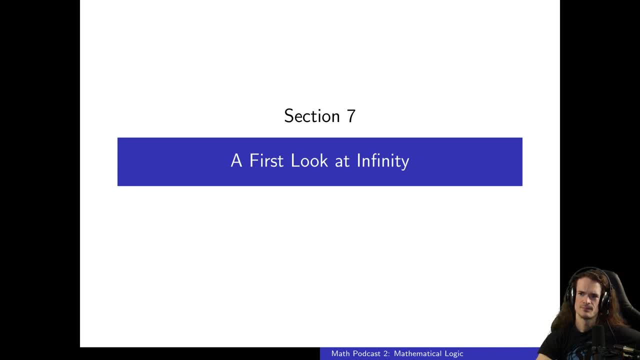 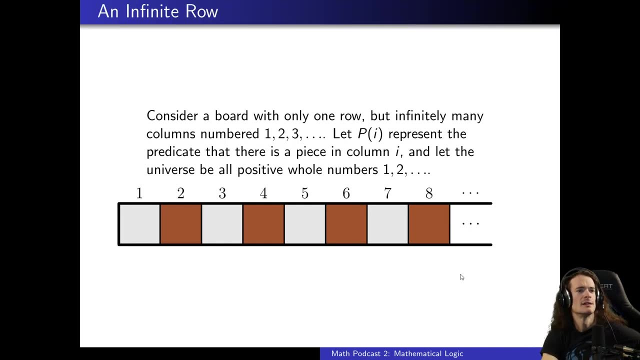 You want to just finish this off. I think this is about maybe 5, 10 minutes. Let's hack and do it, dude, Let's do it. Let's look at infinity, Let's look at infinity. So now we're going to take our, we're going to get a glimpse of math, some more advanced math. 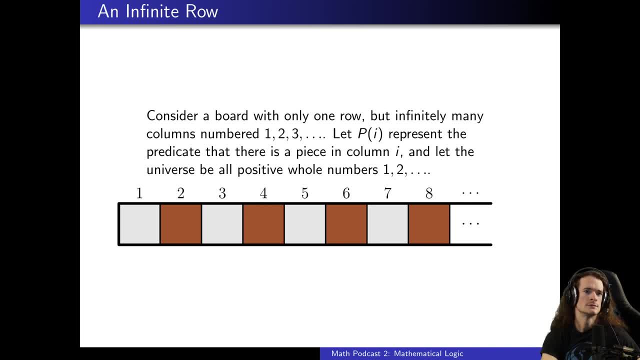 And I want to see if we can use some of our first-order logic that we've learned to think about something that's a little more complicated. But we're going to stay within this like chessboard idea, But I'm going to make the chessboard simpler and harder at the same time. 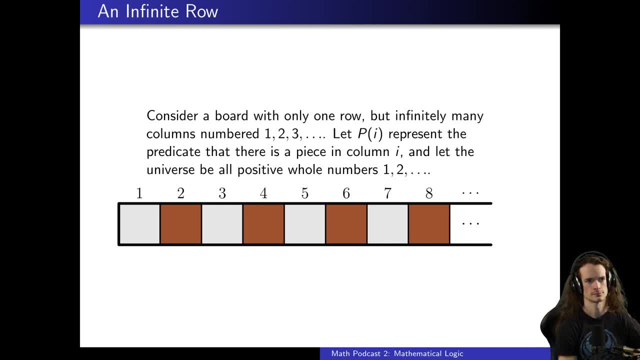 We're going to look at only one row of the board, But I'm going to let there be infinitely many columns. So it's this unending row of squares on a chessboard. The columns will be numbered 1,, 2,, 3,, 4,, 5,, 6,, 7,, 8,, 9,, 10, unending. 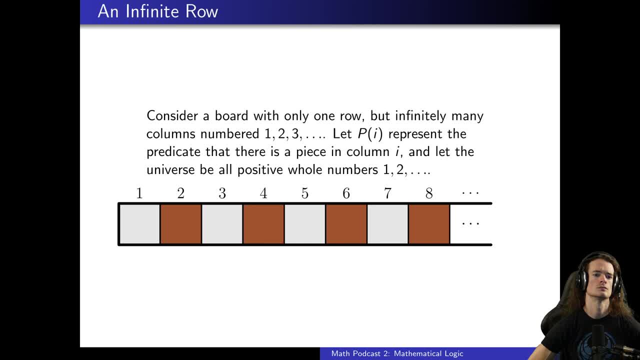 All the positive whole numbers will get a column number. All of them are legal column numbers. So we have one enormous row And we'll let P of I be the predicate that represents. there is a piece in column I. We don't need a row anymore. 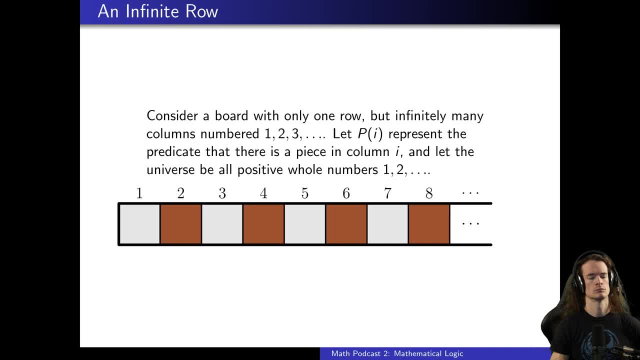 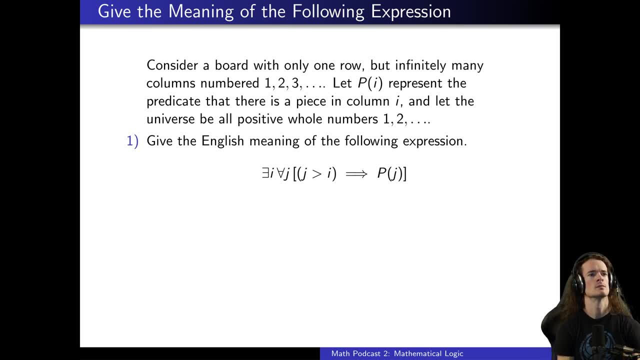 There's just one row, So just the infinite row. So here comes our question, And these are going to get a little sneaky, So we're going to think about this. But this gets to the heart of the notion of infinity and calculus. 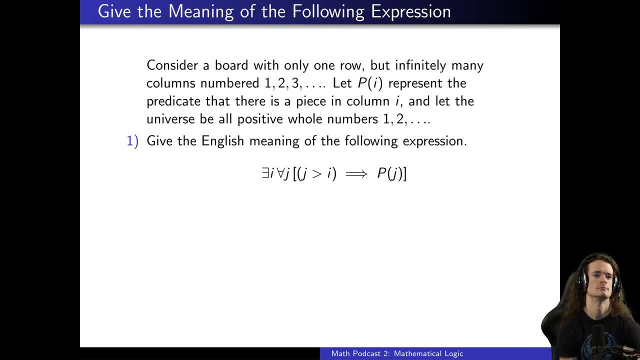 Even though we're not going to talk about any numbers like any, like functions, We're not going to talk about derivatives or any of this stuff in calculus, But we're going to try to get at the heart of some of the concepts in calculus. 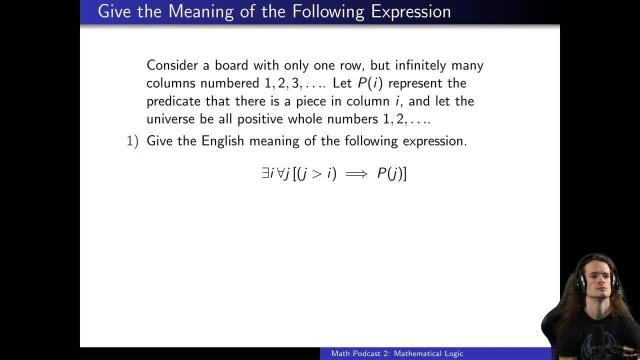 Just using some of the first order logic that we've learned. So I want to give the English meaning of the following expression: There exists I, such that for all J, J greater than I implies P of J. Okay, So these statements about this infinite board are not going to be trivial. 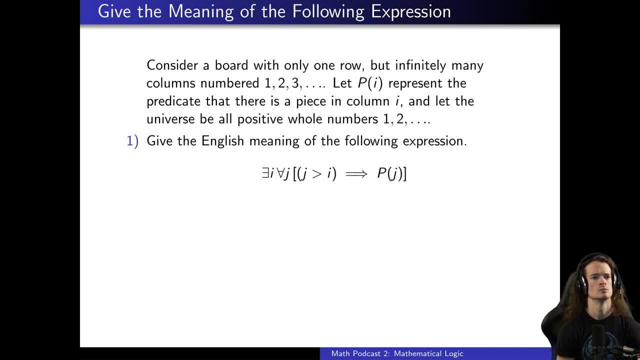 So it's really going to require some thinking to understand what they mean. So it's good to think of, like, what kinds of boards, what kinds of rows and pieces on those rows would satisfy this statement. So one more time, There is an I such that for all J. 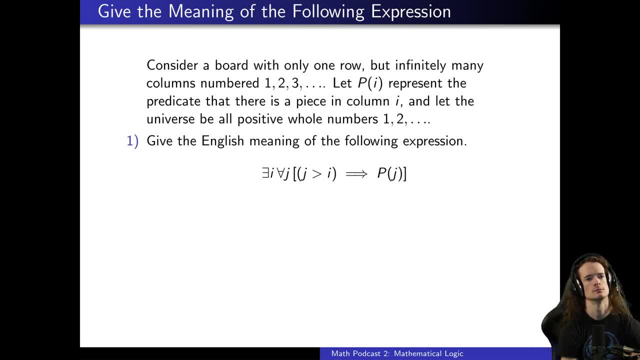 If J is greater than I, then P of J. What does this mean? And pay close attention to the order of the exists and for all. So let's try to come up with an English meaning for this statement. And just as a reminder, P of J here means there is a piece in column J. 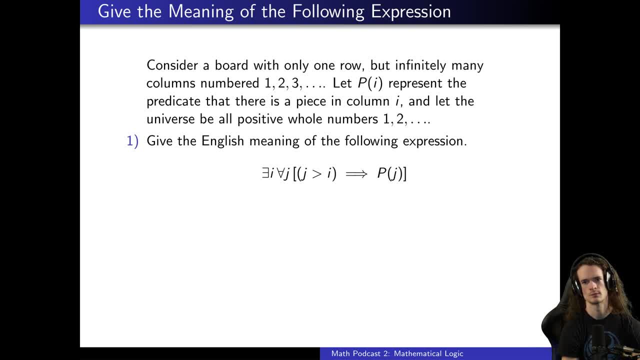 And this is not easy. So just fine, chat If you want us to answer. don't worry about being wrong. The stuff we're doing now is getting harder. This is tricky stuff, So just think aloud. Okay, Someone is saying: oh, this is giving me the idea of kind of like sequences and convergence. 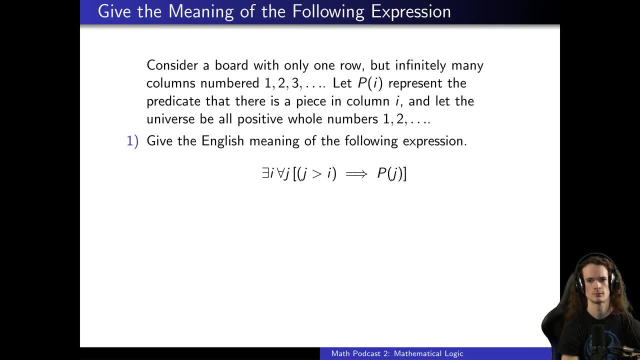 This is like the beginning of the idea of like thinking about sequences And sequences. It's like one of the core ideas in calculus Someone is talking about: okay, think about where the row is filled. There's pieces, There's infinite columns. 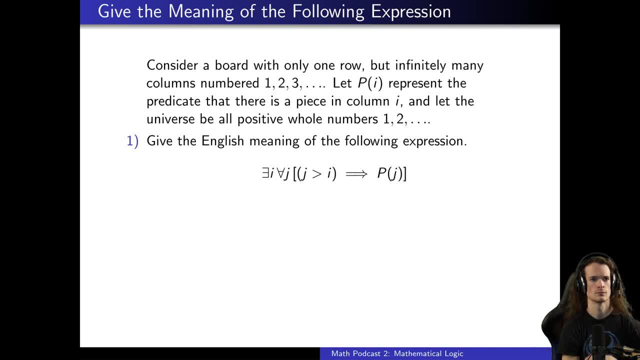 Okay, I like what Chad is saying here. So let's see. So we're first saying there exists an I, So there is a position I somewhere on the board. That's the exists I. And then it's saying, for all J bigger than I, there's a piece in J. 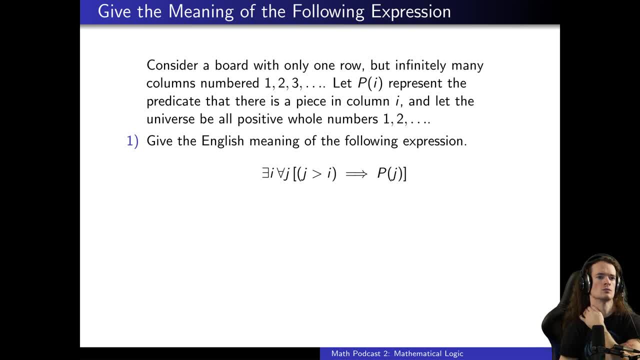 So what do we think that looks like? It's like there's a position I such that everything to the right of it has a piece in it. So at some point, at some column after that column, the row is full. 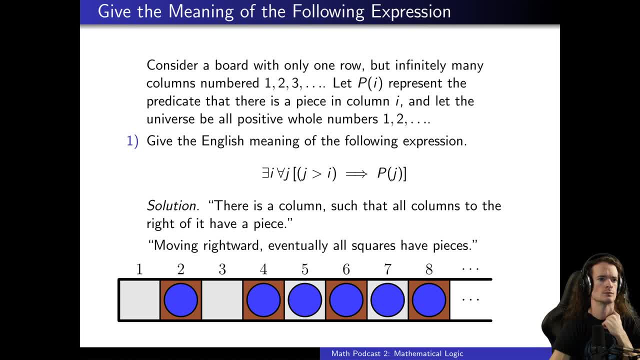 So hopefully that's what it says in the solution And hopefully I have a picture there, Yep, That says so. in this picture you can see like position three, Position three and on all pieces. Sorry, position four and on all pieces. 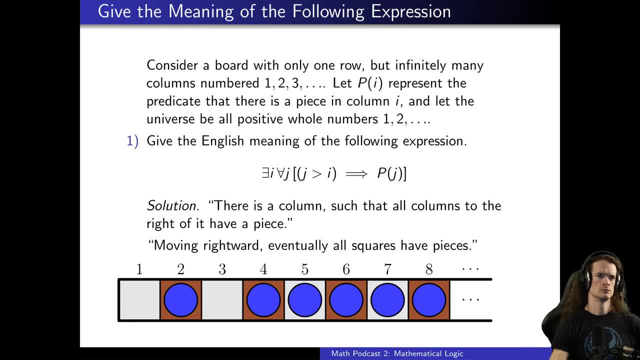 So everything to the right of position three is full. So one way of saying it is: there is a column such that all columns to the right of it have a piece. Or in other words, if we're moving rightward along this row, eventually at some point all squares have pieces. 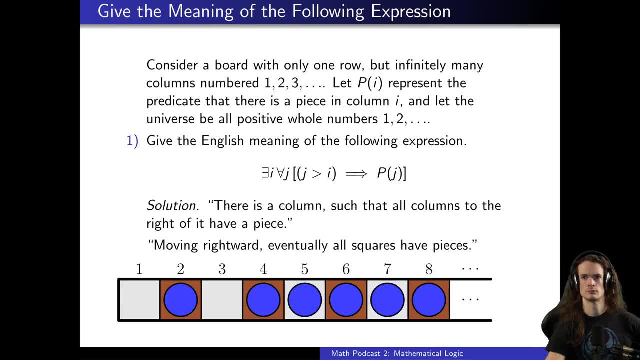 Because eventually there's going to be some position where everything to the right of it has a piece. So this notion of eventually is full, So it's key to thinking about infinities and the way calculus is sort of thought about and the core concepts of calculus. 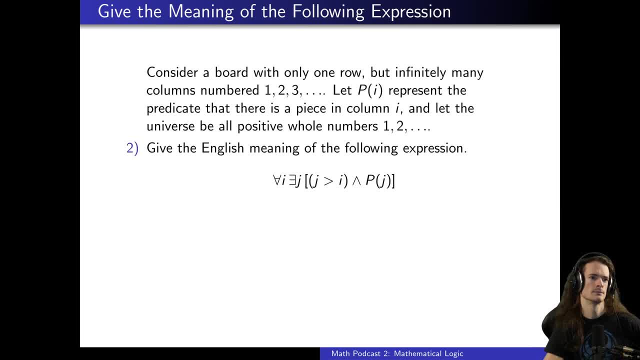 Think about things like: eventually, Let's try another one. Give the English meaning of the following expression: For all i, there exists a j, such that j is greater than i and pj, So this one's a little bit easier, Okay. 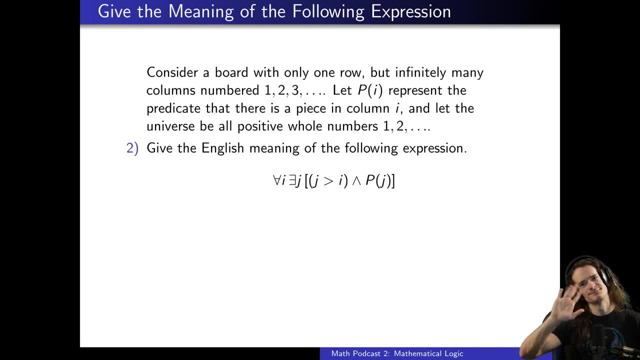 It's a little different, The order is different And then now there's an and symbol inside. So try to think of what this one means. And again, these are not easy. These are starting to really get at something deep That took mathematicians hundreds of years to come up with. 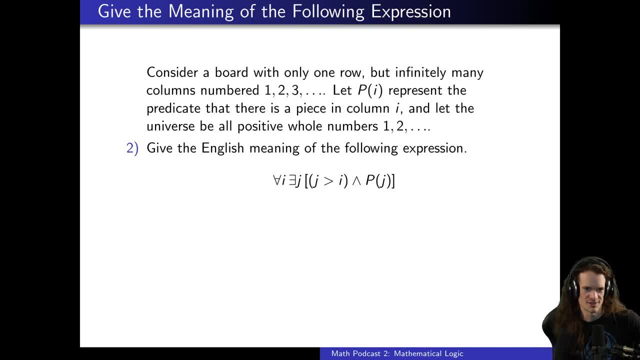 So we're doing hundreds of years in about five, ten minutes, Which means if you can answer this question, you're smarter than all of them. We're learning at an incredible pace. So someone's saying: however high you count, there's a piece. 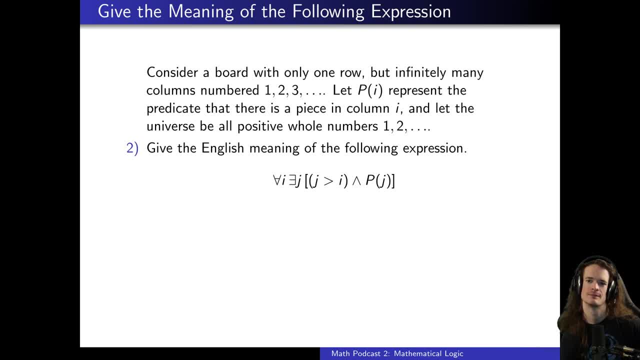 Yeah, So that's a good answer. Yeah, yeah, yeah. So someone's saying it isn't the same as before. There's a subtle way this is different And we want to think about that. So let's think about what this means. 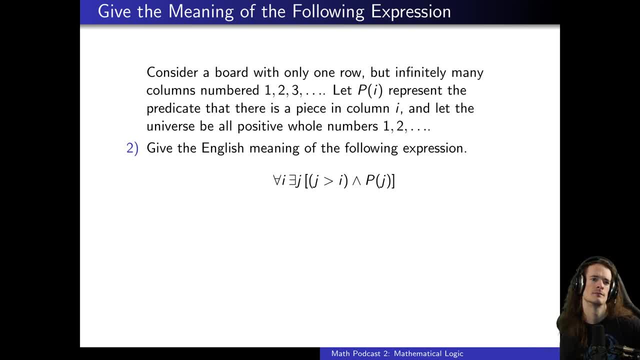 It's saying: for every position there is a position to the right of that position that has a piece. There's another way of saying this in a very short way. I'm not saying it's tricky, but it's like hard to know that that's what that meaning is. 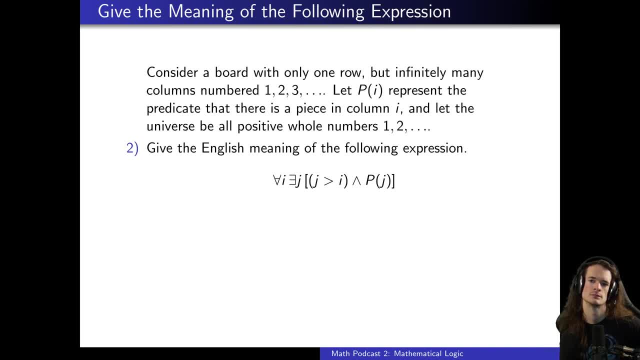 So another way of saying this- and this is interesting to think about- is that this is the same exact thing as saying that there's infinitely many pieces in the row. Let's think about that, Because if there exists another piece every single time, 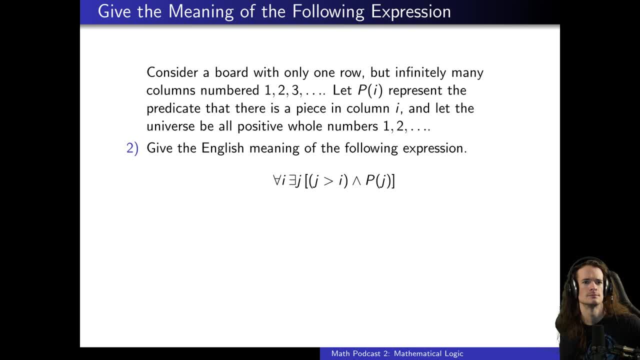 Exactly. You're never going to run out. Yes. It's saying: for every position there's going to be a position to the right of you, a piece to the right of you, So there's always going to be more. It is not saying the same thing as the first statement. 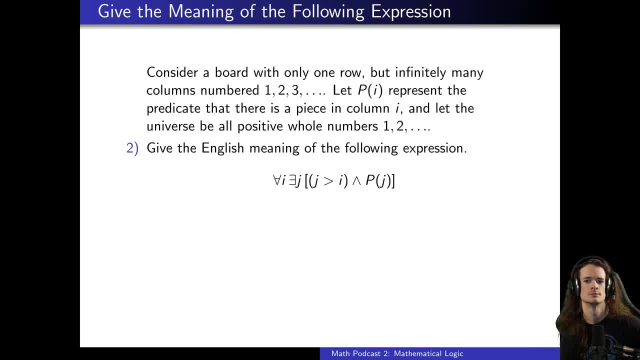 So the first statement we had was that at some point, everything to the right of it has pieces in it that you eventually are full. It is true that if you are eventually full, then you have infinitely many pieces, But you can have infinitely many pieces and not eventually be full. 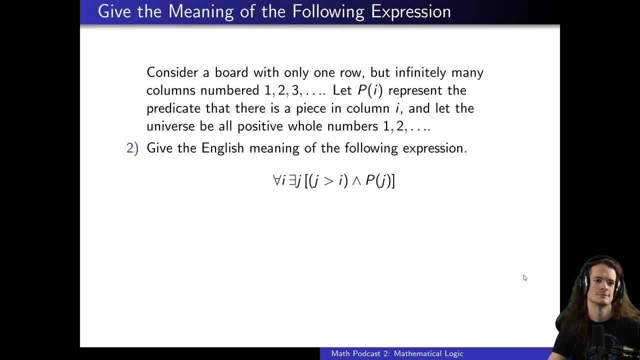 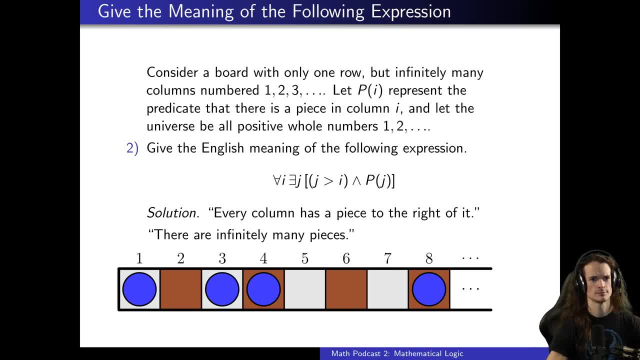 And then I can't draw the infinitely many columns, So assume that you keep going and there's going to be a no piece and then a piece, and then a no piece and a piece, And maybe there's a bunch of pieces in a row. 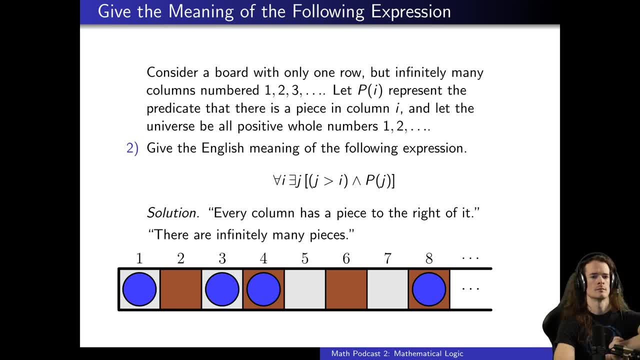 Maybe it's even eventually all pieces, But this is not saying that that has to happen. It's just saying that there's infinitely many. Or, as we said, another way of saying it is that every column has a piece to the right of it. 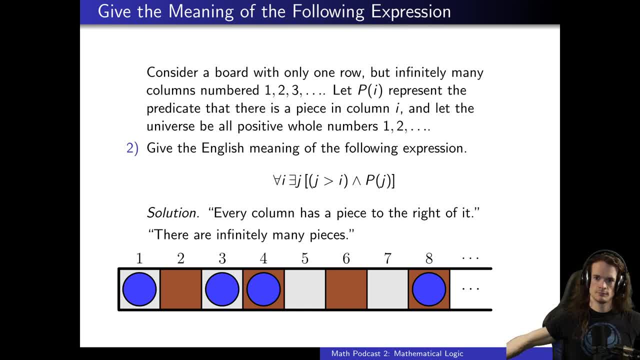 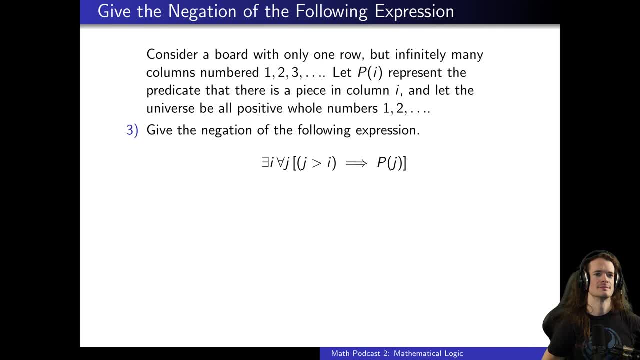 And these are saying the same thing. Okay, I think we have two left And then we are officially done. What is the negation of the following statement? So we're getting tricky here. Here's the statement, And I want its negation. 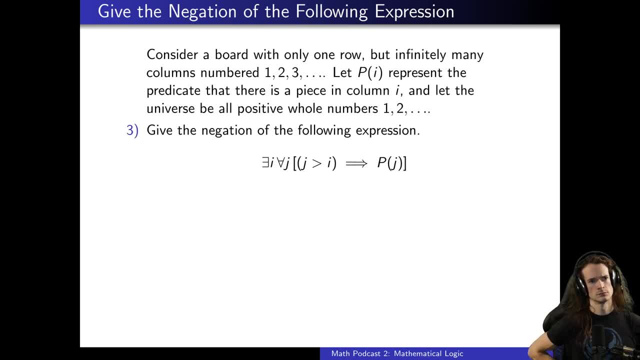 There is an I, such that for all J, J greater than I implies P of J. So this is the same statement from question one. What is its negation? So, if we recall what this statement means is, there is a position where everything to the right of it is full. 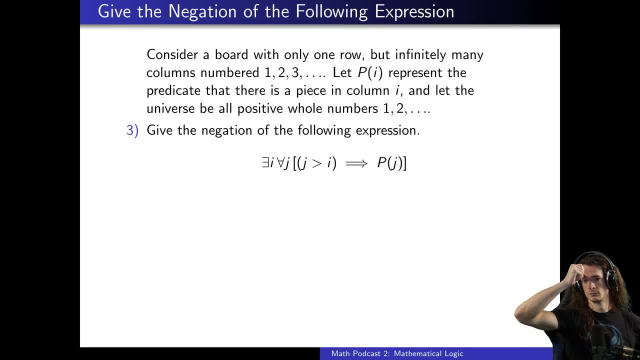 So eventually, all the squares are full. What is the negation of that statement? So a simple way of saying it is: it is not true that eventually all the pieces are, all the squares are full. So that's a simple way of saying it. 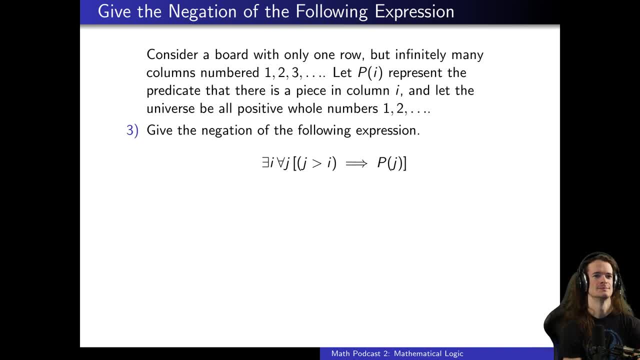 Another way is we could just be one of these symbolic robots and just go through it with a not symbol, And so the negation of this would be for all I. there exists a- J Where the statement in there is not true, Which would mean that 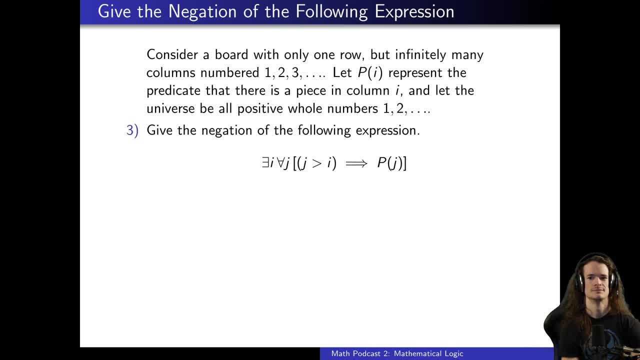 Yeah. So the negation of this implication would be that J is greater than I and there's no square in it. So you could either So two ways of saying this. You could either say it is not true that it is eventually all full. 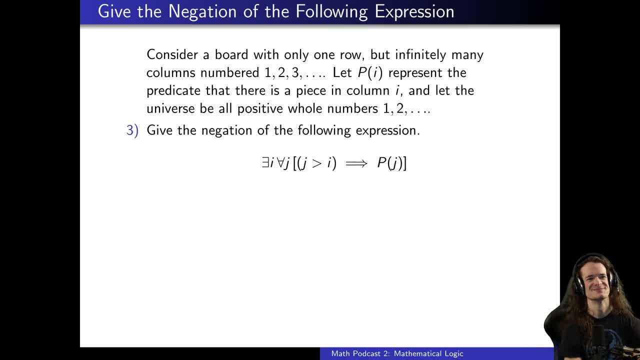 You could also Another way of saying that is: there are- And this is a- This is a little bit of a leap, but I'll say it anyway- There are infinitely many empty squares, which is sneaky, But that's the answer and I think, hopefully. 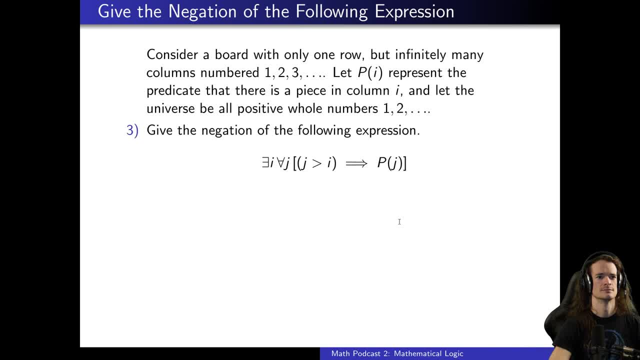 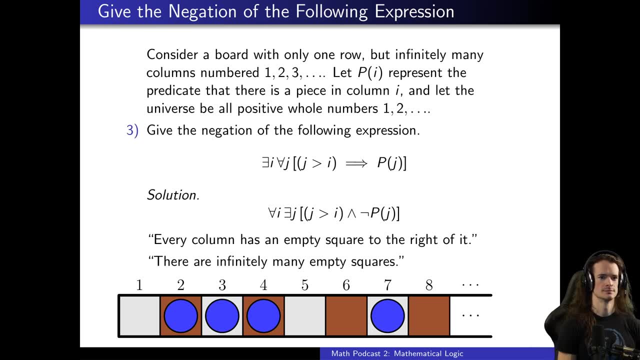 the solution reveals that. But these are not simple. These require thinking about what's going on and really thinking about what the logic means. And I think it's good to ponder about these, because these concepts are core to things in calculus. So let's do the final one and then we'll. 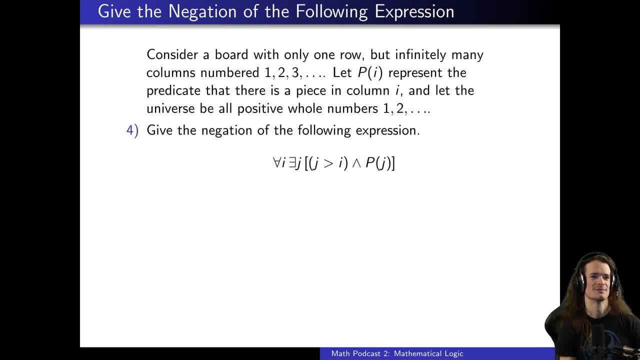 give everyone's brain a rest because it's been a lot of logic. The last one, question four. So I want the negation of the second statement we did, which is: for all i, there exists a j such that j is greater than i and pj. 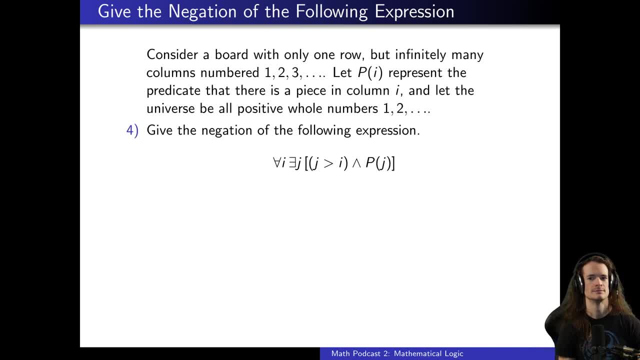 In other words, as we said, for every position there is a position to the right of it that has a piece which we said, if we recall, is the same thing as saying it's infinite. There are infinitely many pieces, So what's the negation of that? 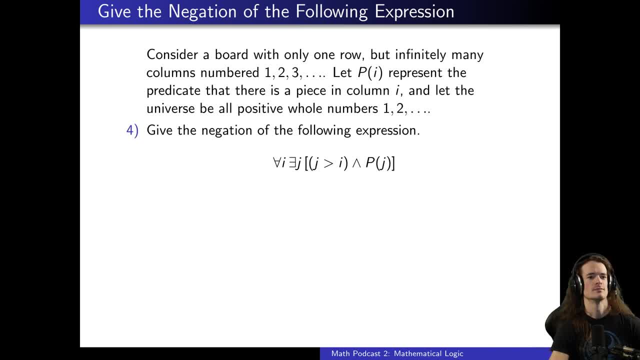 So what's the negation of there being infinitely many pieces? You are going to run out at some point. Exactly, There are finitely many pieces. So, and hopefully that's the answer, Another way of saying it, if we just. 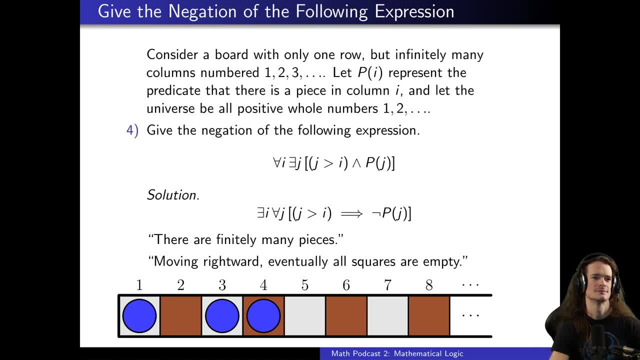 go through the symbolic robot and we look at the solution, you'll see that there is an i, such that for all j, j is greater than i and pj, which implies not pj, Or in other words, eventually all the squares are empty. 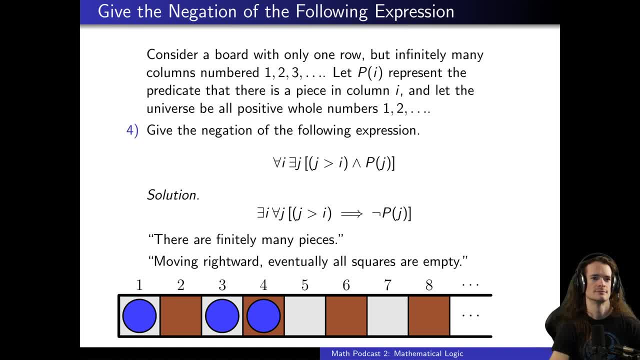 And you can think about why. that's exactly the same thing as saying that there are finitely many pieces. That saying eventually all the squares are empty is exactly the same concept as there are finitely many pieces, And these are like a bit of a brain twister. 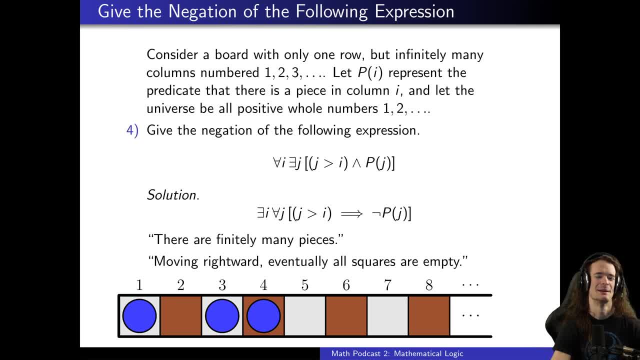 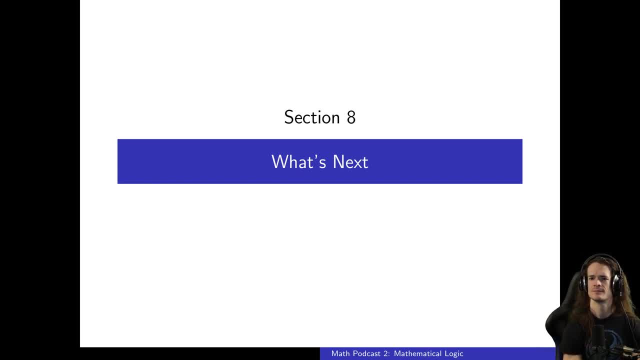 They're hard to think about, but they're interesting And I think that's it. So the next page just says what's next, And I think that's a question that we're going to think about, but also we'd love input from chat about what topics. 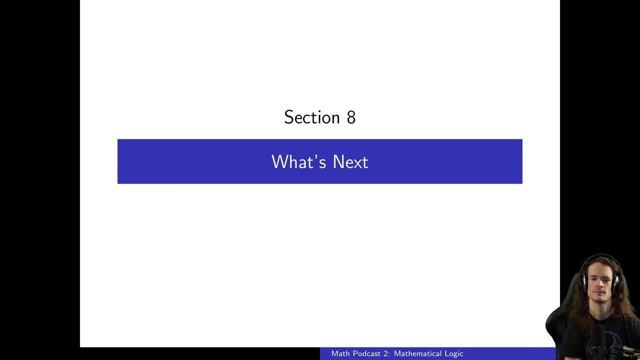 we find interesting. I know we've had ideas to try to make them connected to games. Maybe there might be some probability. there could be poker or maybe some probability that occurs in some of the video games. NeuroPlay is like wow, We could talk about one of the topics I've thought about talking about. 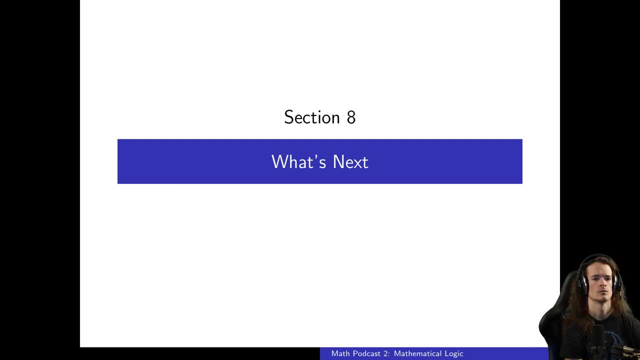 is like explaining the universe, Explaining what is statistics and giving some simple examples about how statistics works. some of the core ideas in statistics, But we're open to suggestions. We'd love to talk about tons of topics. Math is broad, One of the domains that was really exciting for me in university. 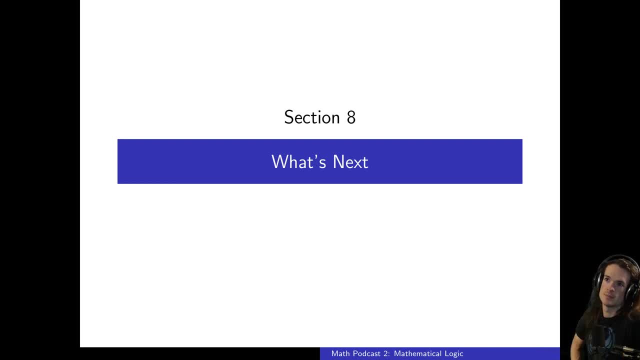 was, in judgments and decision making, the difference between the mathematically correct approach and the intuitive, natural, human approach. We have a bunch of heuristics which cause us to take mental shortcuts that lead us to make predictable errors kind of across the board. 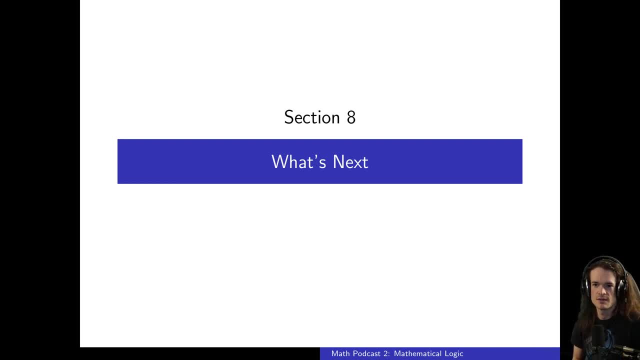 just how we're wired. So gambler's fallacy is one of those. So I think having a pass at a lot of those biases that we carry around and oftentimes aren't aware of, and then how to be rigorous and logical moving through those, 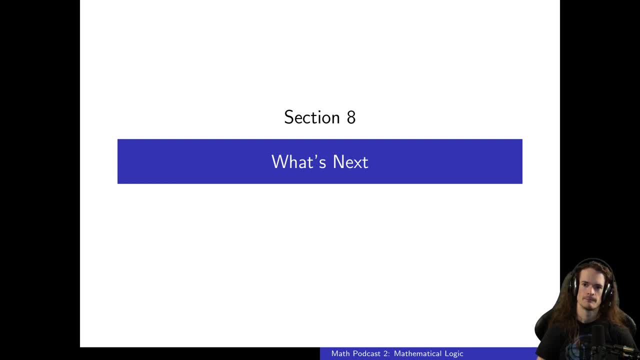 Sure We could do. yeah, So I think those are great. Yeah, I mean, people are notoriously bad at probabilistic intuition and you sort of have to relearn it. And then you said- I think you said previously that, like when you were studying to be good at poker- 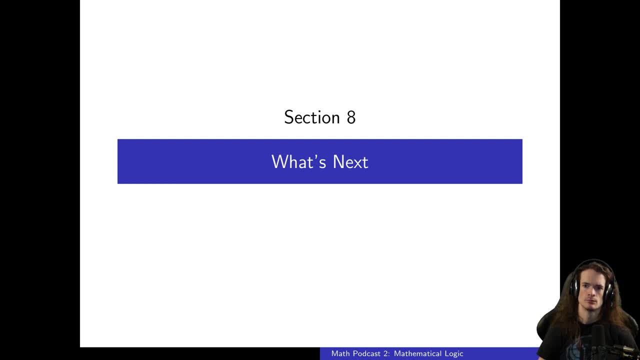 you had to like, fix some of these biases and train yourself to spot things. And then these come up all the time when people are doing studies, these notions of selection bias or regression to the mean. There's lots of things you have to know to look out for. 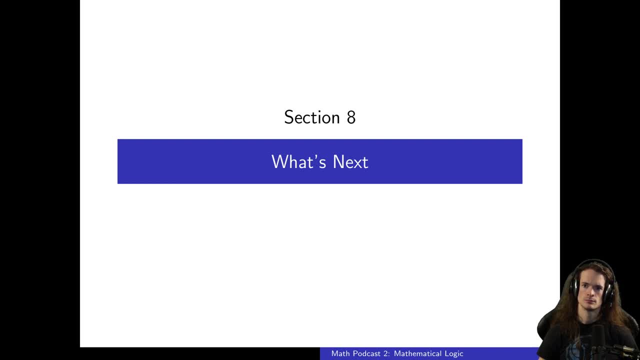 because they can definitely ruin both your- if you're doing a statistical study- your results. They can also ruin your intuition. They can ruin your intuition about what's going on in a game and cause you to make inferior decisions, or in life in general. 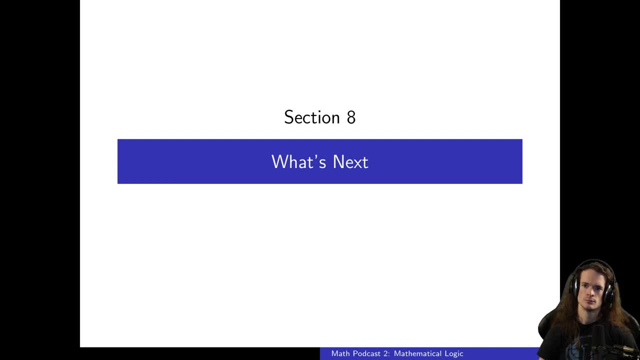 And learning how to be objective and to properly understand how the probability and the various mathematics underlying these processes works, will help you to just make superior decisions. So, but in general, we are open to lots, of, lots of topics. We'll try to present them in a similar way. 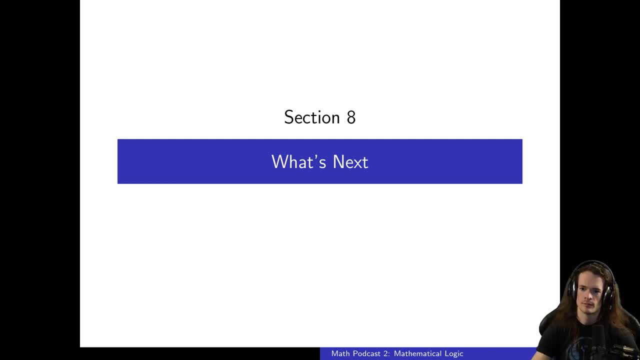 where there's little prerequisites, but hopefully by the end of it we can talk about some interesting things that really have some importance And as a result of this, I hope, if you ever do want to look at a book on logic or think logically about topics. 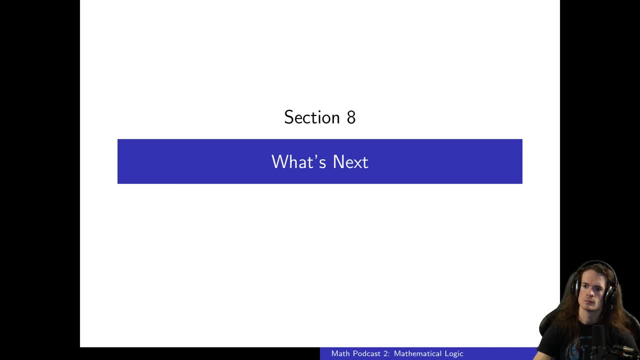 or want to get into more math or computer science, that this will give you a primer that helps you with all the logical content, both the propositions and the first order. There was a question about whether these slides could be uploaded somewhere. I could just upload them to the math channel in Discord. 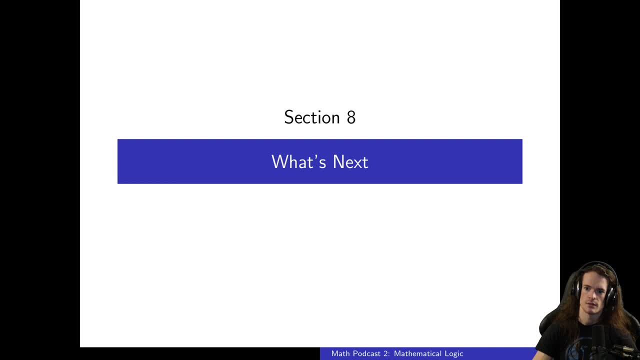 Does that work for you? Absolutely, Neuro has all the slides, Sweet. Any other questions I'm happy to answer, but I hope all of you enjoyed it. I hope it was informative. Yeah, I really liked the progression from at the very start. 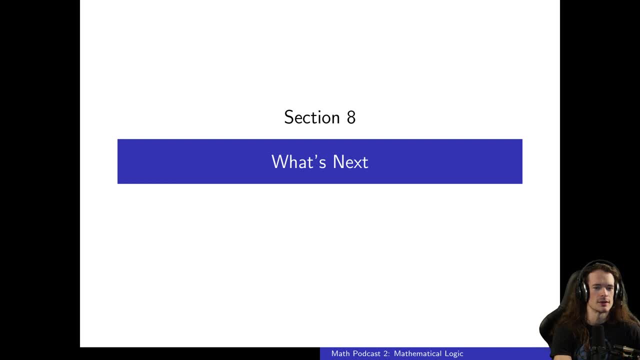 It's so simple that you're like, oh man, come on, Like everybody knows this, And then by the end, some people they got raided in here from Ragnarok And it's like you're at the most confusing part, at the very end, where all the other knowledge. 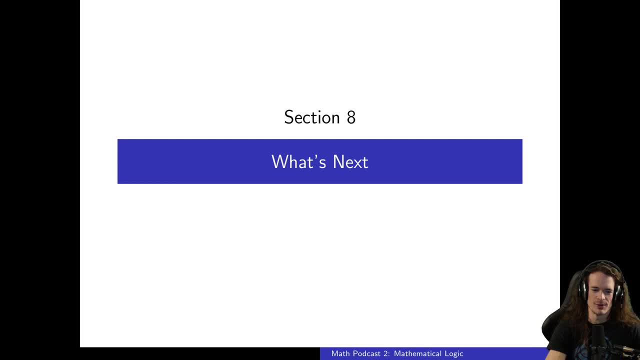 over the course of the lecture is built up And you're like: why does my brain feel like I just got thrown into a washing machine? I think I was here before and Brett said no prerequisites, And now you're talking about infinite rows, and there exists. 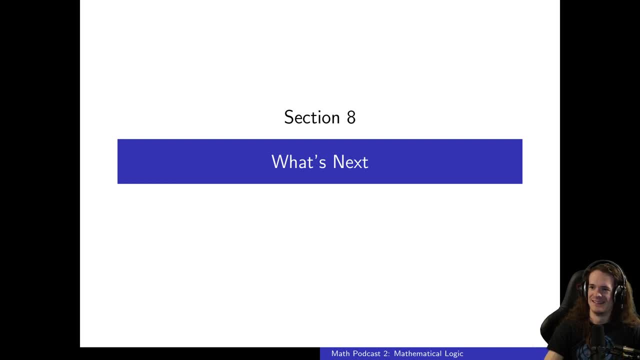 What just happened? I made a wrong turn somewhere. This raid- Yeah, I was taking a right where it took a left. Yeah, Nice. So these slides are in the math discord channel And, as we said earlier, the logic comes up everywhere in mathematics. 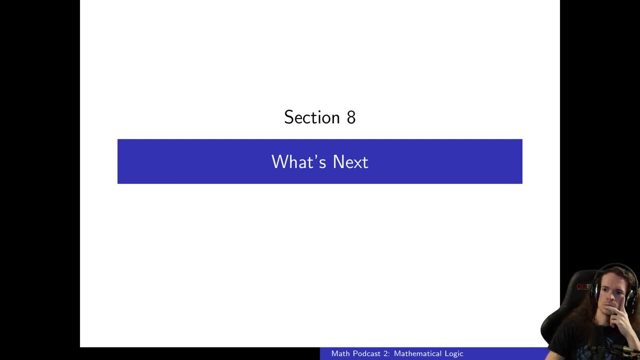 and philosophy and just in law. obviously It's like a sort of general thought that the people who study logic and philosophy and math tend to do very well in their LSATs because they're sort of these logic monsters. So it comes up in law, philosophy, mathematics. 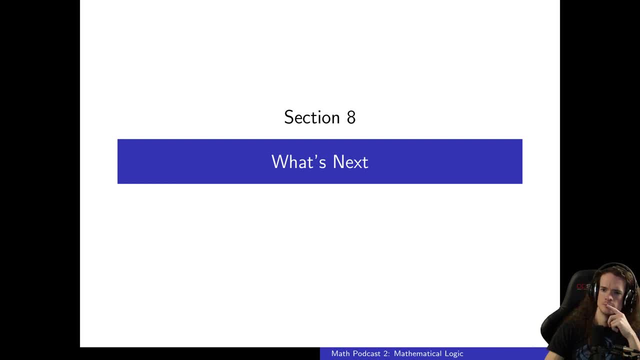 I mean all the fields that build off of math have strong ties to mathematical logic. There were mentions of music theory before. How connected do you feel you are to that? Yeah, So there's OK. So there's certain aspects of music based on. 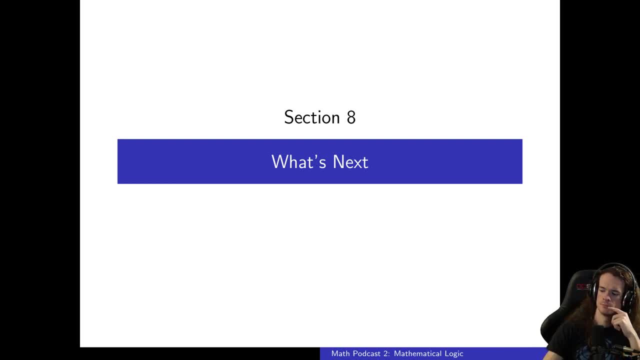 So let me put this in context. So part of the answer is not at all. I mean, basically, to prepare for the next session, I would just become a musician and then teach on it. So I don't really have that much music background. 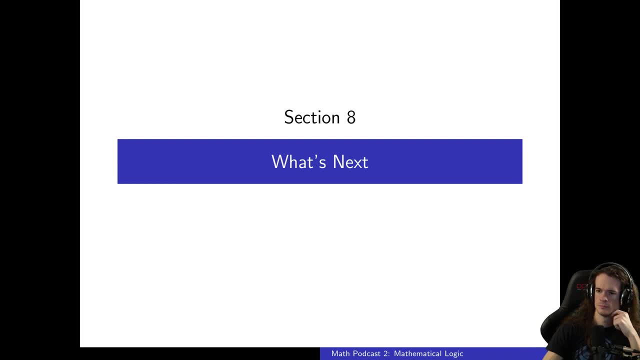 That said, I mean through the math I've studied. I do know a topic which is called harmonic analysis And that is sort of used to understand and take a signal that you would produce with an instrument or with your voice and decompose it into its frequency components. 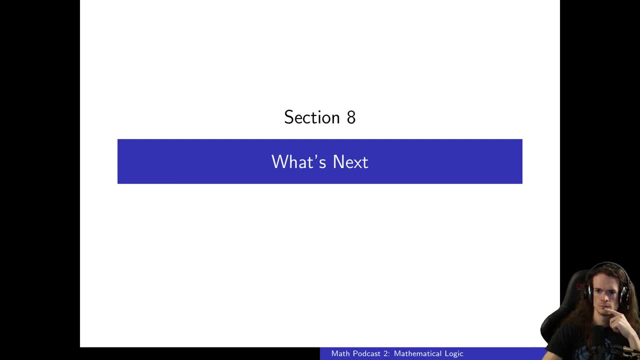 and say, oh, these are these pitches, and understand how to do the signal processing on music. So I know how to do that And I could describe that, And I try to describe it at a level that is understandable, But I wouldn't be able to give all of the color. 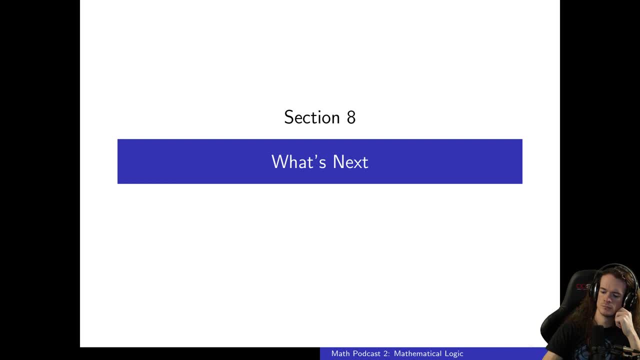 that a musician would and to explain maybe some of the deeper music theoretic aspects of it. So it's possible that I might not be the perfect person for that, even though I could definitely give you a purely math angle on it. Yeah, I mean I've done some frequency analysis on musical notes. 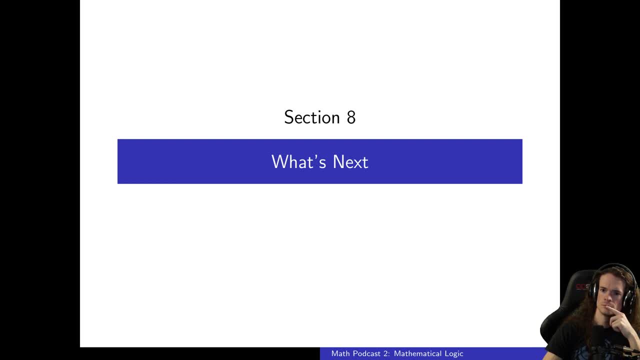 and musics being played and understanding what the overtones are and how the different harmonies combine to produce different notes and why a human voice singing a note is different from each different instrument playing the note. And you can see that pictorially by decomposing these notes. 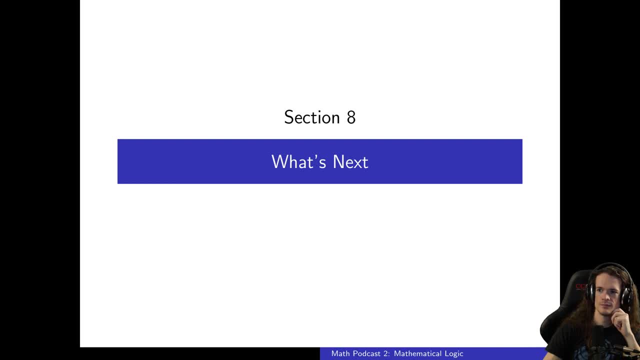 using signal processing, And that's the kind of signal processing that is done in the tools that audio engineers use, And that's something I can talk about. But I think, to do this justice, you probably want someone who is more of a musician. 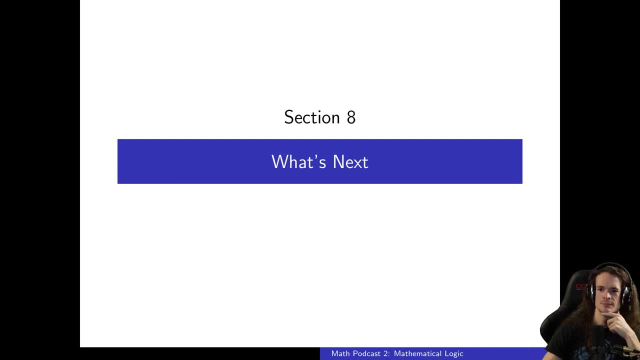 Incompleteness theorems. So incompleteness theorems is not the same, but it's kind of related. So, if you remember so people, if they haven't, we did a podcast before this one. We did a little bit of an intro to why we're doing these podcasts. 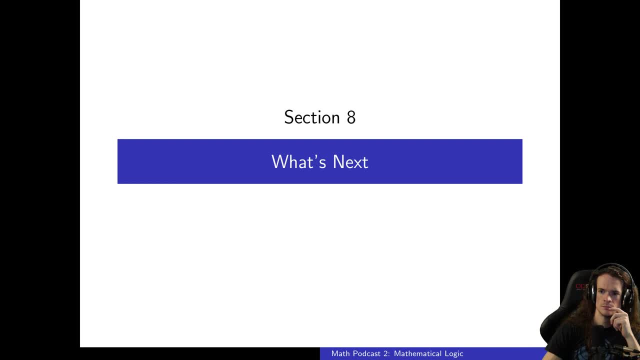 And we did a history of probability And in the history of probability we came to this guy, David Hilbert, who basically in the beginning of the 1900s said like hey, these are some problems that are really important. And everyone said this guy knows what he's talking about. 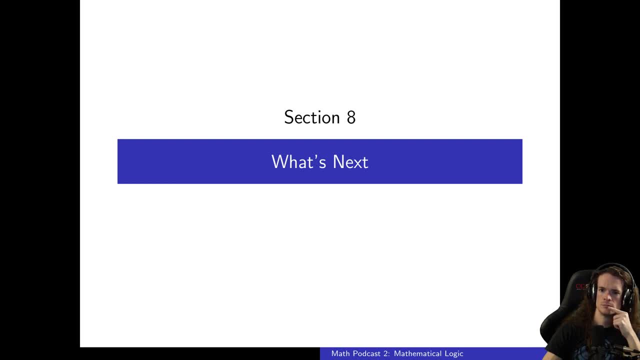 This is obviously a joke And David Hilbert is an amazing mathematician. It wasn't just those problems, But he came up with this list of problems which are very famous and everyone was working on them, And I said as a digression that one of those problems was: 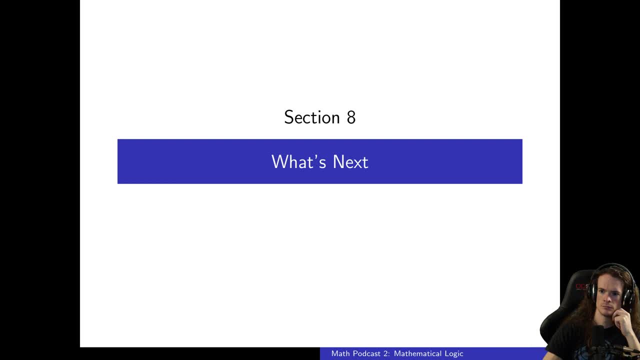 ended up being that a certain type of mathematical problem is unsolvable. It was these things called Diophantine equations solving them, And it's like an impossible task. The actual solution was that this is impossible And that is somehow related to the incompleteness theorem. 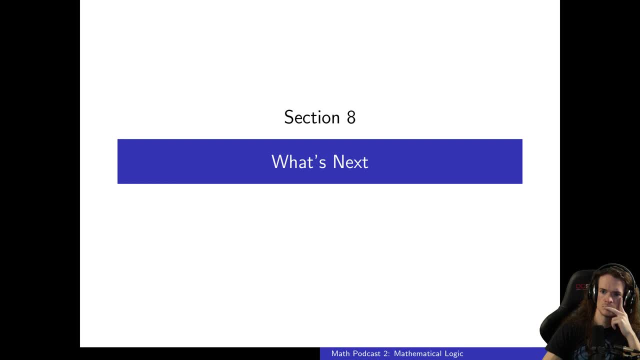 And I'm going to talk a little bit more about that in this book, which I unfortunately haven't read- Gödel-Escher Bach, which also talks about similar things, And it talks about a little bit of a dire situation, about how there's different parts of the incompleteness theorem. 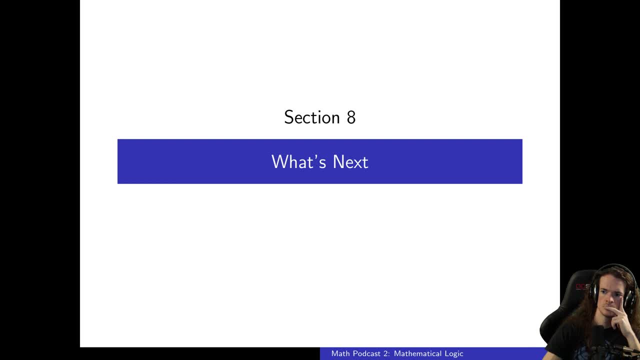 but it talks about how this aspect of logic, which says you can talk about statements that are true and you can talk about statements that are provable, Doesn't always mean the same thing. So it is the case that if you prove something to be true, 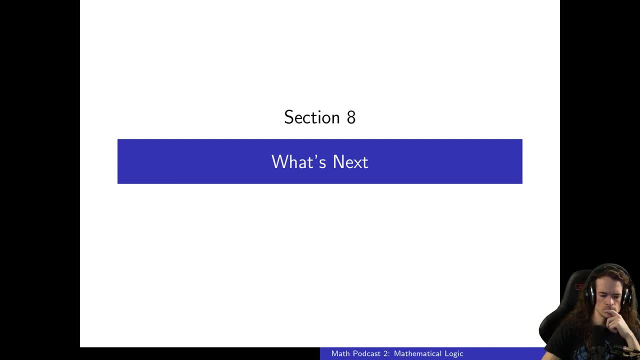 it is true, But there could be statements that are true that you can't prove to be true. Just going to have to take my word for it, Okay, So this is a deep statement. This is not something I'm going to justify. 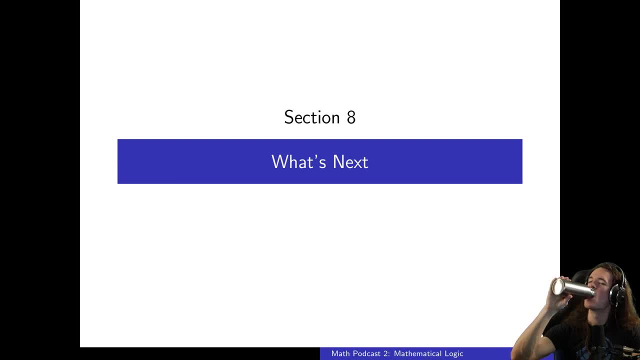 But the fact that that's the case and the fact that there's a difference between the notion of truth and the notion of provability is like at the heart of this, And it's also deeply connected to this, this notion of what it means to be able to solve something on a computer. 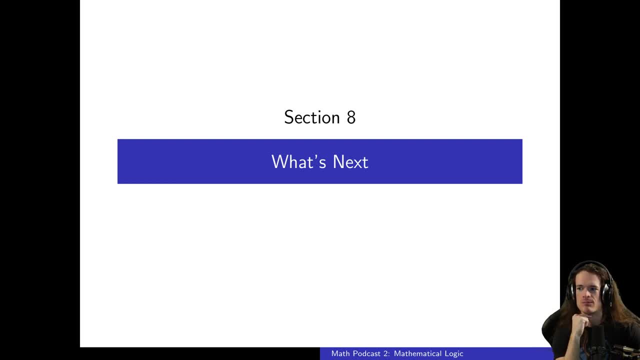 And the thesis is that what we can solve on computers is what can be solved in general. So the idea that there could be things we can't prove or there could be problems we can't solve, It's really like a if you believe that essentially computers represent what we can do in our 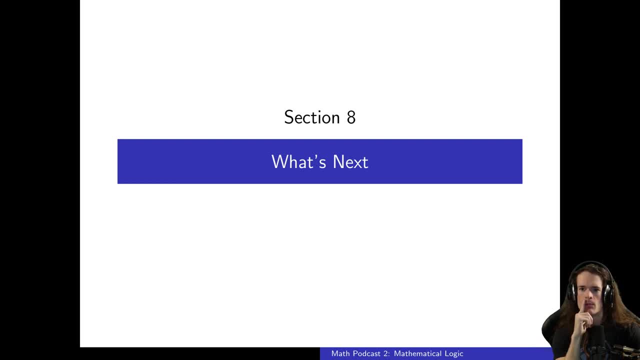 brains like the computers are sort of like a, are mimicking the kinds of thought patterns we're capable of, then these problems are impossible for all of humanity, And they're. they have interesting philosophical ramifications, And so it's a, it's a deep. 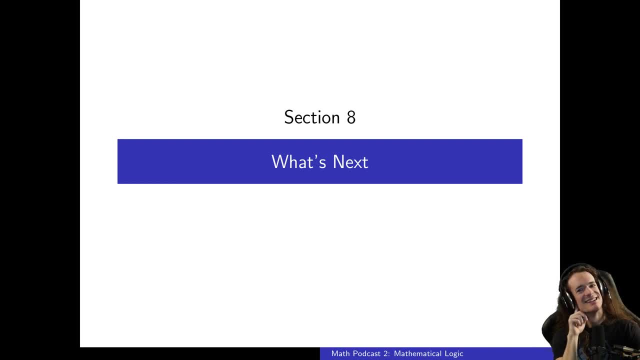 interesting topic involving things that you can't solve with a computer and things that are are not possible to be done using proofs and logic, And I understand why people want to hear about this, because it's it's. it touches on like philosophy and like the nature of things. 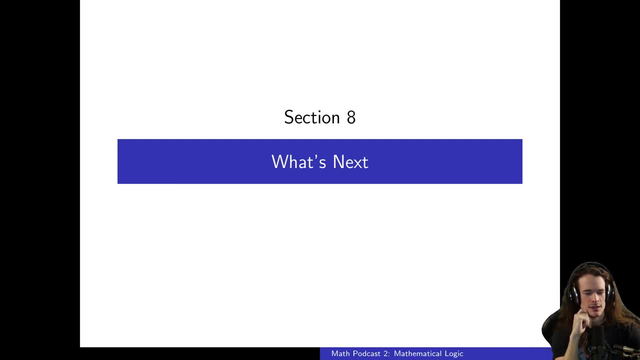 but it. but it can get a little technical and deep. A set of problems, impossible for all of humanity But easy for a Protoss child. All you have to do is keep hitting the C button and the carriers just pop out and just take out everything. 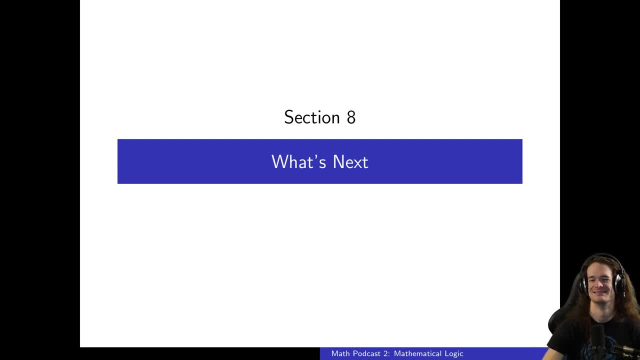 I think the bias is coming through again. Yeah, Yeah. Well, we're aware of our community base. We've got a bunch of nice Starcraft people. Some people saying: what is this? This is confusing. Other people are like: 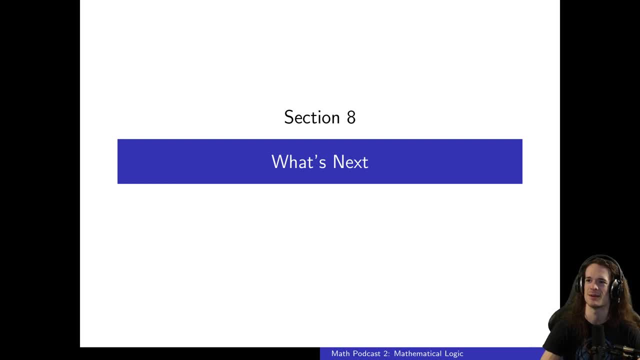 this is amazing. How do a Zerg and a Protoss, how do a Zerg and a Terran come together and become friends? Talk about Protoss, Yep. Ah yes, we found some common ground. Well, awesome So. 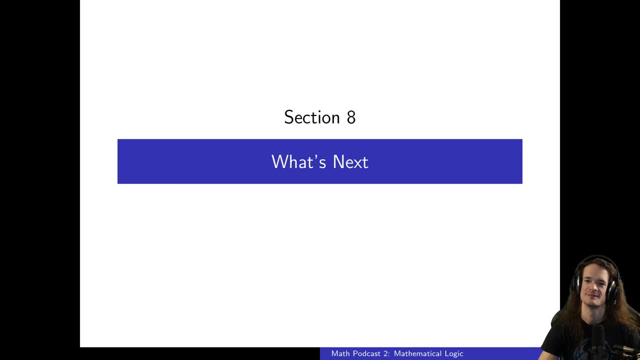 yeah, And so well. thank you for the suggestions, and maybe I really like your idea about the kind of- not fallacies but the biases that humans have, and like how you can look at certain problems. They seem to have obvious answers, but then you have to be wary of these. 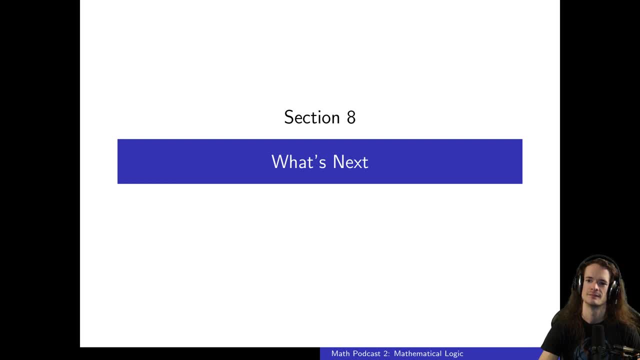 these loopholes that we kind of weren't evolved to solve. So evolution didn't teach us to become probabilists And as a result, we look at some situations that come up in everyday life and we just have the wrong, the wrong intuition and try to fix those biases. is 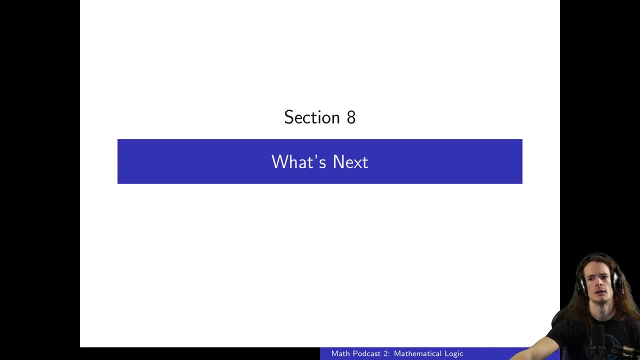 sounds like a good idea. So devoting some time to that, Yeah, And and yeah, maybe talking about poker or maybe things with the current wow or and there's a lot of other games that people play that involve problems, So we can. 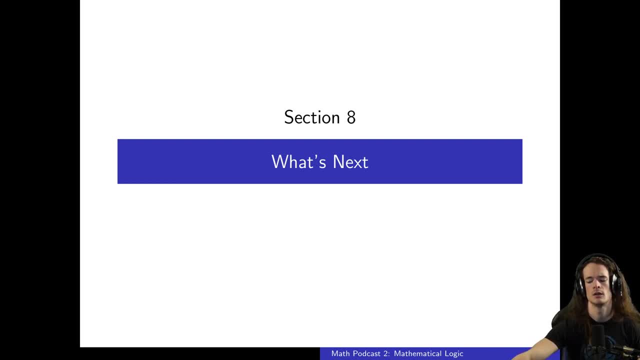 we can. we can dive into that, but lots of ideas and we'll think about what to do, What would be the ideal route for someone to contact you if they had a question. So I keep an eye on, even though I haven't typed a lot yet. 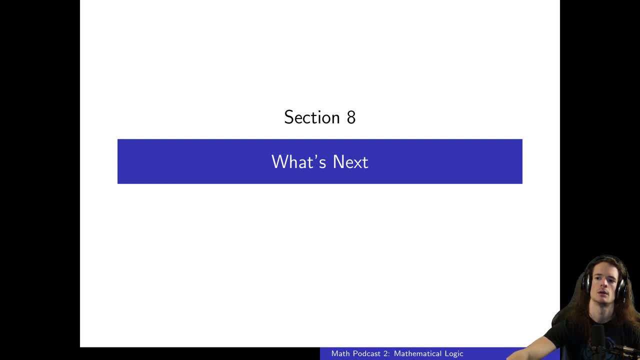 I keep an eye on your discord MathChats channel, So you created one Yep- That's very nice- Where I think you put the slides from this chat. So I will go there and if someone wants to ask questions, I will. 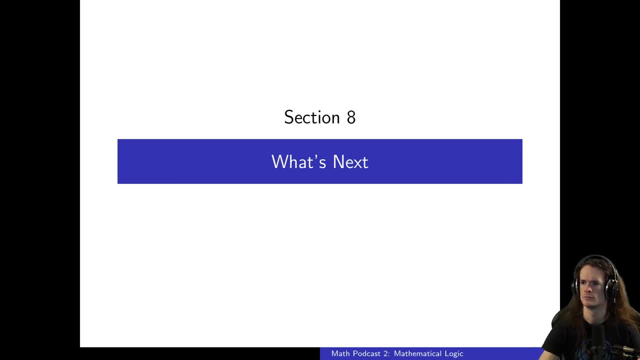 I will answer them there. I think I will go there And I think I will also. I could also in that discord channel put a a Gmail account I have just for this podcast, which I think I called Brett Mathcast, at gmailcom. 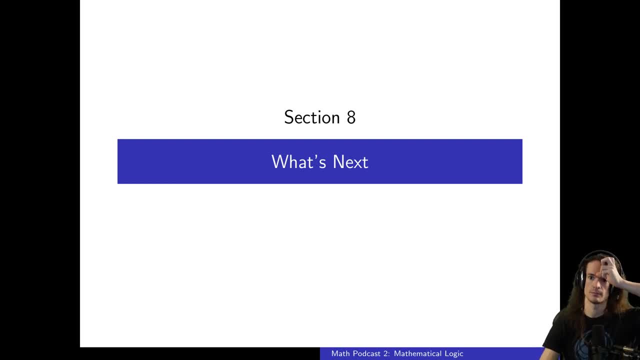 Cool, I can pin that as well, So it stays. Let me just let me double check. I'm not giving away some random it's. it is exactly right. Brett Mathcast at gmailcom. So you, if you email Brett Mathcast at gmailcom? 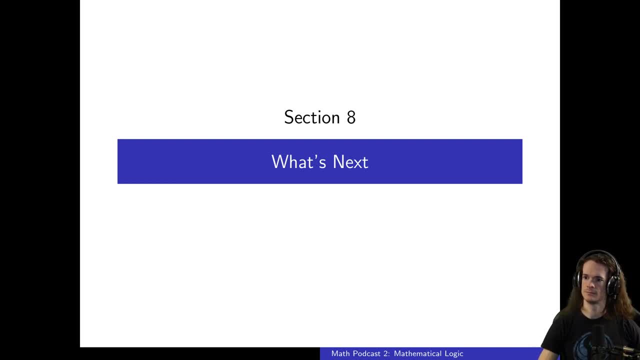 I will. I could also try to answer them. Unless I get a deluge of questions, I will try to do my best. So so at this point, do we have, are we like mandatory have to talk about science and technology now? 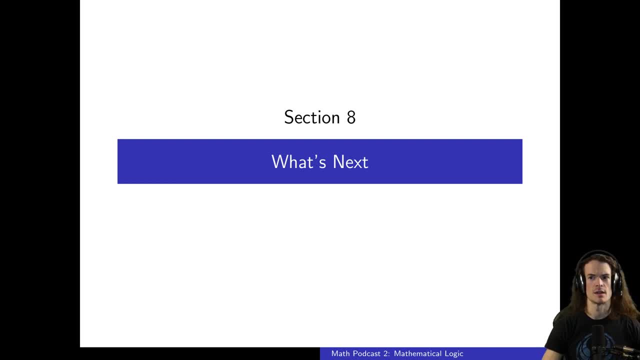 No, there wasn't a specifically mathematics question. No, there wasn't a specifically mathematics category, So this is the closest that we could get, I think. Well, I did talk about robots, You did, And we talked about Protoss units. 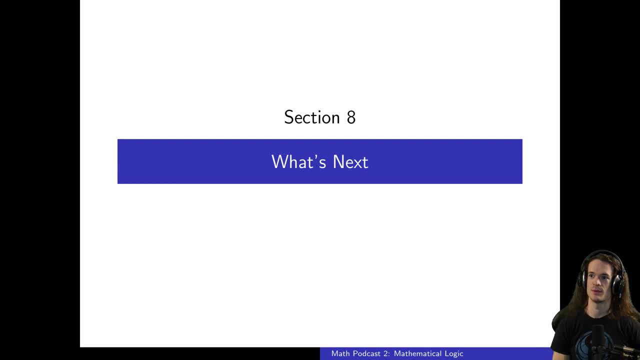 That's not pairing things, which is technology. So, absolutely, We get a pass here. We hit all the bases. Yeah, we did it. Yeah, There may be a referee who's like seeing if we're over the line or not. 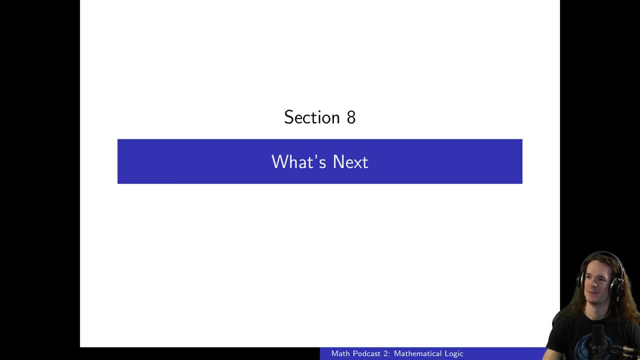 but I think we're solid, I think we got it. Yeah, Yeah, absolutely Well. it's very fulfilling for me to be able to share this kind of content with people on Twitch. Thank you very much, Brett, for bringing this up as your idea. 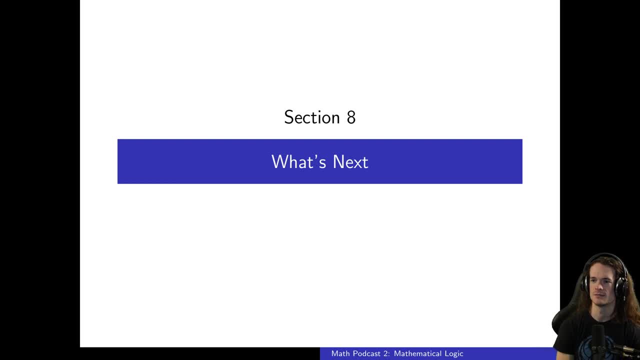 basically of getting this knowledge and wisdom out there. My pleasure And thank you for having me, And thank you for being such a a great host and someone who just amazingly intuited the slides before they existed each time. It was really amazing. 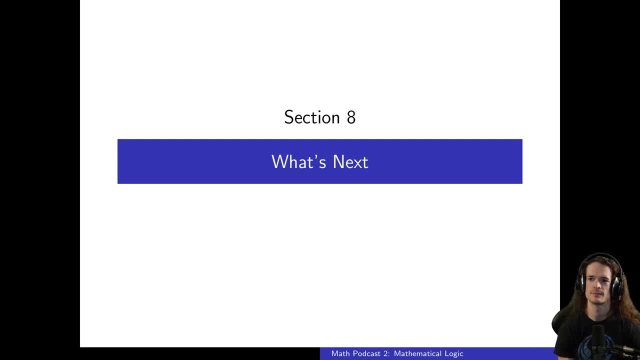 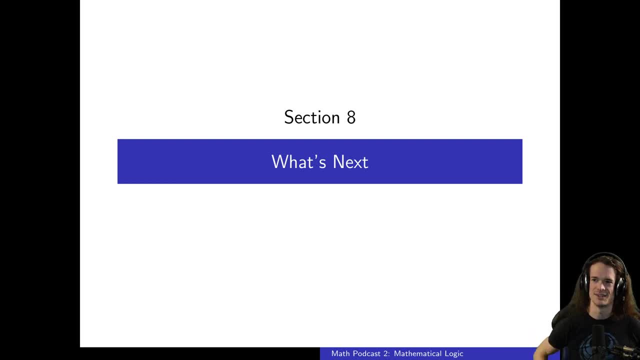 Yeah, Yeah, Yeah, Yeah, Yeah, Yeah, Yeah That's. that's pretty cool And thanks. Thank you for your time today, Matt. Really fun time. I hope everyone liked it, hope it was educational and interesting And maybe we'll try to continue this trend. 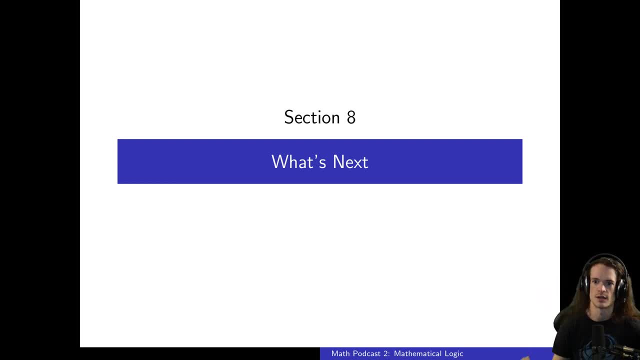 Yeah, I like the interaction with the chat as well, where you give some multiple choice- Some people can guess at that- or you give a open-ended question and they can try their best for it. Yeah, Yeah, Yeah, I know the. I know they got a little tricky at the end. 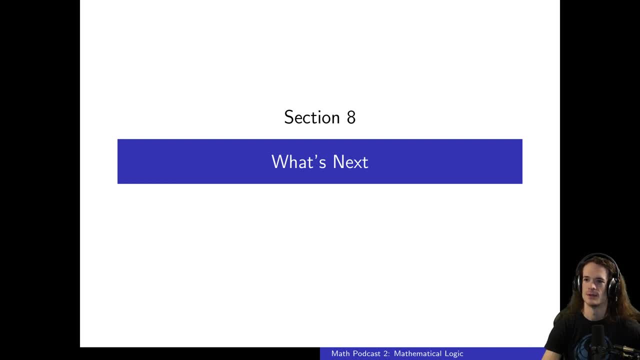 We, we, we know that and that, but, yeah, the chat was great form, and also on youtube. youtube probably the best avenue for these because we do have a good bit of visual through the slides. the slides were posted to the math discord channel. 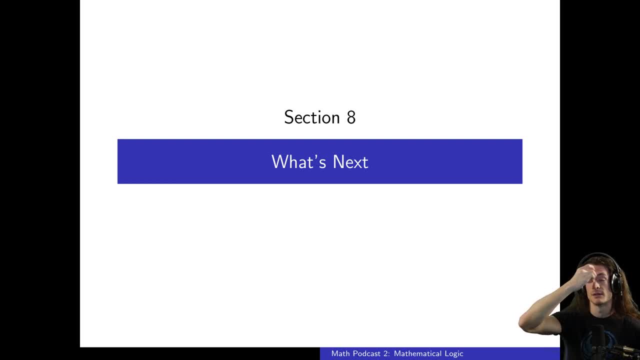 if you want to contact brett, you can do so there. he's going to put his email in that area. thank you so much, chat, for your interaction, your viewership, your interest in this kind of content. thank you very much, brett, for giving us your knowledge and expertise and leading. 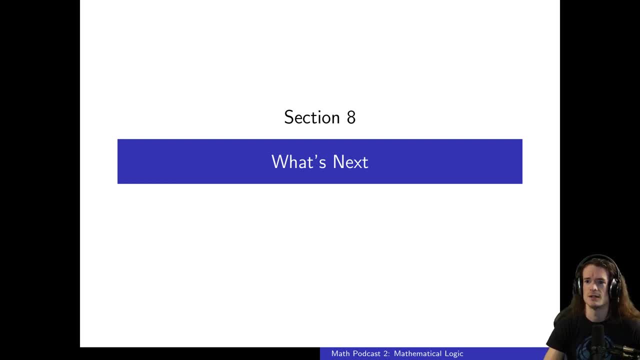 this discussion and we will see you on math lecture number three coming up- exciting. thank you, brett. very welcome and thank you for having me boom recording stopped. let's see upload. and your upload is good sir, sweet, superb. so this will be. oh yeah, i got the you're all done message. 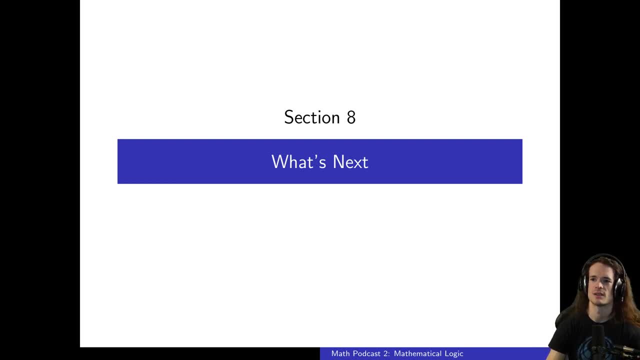 oh wow, mission accomplished. yeah, the previous ones, i think we did wave files which take longer to upload, but these mp3s are done pretty fast and it seems like, yeah, that was, that was instant. yeah, also, i was worried about the uh smoothness of the uh slide transitions because that was. 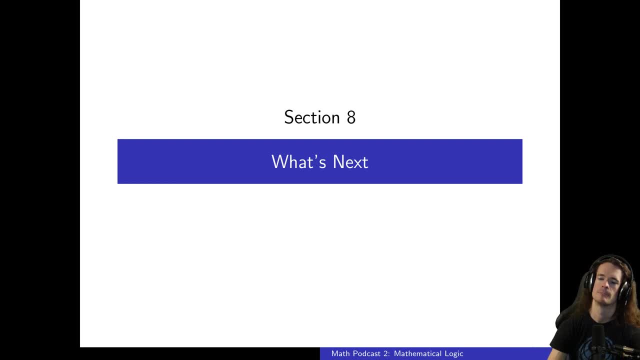 neuro doing all the slide transitions and it was spot on. well done, yeah, i'm- i'm like the try hard kid in the front of the class who's like paying super close attention and yeah, if i'm not paying close attention then the whole lecture gets bogged up. 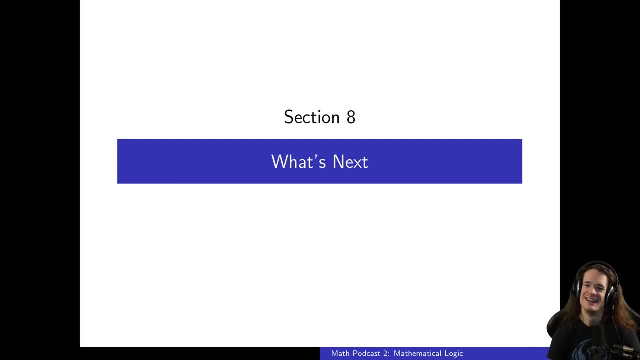 it was like like what are the- uh, the other uses for apm outside of starcraft? they're like bam bam, hit those slides. well, yeah, that was amazing. i, i was, i was, that was, i was stressing about that. i was like, oh, there's gonna be so many slides and he has to always switch and has to be. 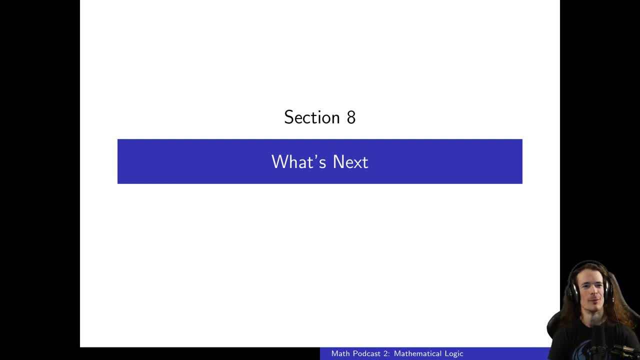 seamless. and then you were just on point. i'm not a noob dude, come on. yeah, i've had the full range of class experience from my university career. some of the classes i'm like not attending or i'm way in the back and kind of distracted. but then for certain classes where i would feel really amped up and engaged and i love 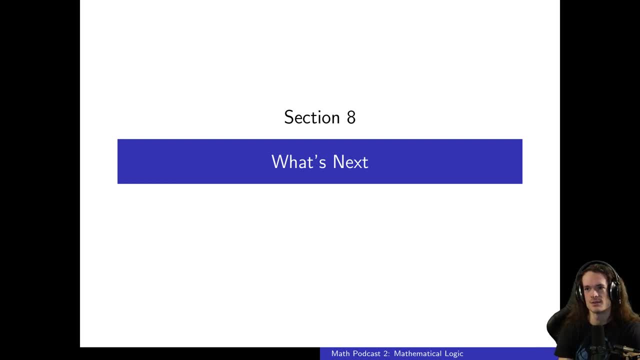 the material. i'm like in the front full try hard answering questions and trying to be plugged in. that was part of me switching to cognitive science from psychology- the psychology classes i was in. they didn't really connect with me in the same capacity but i took the first cog psych course and 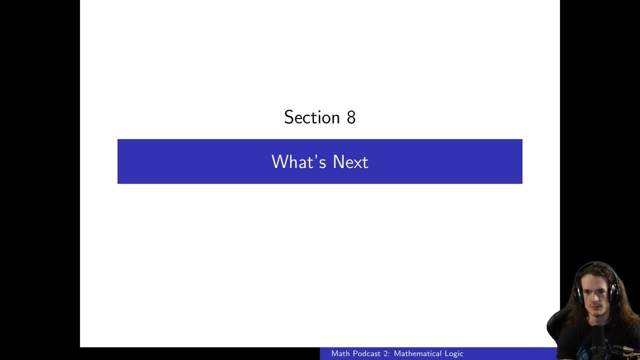 it was like a real one across the board, so for me that was like a really good experience. yeah, that was awesome this class, because i'm having so much fun with it. yeah, motive: yeah, finding something you love means it means means so much, yeah, i mean, yeah, i had friends that had different tricks with this. 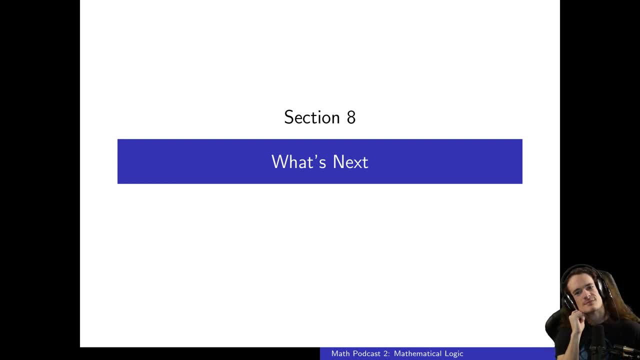 because, like i had some, i had a friend who- and we had this on tape, because you know that you go to classes and they tape the classes and she, uh, she would fall asleep in almost every class. on tape we'd see her, we'd, yeah, we'd see her falling asleep in the class like, oh, there she. 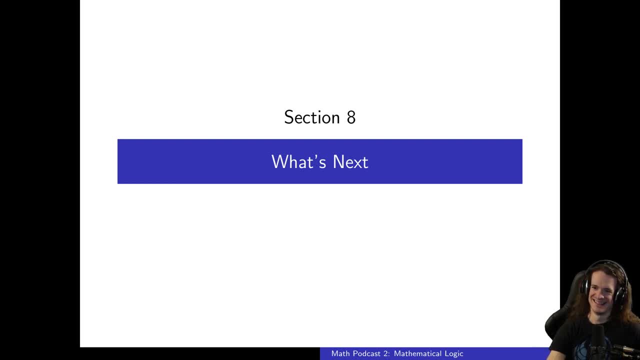 is: yeah, oh, she's looking at the professor. oh, no, not anymore. oh, sleep time. right. so, and then her trick was to, uh, to just take careful notes, like she was like writing a book and and like she was like the scribe for the class and like the event, the, the action of trying to take the best notes. 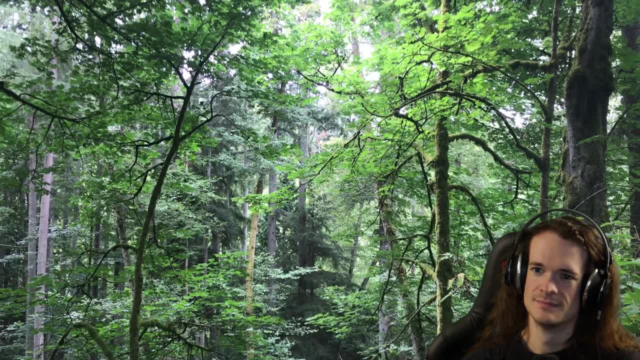 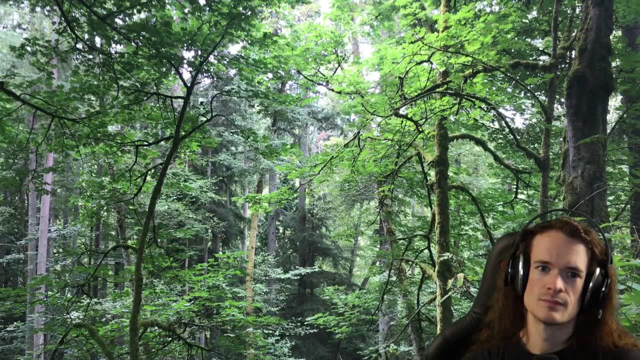 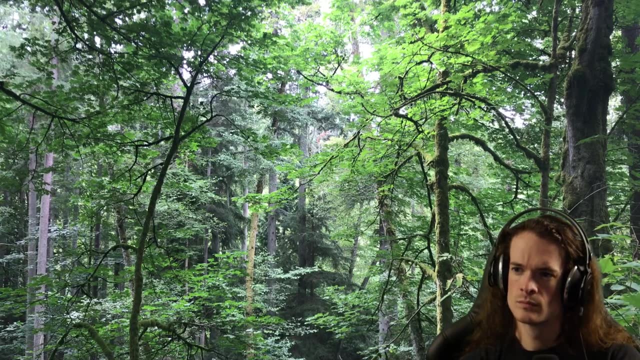 possible kept her like awake and alert and amazed: oh are we getting a linear i? i? i'm happy to do linear algebra. i know one. one reason that linear algebra is cool also is i could, i could give an introduction to linear algebra and then sort of connect it to how neural networks work. so that might be something. 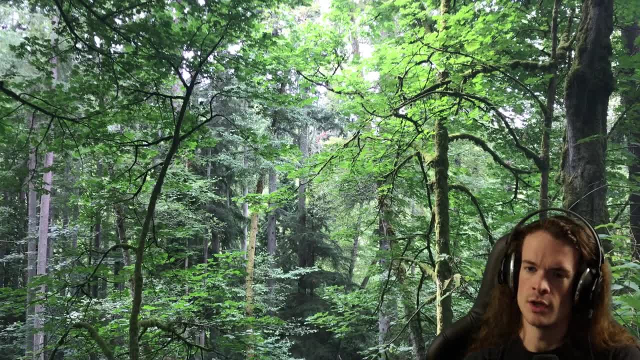 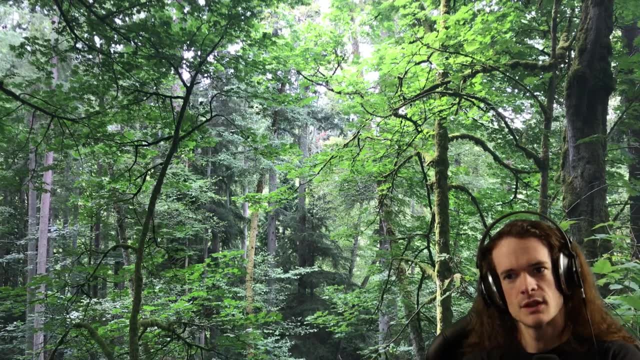 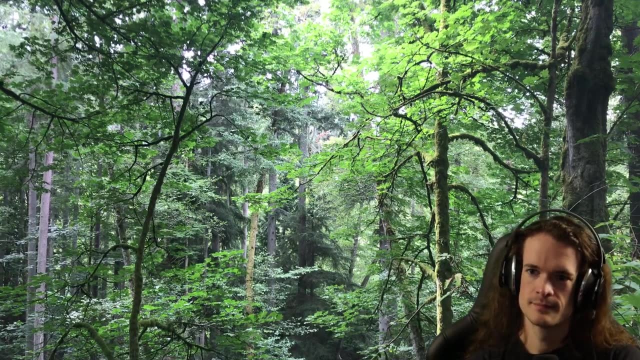 cool because neural networks- firstly, your name is neuro, yeah, um. secondly, people are like: oh, neural networks, robots taking over. i want to understand them. linear algebra was a pretty fun class, yeah, so that could be a definitely good choice for another topic. i think about the best way to